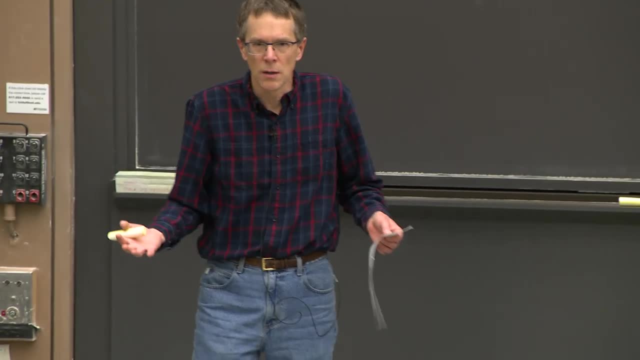 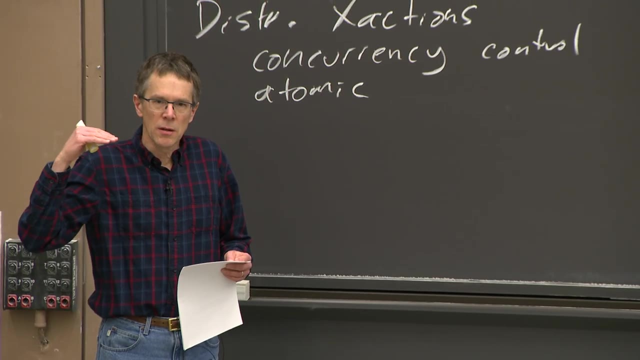 millions and millions of articles. half the vote counts are on one server and half the vote counts are on another. But some operations require touching, modifying or reading data on multiple different servers. So if we're doing a bank transfer from one customer to another, well, 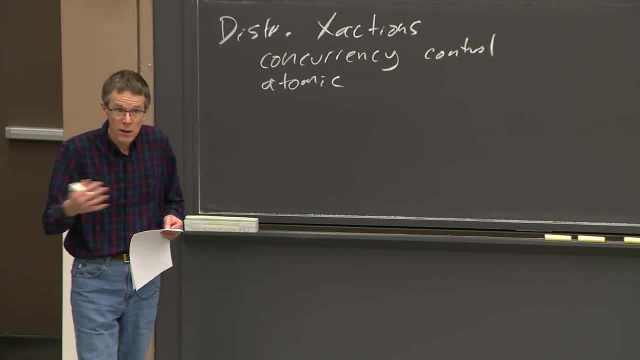 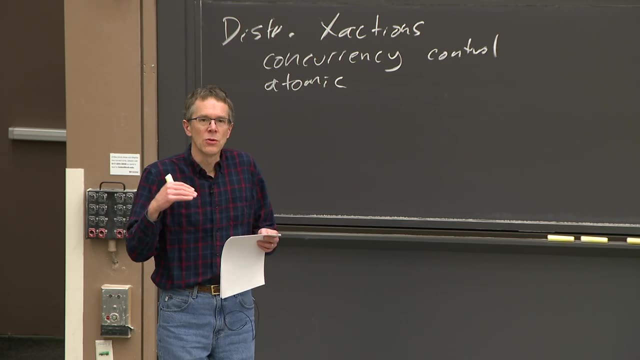 their balances may be on different servers And therefore, in order to do the balance, we have to modify data, read and write data on two different servers, And we'd really like to, or one way of building these systems, and we'll see others later on in the course. 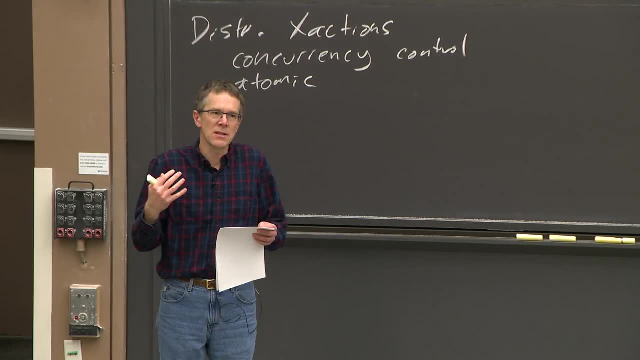 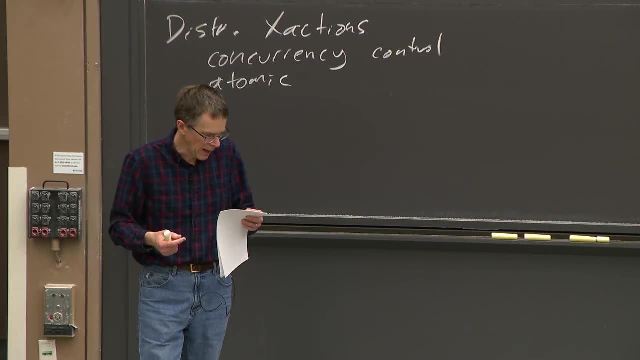 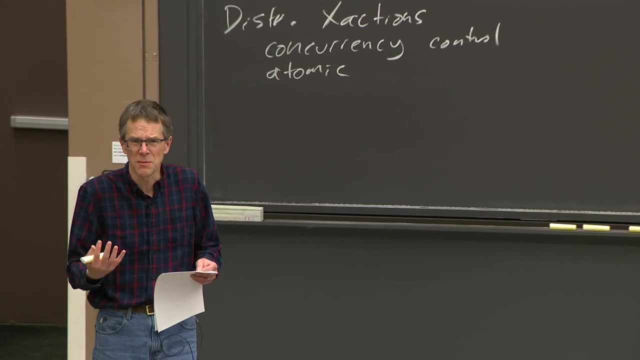 one way to build the system is try to hide the complexity of splitting this data across multiple servers. try to hide it from the application programmer, And this is like a traditionally has been a database concern for many decades, And so a lot of today's material originated with databases, But the ideas have been used much more widely. 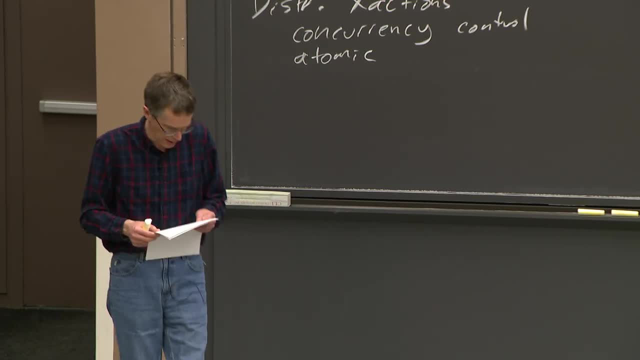 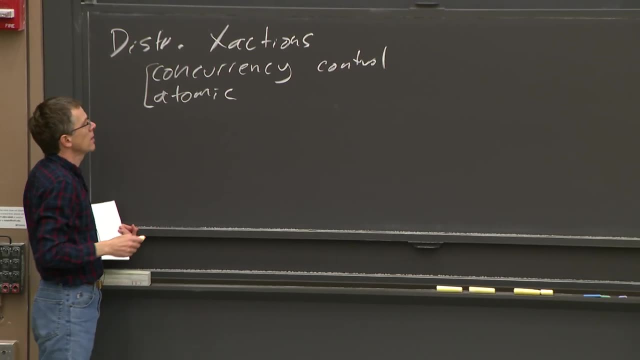 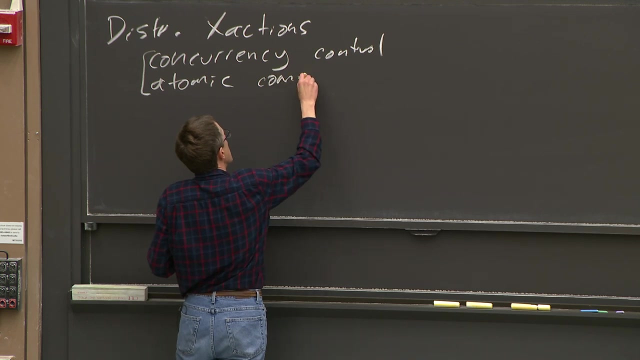 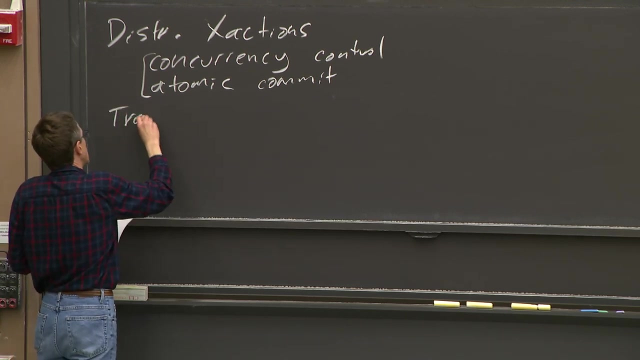 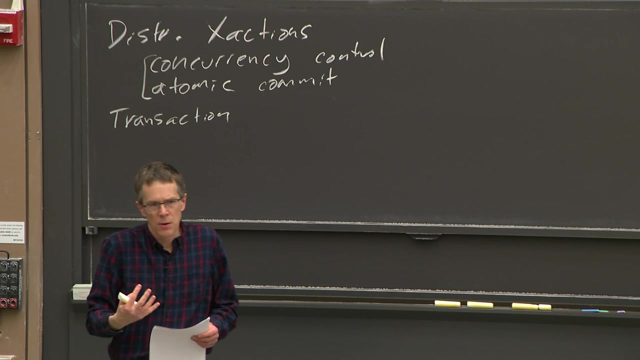 in distributed systems which you wouldn't necessarily call a traditional database. The way people sort of usually package up concurrency control plus atomic commit is in an abstraction called a transaction which we've seen before, And the idea is that the programmer you know has a bunch of different operations. 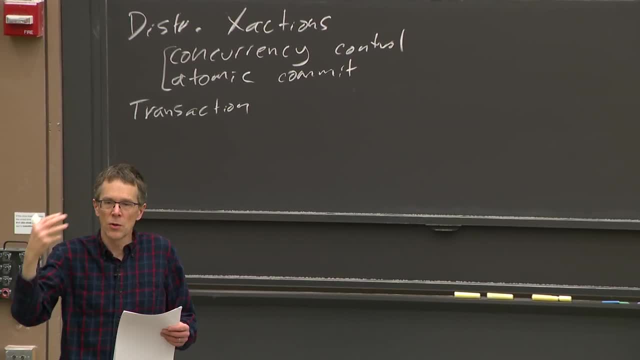 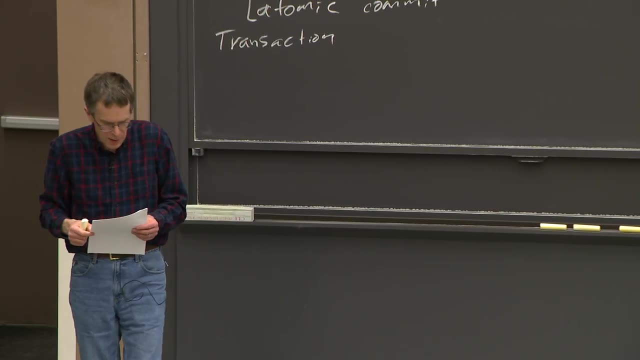 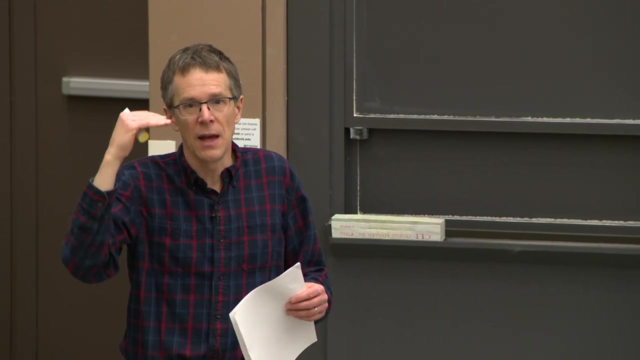 maybe on different records in the database. They'd like all those operations to be sort of a single unit and not split by failures or by observation from other activities, And the transaction processing system will require the programmer to mark the beginning and the end of that. 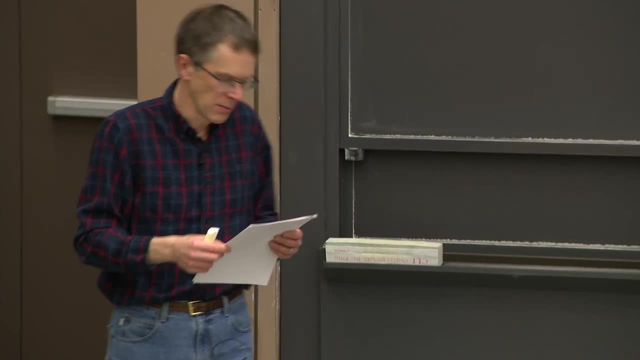 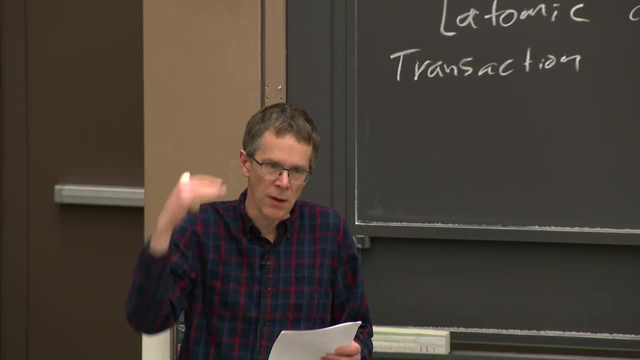 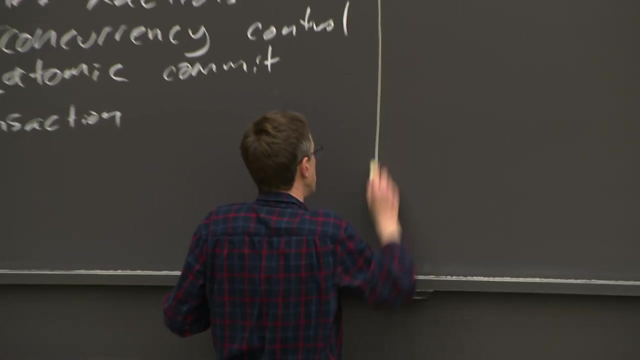 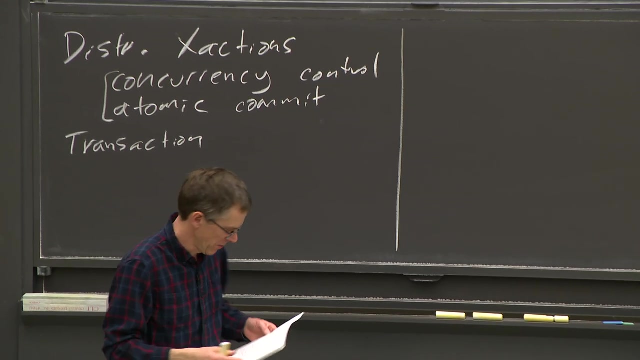 sequence of reading and writing and updating operations in order to mark the beginning and end of the transaction, And the transaction processing system will provide certain guarantees about what happens between the beginning and the end. So, for example, supposing we're running our bank and we want to do a transfer from the account of user X to the account- 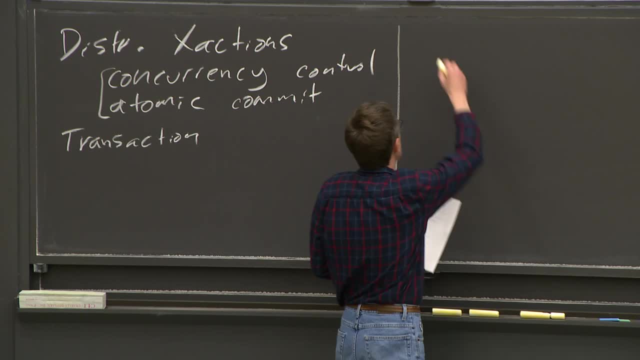 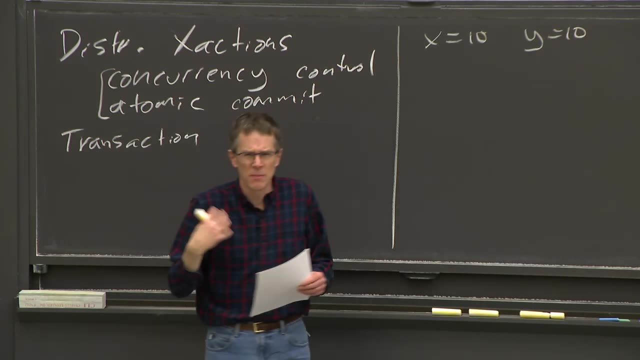 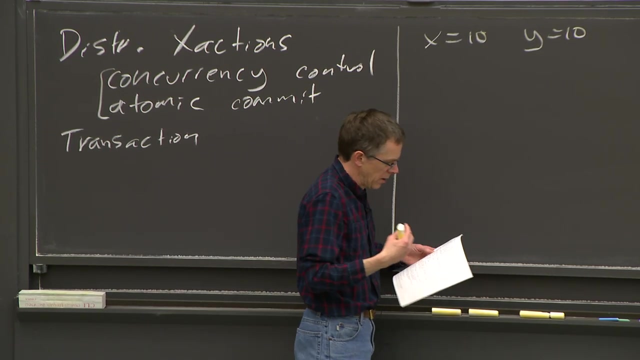 of user Y. Now these balances for both of them start out as 10.. So initially X equals 10, Y equals 10. And X and Y mean to be records in a database And we want to transfer We. 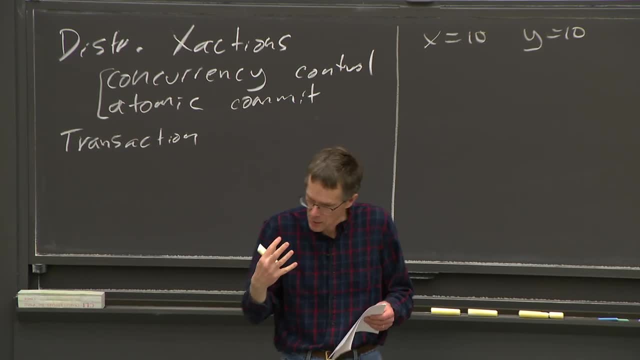 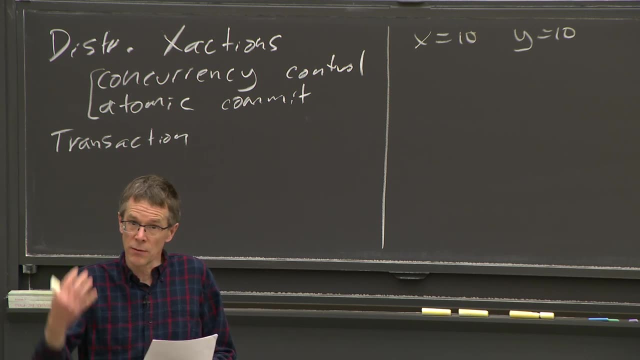 want to actually imagine that there's two transactions that might be running at the same time: one to transfer a dollar from account X to account Y and the other transaction to do an audit of all transactions. So we want to do an audit of all the accounts at the bank to make sure that the total amount 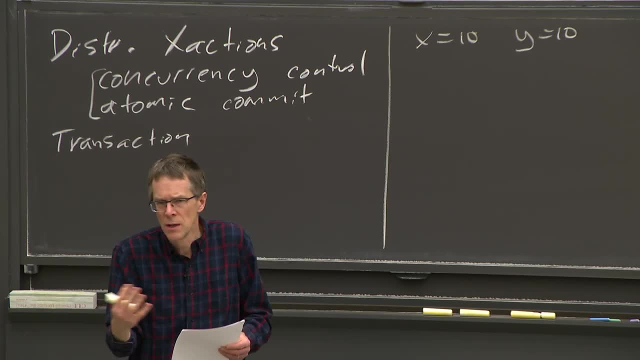 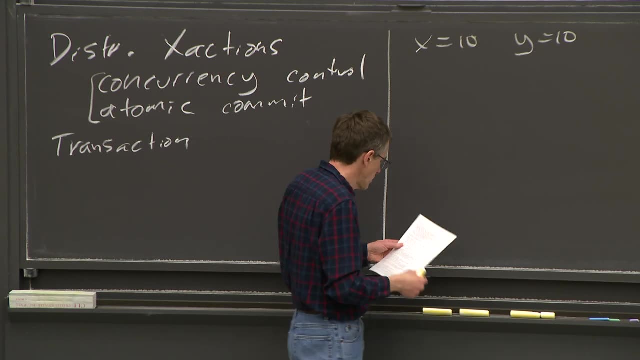 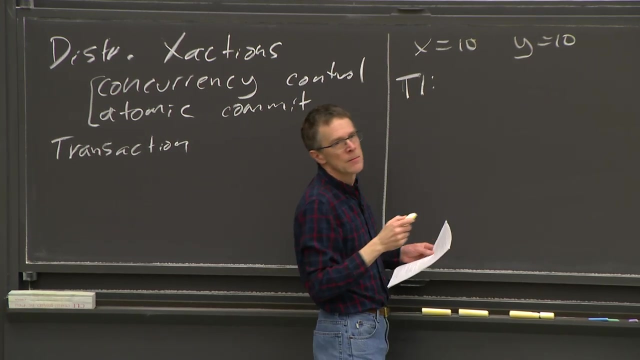 of money in the bank never changes Because, after all, if you do transfers, the total shouldn't change, even if you move money between accounts. In order to express this with transactions, we might have two transactions. The first transaction- we'll call it T1, is the transfer. 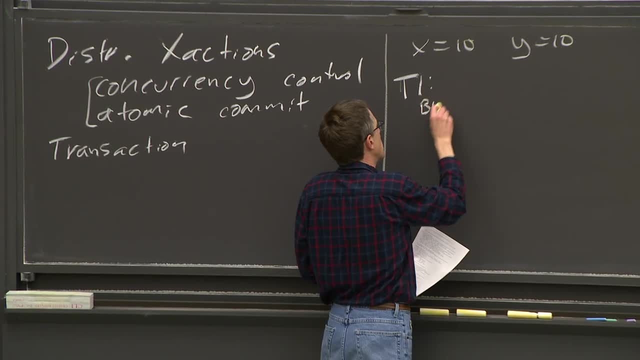 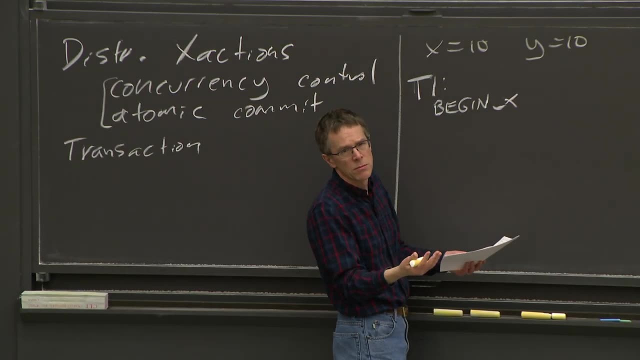 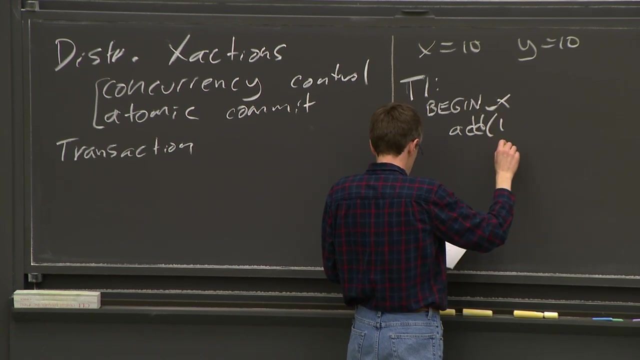 The programmer is expected to mark the beginning of it with the begin transaction, which I'll write as begin X, And then the operations on the two balances, on the two records in the database. So we might add one, might add one to balance X and add minus one to Y. 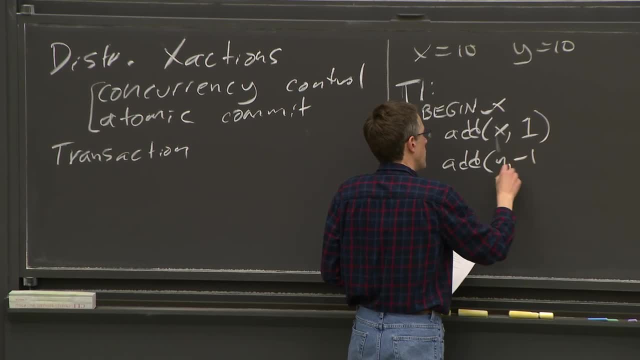 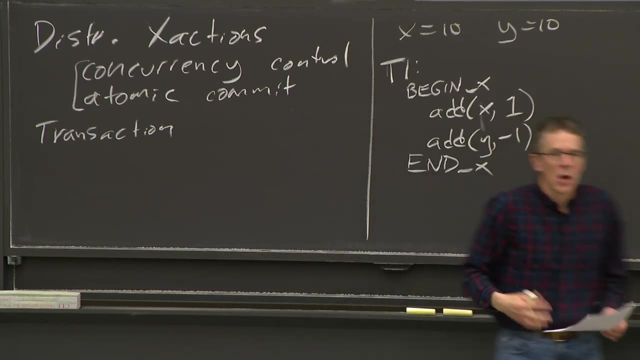 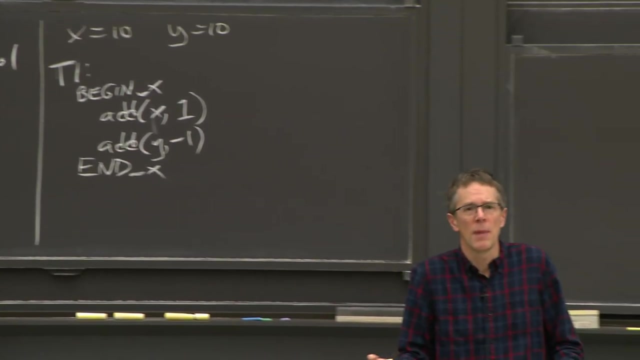 And then we need to mark the end of the transaction. Concurrently, we might have a transaction. check all the balance. do an audit of all the balances, find the sum. or look at all the balances. make sure they add up to the number that doesn't change. 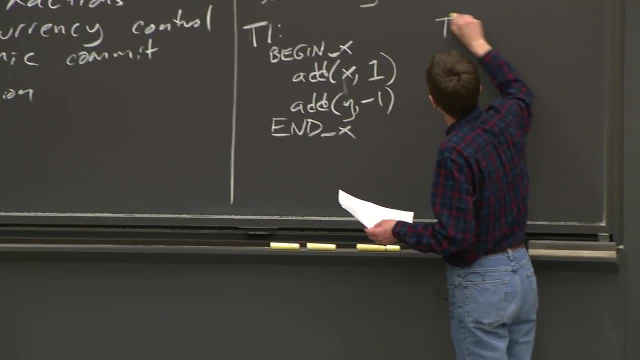 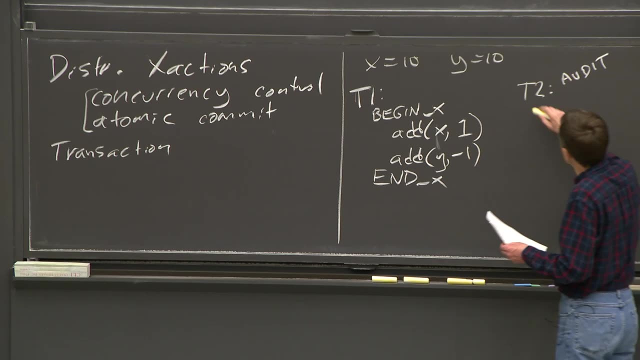 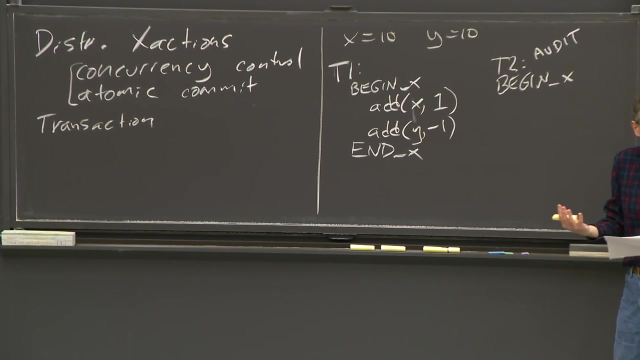 despite transfers. So a second transaction. we have to be thinking about the audit transaction Also. we need to mark the beginning and end. This time we're just reading: this is a read-only transaction. We need to get the current balances of all the accounts. 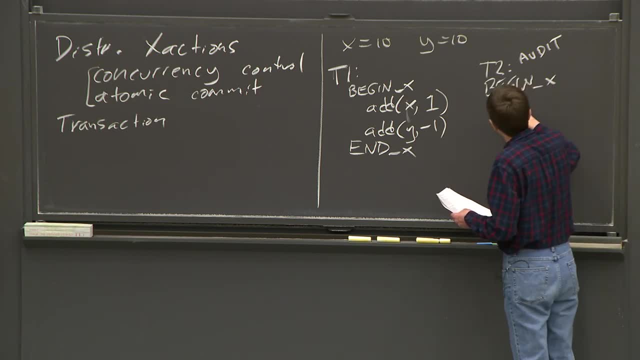 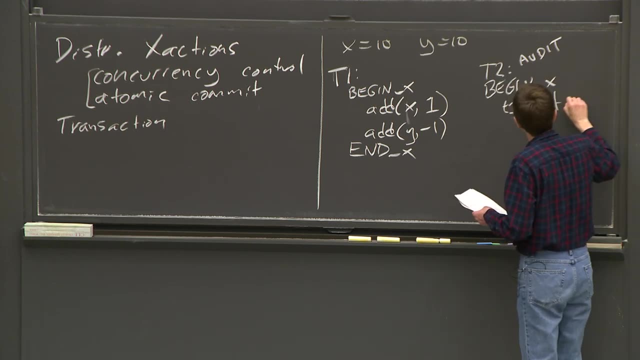 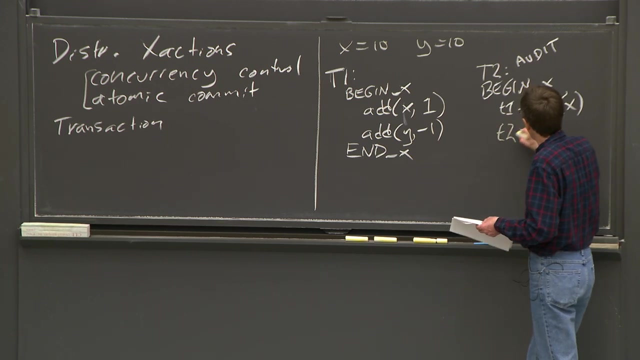 Let's say we're just these two accounts for now. So we have two temporary variables we're going to read. So the first one is going to be the value of balance x. Just write. get to mean we're reading that record. We also read y and we print them both. 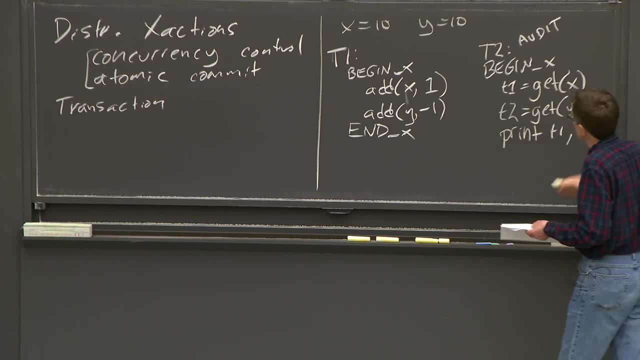 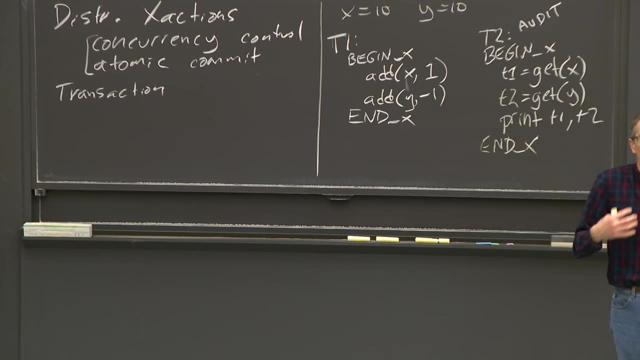 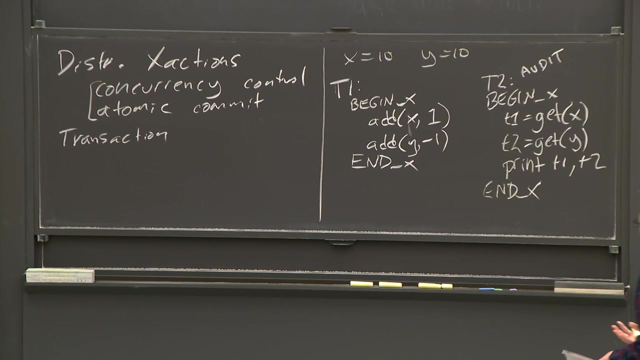 And that's the end of the transaction. And the question is: what are legal results from these two transactions? That's the first thing we want to establish- is what are, given the starting state, namely the two balances for $10, what could be the final results after you've? 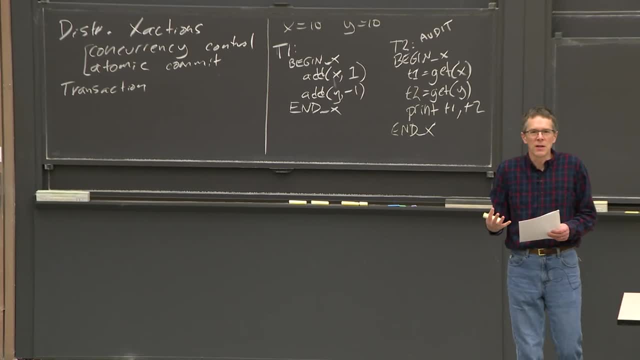 run both these transactions, maybe at the same time, So we need a notion of what would be correct And once we know that we're going to run both of these transactions at the same time. So we need a notion of what would be correct. 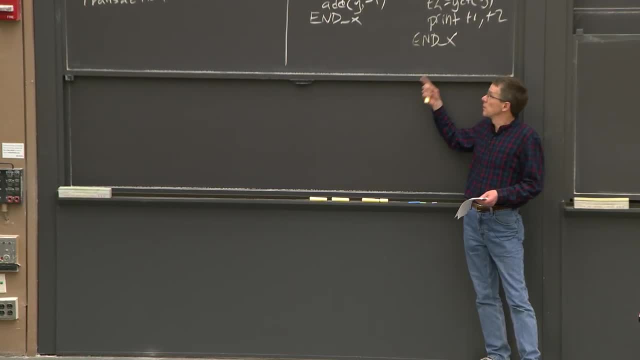 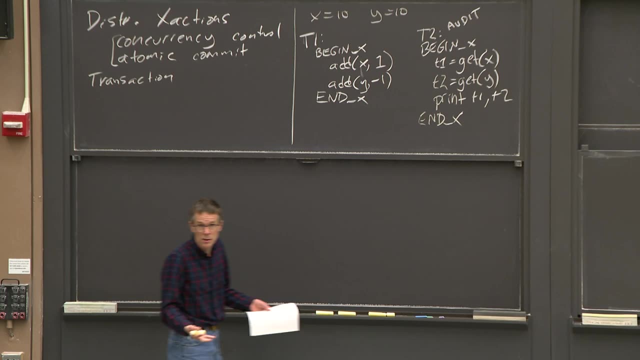 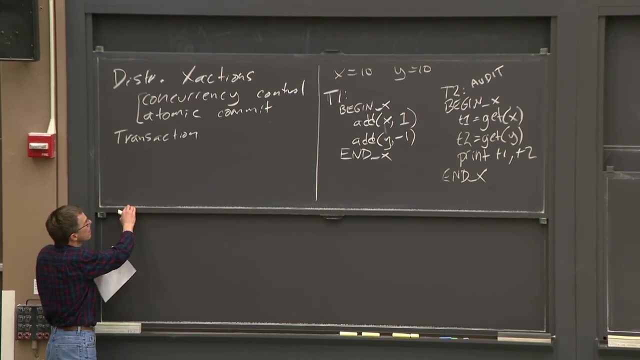 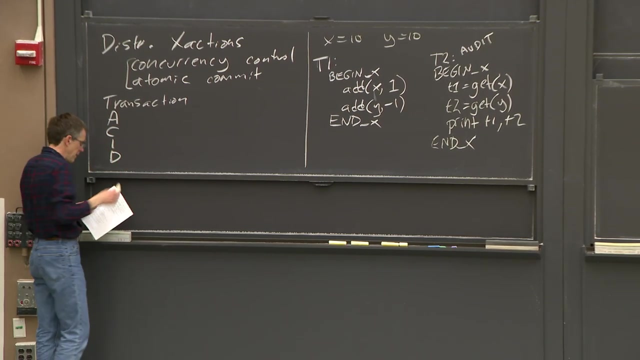 And once we know that we need to be able to build machinery that will actually be able to execute these transactions and get only those correct answers, despite concurrency and failures. So first, what's correctness? Well, databases usually have a notion of correctness called ACID, abbreviated as ACID. 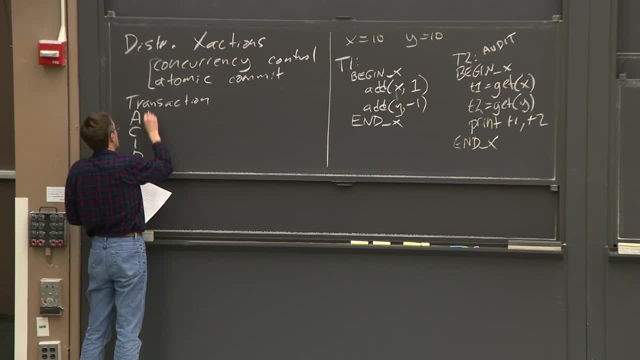 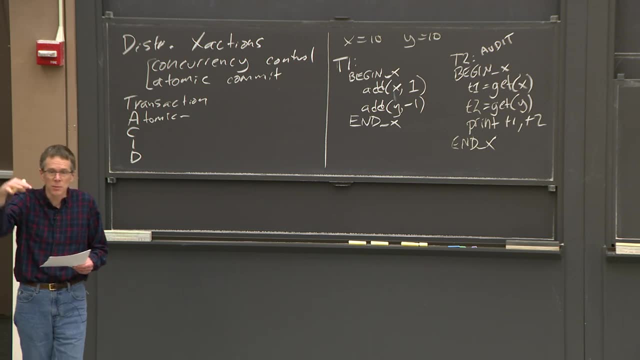 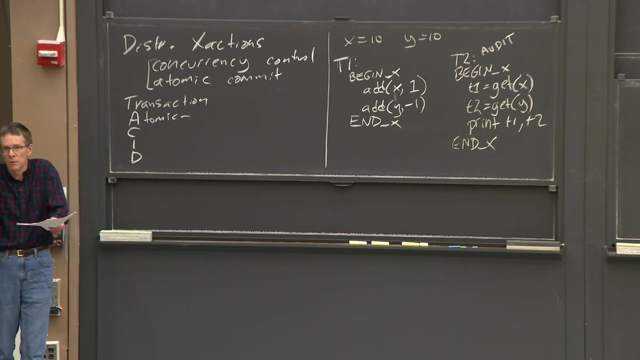 And this stands for atomic, And this means that a transaction that has multiple steps, you know, maybe writes multiple different records. if there's a failure, despite failures, either all of the writes should be done or none of them. It shouldn't be the case that a failure at an awkward time in the middle of a transaction should leave half the updates completed invisible and half the updates never done. 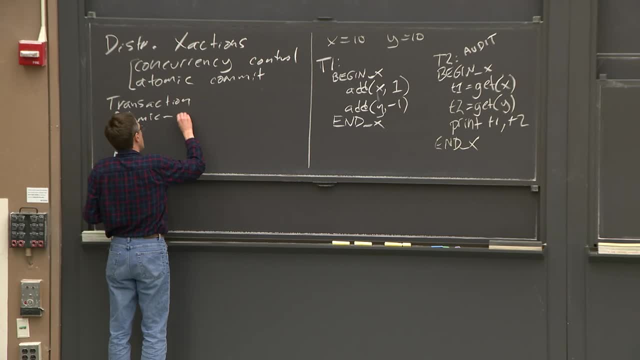 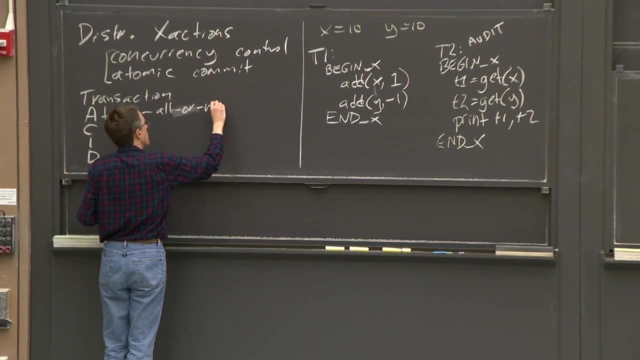 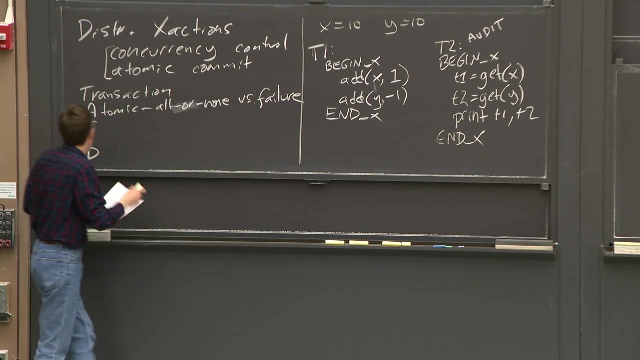 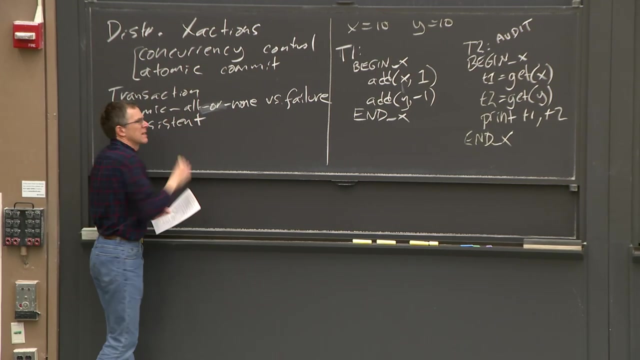 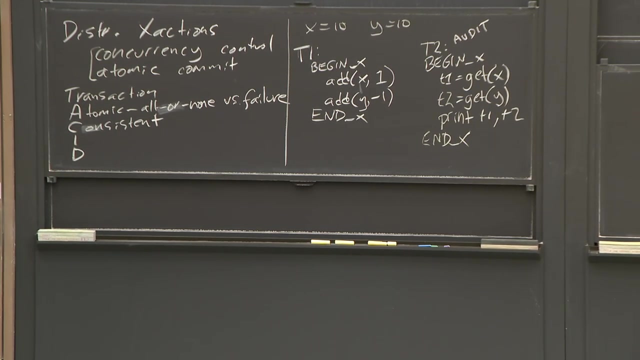 It's all or nothing. So this is all All Or none, despite failures. The C stands for consistent. It's actually. we're not going to worry about that. That's usually meant to refer to the fact that a database will enforce certain invariants declared by the application. 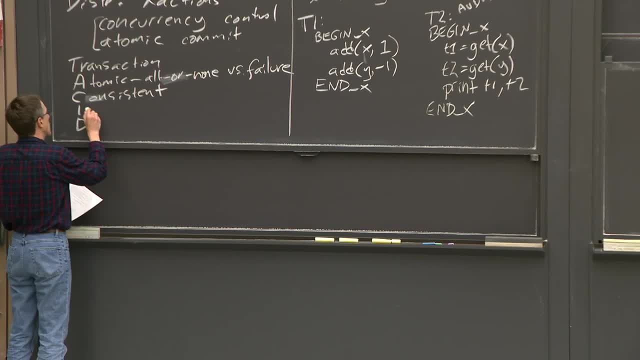 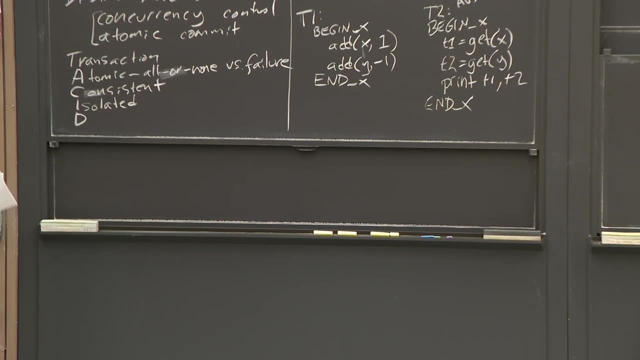 It's not really. It's not really our concern today. The I, though, is quite important. It usually stands for isolated, And this is really a property of whether or not two transactions that run at the same time can see each other's changes before the transactions have finished. 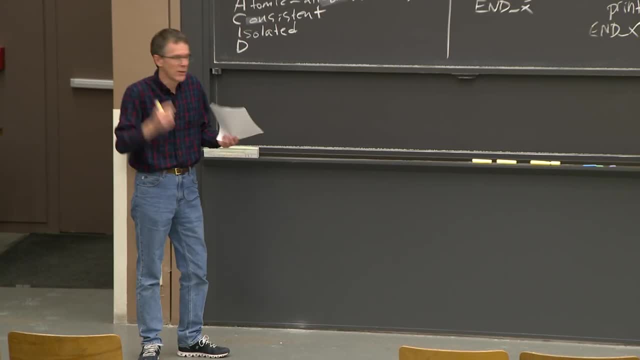 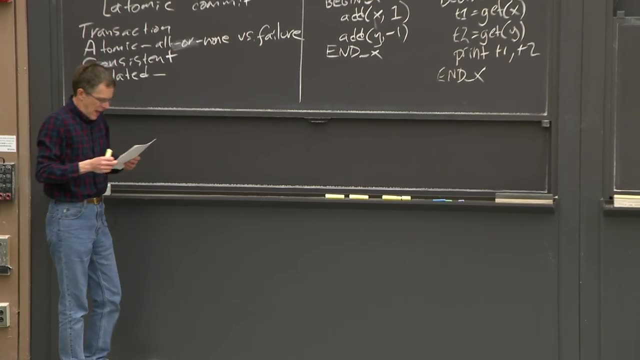 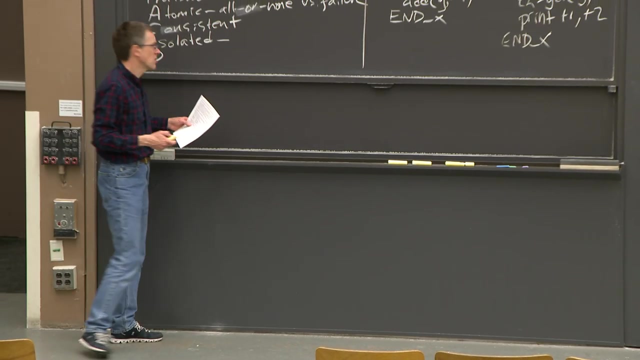 Whether or not they can see sort of intermediate updates from the middle of another transaction. And you know, the goal is no And the sort of technical specifics. And the basic thing that most people generally mean by isolation is that the transaction execution is serializable. 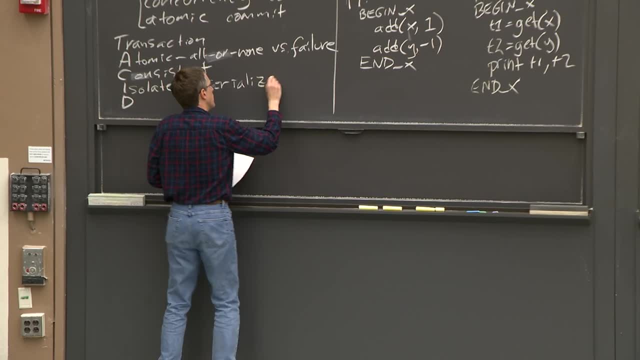 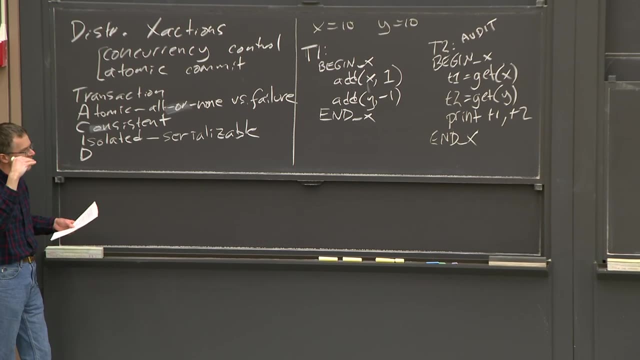 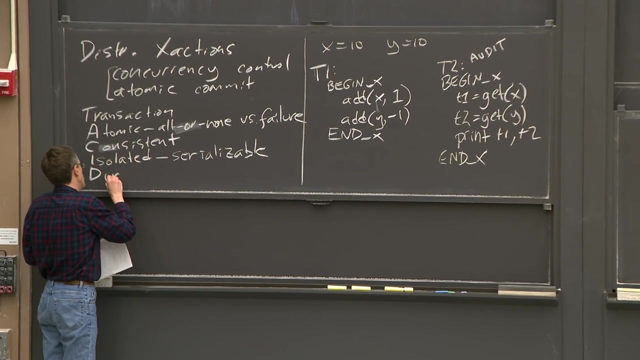 And I'll explain what that means in a bit. But it boils down to transactions. can't see each other's changes, Can't see intermediate states, but only complete transaction results. And the final D stands for durable, And this means that after a transaction commits, 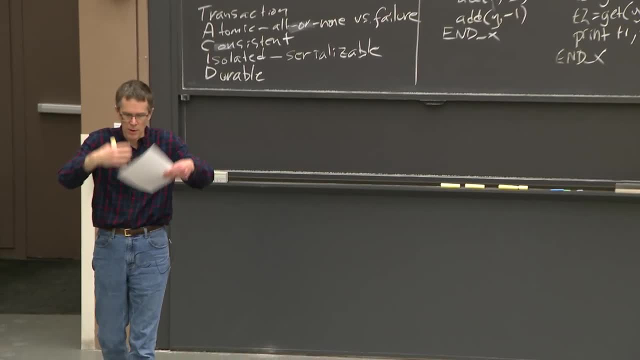 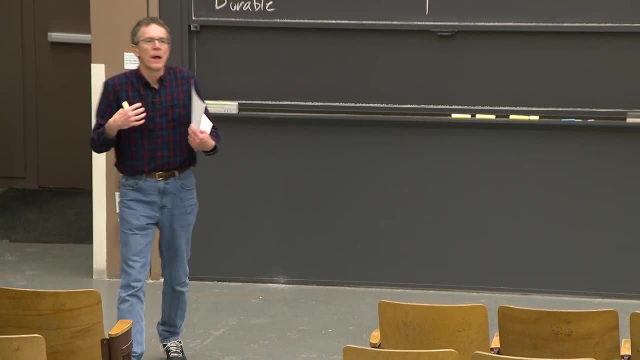 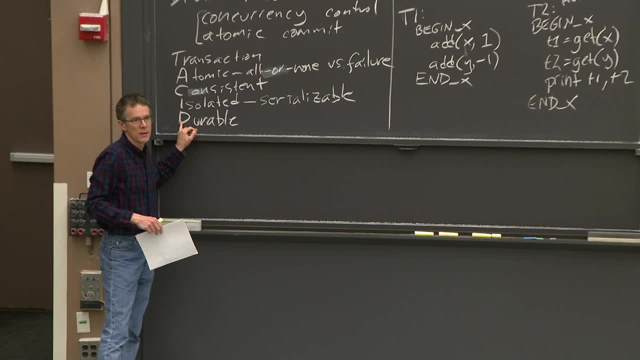 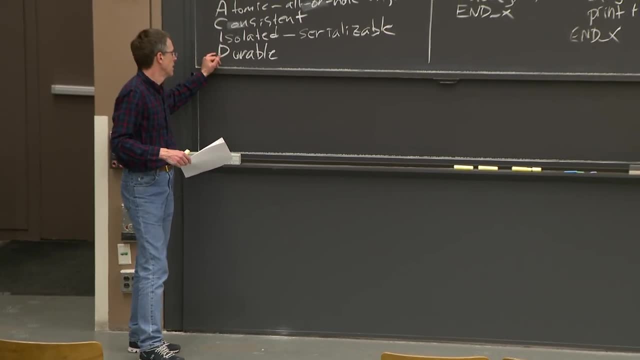 the transaction's modifications to the database will be durable, that they'll still be there. They won't be erased by some sort of failure, And in practice that means that stuff has to be written to some non-volatile storage, persistent storage like a disk. And so today, 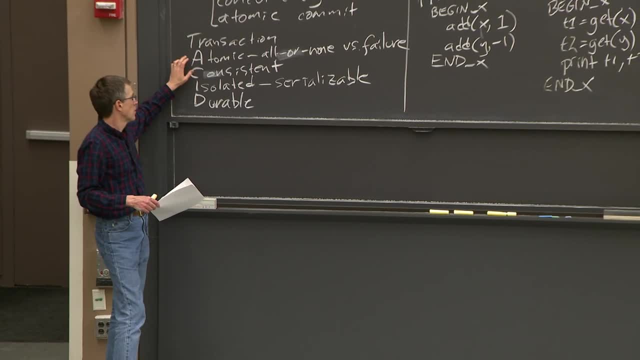 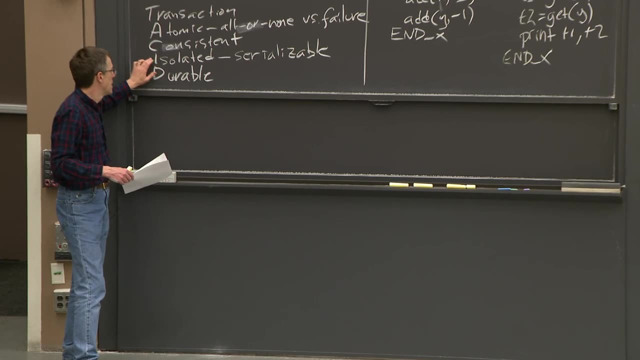 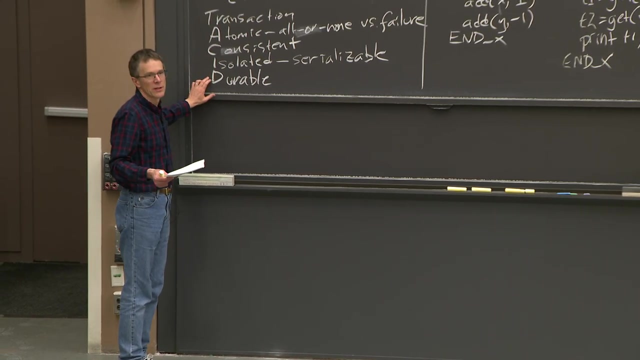 our, in fact, for this whole course. really, our concerns are going to revolve around good behavior with respect to failure, good respect, good behavior with respect to other multiple parallel activities and making sure that the data's there- still there after even. 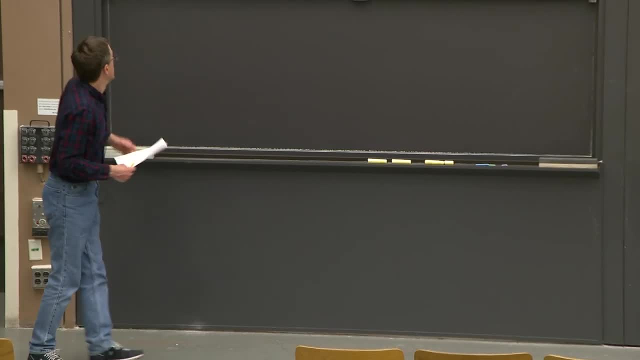 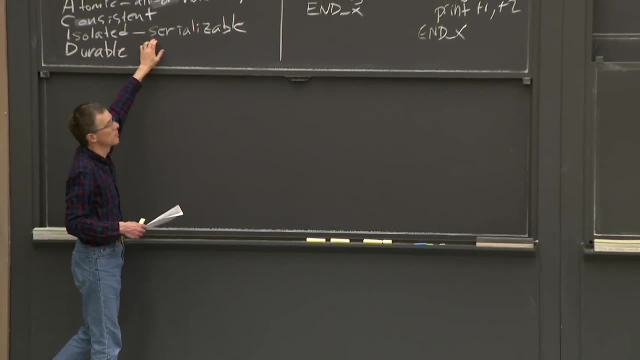 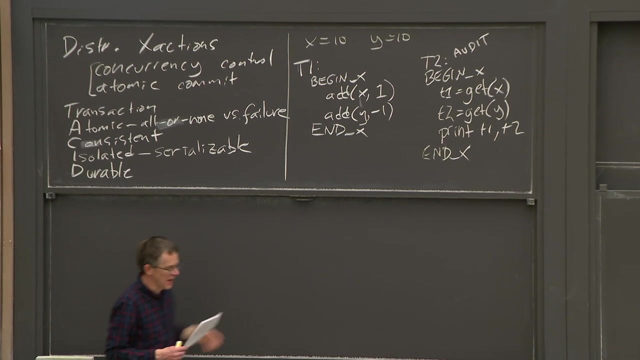 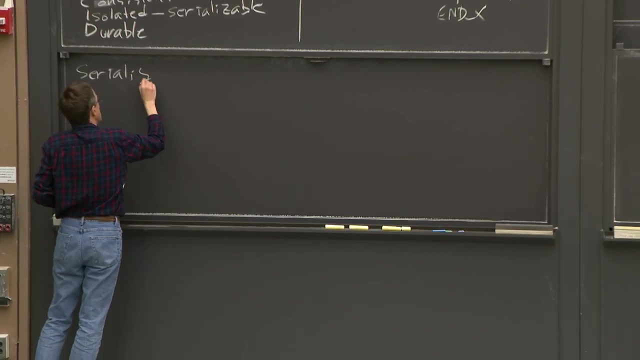 if something crashes. So the most interesting part of this for us is the specific definition of isolated or serializable. So I'm going to lay that out before talking about how it actually applies to these transactions. So the I in isolated is usually means serialized. 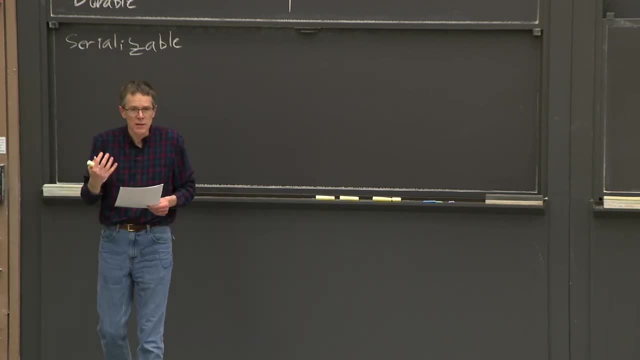 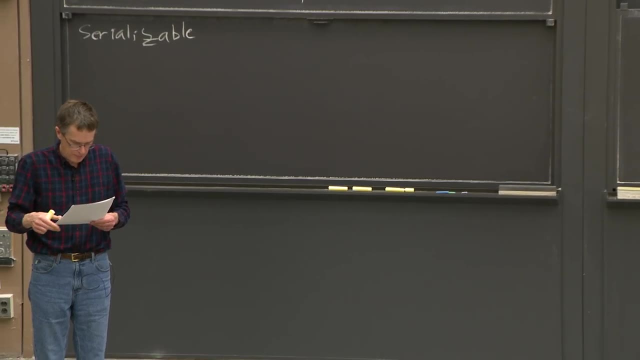 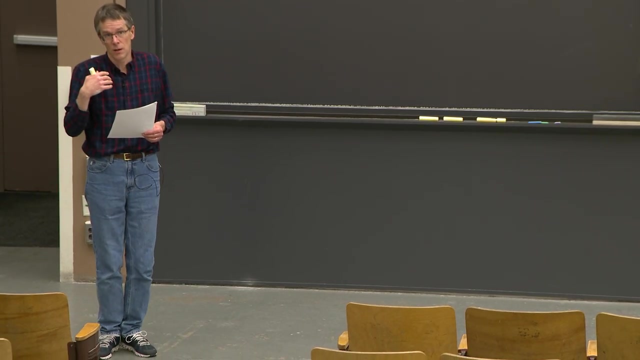 And the definition for this, if a set of transactions executes concurrently more or less at the same time. So if a set of transactions executes concurrently, they yield a set of results, And here the results refer to both the new database records created by any modifications, the transactions. 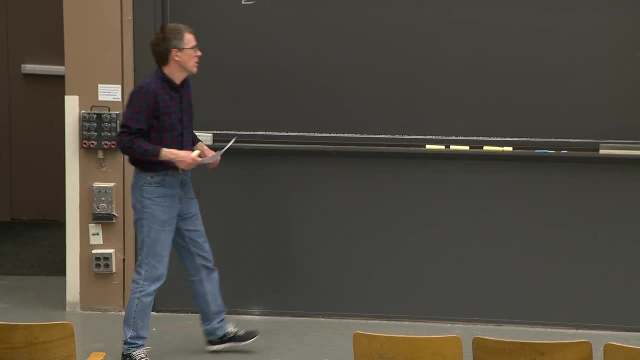 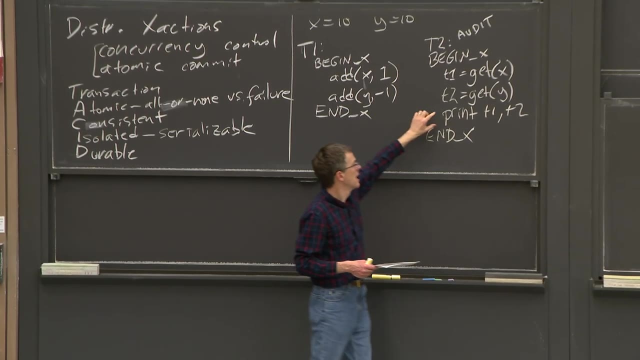 might do and, in addition, any output that the transactions produce. So for our transactions, these two adds, since they change records, they're. these change records are part of the results and the output of this print statement is part of the results. So the definition. 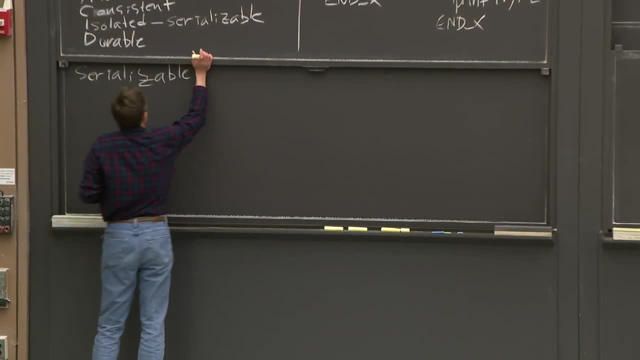 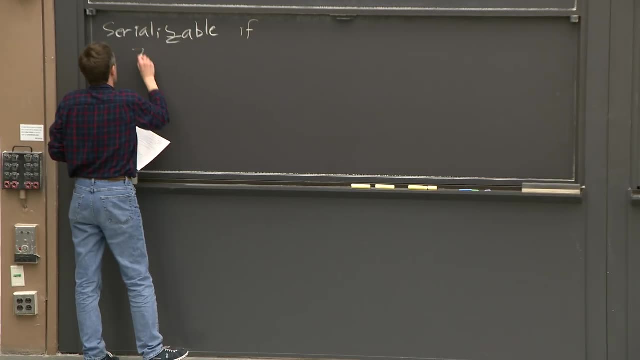 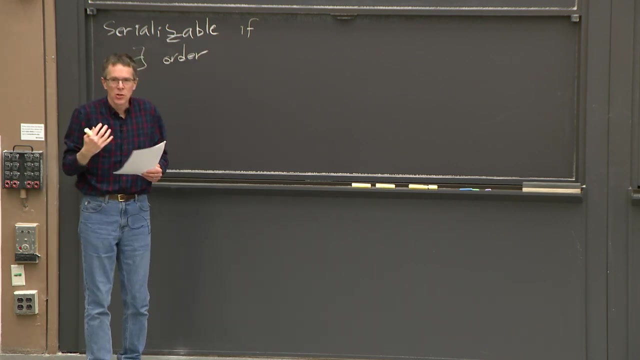 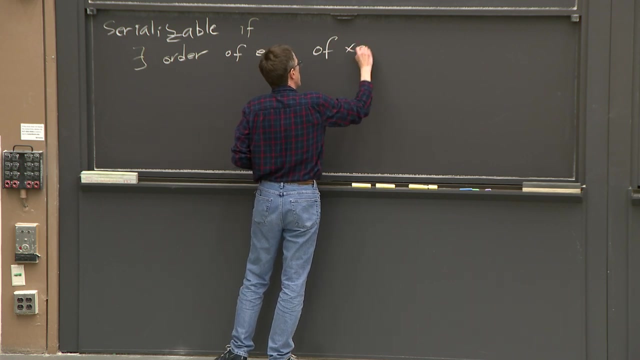 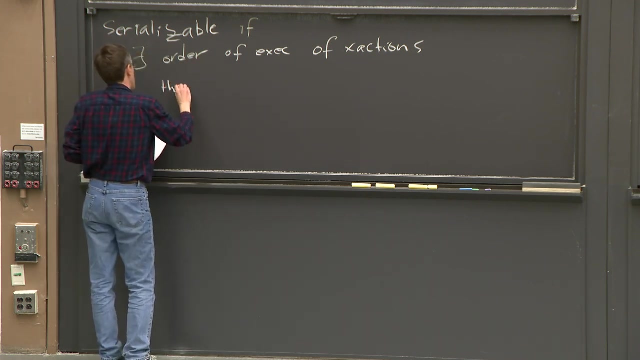 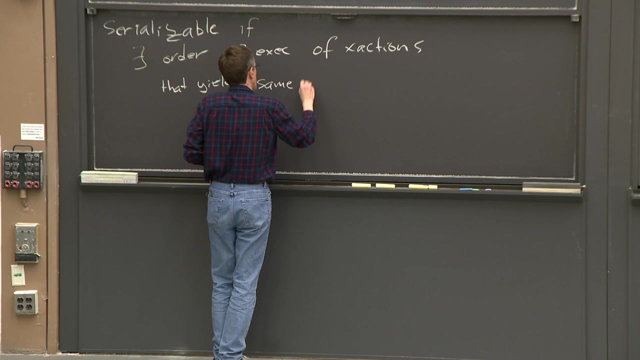 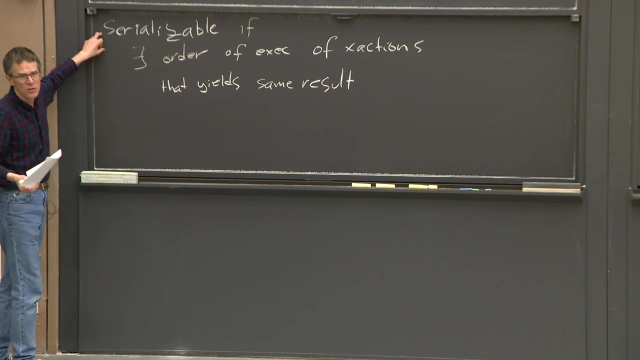 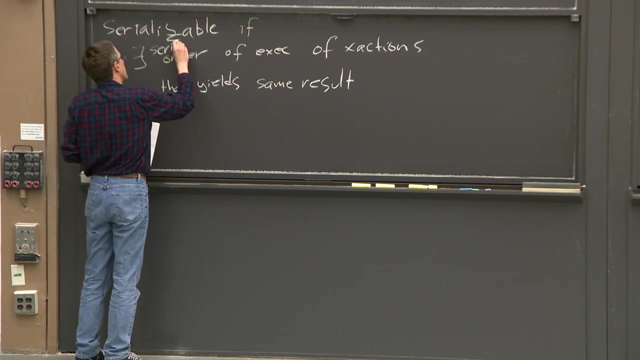 of serializable says the results are serializable. There's steps on this one as well- If there exists some order Of execution of the transactions. So we're going to say a specific execution, parallel, concurrent execution of transactions is serializable if there exists some serial order. I'm really emphasizing serial here. 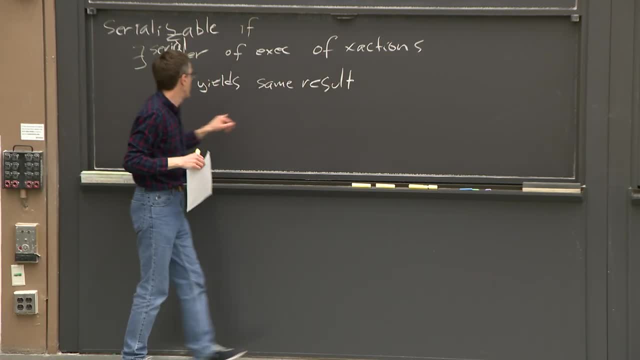 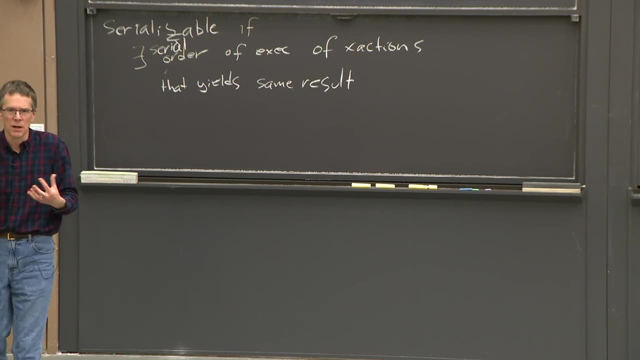 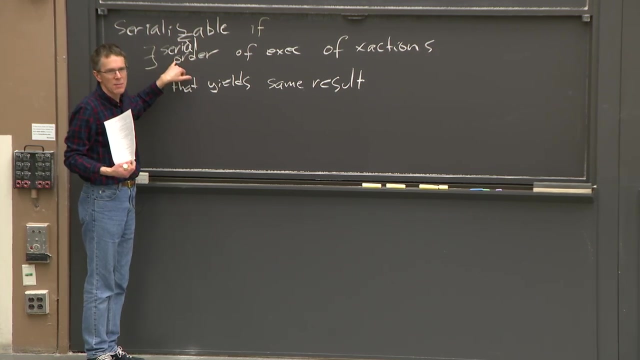 a serial order of execution of those same transactions that yields the same result as the actual execution, And the difference here is the actual execution may have had a lot of parallelism in it, But it's required to produce the same result as some one-at-a-time execution of the same. 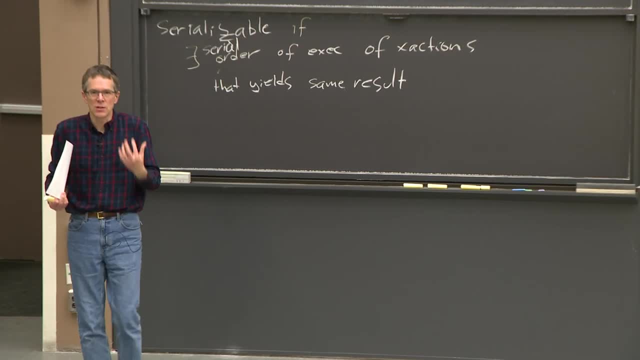 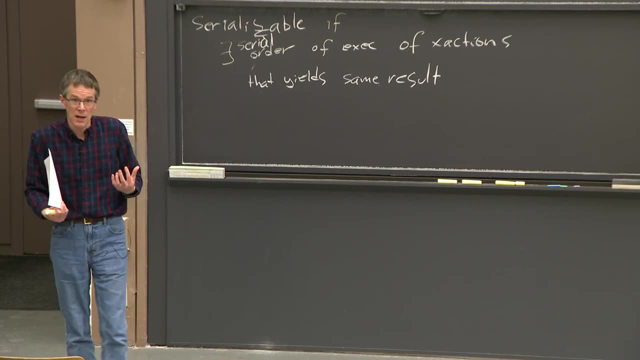 transactions, And so the way you check whether an execution is serializable, whether some concurrent execution is serializable, is you look at the results and see if you can find actually some one-at-a-time execution of the same transactions that does produce the same results. 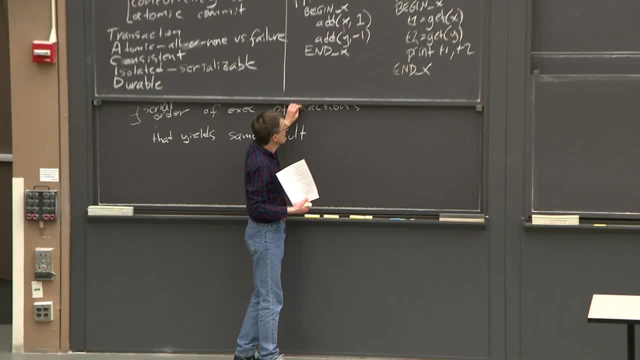 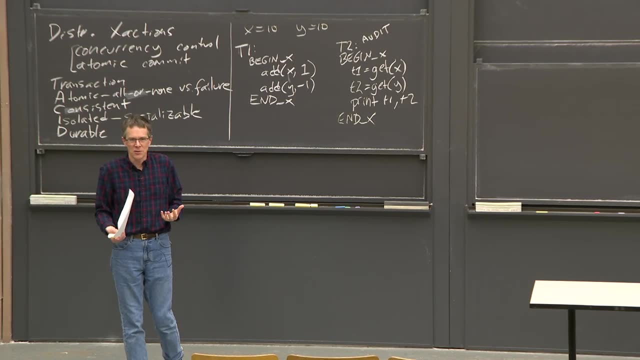 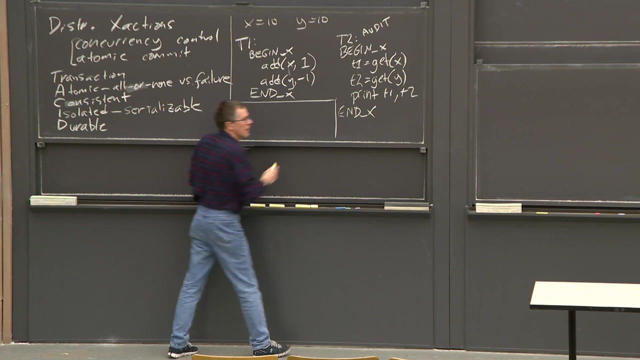 So for our transaction up here, Okay, So There's only two orders, There's only two one-at-a-time serial orders available, Transaction one then transaction two, or transaction two then transaction one, And so we can just look at the results that they would produce if executed one-at-a-time. 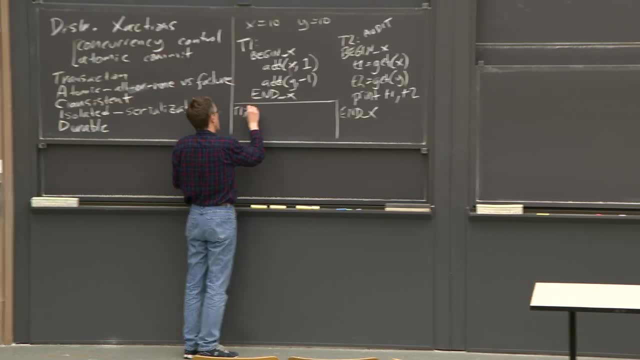 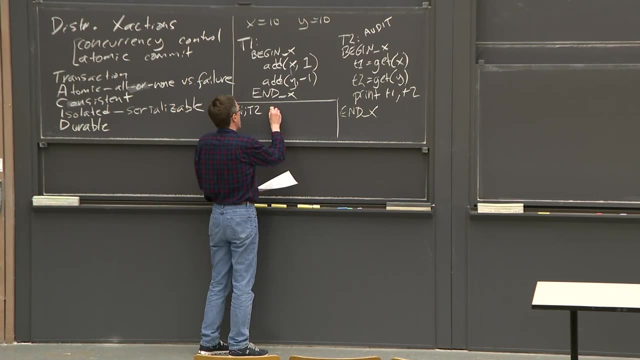 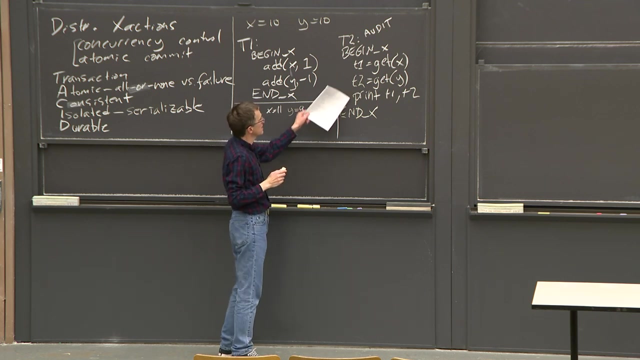 in each of these orders. So if we execute T1 and then T2, then we get X equals 11.. Okay, Okay, So if we execute T1 and then T2, then we get Y equals 9.. And this print statement: since T1 executed first, this print statement sees these two: 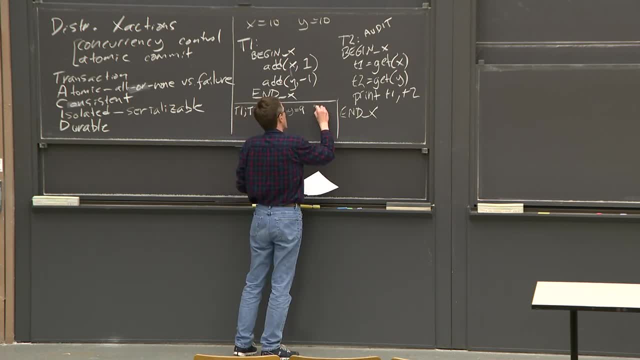 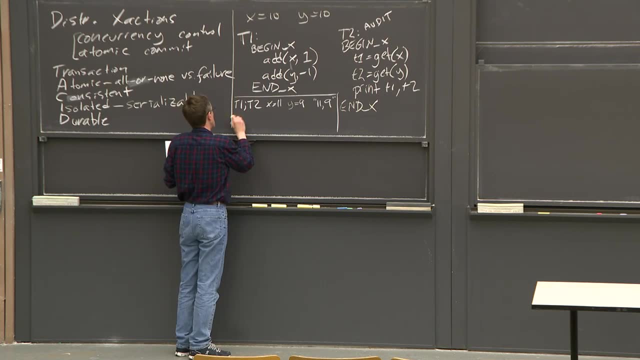 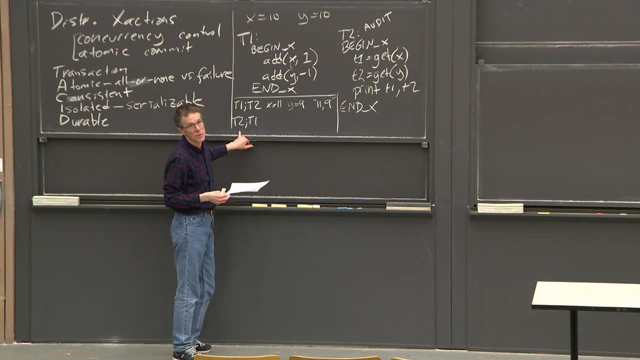 updated values, And so it'll print the string 11, 9.. The other possible order is that perhaps T2 ran first and then T1.. And in that case T2 will see the two records before they were modified, but the modifications. 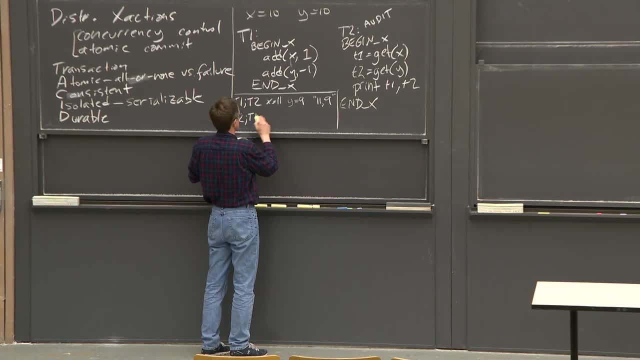 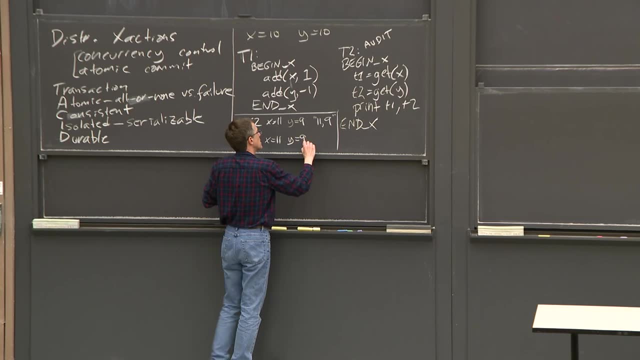 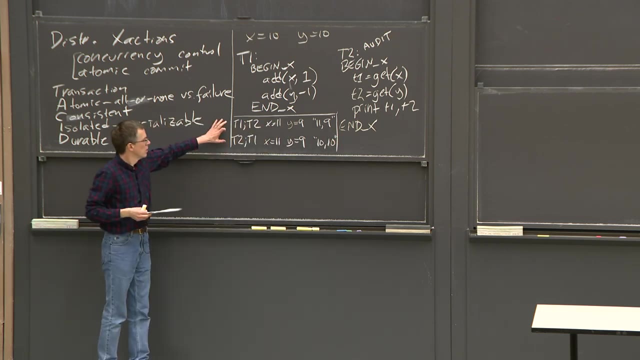 will still play an important role. Okay, So the final results will again be X equals 11,, Y equals 9.. But this time T2 saw the before values. So these are the two legal results for serializability, And if we ever see anything else from running these two transactions at the same time, we'll 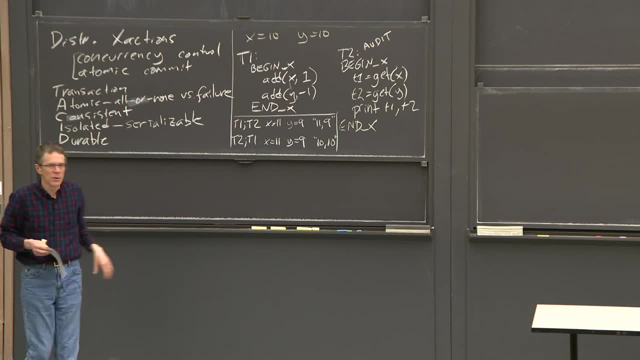 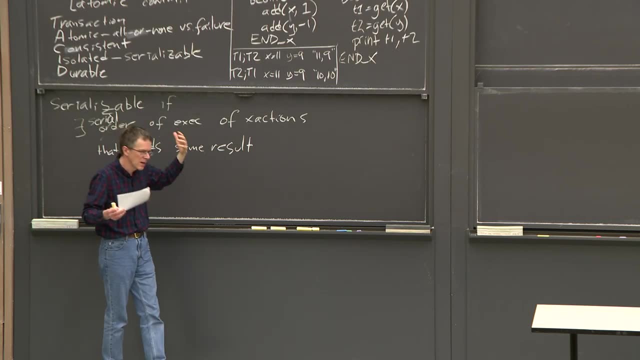 know that the database we're running against does not provide serializable execution, Okay, It's doing something else. And so while we're thinking through, oh, what would happen if? or what would happen if? we'll always be against these? aha, these are the only two legal results we better be doing. 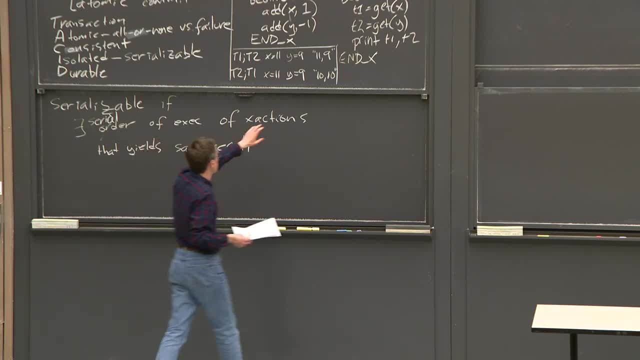 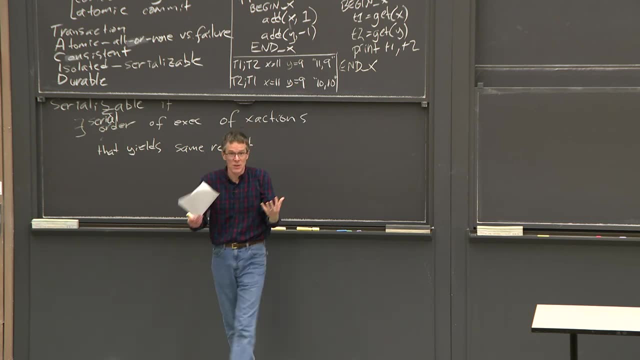 something that produces one or the other. It's interesting to note that there's more than one possible result, depending on the actual order. If you submit these two transactions at the same time, you don't know whether it's going to be T1, T2, or T2, T1.. 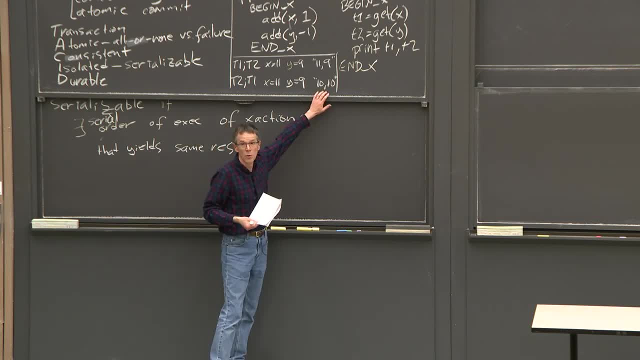 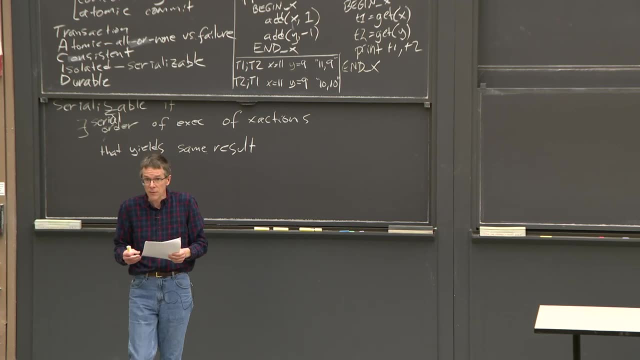 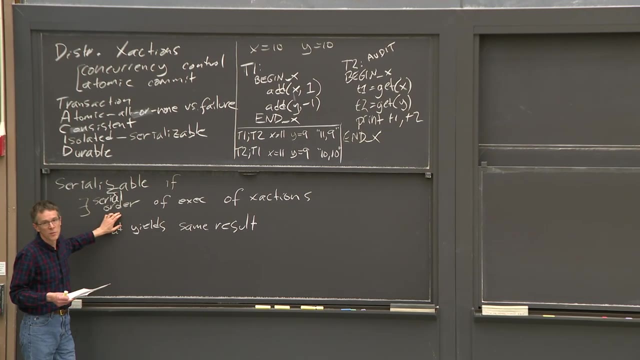 Okay, So you have to be willing to expect more than one possible legal result And, as you have more transactions running concurrently and more complicated, there may be many, many possible different correct results that are all serializable, because there are many, many orders here that could be used to fulfill this requirement. 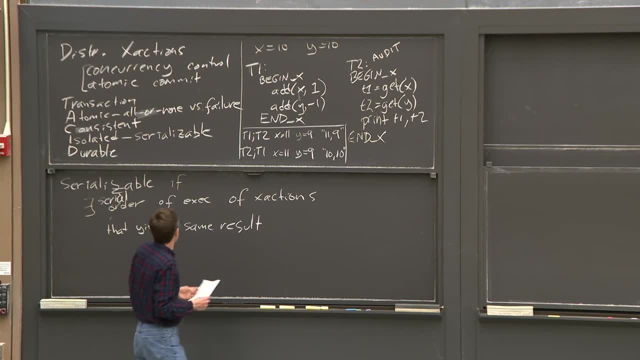 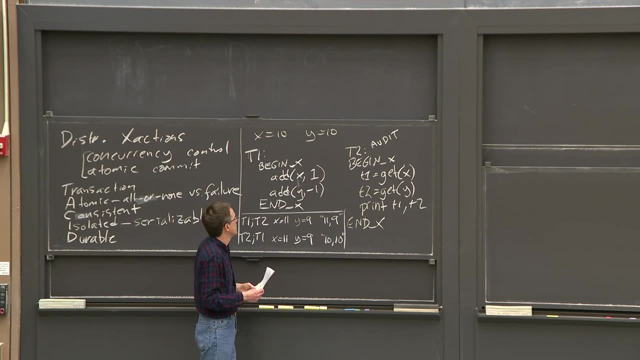 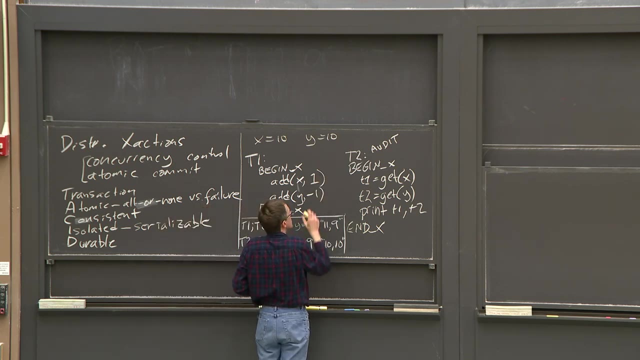 Okay. So now that we have a definition of correctness and we even know what all the possible results are, we can ask a few questions, So a few what-if questions, about how these could execute. So, for example, suppose that the way the system actually executed this was that it started. 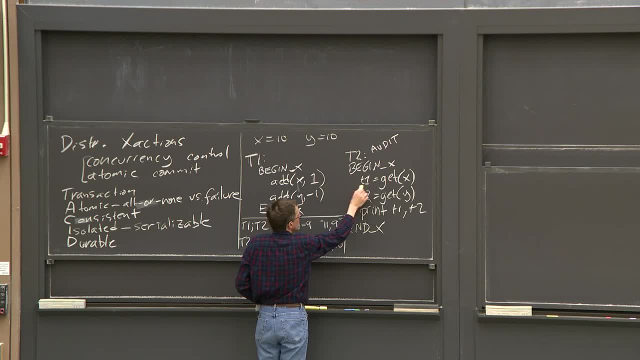 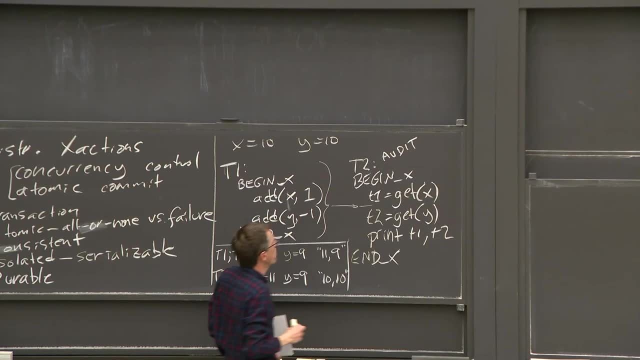 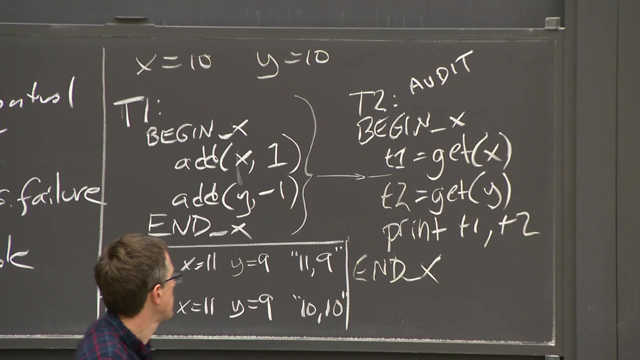 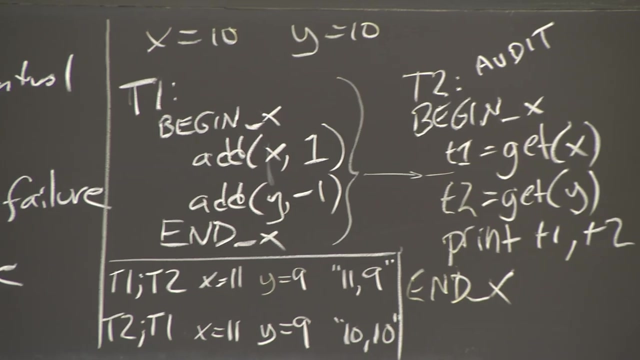 transaction two and got as far as just after reading X, and then transaction one ran at this point and then, after transaction one finished, transaction two continued executing. Okay, Now it turns out with different other transactions than this that might actually be legal. 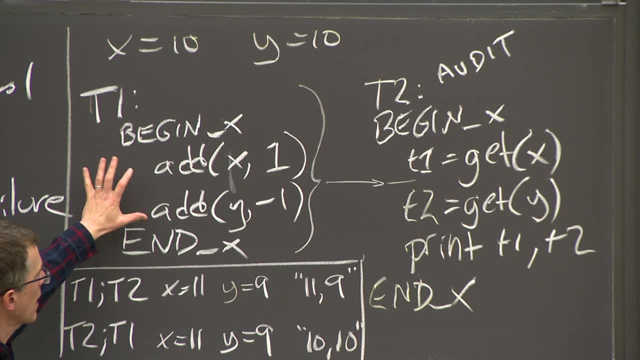 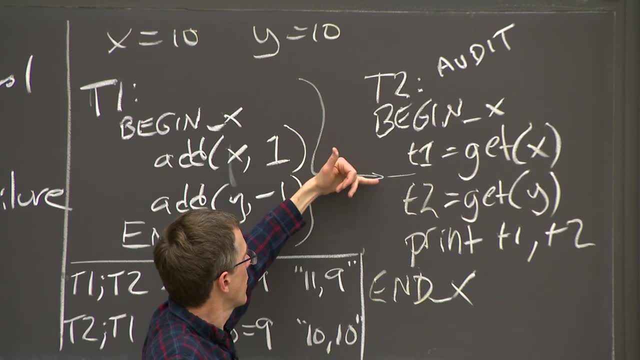 But here we want to know if it's legal. So we're wondering, gosh, if we executed it that way, what results will we get, and are they the same as either of these two? Well, if we execute transaction one here, then T1 is going to see value 10, T2 is going. 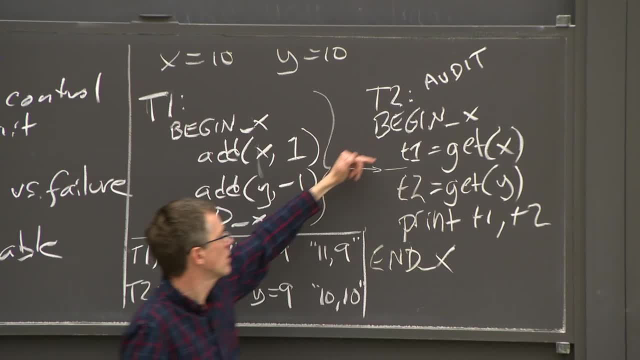 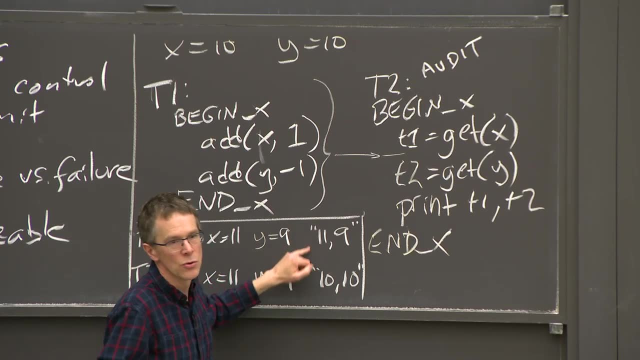 to see the value after decrementing Y. So T1 will be 10,, T2 will be 9, and what this print will be 10.9.. Okay, And that's neither of these two outputs here. So that means executing in this way that I just drew is not serializable. 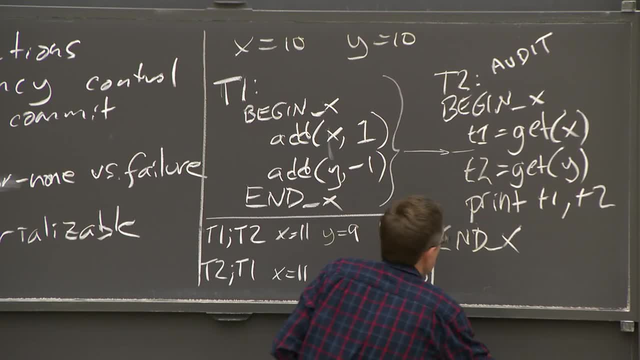 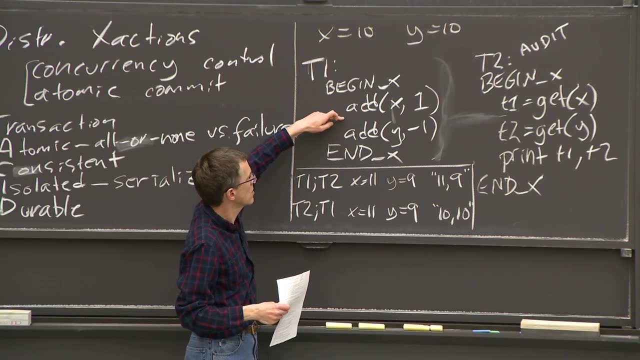 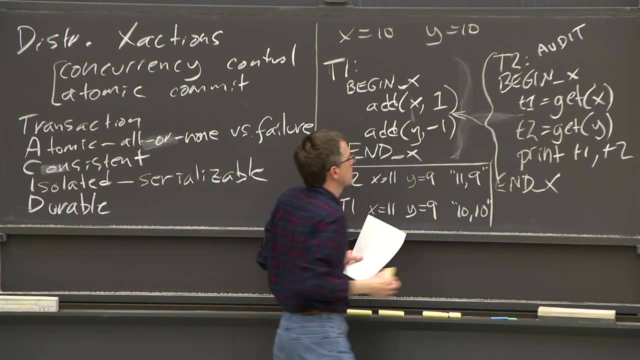 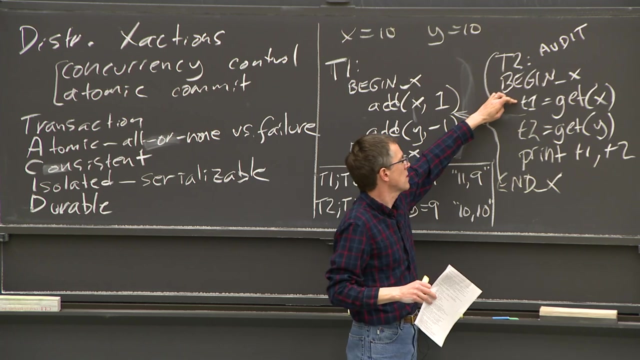 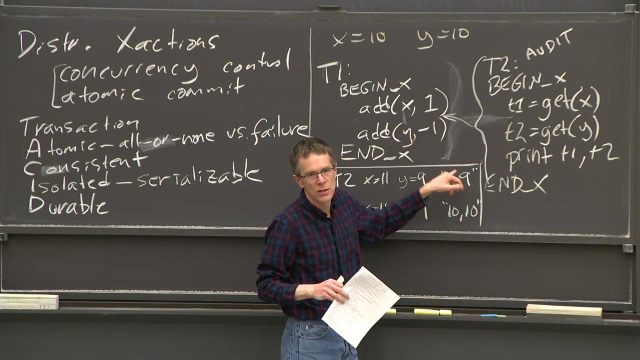 It would not be legal. Another interesting question is what if we started executing transaction one and we got as far as just after the first add and then at that point all of transaction two executed right here? So that would mean at this point, So now we're going to exit the transaction and then we're going to run a little test. 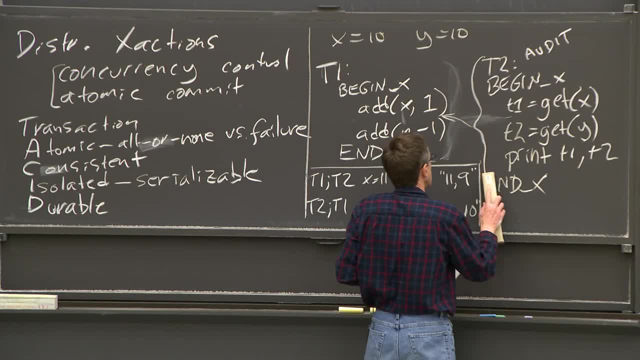 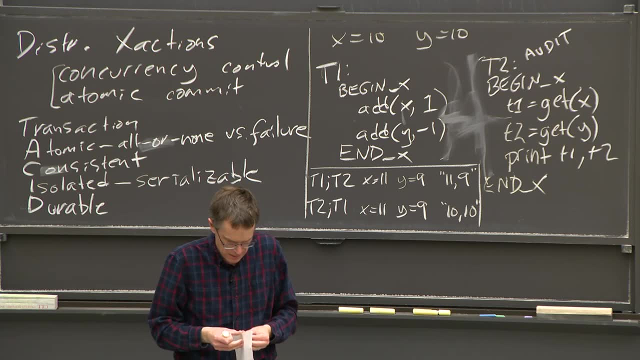 here, So it's going to print X as value 11.. The transaction two would read 11, 10.. It'll print 11, 10.. And 11, 10 is not one of these two legal values, So this execution is also not legal for these two transactions. 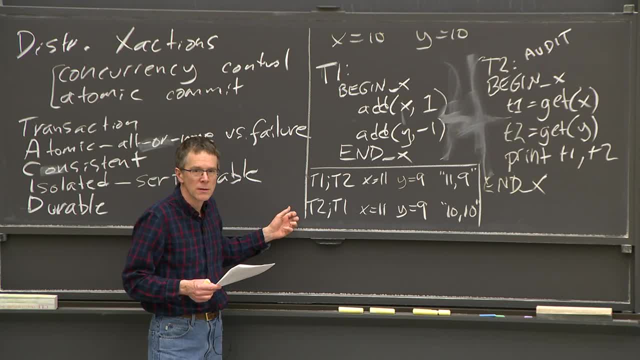 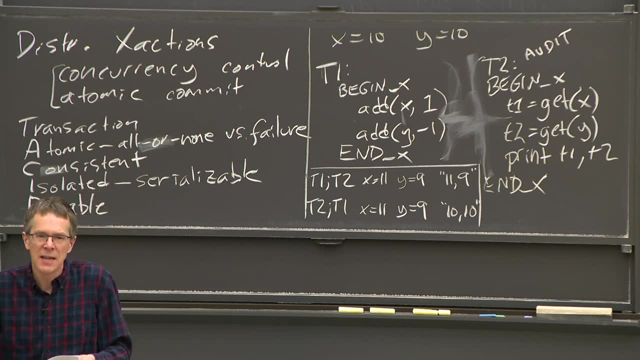 So the reason why serializable serializable is, you know when you're making transactions. serializability is a popular and useful definition of what it means for transactions to be correct, for execution of transactions to be correct, is that it's a very easy model for programmers. 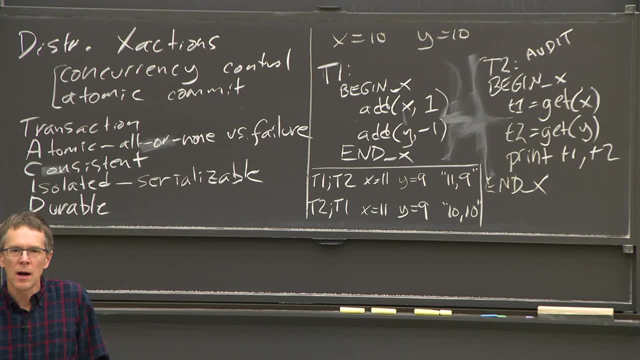 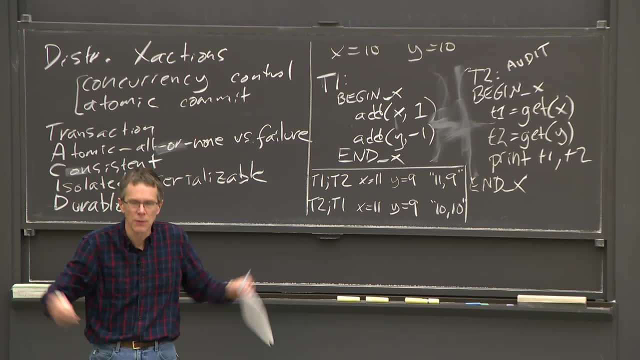 You can write complicated transactions without having to worry about what else may be running in the system. There may be lots of other transactions maybe using the same data as you, maybe trying to read and write it at the same time. There might be failures, Who knows? 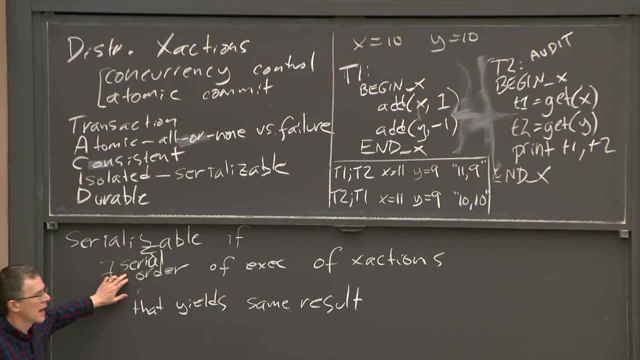 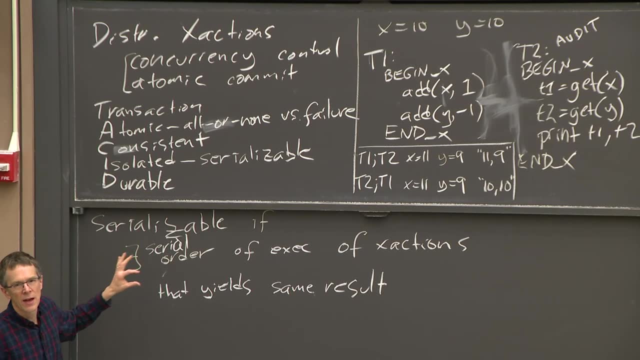 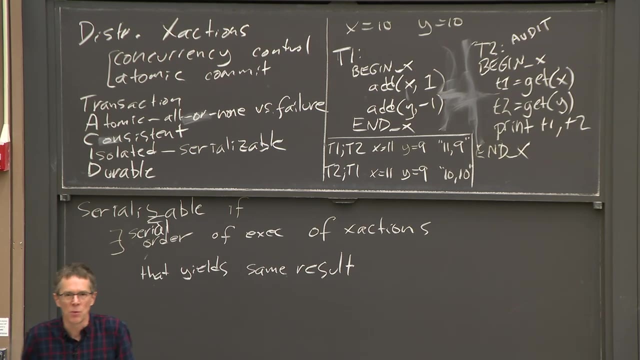 But the guarantee here is that it's safe to write your transactions as if nothing else was happening, because the final results have to be as if your transaction was executed by itself in this one-at-a-time order, which is a very simple, very nice programming model. 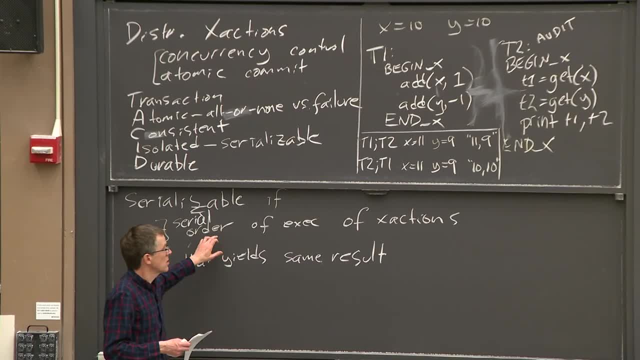 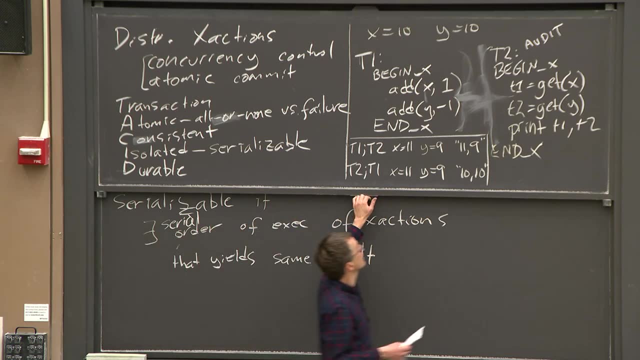 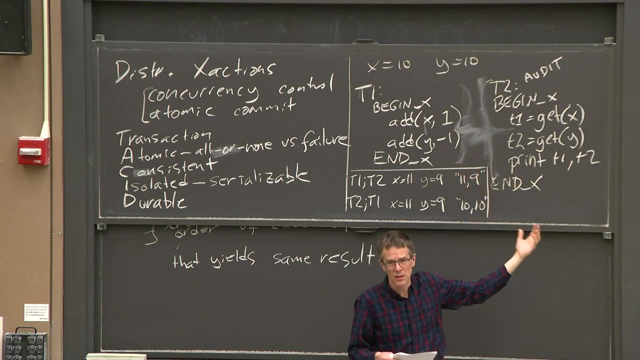 It's also nice that this definition allows truly parallel execution of transactions, as long as they don't use the same data. So we run into trouble here because these two transactions are both reading X and Y, But if they were using completely disjoint database records, it turns out this definition. 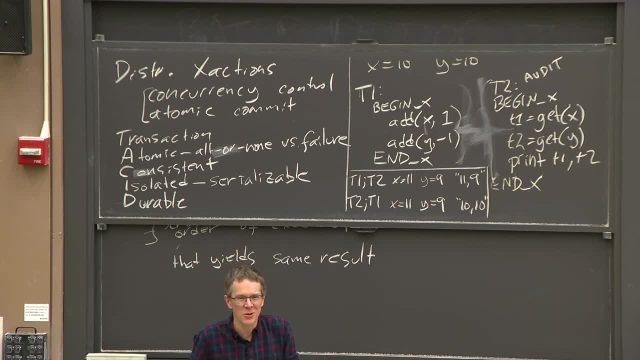 allows you to build a database system that would execute transactions that use disjoint data completely in parallel. And if you have a sharded system, which is what we're sort of working up to today, where the data different data's on different machines, you can get 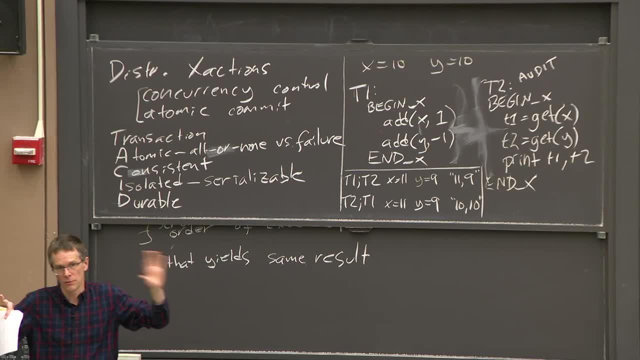 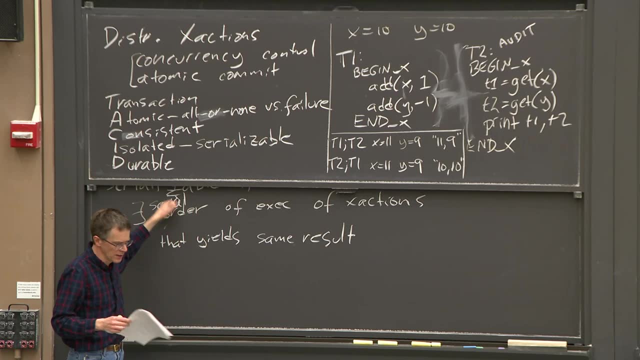 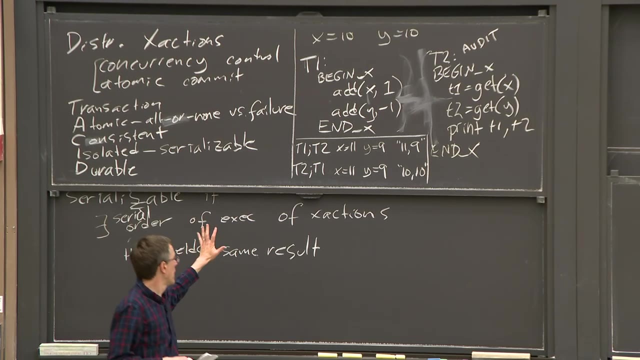 true parallel speedup, because maybe one transaction executes purely in the first shard on the first day And the other in parallel on the second machine. So there are opportunities here for good performance. Before I dig into how to implement serializable transactions, there's one more small point. 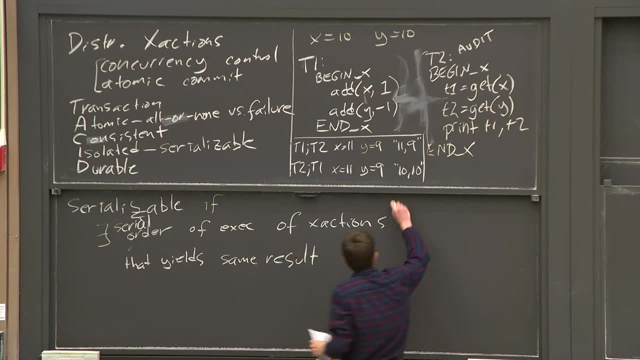 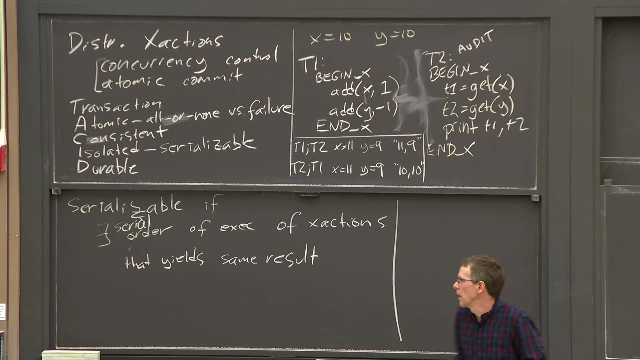 I want to bring up. It turns out that one of the things we need to be able to cope with is that transactions may, for one reason or another, basically Fail or decide to fail in the middle of the transaction, And this is usually called an abort. 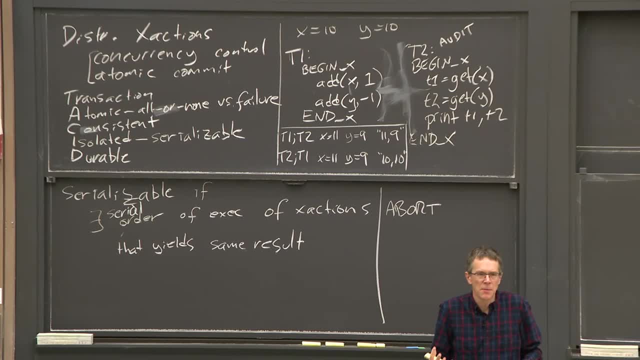 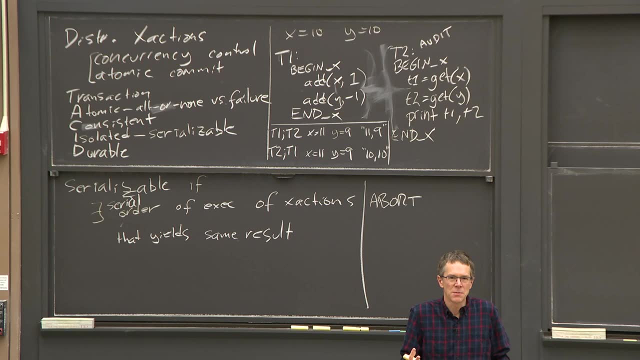 And you know, for many transaction systems we need to be prepared to handle, oh, what should happen if a transaction tries to access a record that doesn't exist, or divides by zero, Or maybe you know, since some transaction implementation schemes use locking, maybe a transaction causes a locking deadlock, And the only way to break that is to lock it, And that's the only way to break that. And the only way to break that is to lock it, And the only way to break that is to lock it. 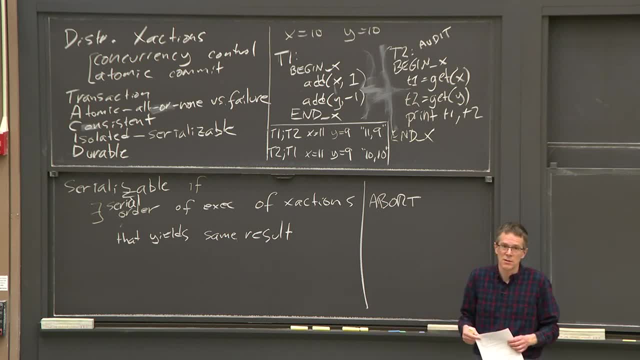 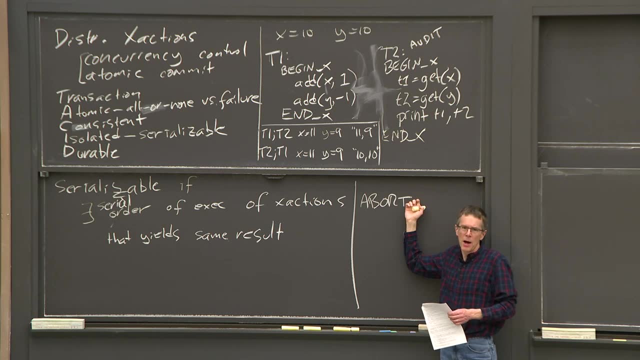 The deadlock is to kill one or more of the transactions that's participating in the deadlock. So one of the things that's going to be kind of hanging in the background and will come up is the necessity of coping with transactions that all of a sudden in the middle decide. 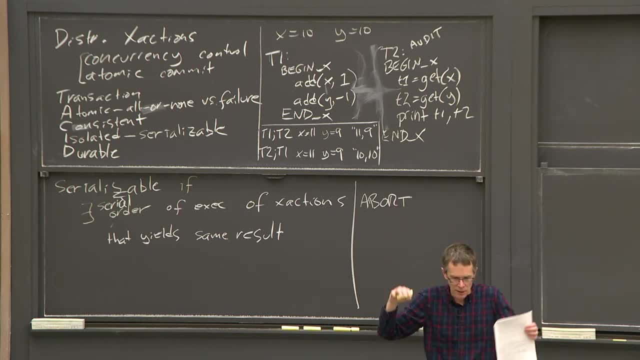 they just cannot proceed. And, you know, maybe really in the middle, after they've done some work and started modifying things, we need to be able to kind of back out of these transactions and undo any modifications they've made. All right, The implementation strategy for transactions, for these asset transactions, I'm going to 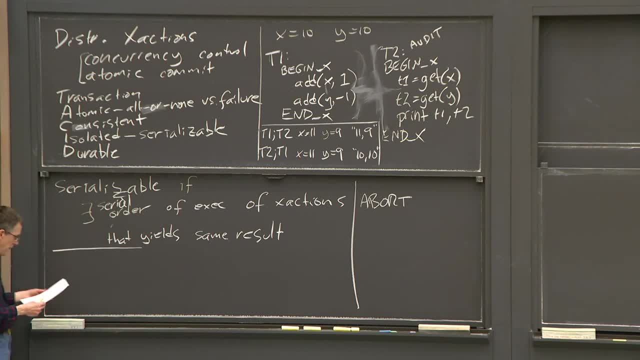 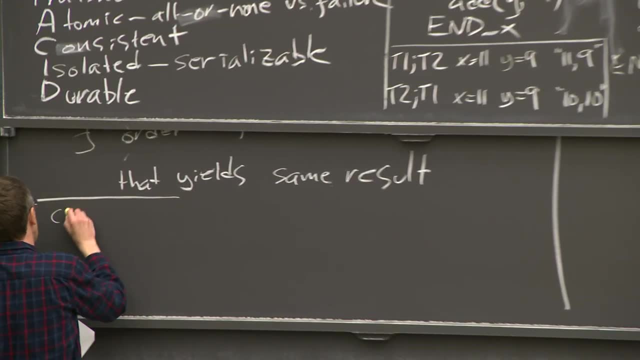 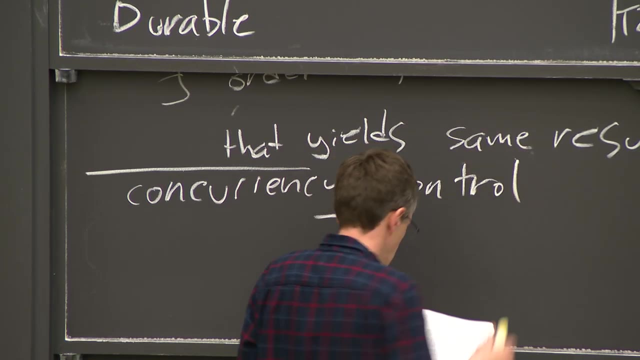 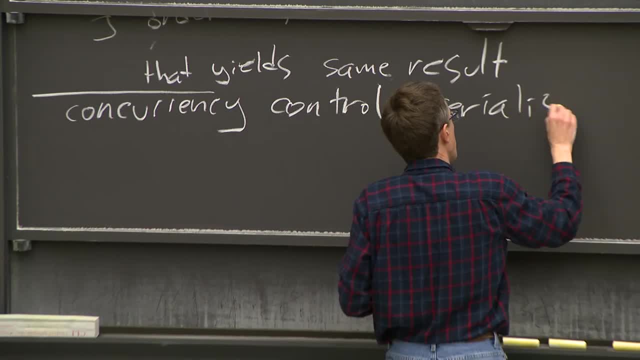 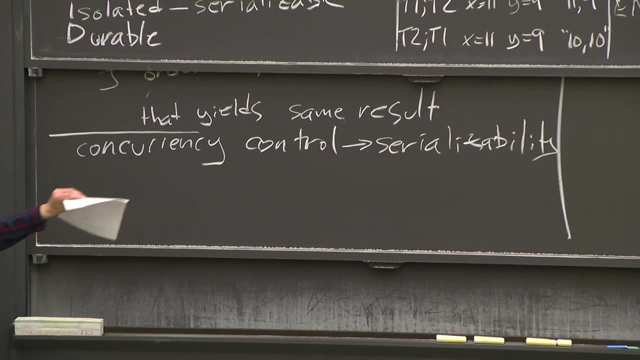 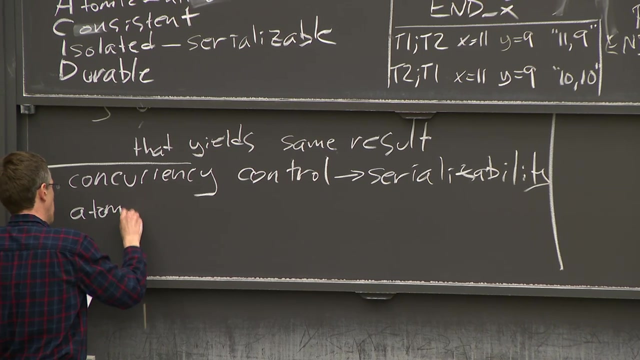 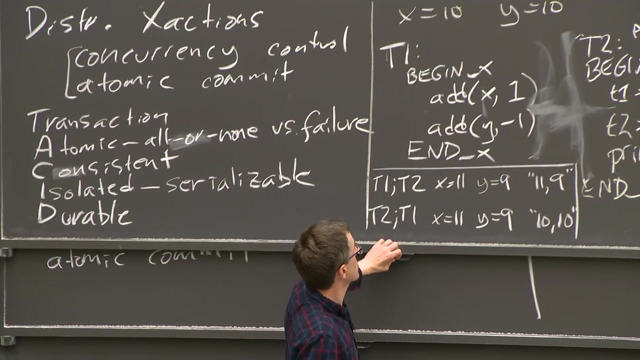 So concurrency control will bias isolation from other concurrent transactions that might be trying to use the same data. And the other big piece that I mentioned is atomic commit, And this is what's going to help us deal with the possibility that- oh yeah, this transaction. 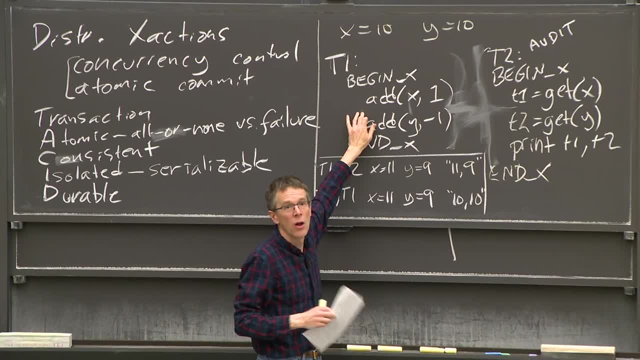 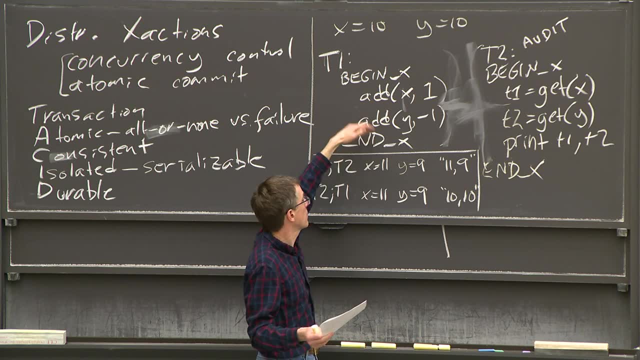 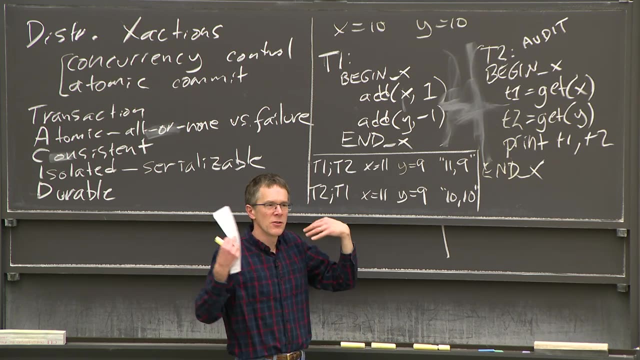 is executing a log And it's maybe modified X, And then all of a sudden there's a failure in one of the servers involved But other servers that were maybe executing other parts of the transaction. that is, if X and Y are in different machines, we need to be able to recover even if there's a partial. 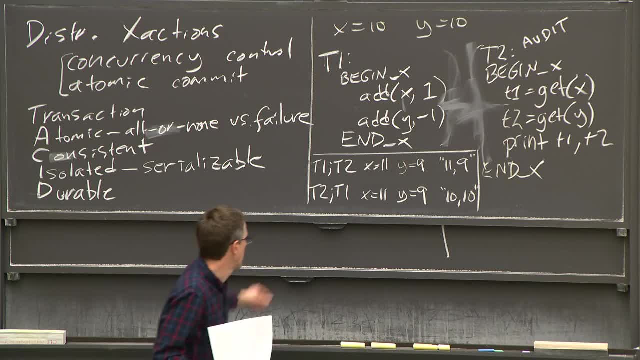 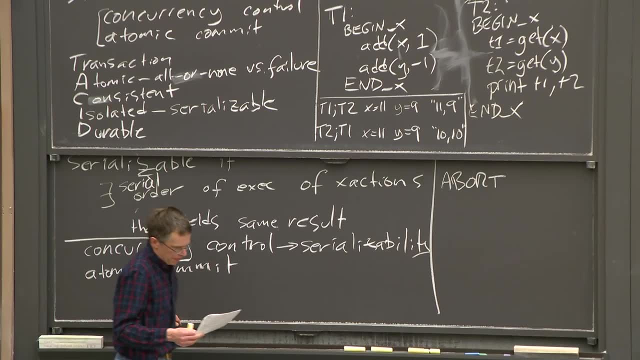 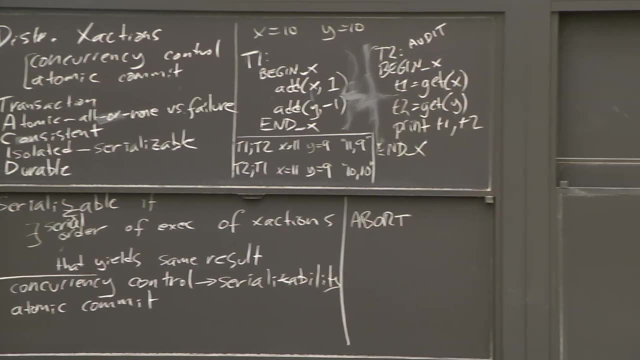 failure of only some of the machines, the transaction is running on, And the big tool people use for that is this atomic commit, which we'll talk about All right. So first, concurrency control. There's really two classes, two major approaches to concurrency control. 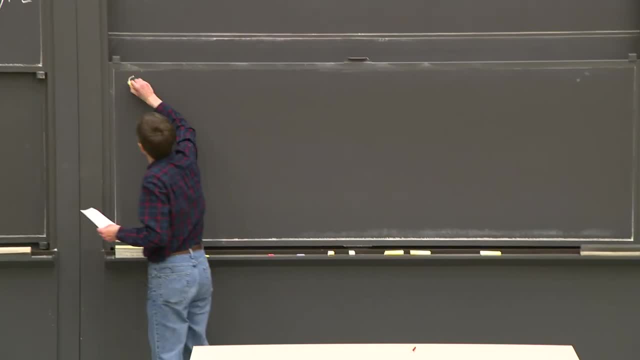 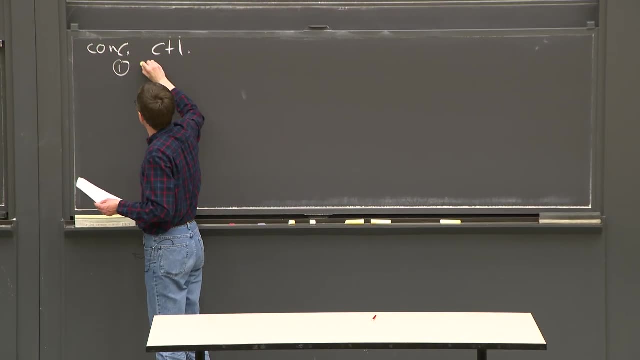 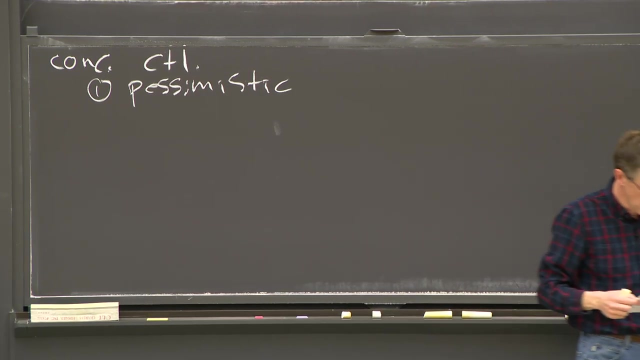 And we'll talk about both during the course. These are just main strategies. The first strategy is pessimistic, Usually called pessimistic concurrency control, And this is usually locking. We've all done locking in the labs And they're all locked. 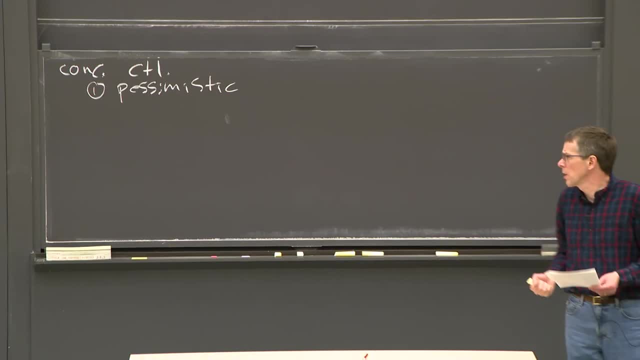 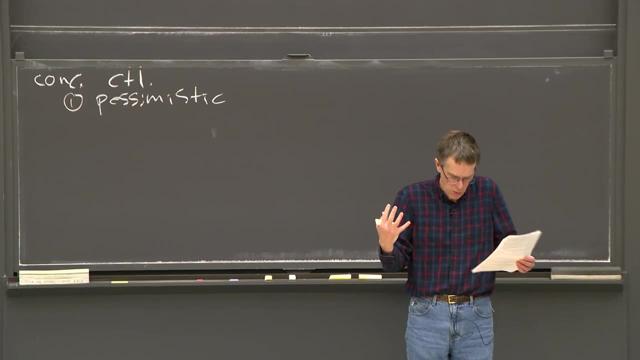 We've all done locking in the context of Go programs. It turns out databases- transaction processing systems also use locking, And the idea here is the same as one you're quite familiar with: is that before a transaction uses any data, it needs to acquire a lock on that data. 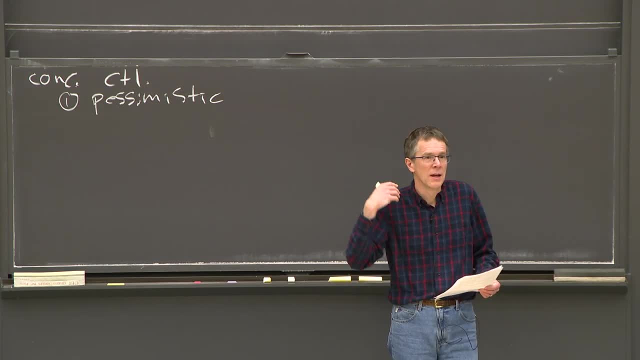 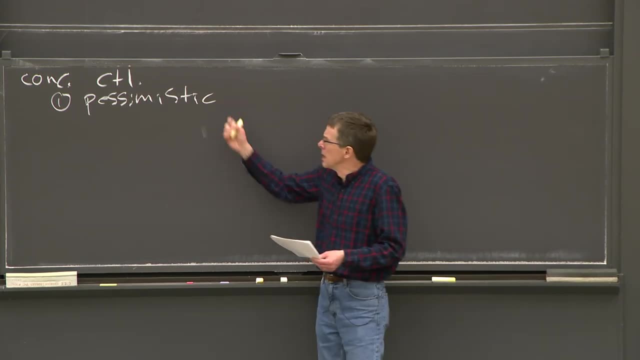 And if some other transaction is already using the data, the lock will be held And we'll have to wait before we can acquire the lock. wait for the other transaction to finish And in pessimistic systems, if there's locking conflicts, somebody else has to lock. 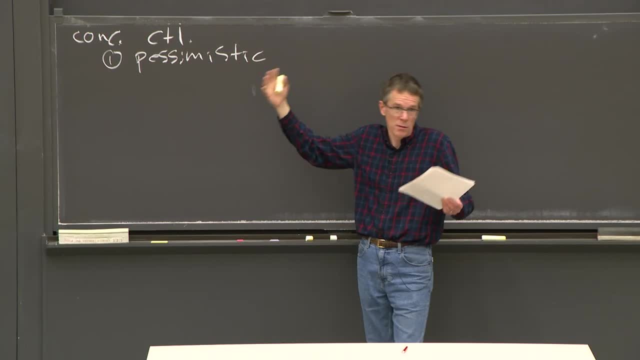 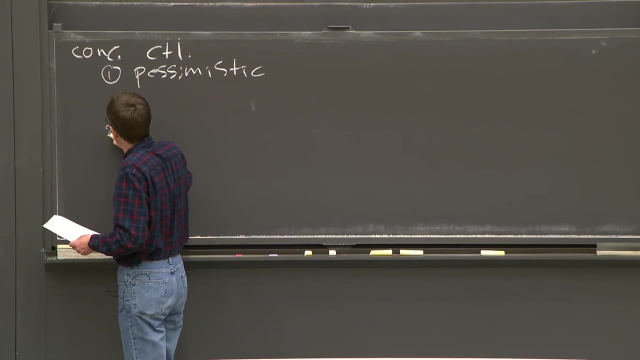 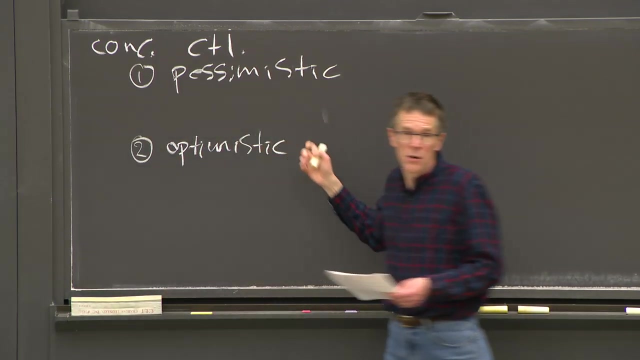 It'll cause delays. So you're sort of trading performance for correctness. The other main approach is optimistic approaches. The basic idea here is you don't worry about whether maybe some other transaction is reading or writing the data at the same time as you. 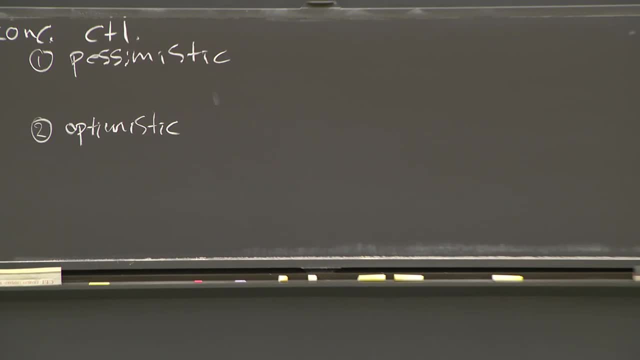 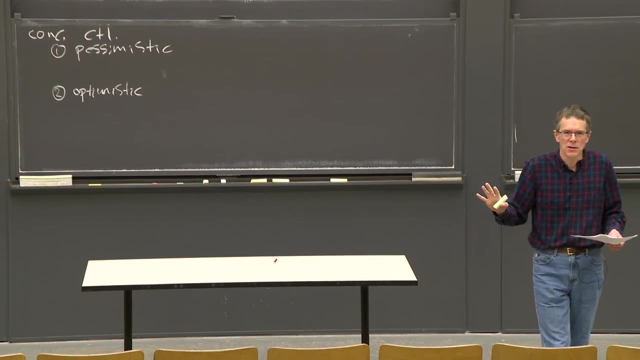 You just go ahead and do whatever reads and writes you're going to do, although typically into some sort of temporary area, And then only at the end You go and check whether actually maybe some other transaction might have been interfering, And if there's no other transaction, ah, you're done. And you never had to go through any of the overhead or waiting of taking out locks. The locks are reasonably expensive to manipulate, But if somebody else was modifying the data in a conflicting way at the same time you were, then you have to abort that transaction and retry. 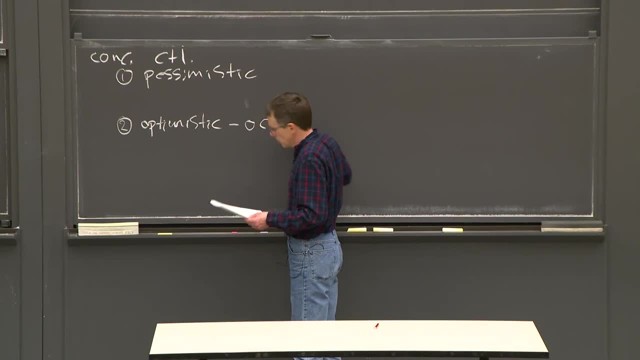 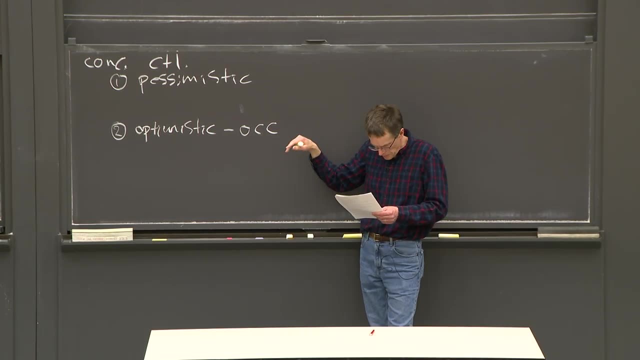 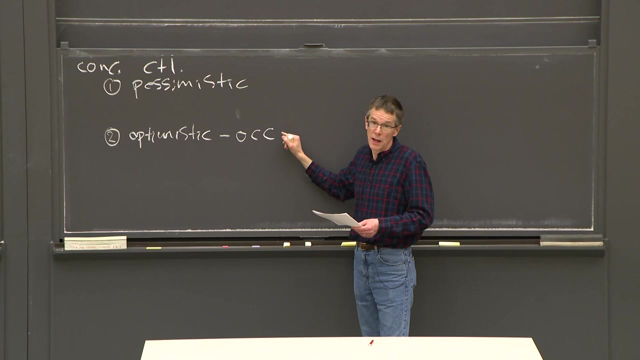 And Yeah, So the abbreviation for this is often optimistic concurrency control. It turns out that under different circumstances, these two strategies one can be faster than the other. If conflicts are very frequent, you probably actually want to use pessimistic concurrency control, because if conflicts are frequent, you're going to get a lot of aborts due to. 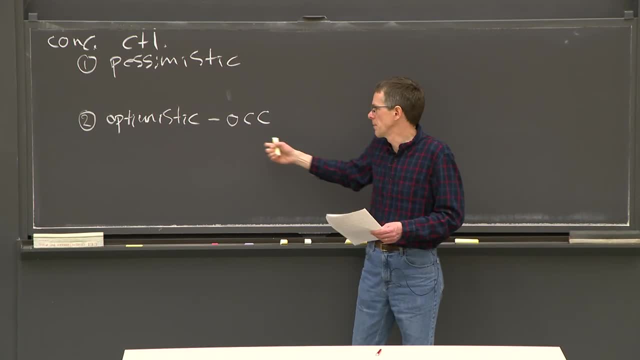 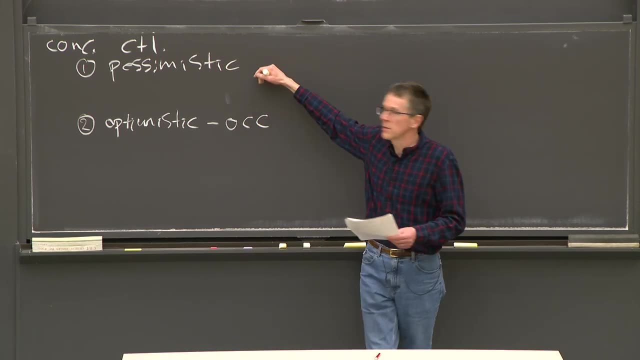 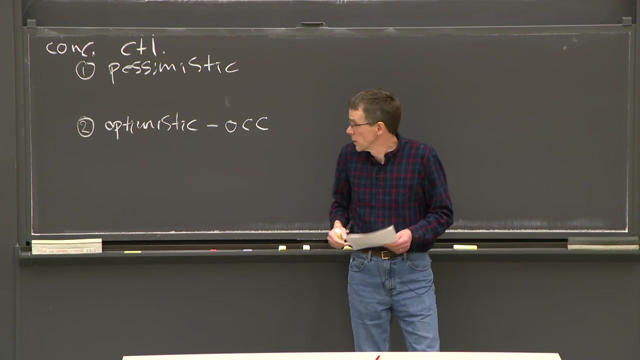 conflicts for optimistic schemes. If conflicts are rare, then optimistic concurrency control can be faster because it completely avoids locking overhead. Today will be all about pessimistic concurrency control And then some later paper, in particular Farm in a couple of weeks, will deal with. 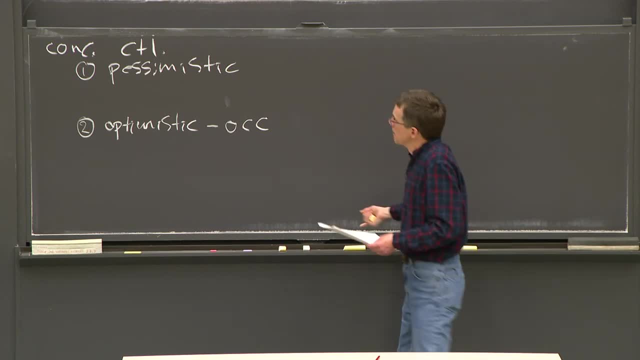 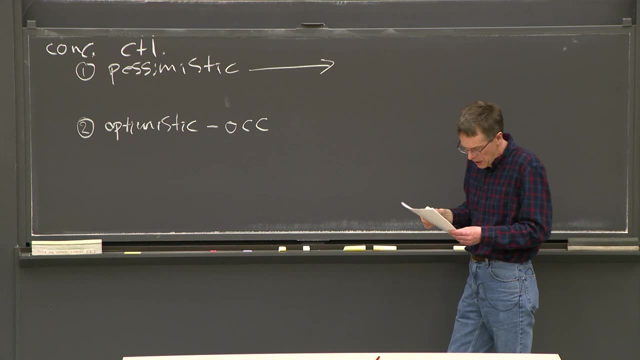 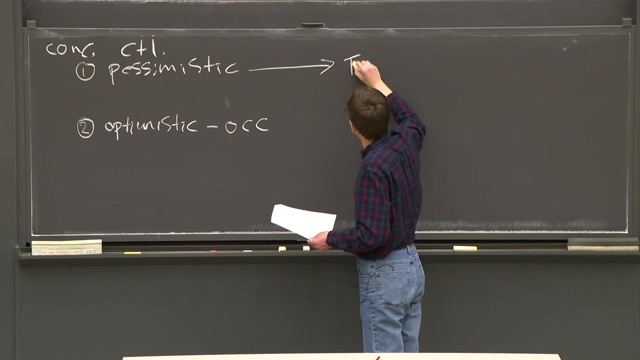 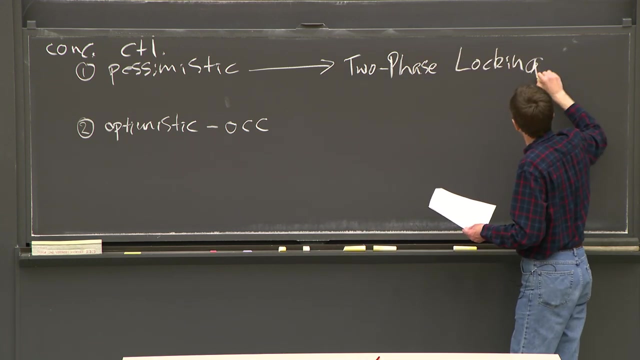 an optimistic scheme. Okay, So today I'm talking about pessimistic schemes. It refers basically to locking And, in particular for today, the reading was about two-phase locking, which is the most common type of locking, And the idea in two-phase locking for transactions is that a transaction is going to use a bunch. 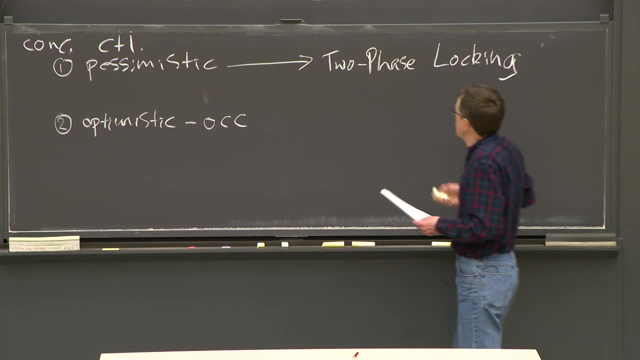 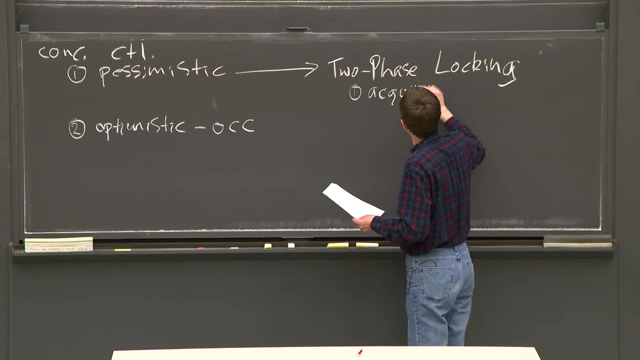 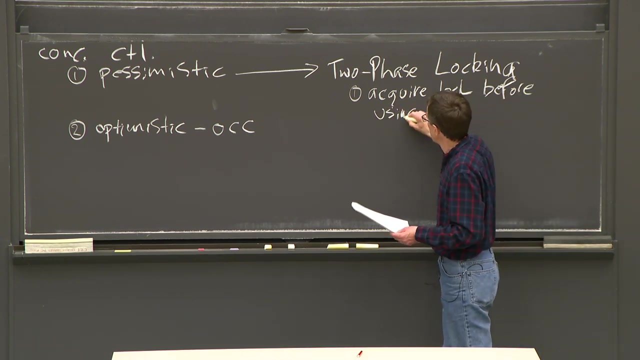 of records like X and Y in our example. The first rule is that you acquire a lock before using any piece of data, before reading or writing any record, And the second rule for transactions is that you acquire a lock before using any piece of data. 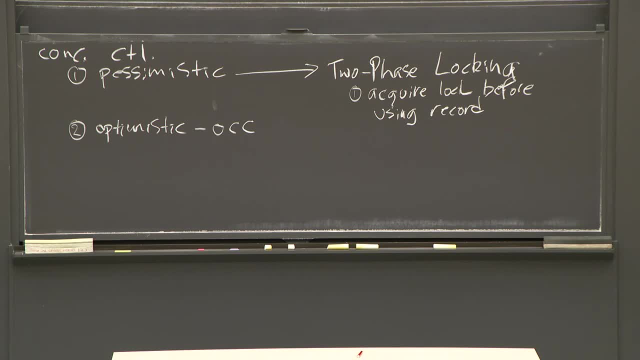 And the third rule for transactions is that a transaction must hold any locks it acquires until after it commits or aborts. So you're not allowed to give up locks in the middle of the transaction. You have to hold them all. You can only accumulate them until you're done, until after you're done. 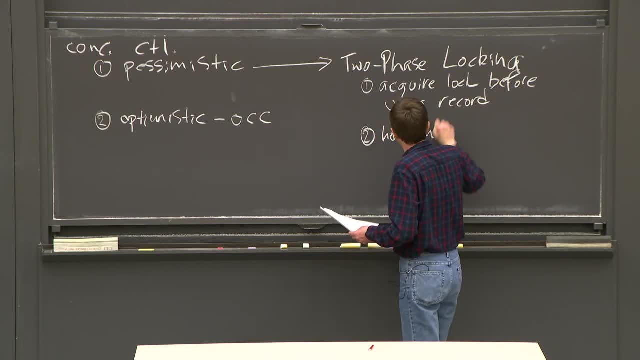 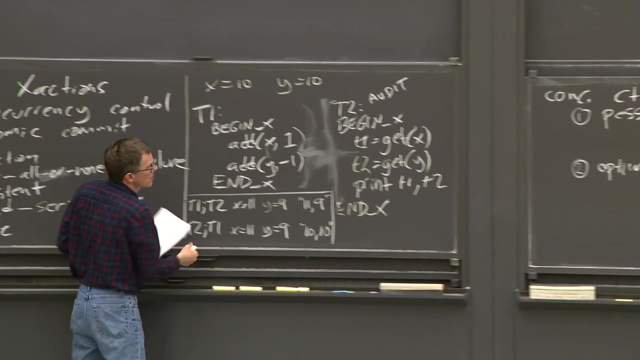 So hold until completely done. So this is two-phase locking. The phases are the phases which we acquire locks and then the phase in which we just hold on to them until we're done. So for two-phase locking, to sort of see why locking works here: typical locking systems. 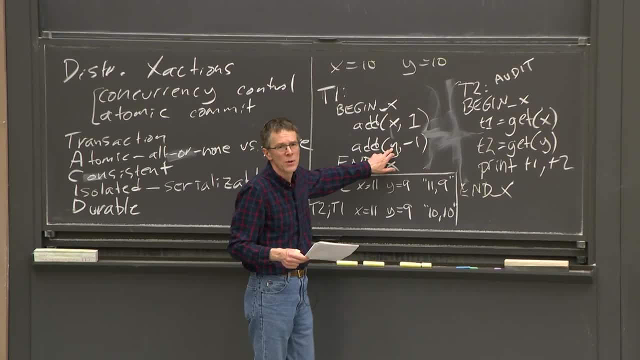 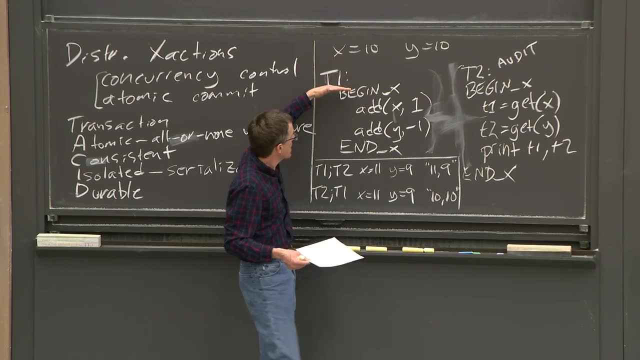 although there's a lot of variation, typical locking systems associate a separate lock with each record in the database, with each row and each table. for example, although they can be more coarse-grained, These transactions start out holding no locks. Let's say, transaction one starts out holding no locks. 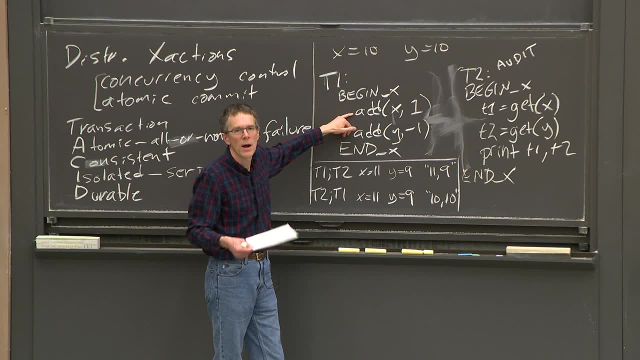 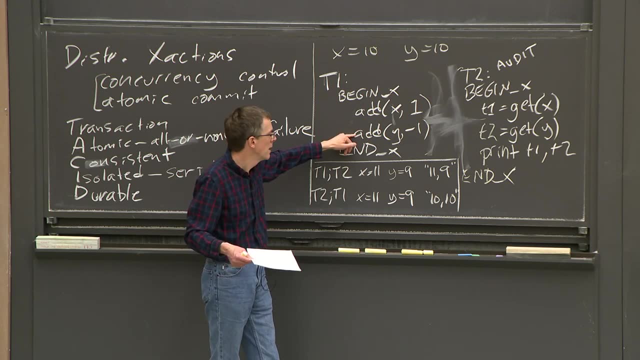 When it first uses X, before it's allowed to use it, it has to acquire a lock. It has to acquire the lock on X. It may have to wait, And when it first uses Y, it acquires another lock, the lock on Y. 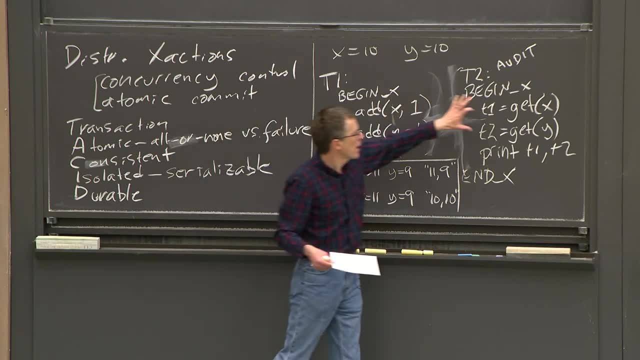 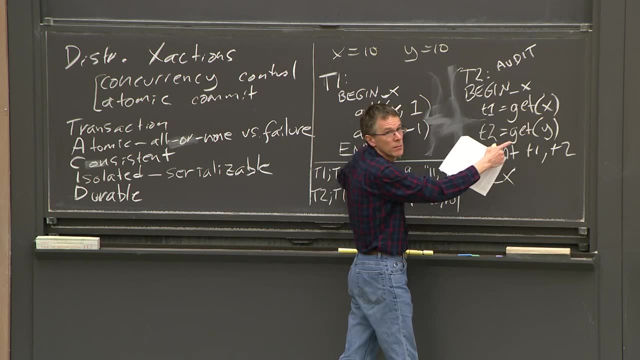 When it finishes, after it's done, it can release both. If we ran both these transactions at the same time, they're going to basically race to get the lock on X, And whichever of them manages to get the lock on X first, it will proceed and finish. and 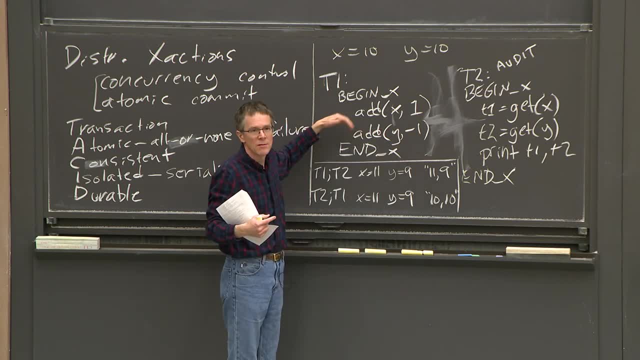 commit Meantime. the other transaction that didn't manage to get the lock on X first is going to sit here. It's going to sit here waiting before it does anything with X until it can acquire the lock. So if transaction two actually got the lock first, it would get the value of X, get the 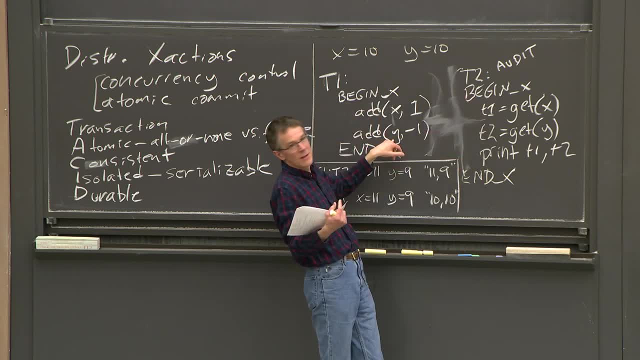 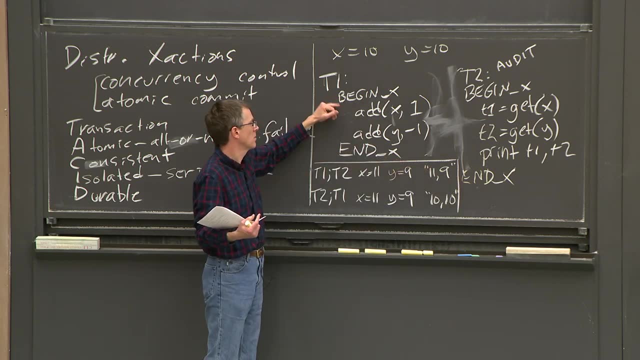 value of Y, because transaction one hasn't gotten to this point, hasn't locked Y yet, It'll print and it'll finish and release its locks And only then transaction one will be able to acquire the lock on X And, as you can see, that basically forces a serial order because it forced in this. 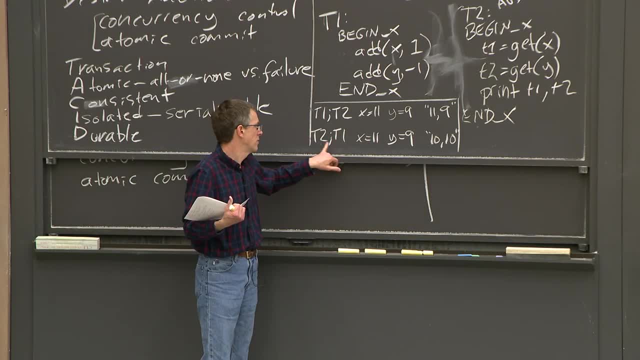 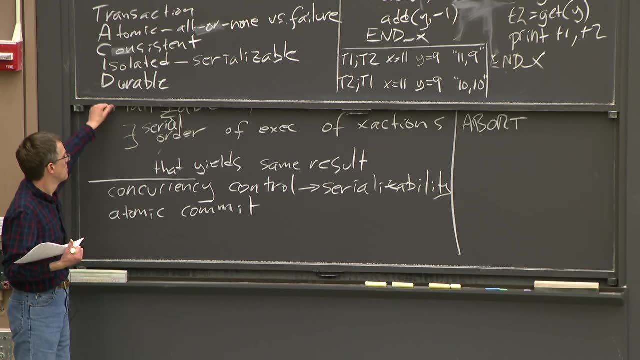 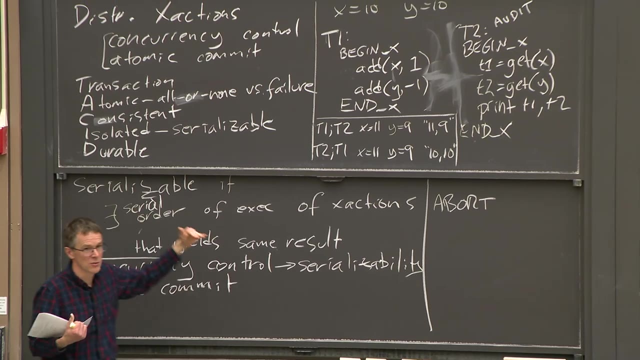 case it forced the order. It forced the order T2, and then, when T2 finishes, only then T1. So it's explicitly forcing an order which causes the execution to follow the definition of serializability. It really is executing T2 to completion and only then T1. 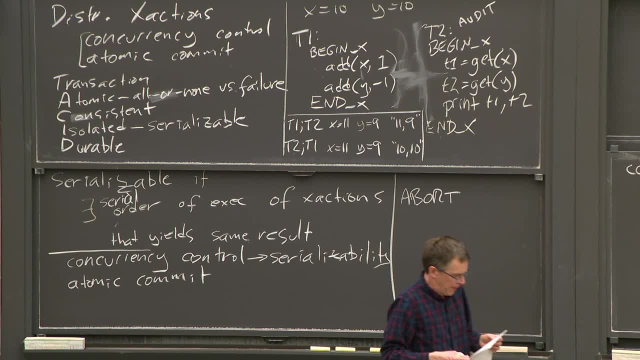 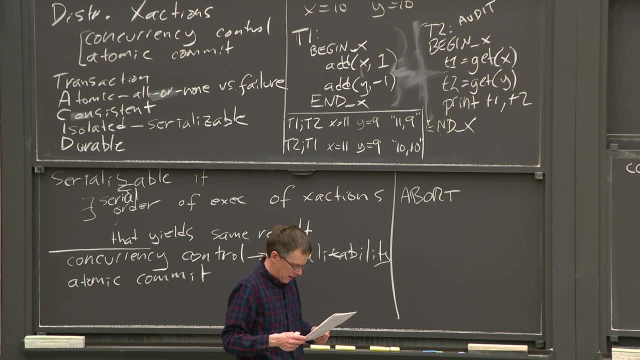 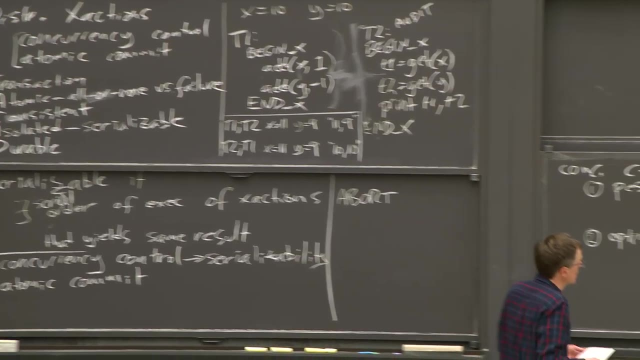 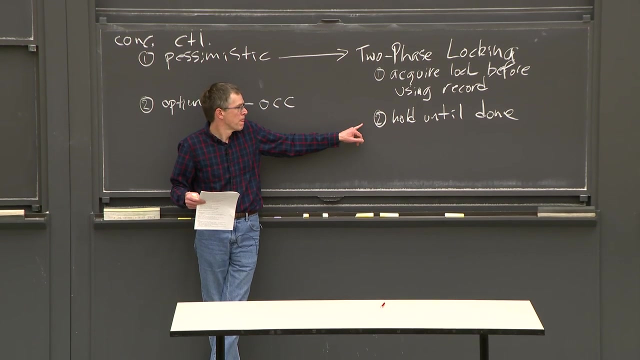 So we do get correct execution, All right. So one question is why you need to hold the locks until a transaction is completely finished. You might think that you could just hold the lock while you were actually using the data, and that would be more efficient. 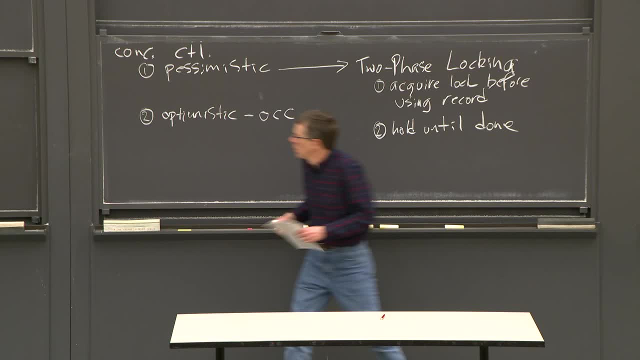 And indeed it would. That is, you know. maybe you only hold the lock for the period of time in which T2 is actually looking at record X, Or maybe you only hold the lock for the period of time in which T2 is actually looking at. 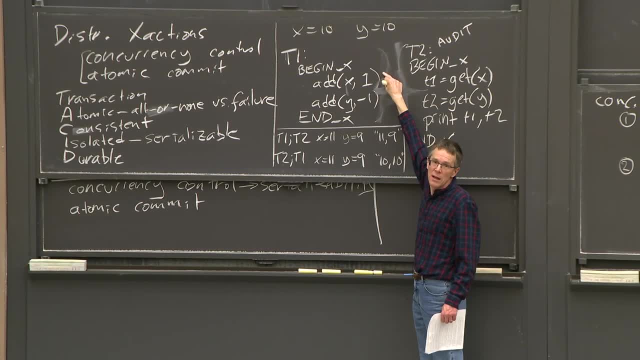 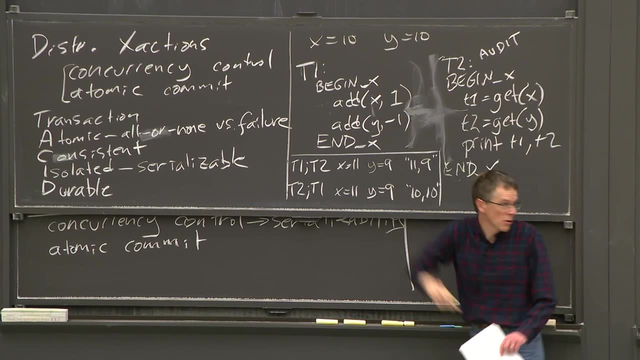 record X. Or maybe you only hold the lock on X here for the duration of the add operation and then immediately release it, And you know in that case that would, if we transaction would immediately release the lock on X, thereby disobeying this rule, of course. 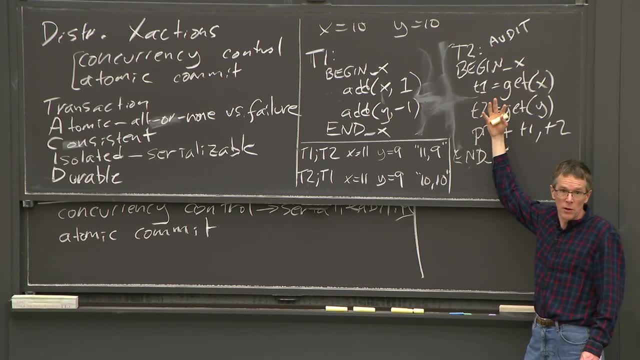 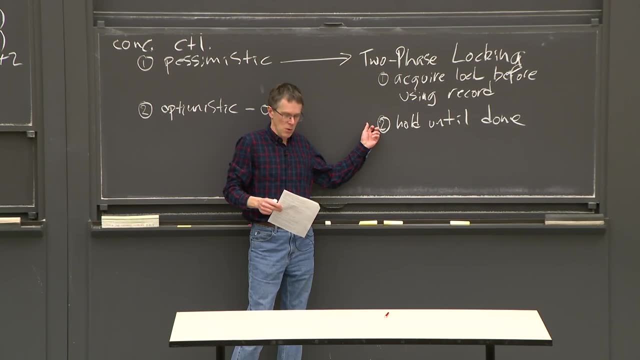 But if it immediately released the lock on X, then transaction 2 might be able to start a little bit earlier. We get more concurrency, more higher performance. So this rule definitely, you know, is bad for performance. So we want to make pretty sure that it's good for that. it's required for correctness. 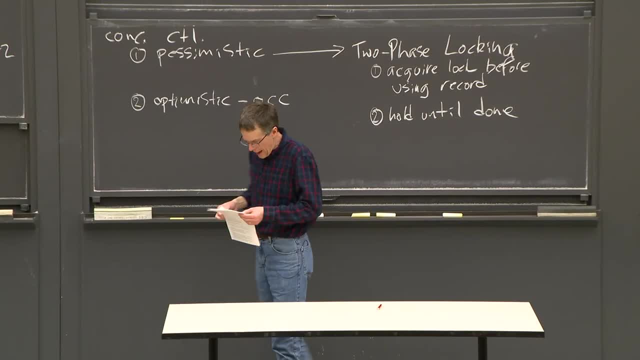 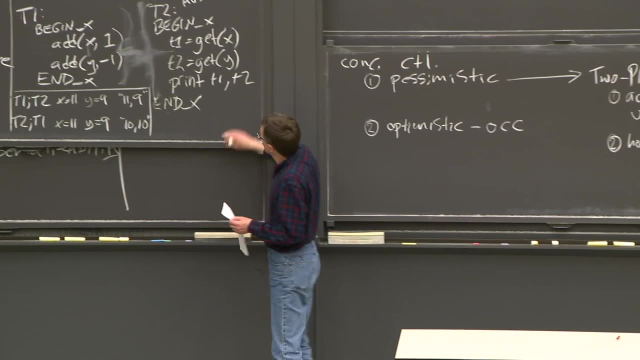 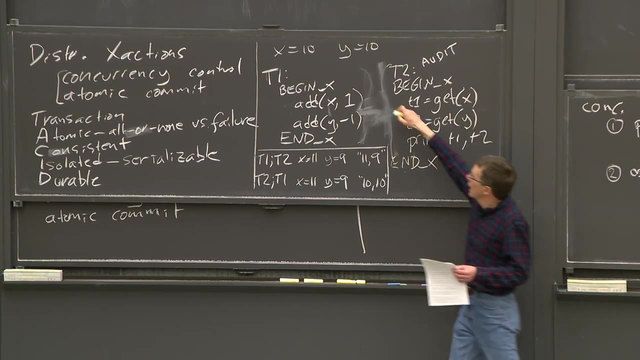 So what might happen if transactions did actually release locks as early as possible? So suppose T2 here reads X and then immediately releases its lock on X, That would allow T1, since now, at this point in the execution, T2 doesn't hold any locks. 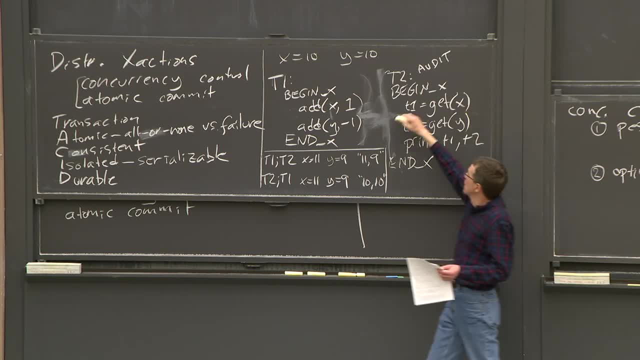 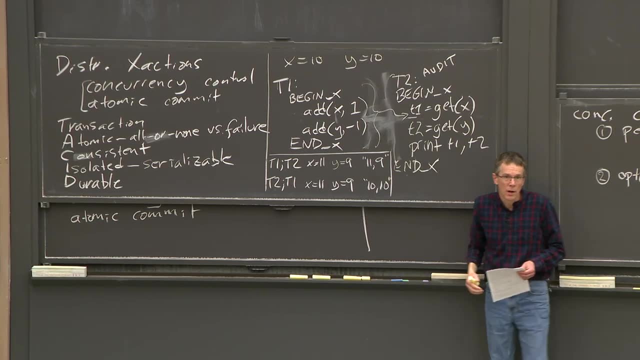 because it's just released- illegally released- the lock on X. Since it holds no locks, that means T1 could completely release the lock on X. T1 could completely execute right here And we already knew from before that this interleaving is not correct as it doesn't. 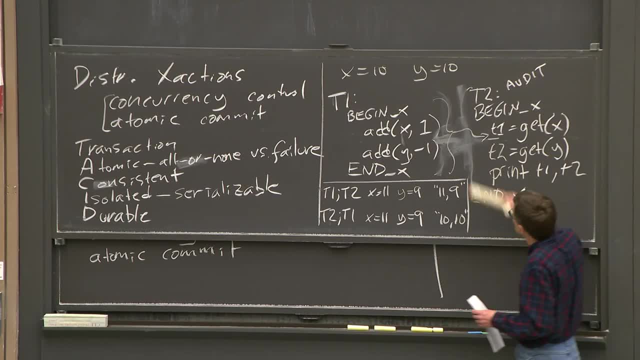 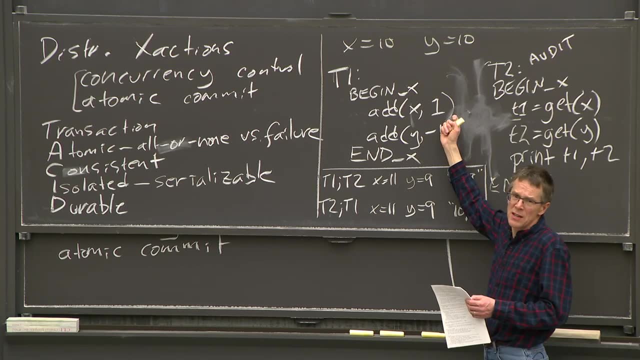 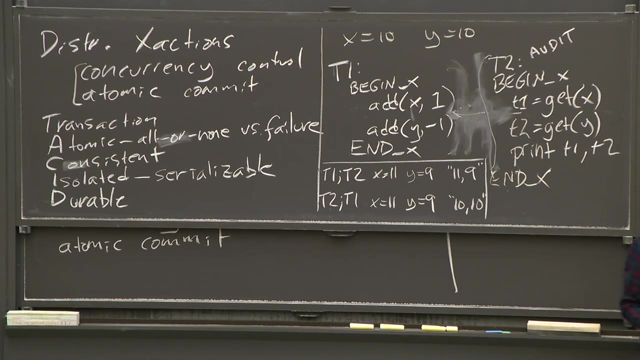 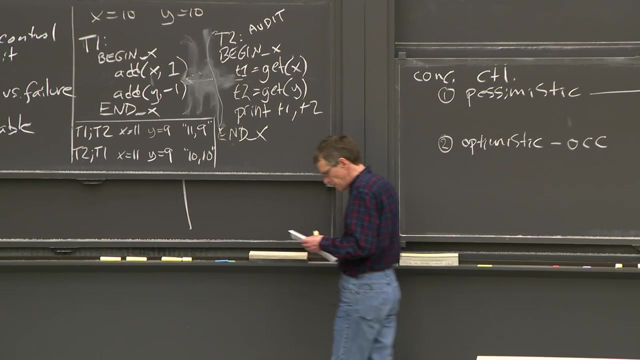 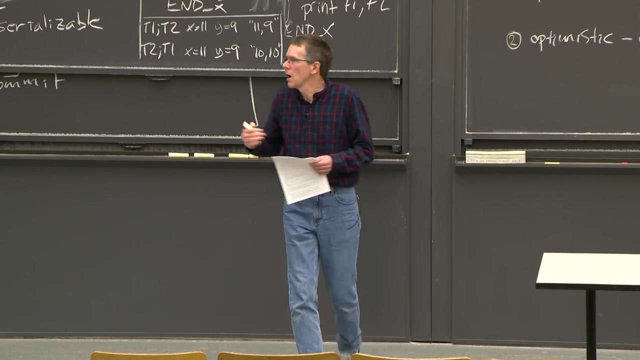 produce either of these two outputs. Similarly, if T1 released its lock on X after it finished adding 1 to X, that would allow all of T2 to slip in right here, And we know also from before that that results in. There's an additional kind of problem that can come up with releasing locks after modifying. 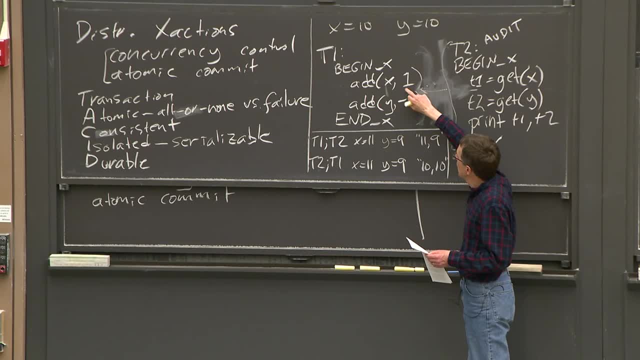 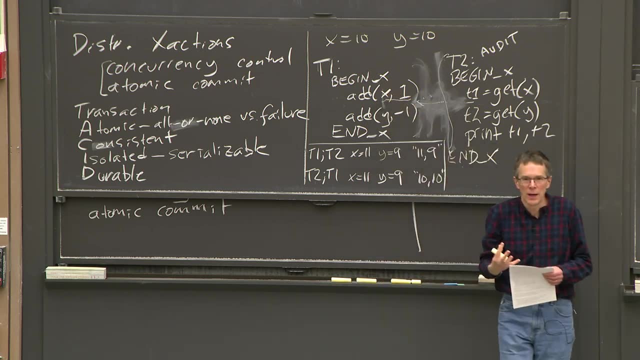 data. If T1 were to release the lock on X, it might allow T2 to see the modified version of X here, to see the X after adding 1 to it and to print that output and then for T2 to complete. 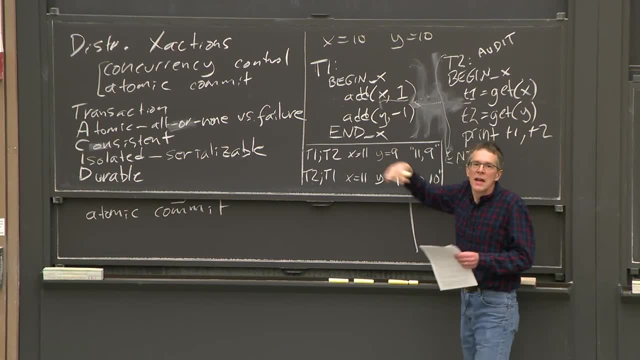 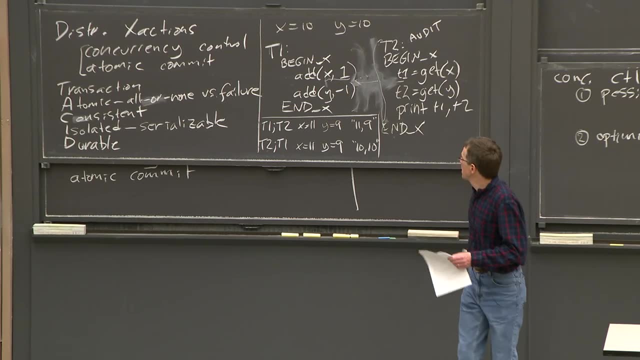 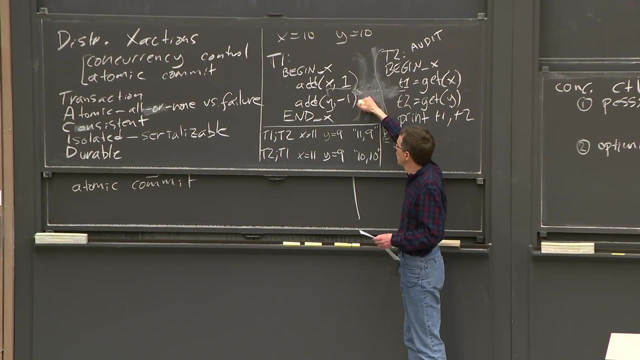 after printing the incremented value of X, If transaction 1 were to abort after that point, maybe because bank balance Y doesn't exist? or maybe bank balance Y exists but its balance is 0, and we're not allowed to decrement below 0 for bank balances because that's an overdraft. 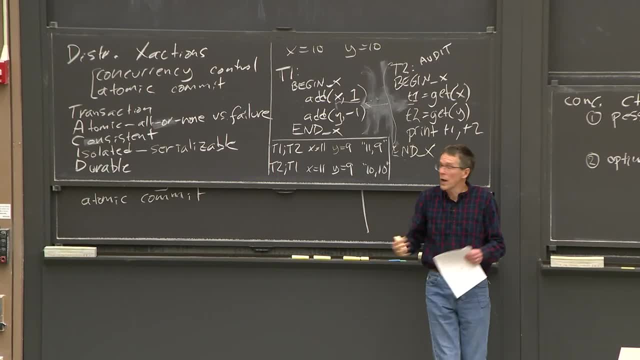 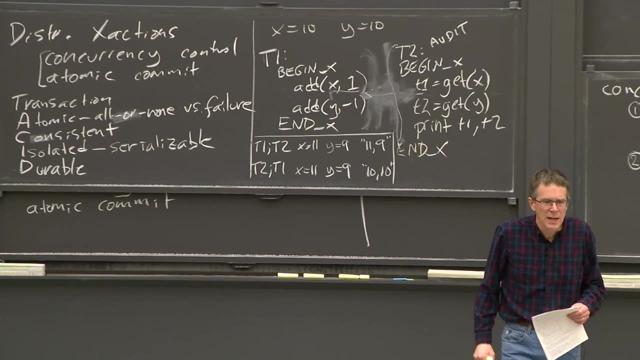 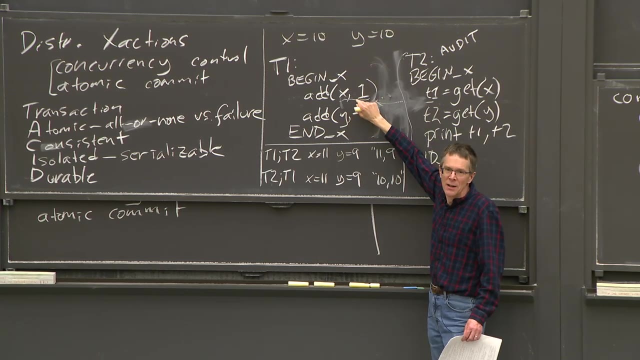 So T1 might modify X, then abort, and part of the abort has to be undoing its update to X in order to maintain atomicity. And what that would mean if it released the locks is that transaction 2 would have seen this sort of phantom value of 11 that went away because T1 aborted. 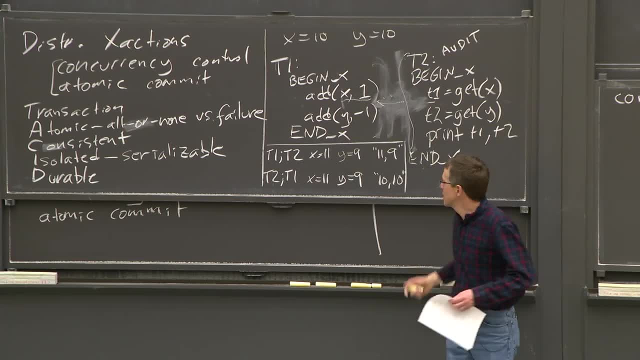 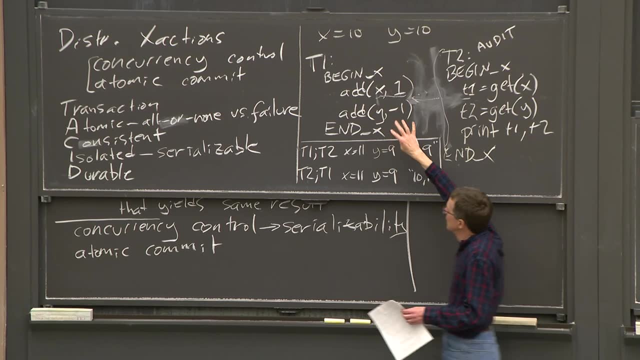 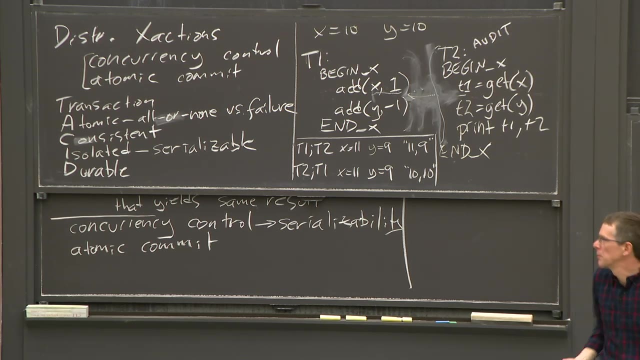 It would have seen a value that, according to the rules, never existed, right? Because then the transaction 1 aborts, then it's as if it never existed, and so that means the results from T2 had better be as if T2 ran by itself, without T1 at all. 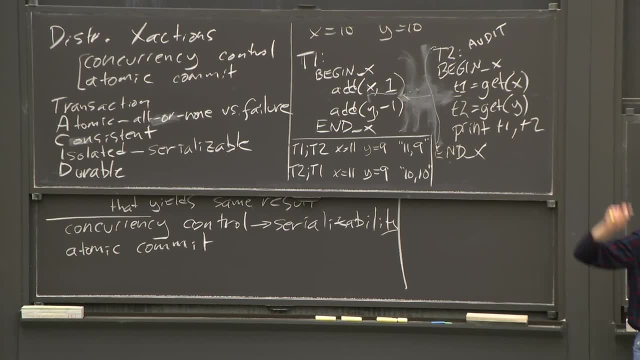 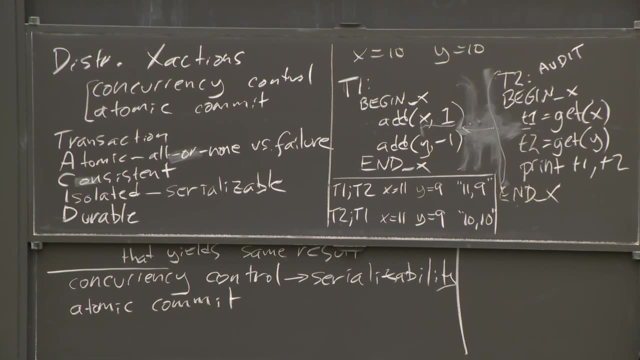 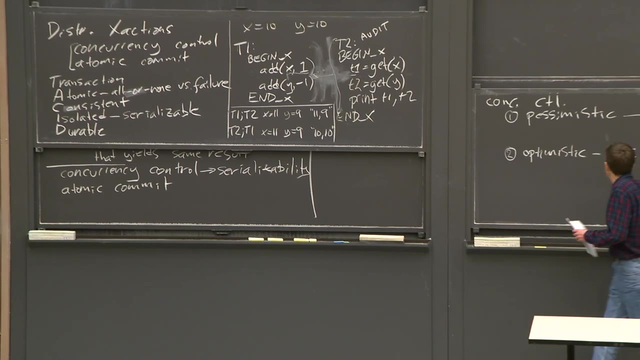 But if it sees the increment, then it's going to print 11 for X, 11, 10 actually, which is It just doesn't correspond to any state in the database, given that T1 didn't really complete. Okay, so that's why those are two dangers that are averted, two violations of serializability. 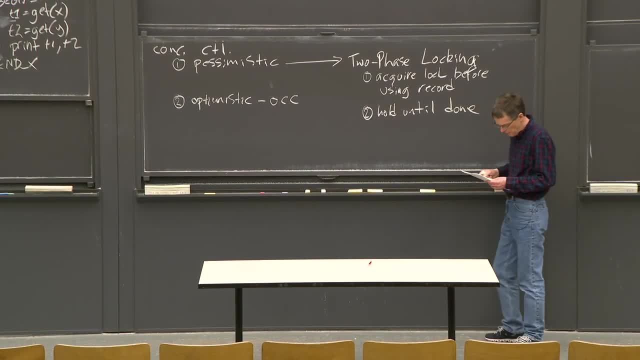 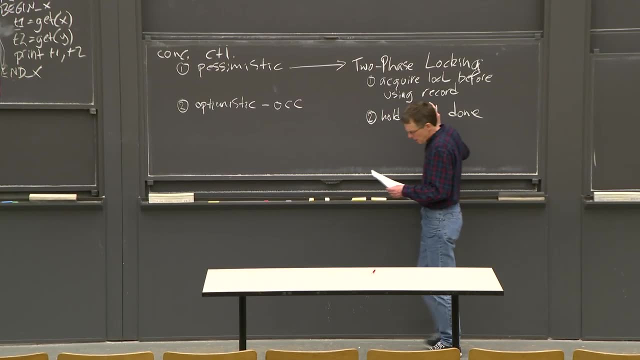 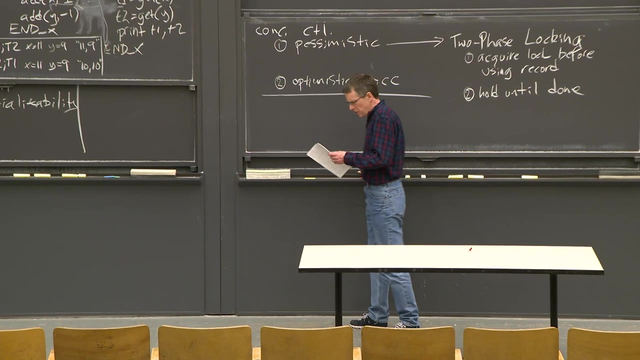 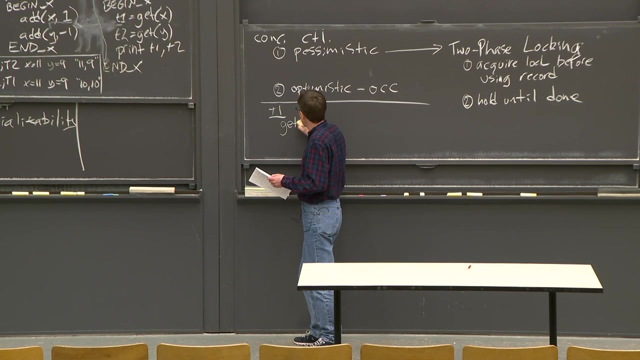 that are averted because transactions hold the locks until they're done. A further thing to note about these rules are that it's very easy for them to produce deadlock. So, for example, if we have two transactions, one of them reads record X and then reads: 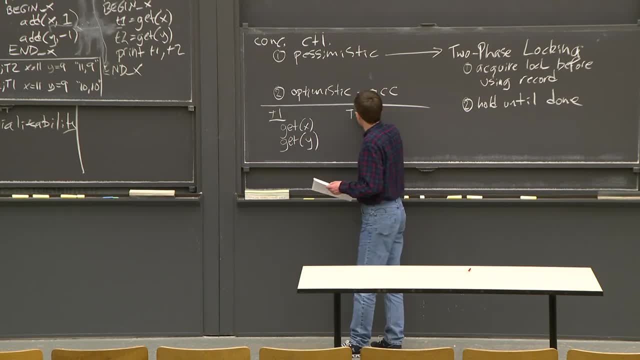 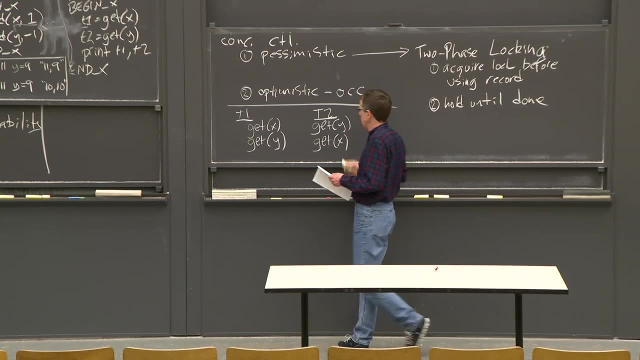 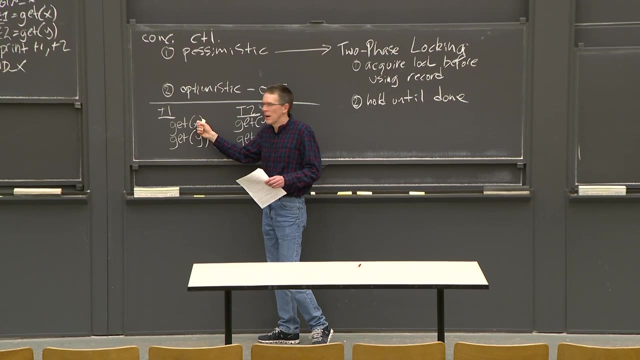 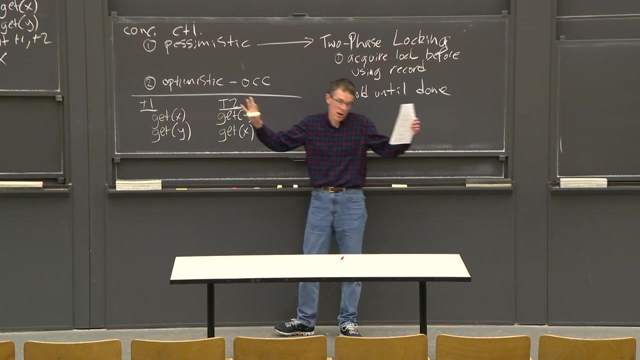 record Y and the other transaction reads Y and then X. that's just a deadlock. if they run at the same time, Each of them gets this lock on the record. Okay, So they both sit there waiting for the lock that's held by the other transaction and 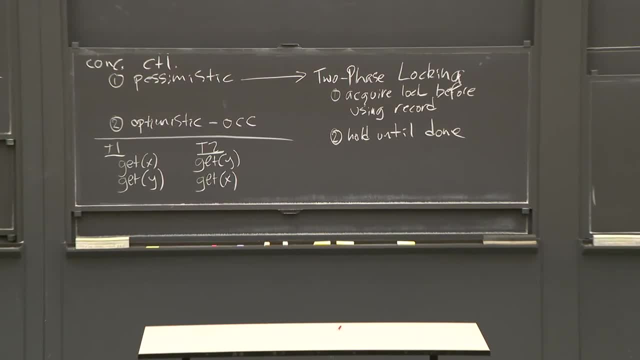 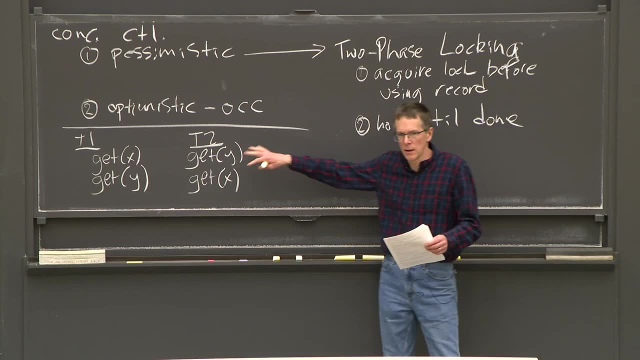 unless the database does something clever- which it will- they'll deadlock forever And, in fact, transactions have various strategies, including tracing cycles or timeouts, in order to detect that they've gotten into this situation. the database will abort one of these two transactions. 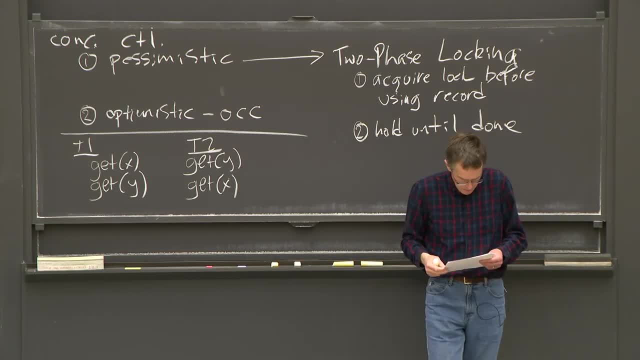 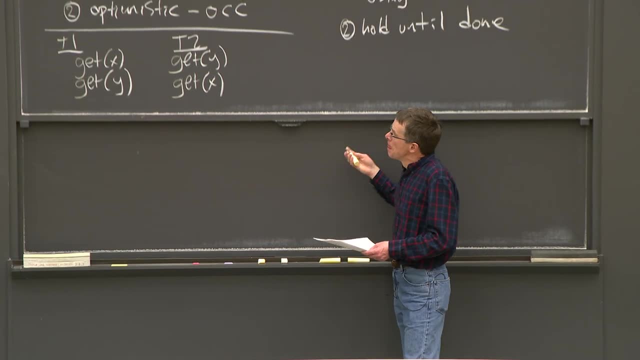 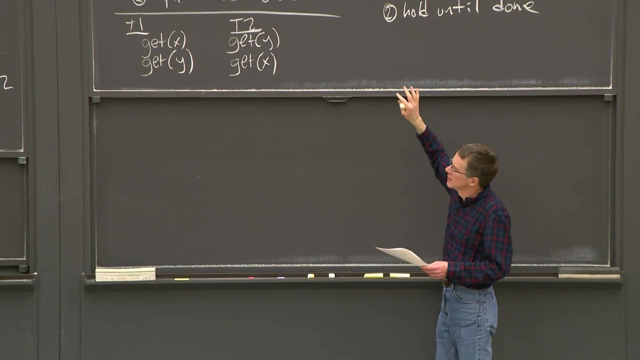 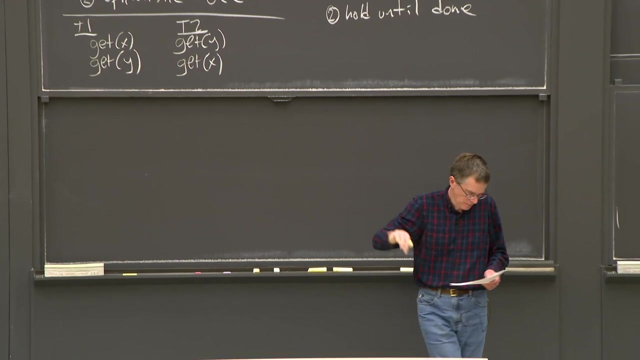 and undo all its changes and act as if the transaction had never occurred. Okay, So that's concurrency control with two-phase locking, And this is just completely standard database behavior so far and is the same in single machine databases as it will be in distributed databases that are of little more interest. 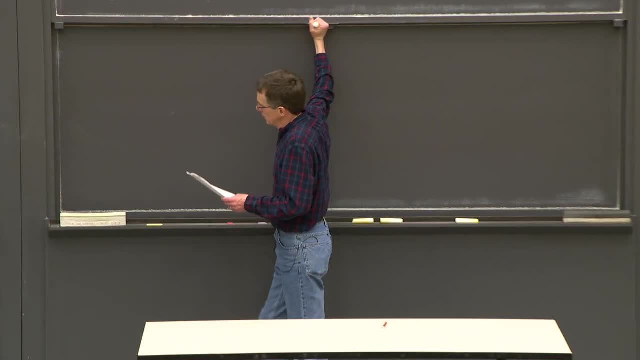 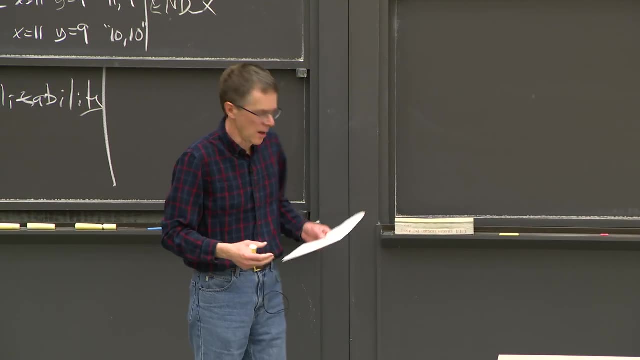 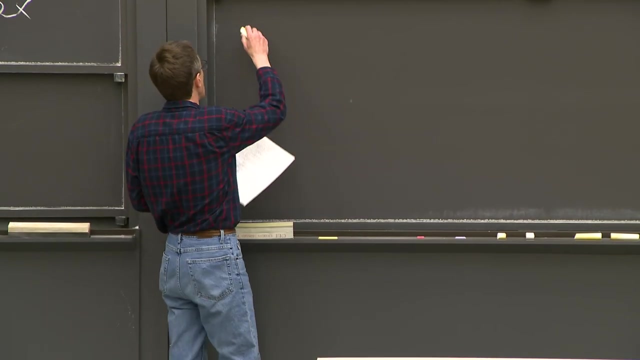 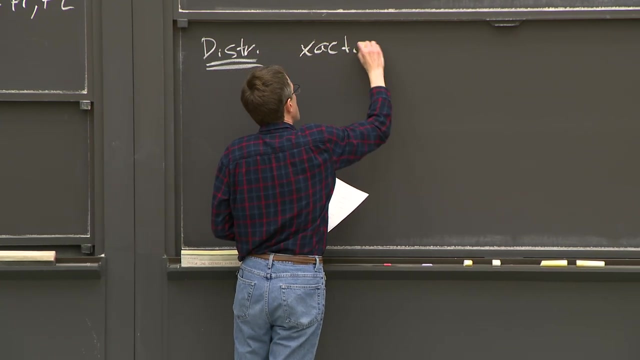 to us, But our next topic is a littleis Okay, Okay. So the next topic is a little bit more specific to building databases or storage systems in general that support transactions on distributed setting, that is, splitting the data over multiple machines. So now the topic is how to build distributed transactions and, in particular, how to cope. 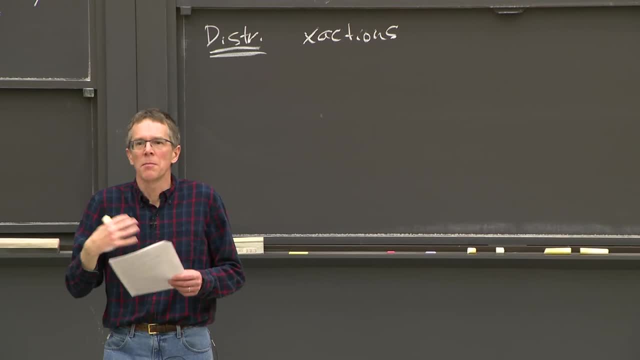 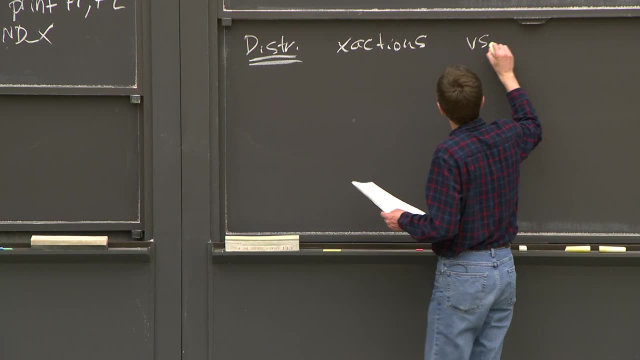 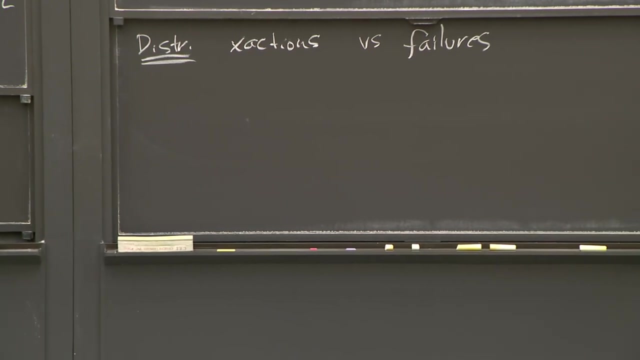 with failures and more specifically the kind of partial failures of just one of many servers that you often see in distributed systems. So we have distributed transactions and we're worried about how they behave and make sure they're serializable and also have sort of all or nothing atomicity even in the face. 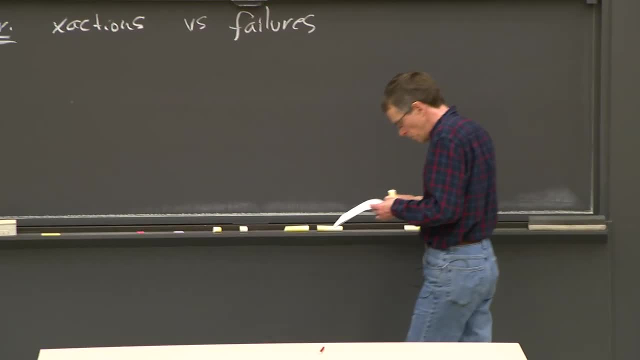 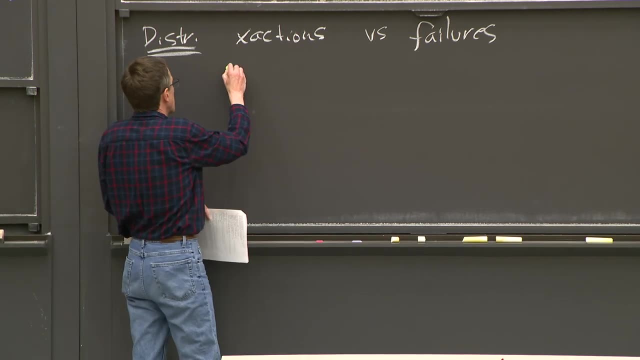 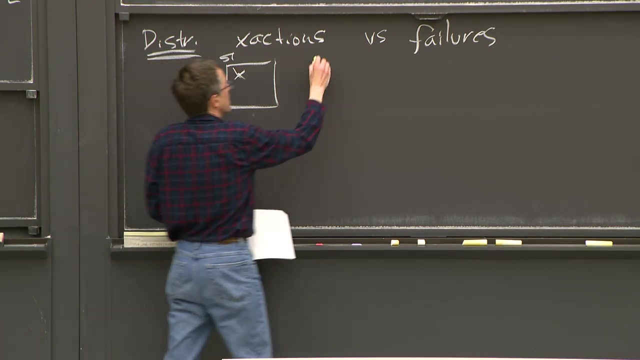 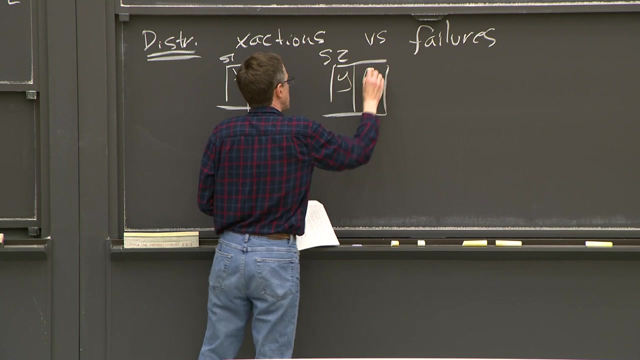 of failures. So you know, the way this looks like is that we might have two servers. right, we got server one and maybe it stores record X in our bank, and we have server two and maybe it stores record Y, So they all start out with value 10, and we need to run these two transactions. 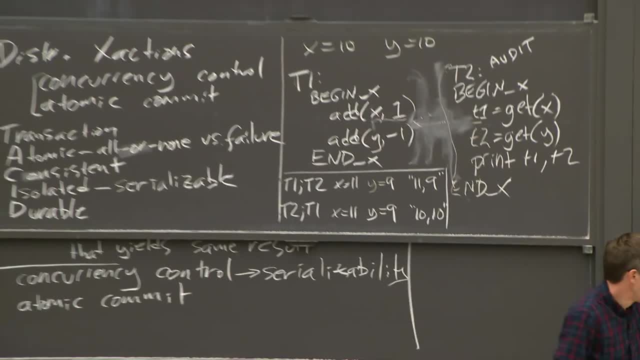 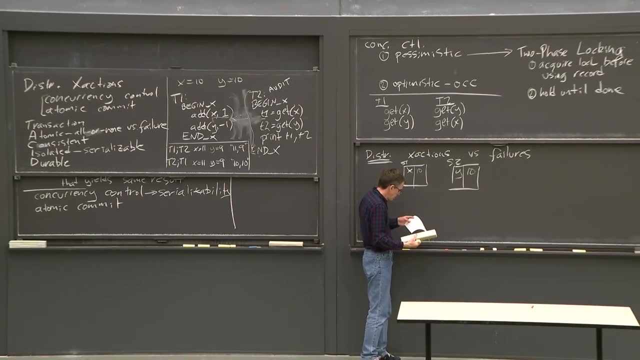 And transaction one, of course, modifies both X and Y. So now we need to send messages to the databases saying: oh, please increment X, please decrement Y. But it would be easy, if we weren't careful, to get into a situation where we had told: server one to increase X, So we increase the balance for X, but then something failed. Maybe the client's sending the requests, or maybe server two that's holding Y fails, or something, And we never manage to do the second update right. 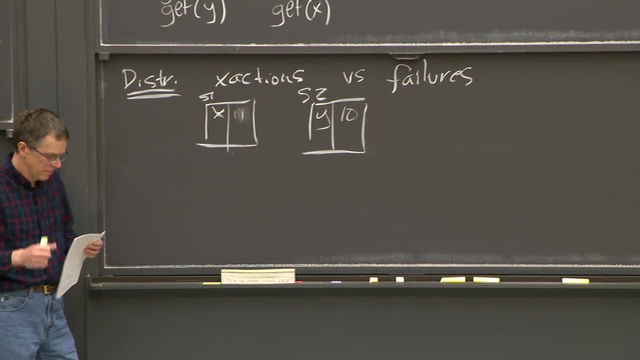 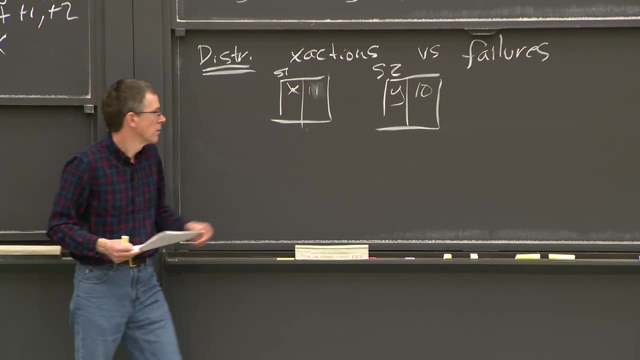 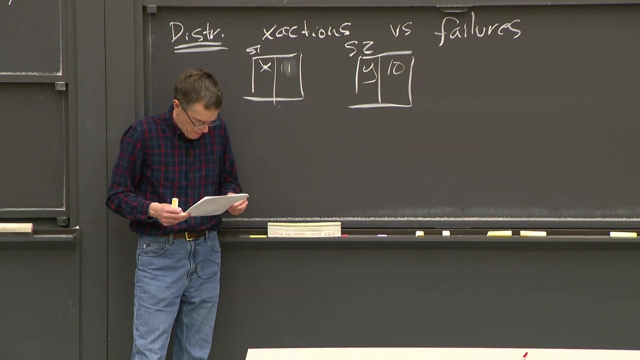 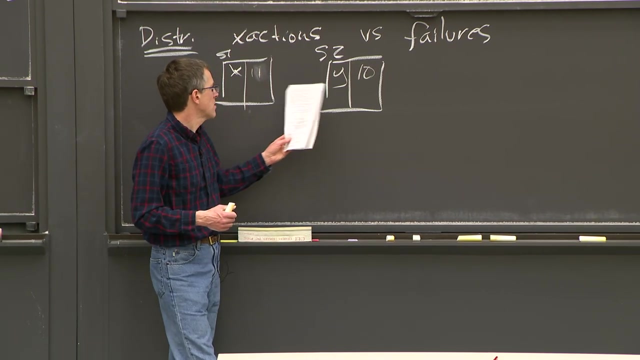 So that's one problem is failure somewhere may sort of cut the transaction in half, And if we're not careful it calls only half of the transaction to actually take effect. All right, Thanks. This can happen even without crashes. If X does its part in the transaction, it could be that over on server two, server two, 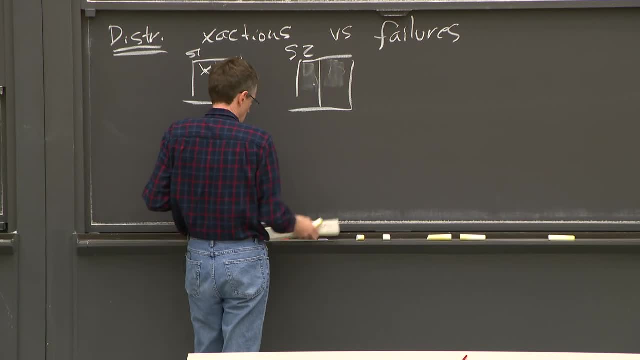 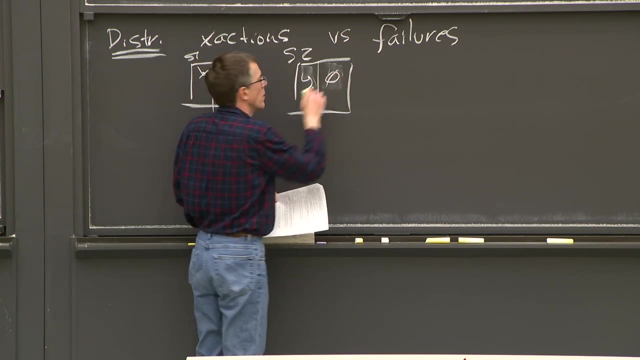 actually gets the request to decrement bank account Y, but maybe server two discovers this bank account doesn't exist, or maybe it does exist and its balance is already zero and can't be decreased and so it can't do its part of the transaction. 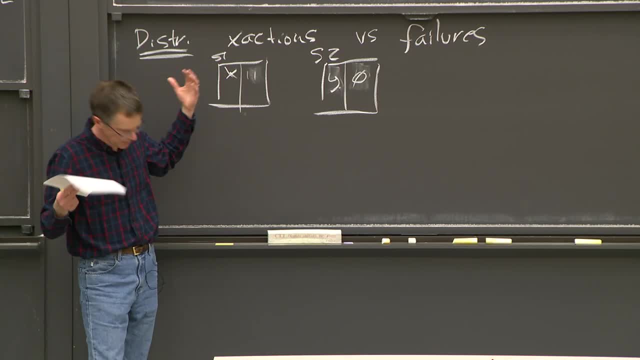 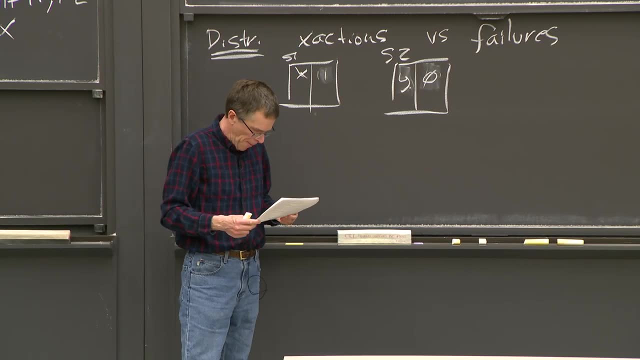 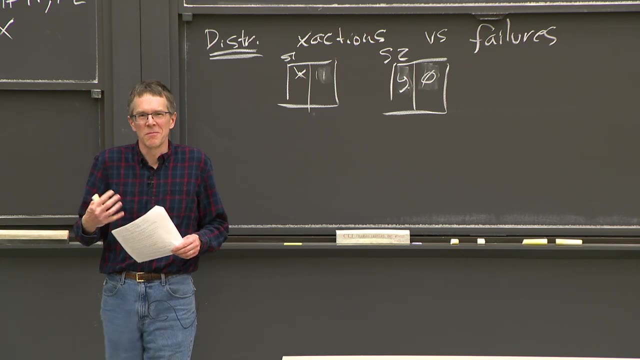 But X look has already done its part of the transaction. Okay, So that's a problem that needs to be dealt with. So the property we want, as I mentioned before, is that all the pieces of the system, either, all the pieces of the system. 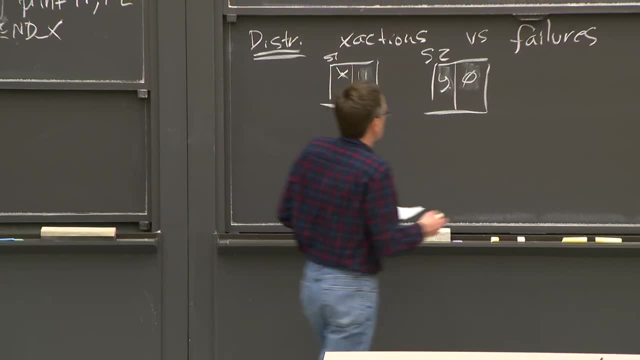 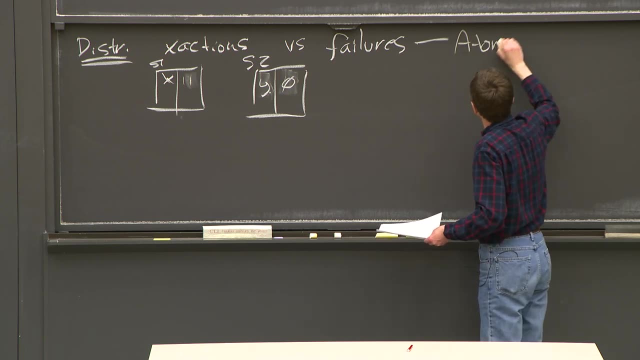 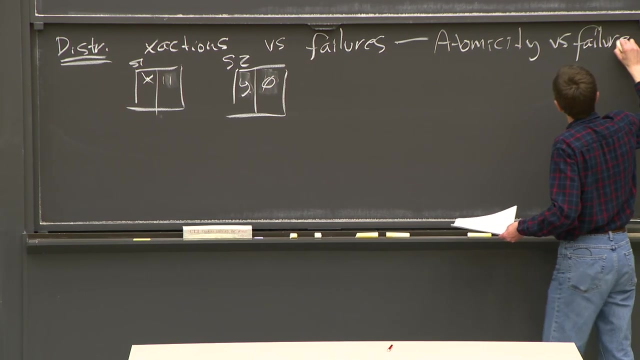 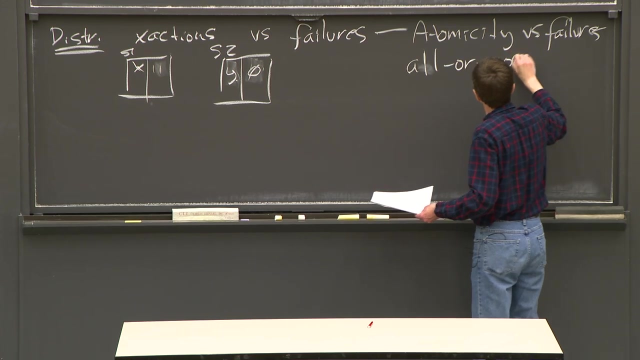 should do their part of the transaction or none, right? So the thing we've violated here is we want atomicity against crashes Or versus failures, Where atomicity is all or none- All parts of the transaction that we're trying to execute, or none of them. 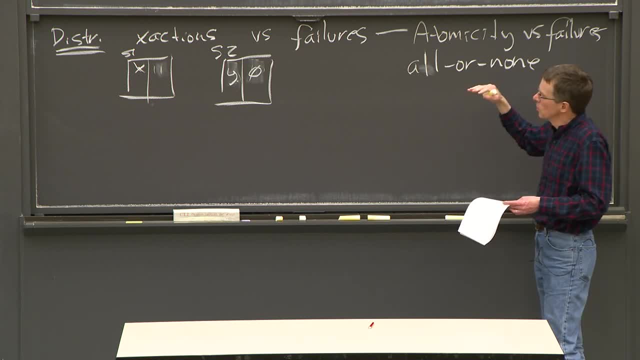 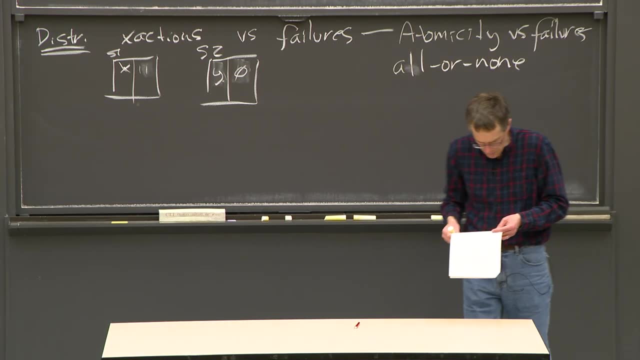 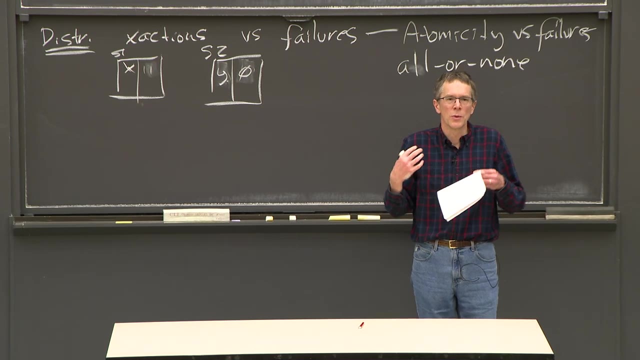 And for even more. the kind of solution we're going to be looking at is atomic commitments, atomic commit protocols, And the general kind of flavor of atomic commit protocols is that you have a bunch of computers that are all doing different parts of some larger task. 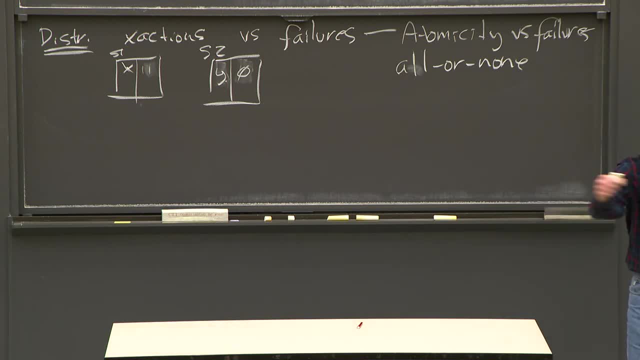 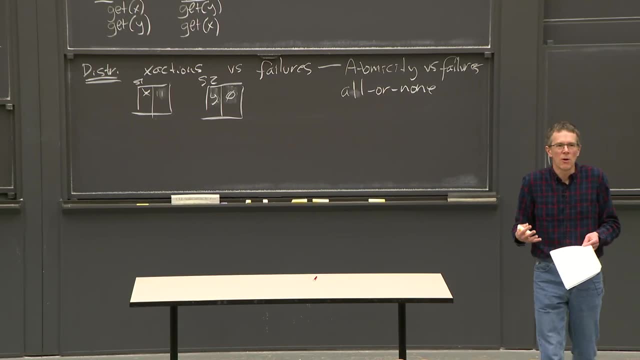 And the atomic commit protocol is going to help the computers decide that either they're all going to do their, they're all capable of doing their part and they're actually going to do it, Or something has gone wrong and they're all going to agree that. 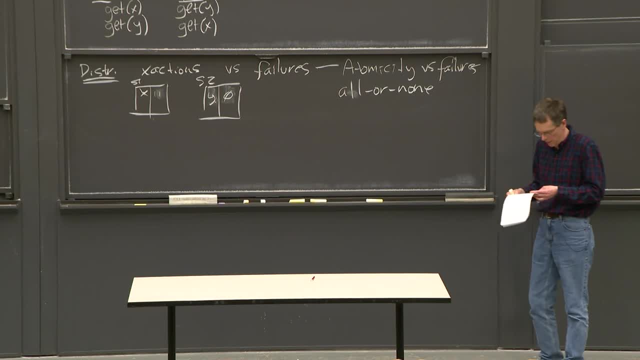 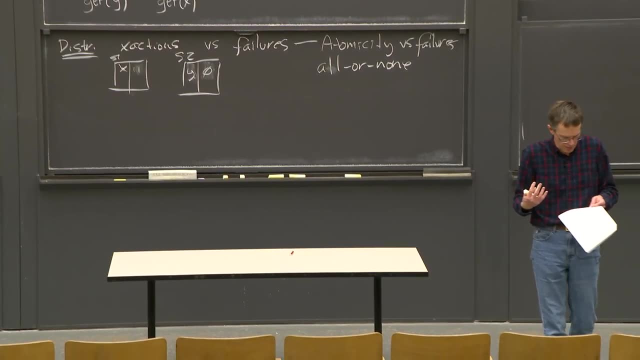 oh, actually, none of them are going to do their part of the. whatever the overall task is, And the big challenges are, of course, how to cope with various failures- machine failures, loss of messages- And it'll turn out that performance. 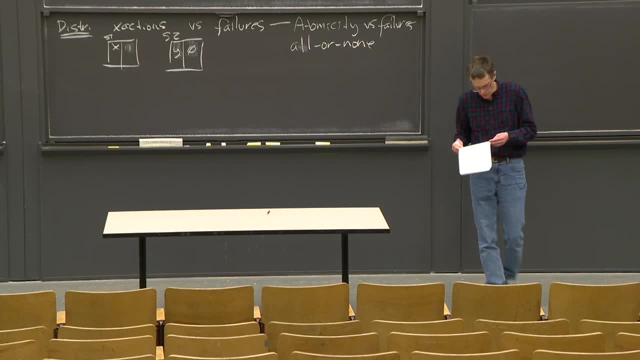 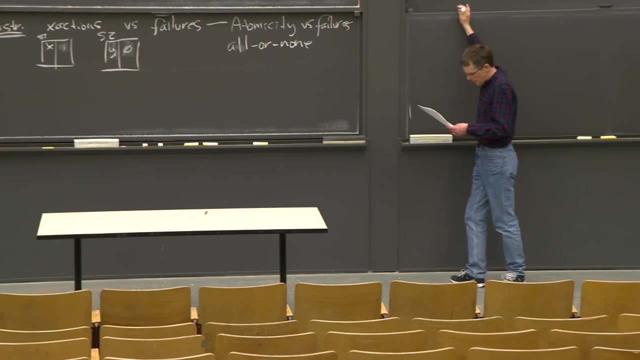 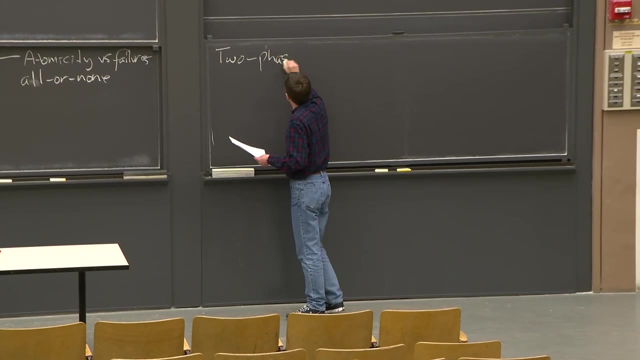 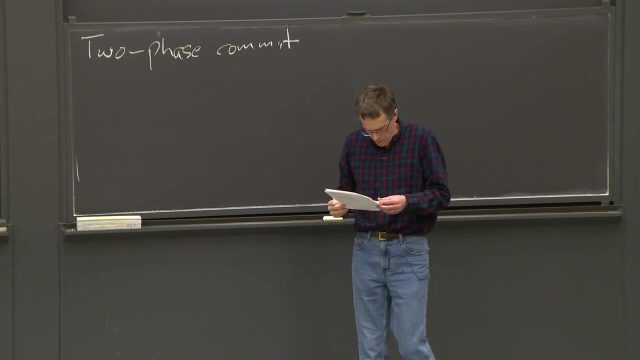 is also a little bit difficult to do a good job with. The specific protocol we're going to look at- and this is the protocol explained in a reading for today- our two-phase commit. This is an atomic commitment protocol And this is used both by distributed databases. 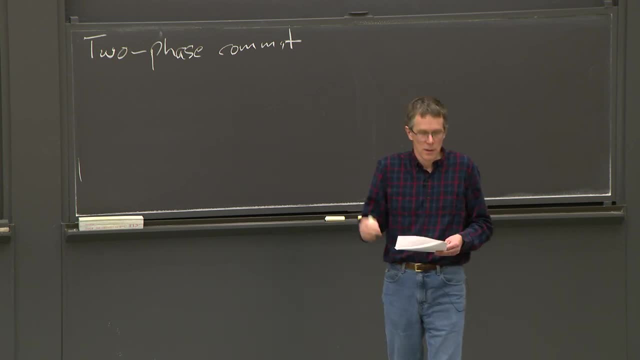 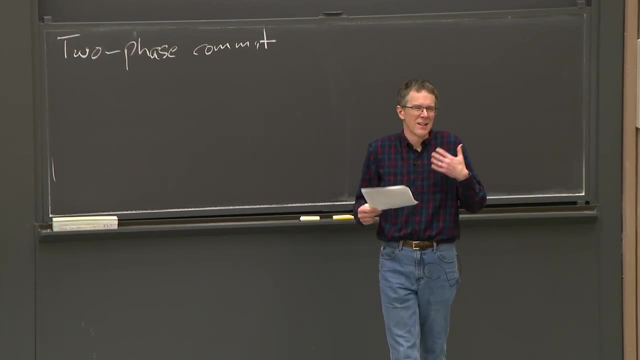 and also by all kinds of other distributed systems that might not at first look like traditional databases. The general setting is: we assume that, in one way or another, the task we need to perform is split up over multiple servers, each of which needs to do some part. 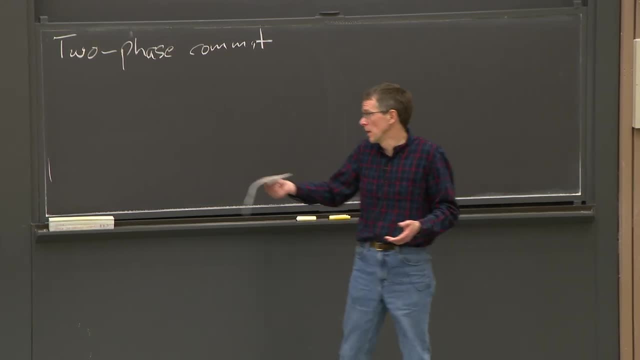 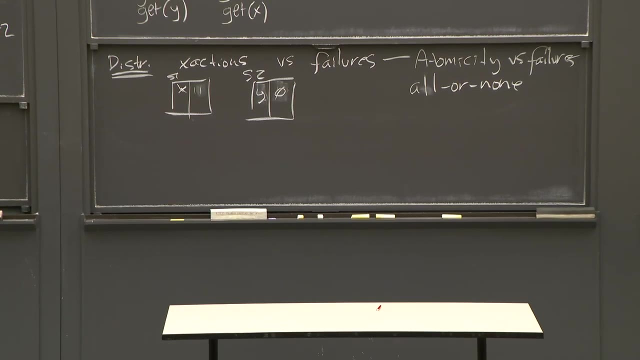 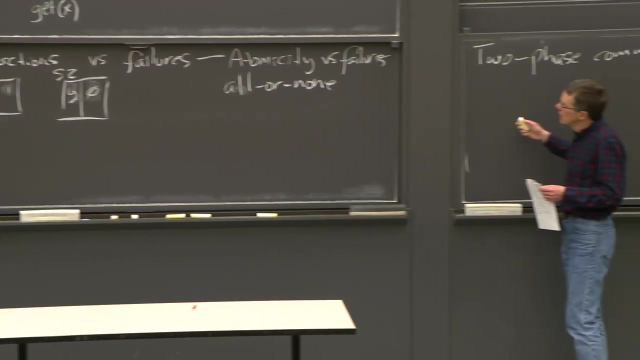 a different part each one of them. So, for example, this setup I showed here, in which it's really the data that's split up, and so the tasks being split up are incrementing X and decrementing Y. We're going to assume that there's one computer. 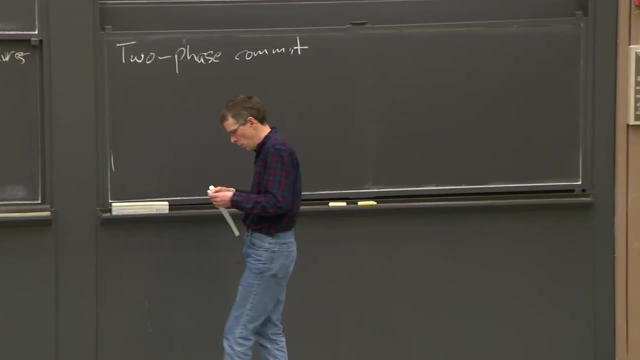 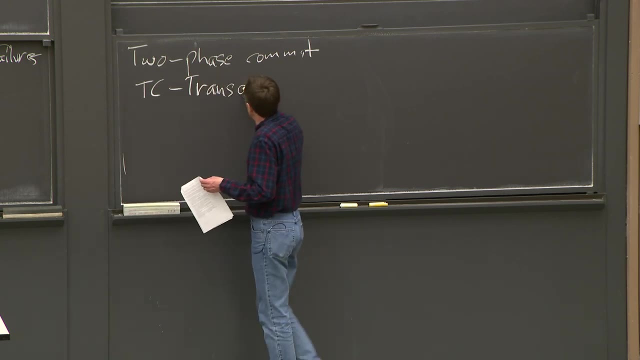 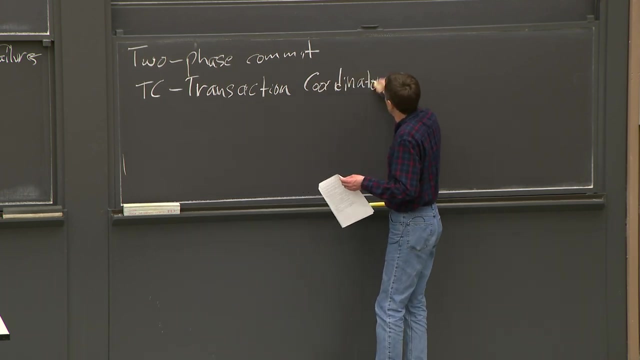 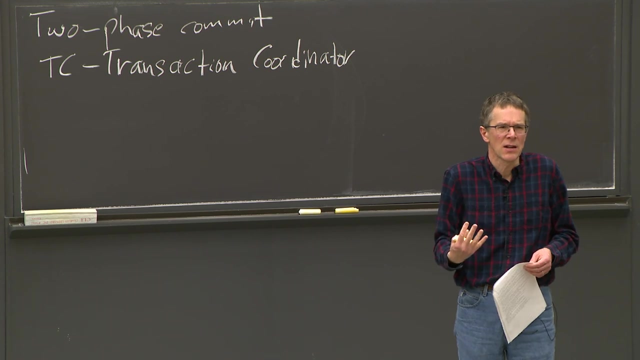 that's driving the transaction, called the transaction coordinator. There's lots of ways of arranging how the transaction coordinator steps in, but we'll just imagine it as a computer that's actually running the transaction. There's one computer, the transaction coordinator, that's executing the sort of code for the transaction. 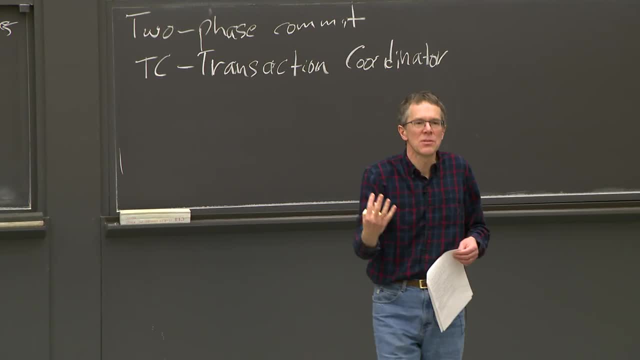 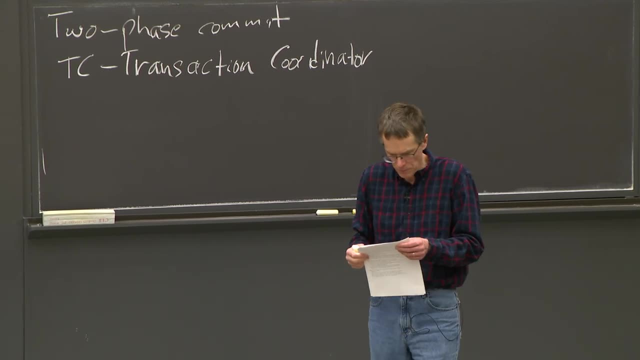 like the puts and the gets and the adds, and it sends messages to the computers that hold the different pieces of data that need to actually execute the different parts. So for our setup we're going to have one computer, the transaction coordinator. 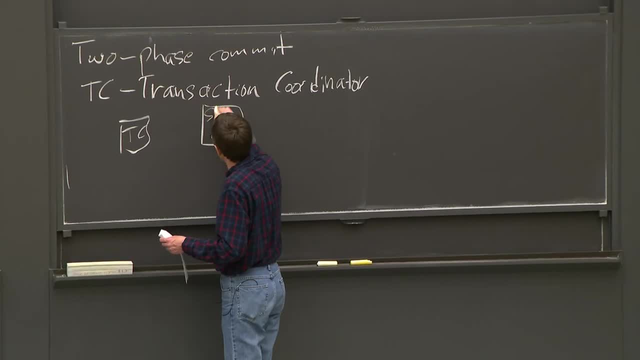 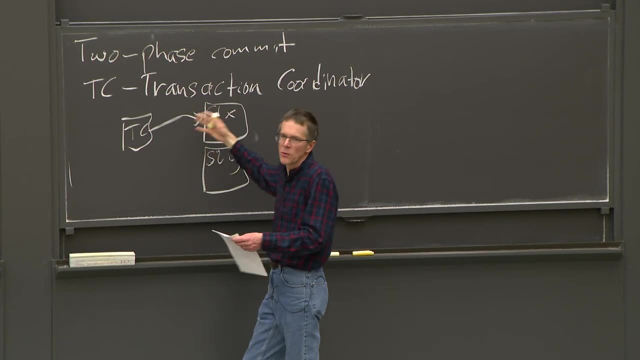 and it's going to be these server one and server two. So we're going to have one computer, the transaction coordinator, and it's going to be these server two that hold X and Y. The transaction coordinator will send a message to server one saying: 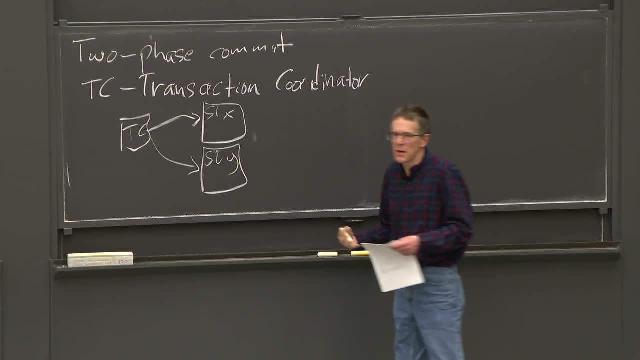 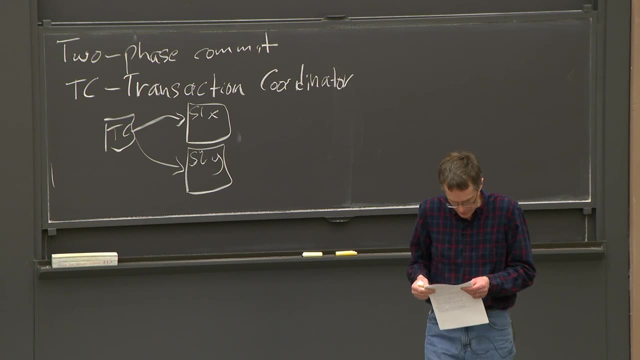 oh, please, increment X. send a message to server Y saying: oh please, decrement Y, and then there'll be more messages in order to make sure that either they both do it or neither of them do it. and that's where two-phase commit steps in. 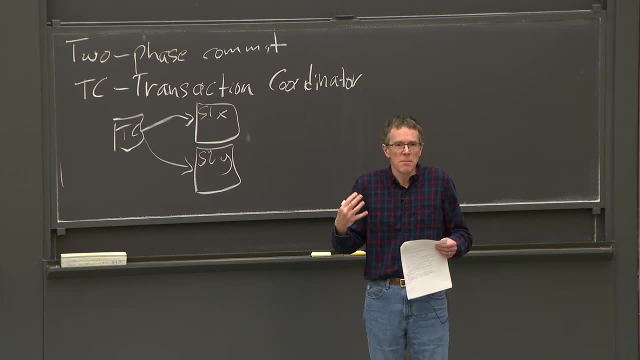 Something to keep in the back of your mind is that in the full system there may be many different transactions running concurrently and many transaction coordinators sort of executing their own transactions, And so the various parties here need to keep track of. 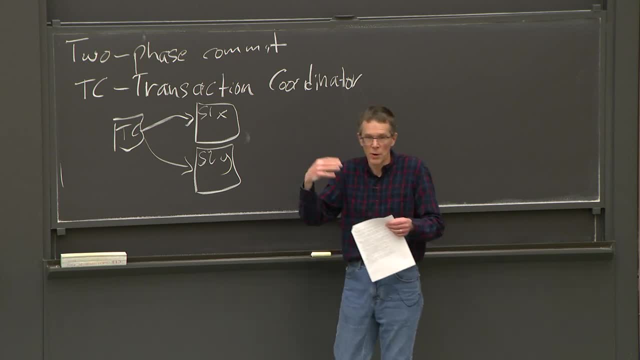 oh, you know, this is a message for such and such a transaction, and where they keep state like these turns out these servers are going to maintain tables of locks, for example, and when they keep state like that, they need to keep track of. 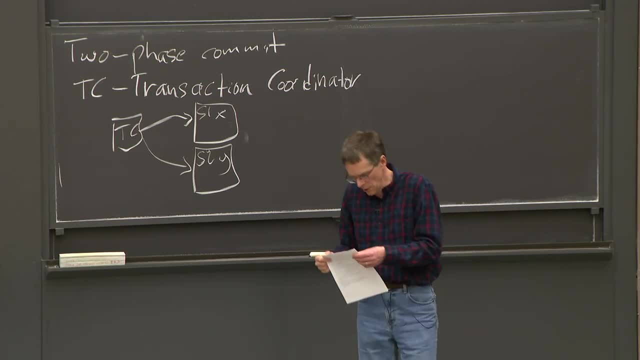 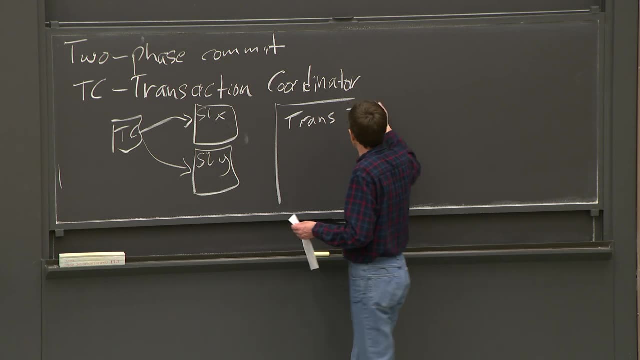 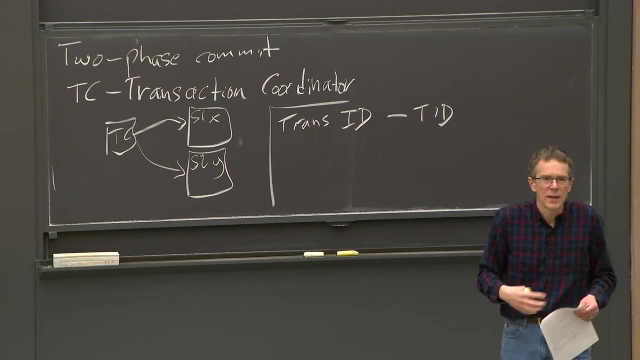 oh, this is a lock that's being held for transaction 17.. So there's a notion of transaction IDs, or TID, and I'm just going to assume- although I'll, you know, not actually show it- that every message in the system. 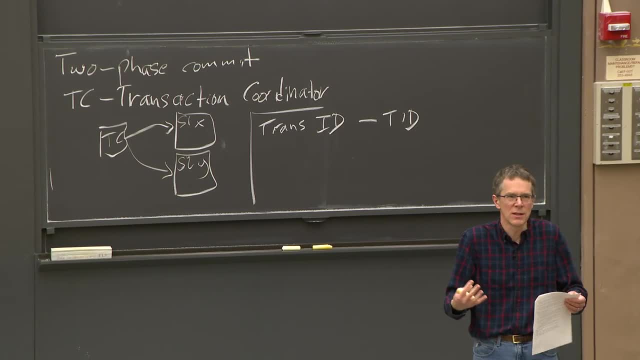 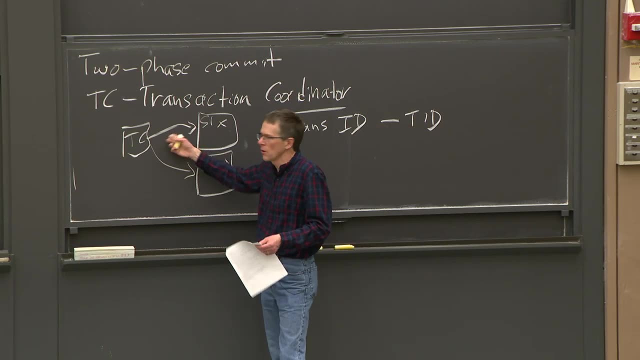 is tagged with the transaction with the unique transaction ID of the transaction it applies to, and these IDs are chosen by the transaction coordinator. when the transaction starts, The transaction coordinator will send out: oh, this is a message for transaction ID 95,. 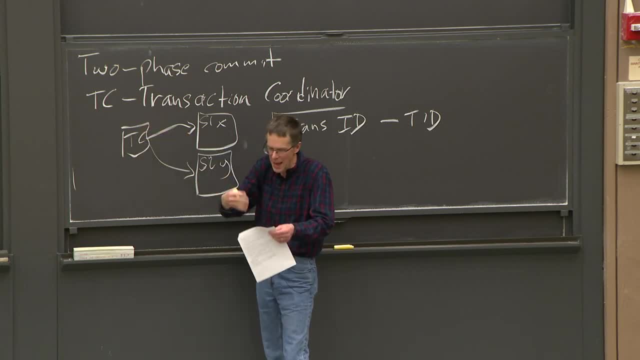 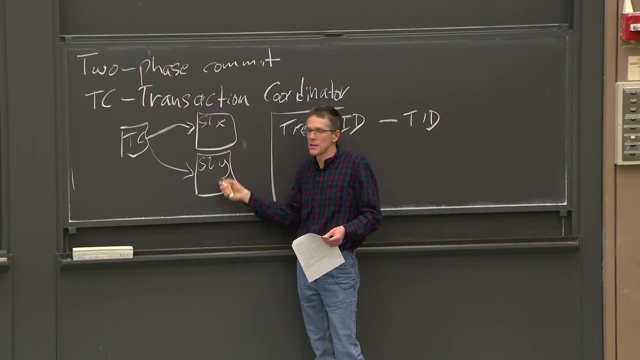 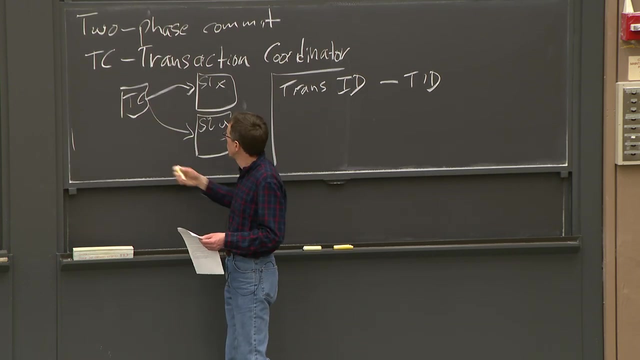 and it'll keep all its state here about the transaction will be tagged with 95, and the various tables in the different participants in the transaction will be tagged with the transaction IDs, And so that's another piece of terminology We have the transaction coordinator. 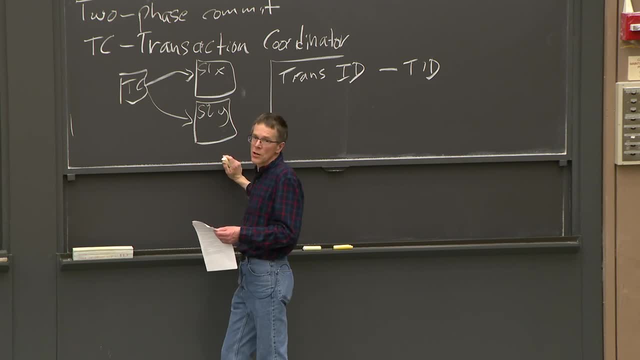 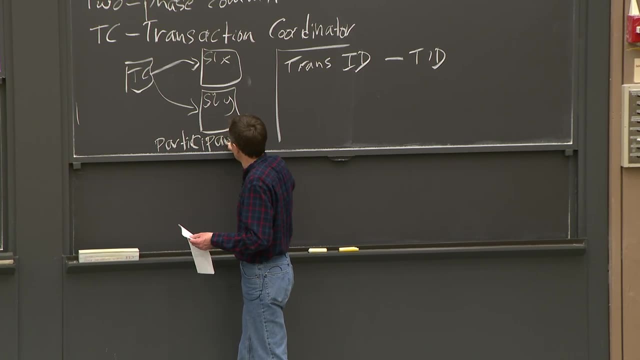 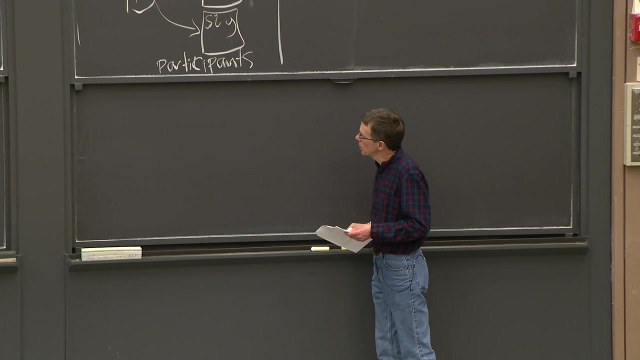 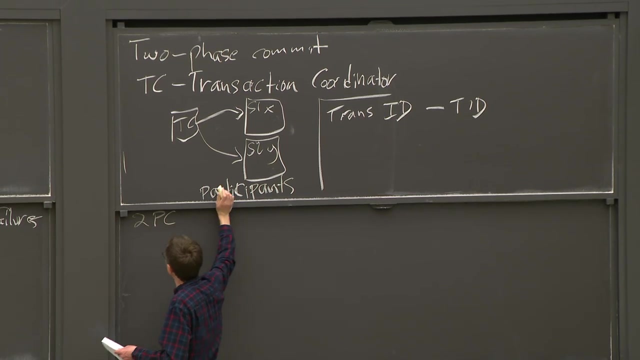 and then the other servers that are doing parts of the transaction are called participants. All right, So let me draw out the two-phase commit protocol example execution. So this is- I'll abbreviate this- 2PC for two-phase commit. 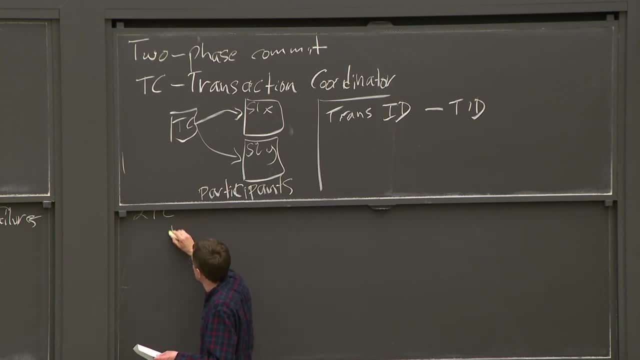 The parties involved are the transaction coordinator and we'll just say there's two participants, That is, you know. maybe we're executing the transactions I've shown. X and Y are on different servers. Maybe we've got participant A and 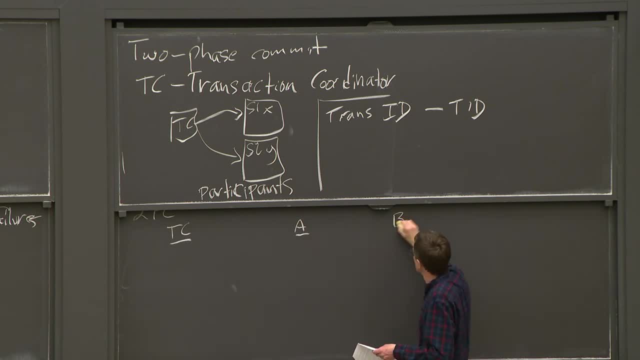 and and participant B. These are two different servers holding data. So the transaction coordinator, it's running the whole transaction. It's going to send puts and gets to A and B to tell them to. you know, read the value of X or Y. 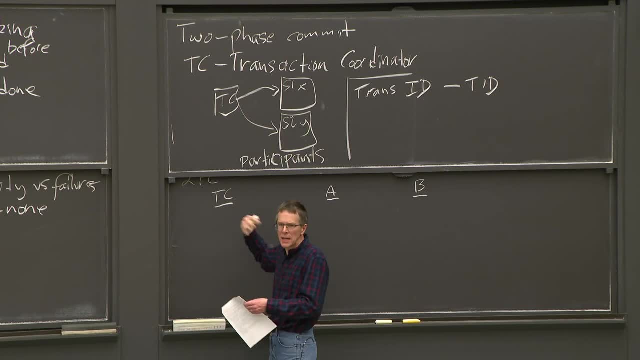 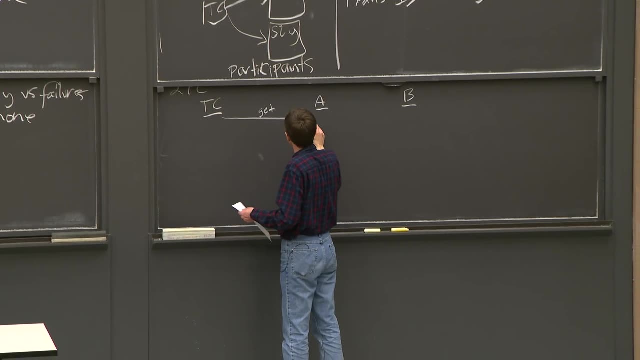 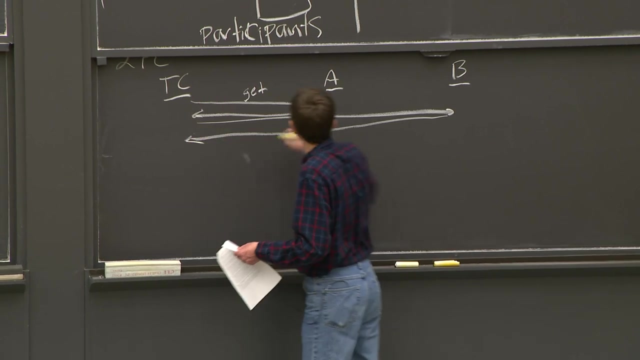 or add one to X. So we're going to see at the beginning of the transaction that the transaction coordinator is sending, for example, maybe a get request to participant A and it gets a reply, and then maybe it sends so that put for whatever. 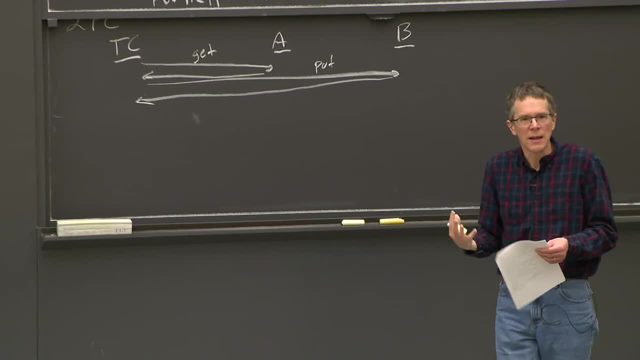 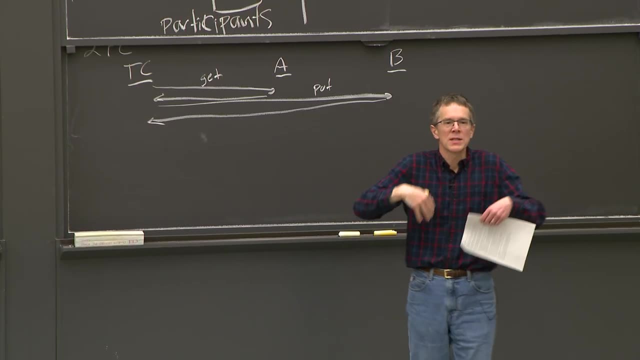 And we might see a long sequence of these. if there's a complicated transaction, Then when transaction coordinator gets to the end of the transaction and wants to commit it and be able to, you know, release all those locks and make the transaction's results visible. 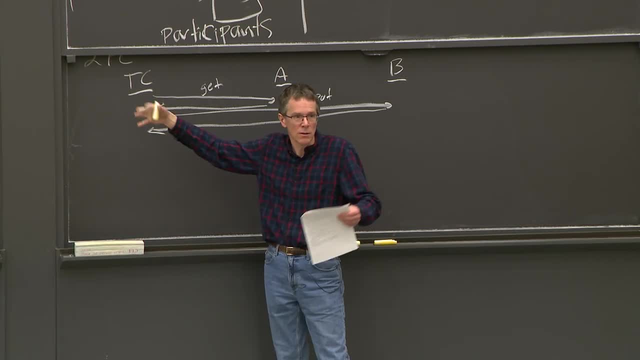 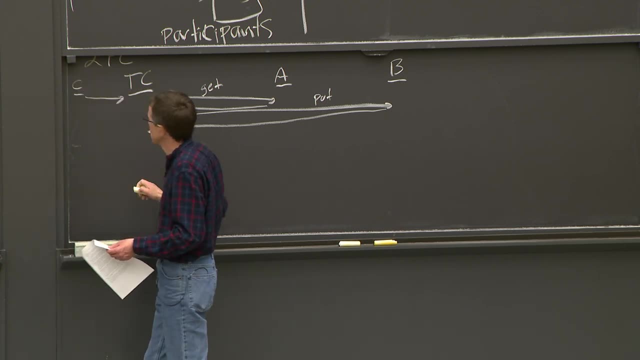 to the outside world and maybe reply to a client or a human user. So maybe we're assuming there's a sort of external client or human, a human that said, oh, please run this transaction and is waiting for a response, And before we can do any of that, 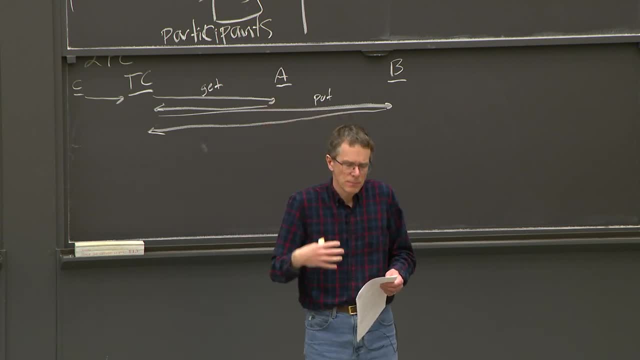 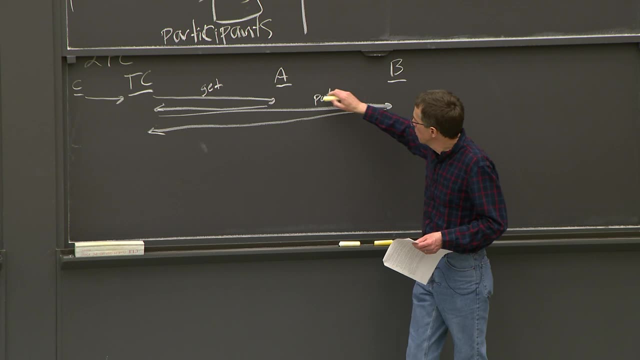 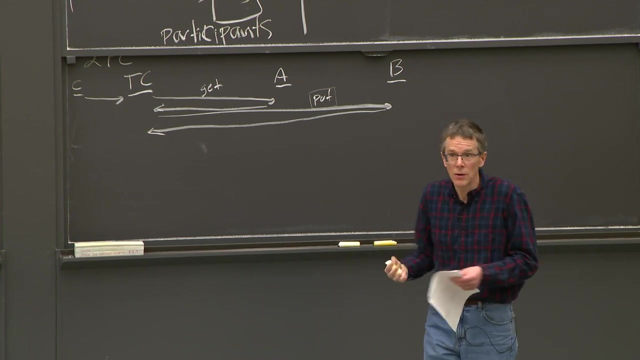 the transaction coordinator has to make sure that all the different participants can actually do their part of the transaction And, in particular, if there were any puts in the transaction, we need to make sure that the participants who are doing those puts well are actually still capable of doing the puts. 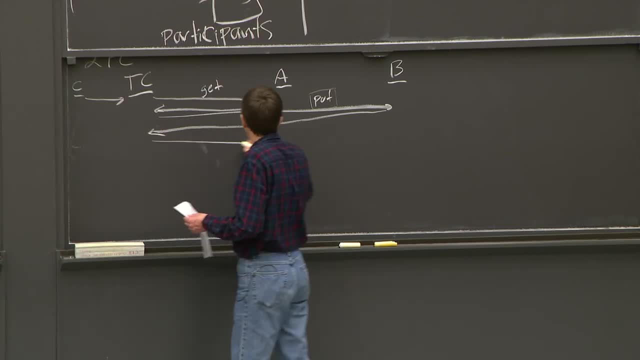 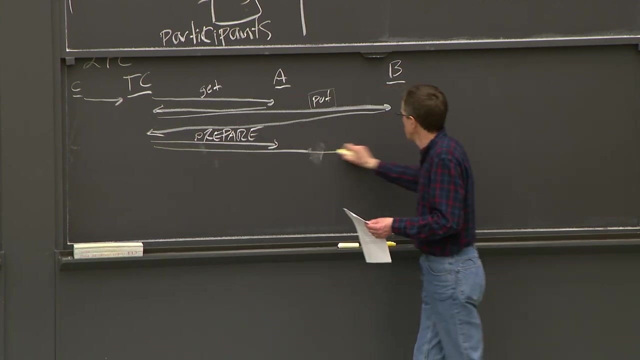 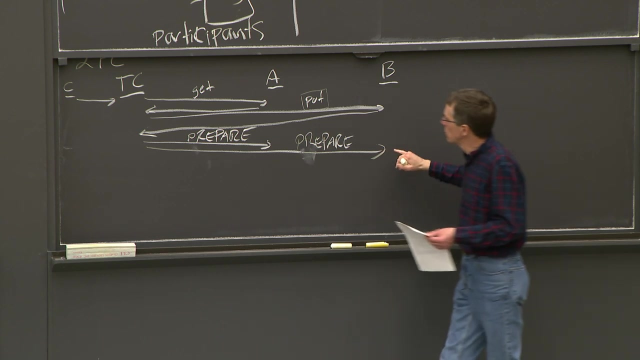 So, in order to find that out, the transaction coordinator sends prepare messages to all of the participants. So we're going to send prepare messages to both A and B, And when A or B receive a prepare message, you know they know the transaction is nearing completion. 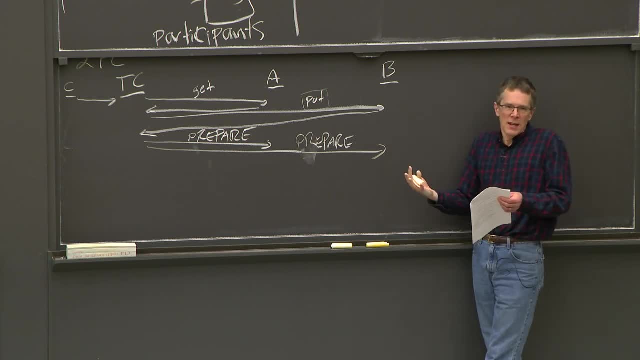 but not over yet. They look at their state and decide whether they are actually able to complete the transaction. You know, maybe they needed to abort it to break a deadlock, or maybe they've crashed and restarted between. you know when they did the last operation, or now. 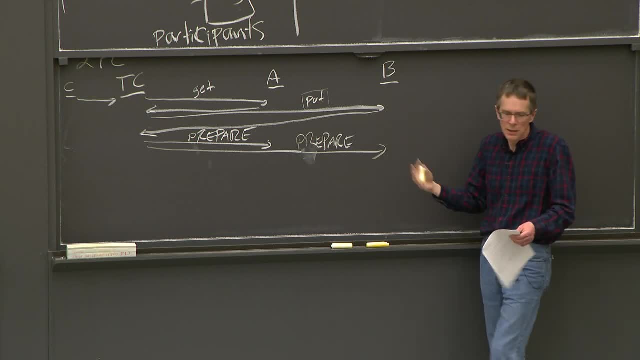 and they've completely forgotten about the transaction and can't complete it. So A and B, you know, look at their state and say, oh, I'm going to be able to or I'm not going to be able to do this transaction. 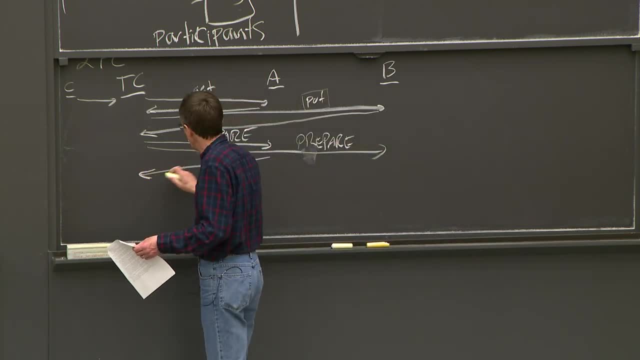 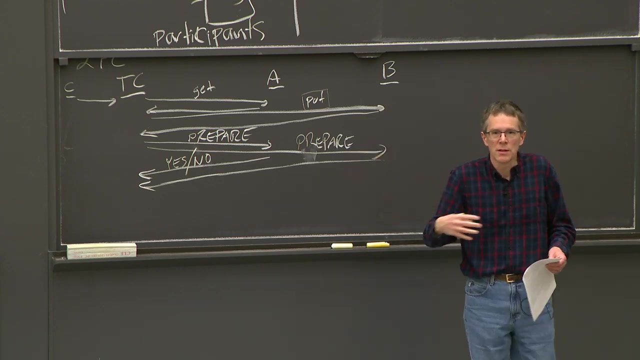 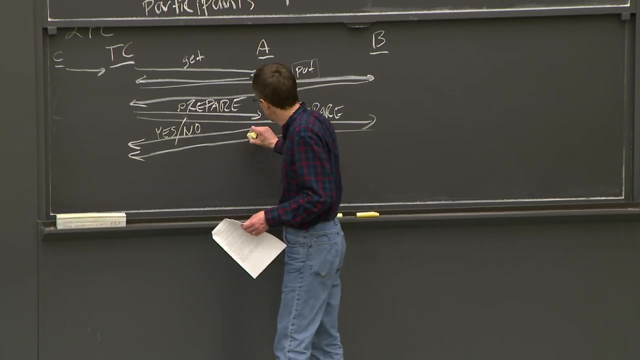 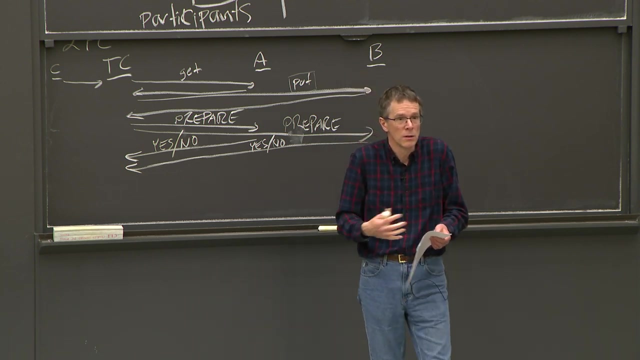 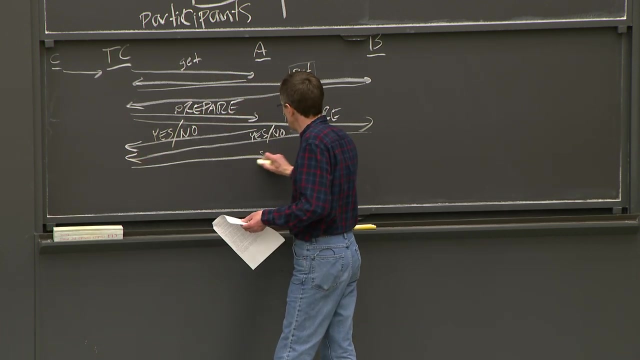 And they respond with either yes or no. So the transaction coordinator is waiting for these yes or no votes from each of the participants. If they all say yes, then the transaction can commit. Nothing goes wrong. The transaction can commit and the transaction coordinator sends out a commit message. 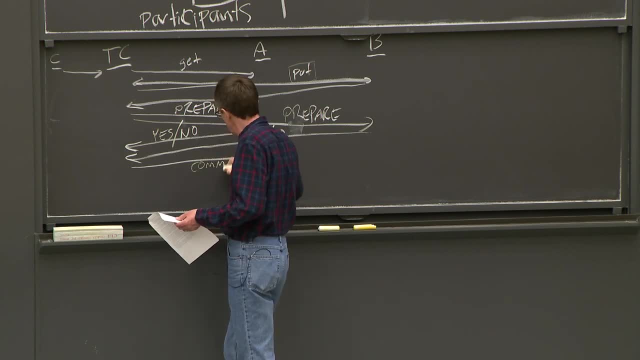 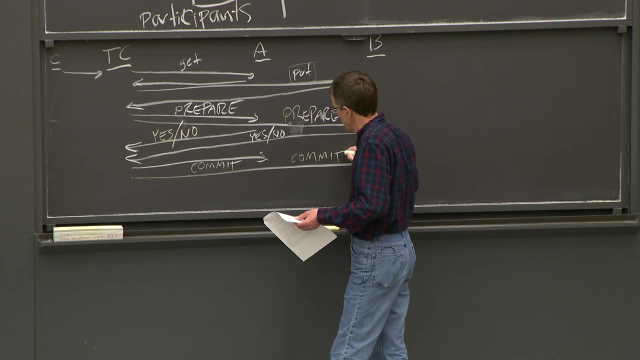 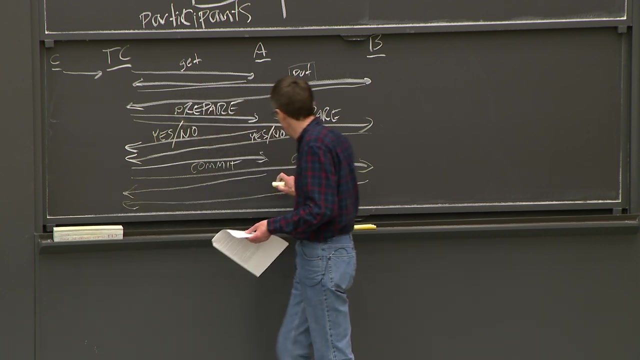 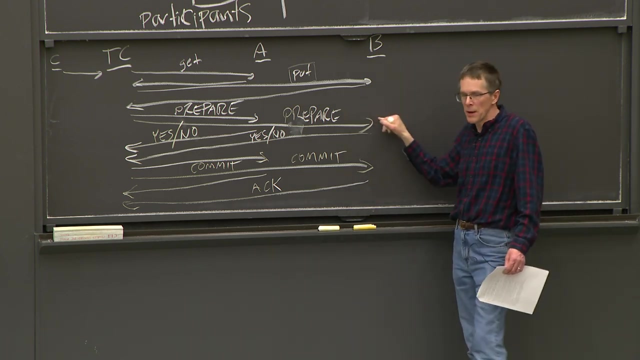 To each of the participants And then the participants usually reply with an acknowledgment saying yes, we now know the outcome, So this is called the acknowledgment. All right, So they all. the transaction coordinator sends out, prepares If all of the participants say yes. 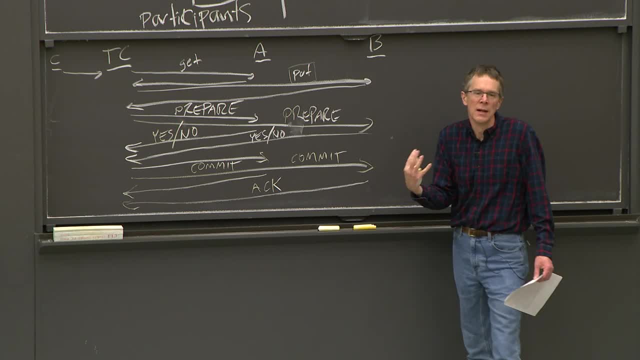 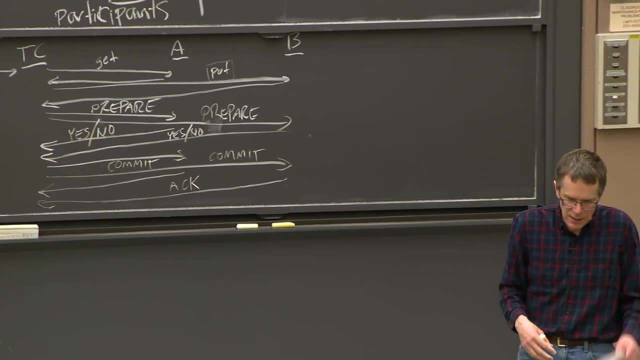 they can commit If any one of them, any of them, even a single one, says no. actually, I cannot complete this transaction because I had a failure or there was an inconsistency like a missing record, and I have to abort If even a single participant says no at this point. 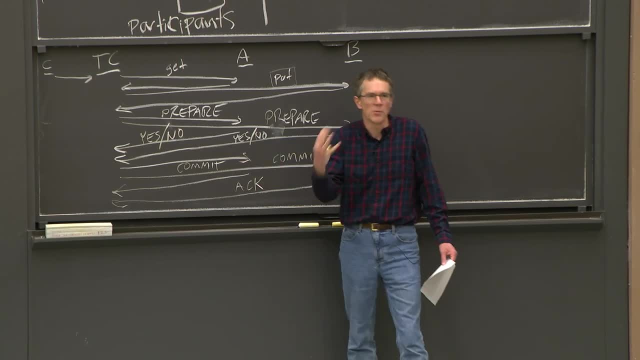 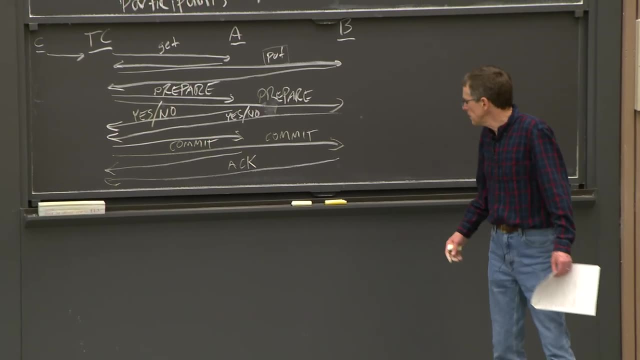 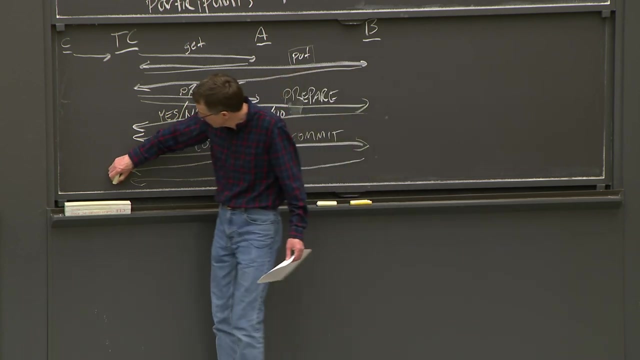 then the transaction coordinator won't commit. It'll send out a round of abort messages saying: oops, please retract this transaction Either way, the after the commit sort of two. two things happen of interest to us. One is the transaction coordinator will emit, whatever the transactions output is. 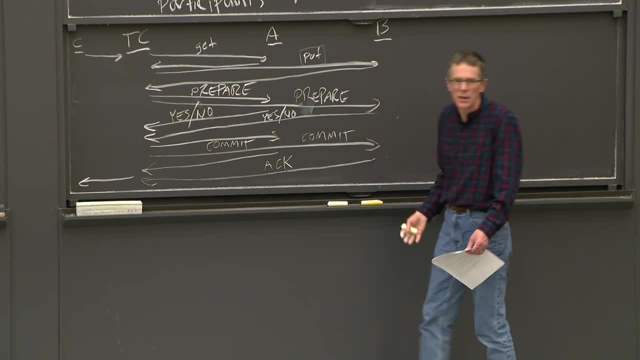 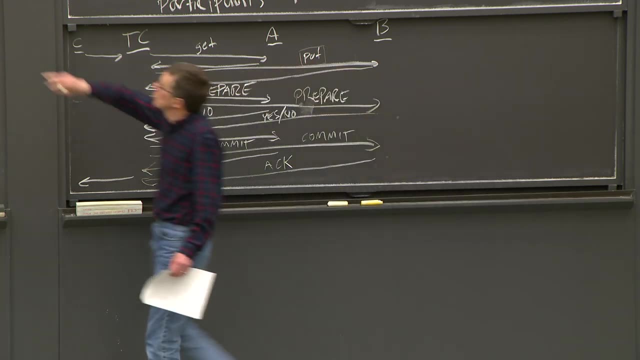 to the client or human that requested it and say: look, oh yes, the transaction's finished. And so now, if it didn't abort, if it committed, it's durable. The other interesting thing is that, in order to obey these locking rules, 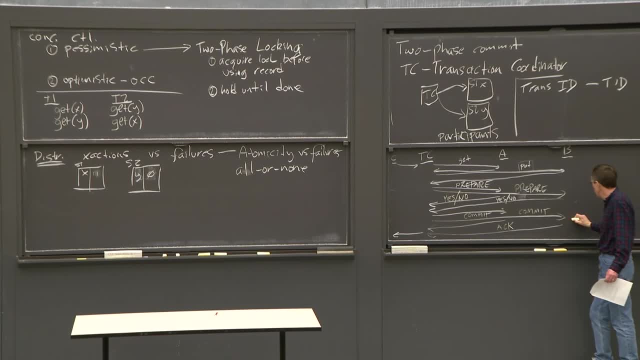 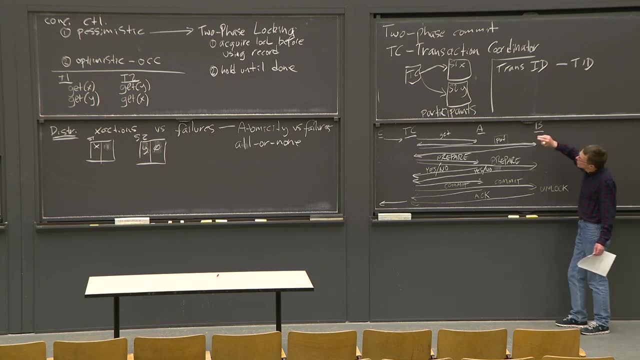 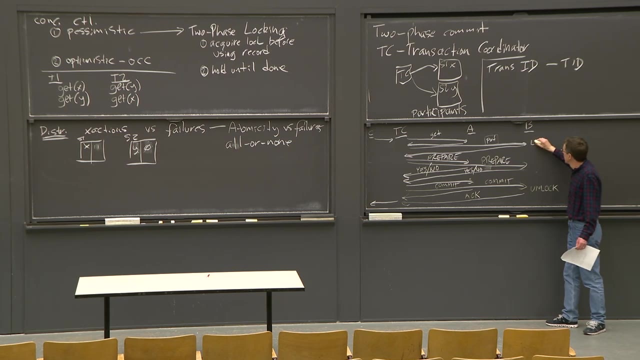 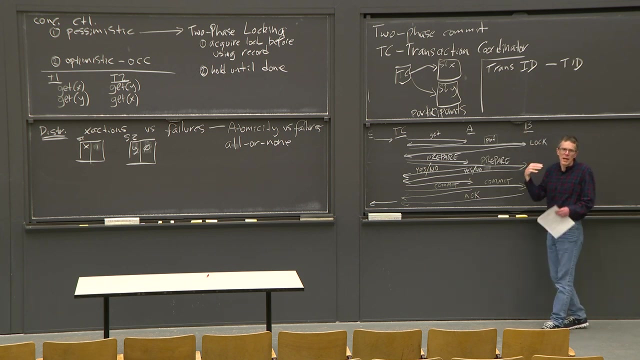 the participants unlock when they see either a commit or an abort And indeed, in order to obey the two phase locking rule, each participant locked any data that it read as part of doing its part of the transaction. So we're imagining that in each participant. 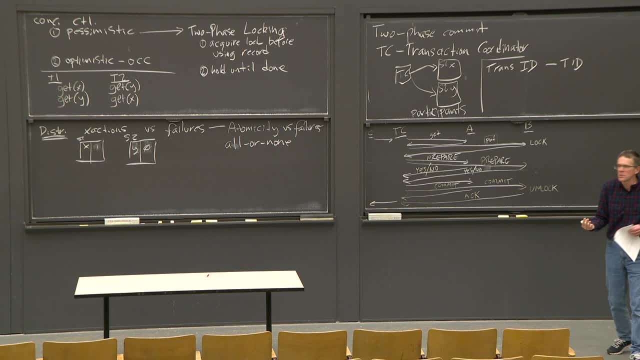 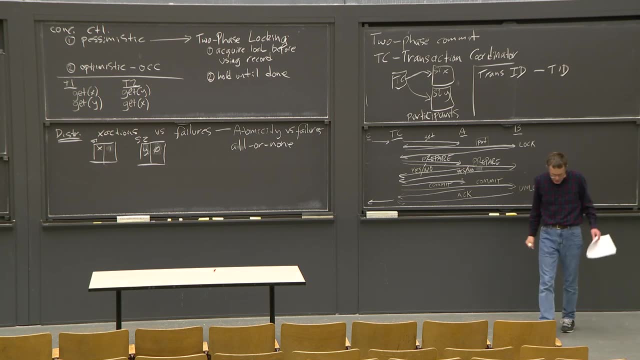 there's a table of the locks associated with the data stored at that participant and the participants sort of lock things in those tables. remember? oh, this is, you know, this piece of data. this record is locked for transaction 29,. 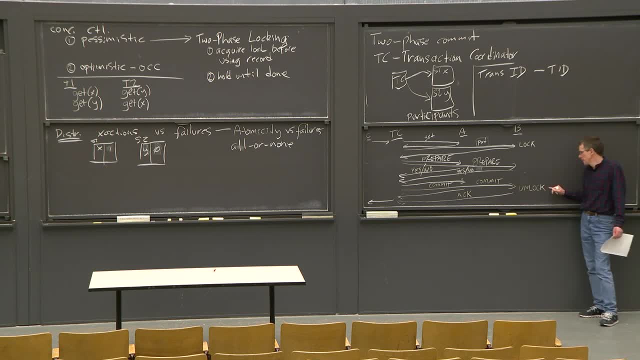 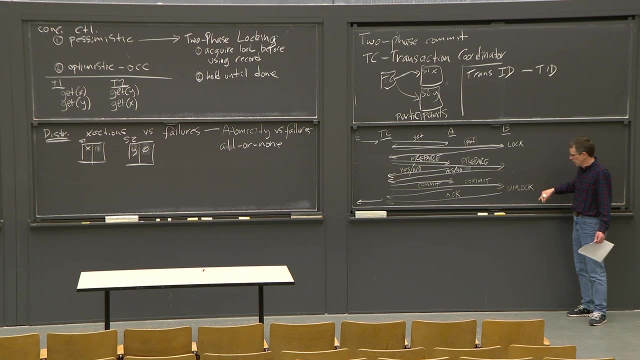 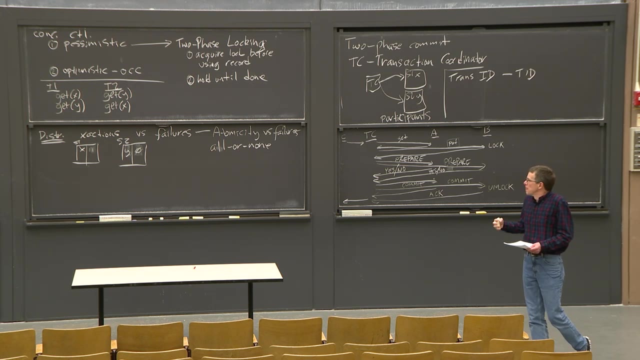 And when, finally, the commit or abort comes back for transaction 29,, the participant unlocks that data and then other transactions can use it. So we may have to wait here and this unlock may unblock other transactions. That's really part of the serializability machinery. 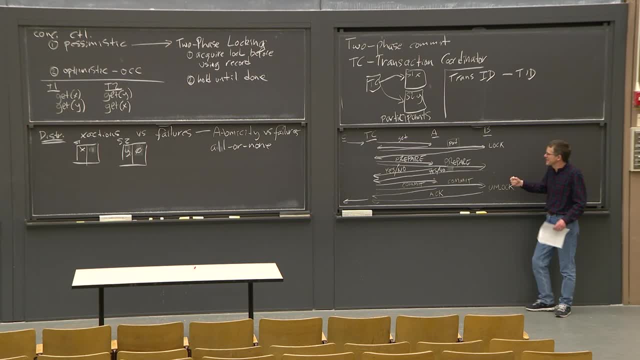 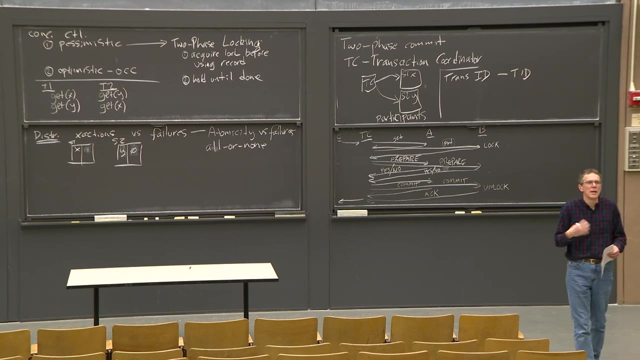 So far. the reason why this is correct basically is that if everybody's following this protocol and there's no failures, then the two participants only commit if both of them commit, and if either of them can't commit, if either of them has to abort, then they both abort. 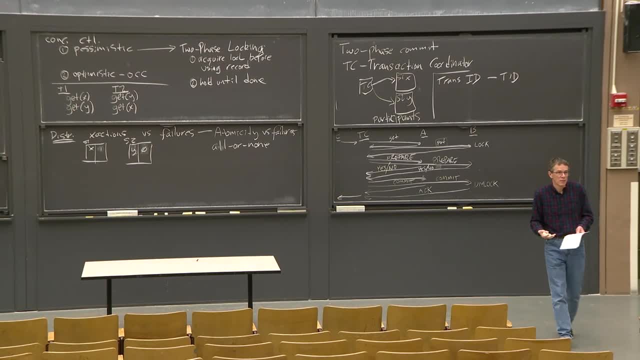 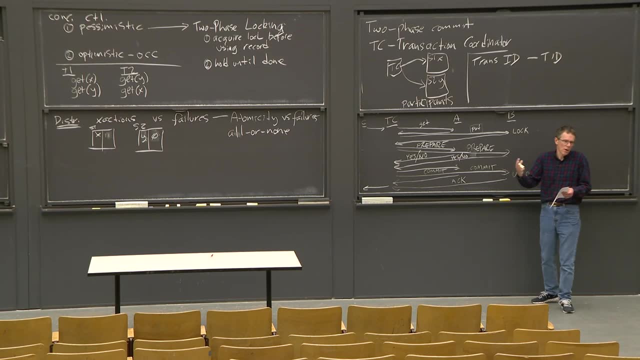 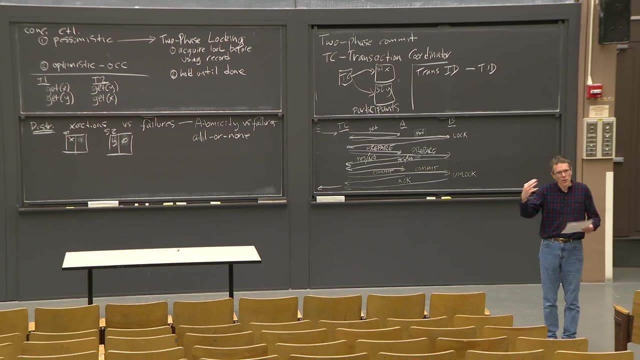 So we get that either they all do it or none of them. do it result that we wanted the atomicity result with this protocol? so far without thinking about failures, And so now our job is to think through in our head all sort of the different kinds of failures. 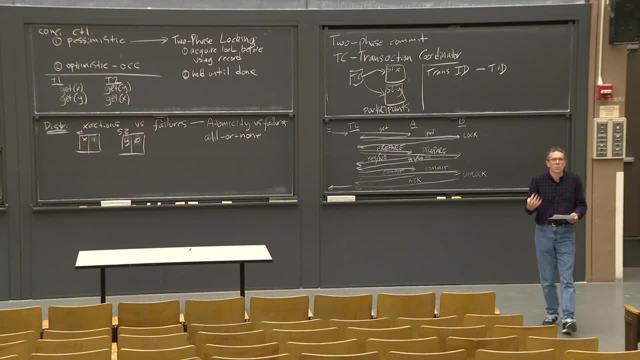 that might occur and figure out whether the protocol still provides atomicity- either both do it or neither do it- in the face of these failures, and how we have to adjust or extend the protocol in order to cause it to do the right thing, 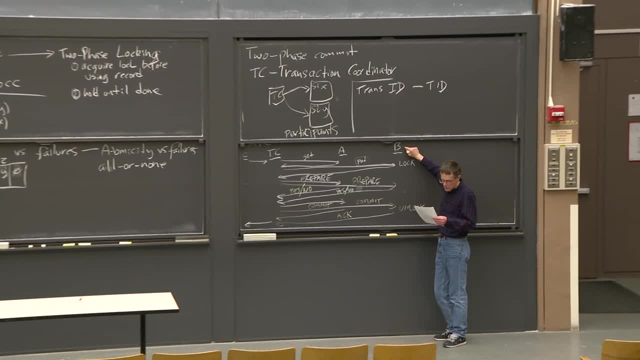 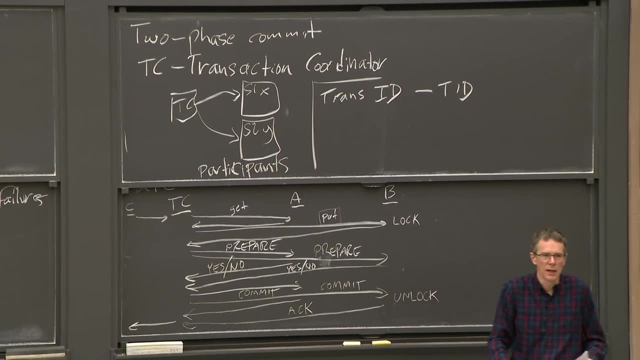 So the first thing I want to consider is what if B crashes and restarts- I mean power failure or something. B just suddenly stops executing and then power is restored and it's brought back. It's brought back to life and runs. maybe some sort of recovery software. 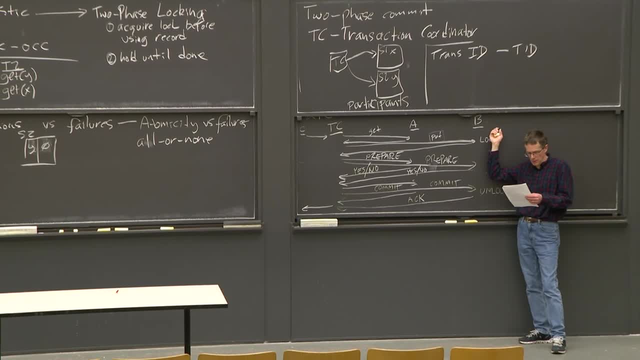 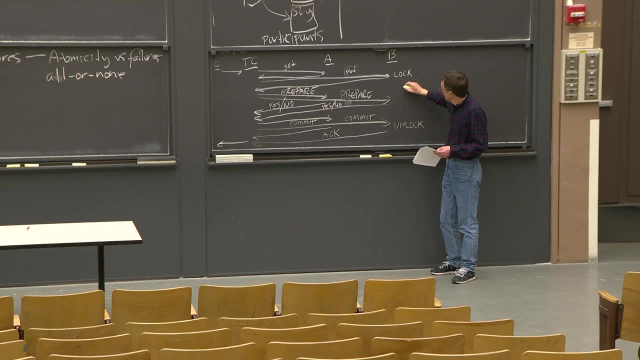 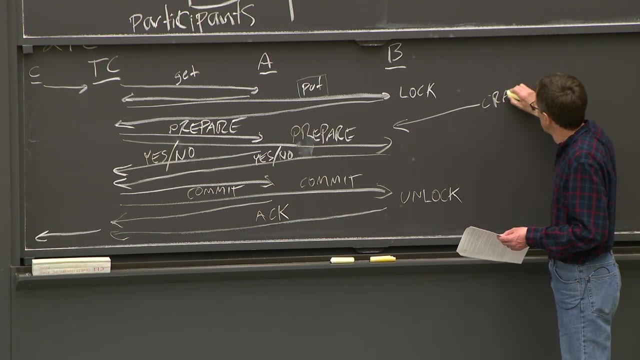 as part of the transaction processing system. Well, there's really two scenarios we have to worry about. One is B might have crashed before sending its yes message back. So if B crashed before sending its yes message back, then it never said yes. 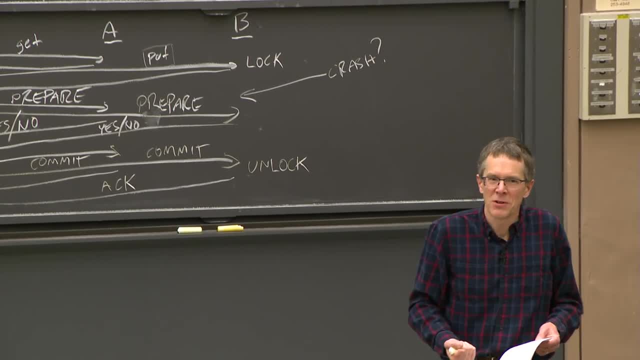 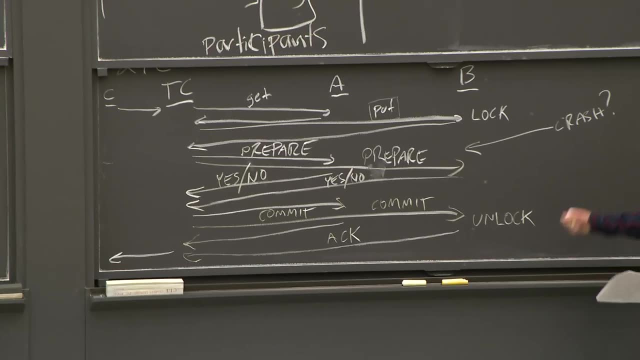 So the transaction coordinator couldn't possibly have committed or be about to commit because it has to wait for a yes from all participants. So if B can convince itself that it could not possibly have sent a yes back, that is it crashed before sending the yes. 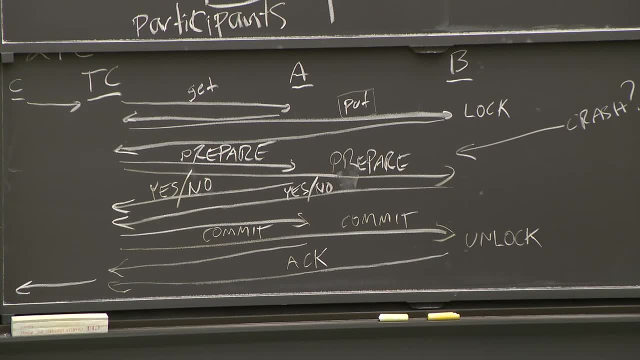 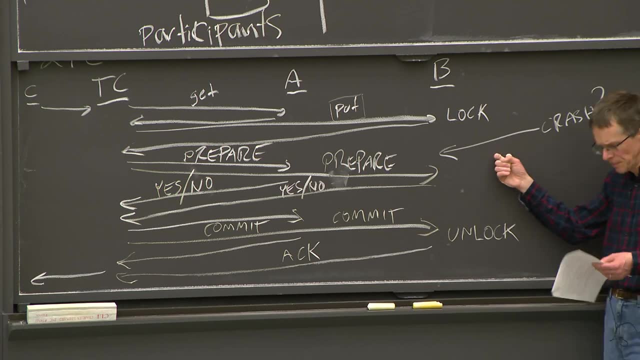 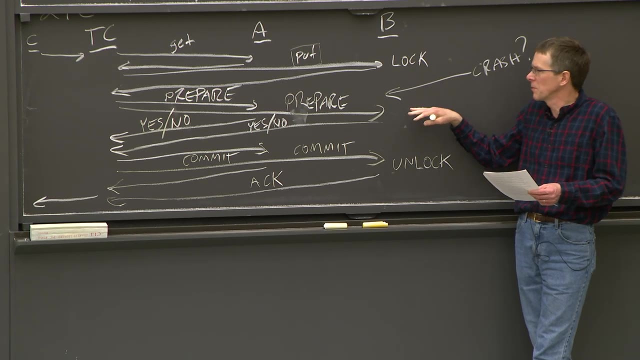 then B is entitled to unilaterally abort the transaction itself and forget about it because it knows the transaction coordinator can't possibly commit it. So there's a number of ways of implementing this. One possibility is that all of B's information about transactions 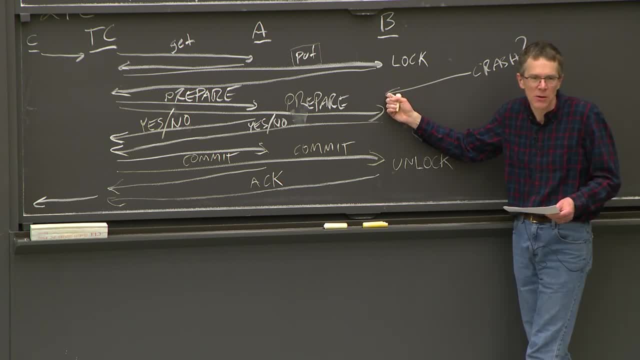 that haven't reached this point is in memory and is simply lost if B crashes and reboots, So B just won't know anything about transactions that haven't sent yes back yet. And then if the transaction coordinator sends a prepare message to a participant that doesn't know anything about the transaction. 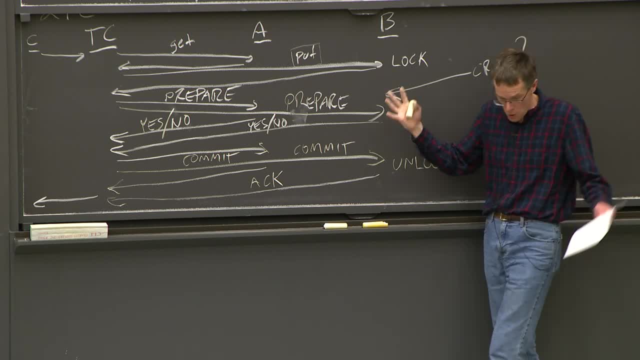 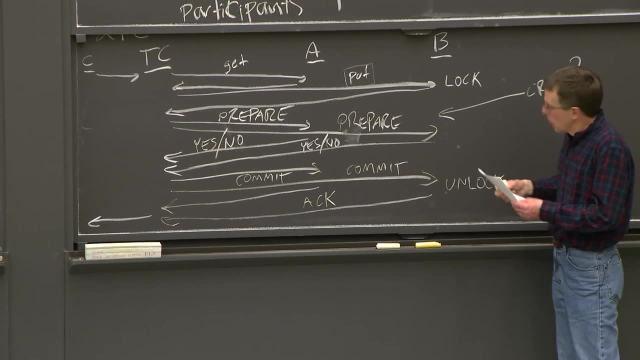 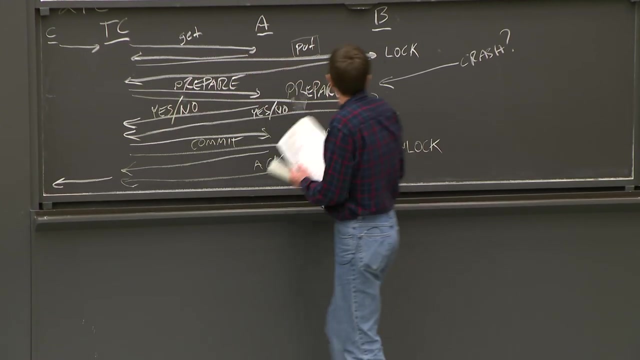 because it crashed before sending yes. then the participant will say no, no, I cannot possibly agree to that. You know, please abort. Okay, but of course maybe B crashed after sending a yes back, So that's a little more tricky. 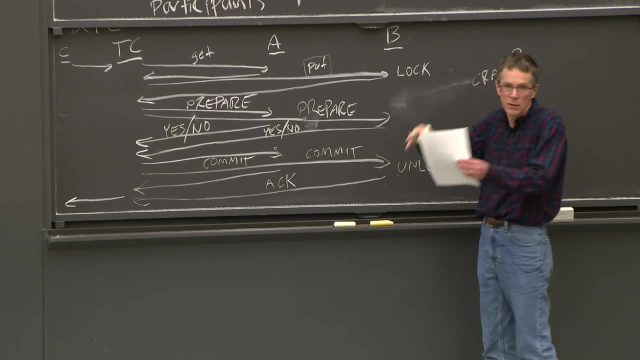 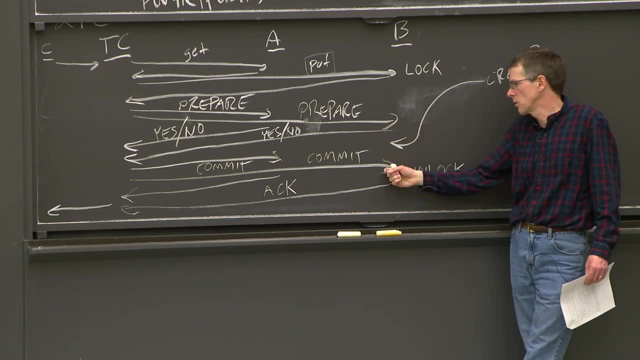 Supposing the crash. supposing that B gets a prepare, it's happy, it says yes, I'm gonna commit, and then it crashes before it gets the commit message from the transaction coordinator- Coordinator. Now we're in a totally different situation. 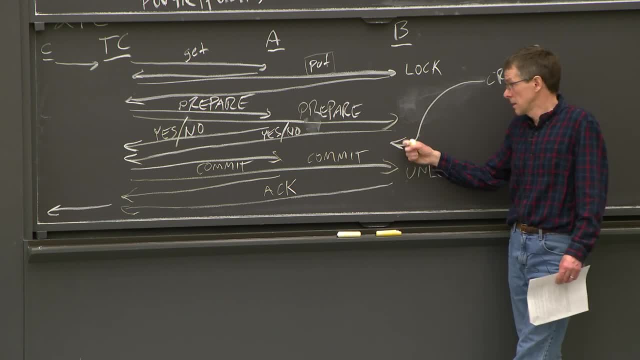 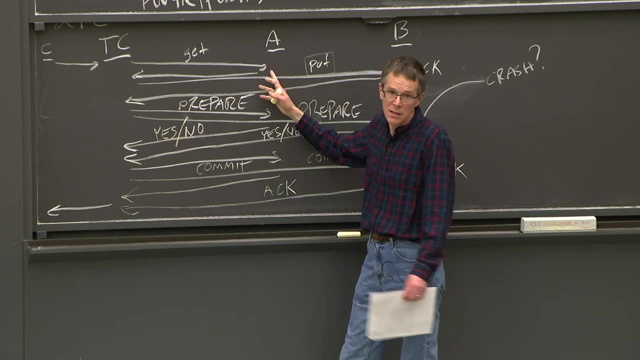 B has promised to commit if told to do so, because it sent a yes back and for all it knows, and indeed the most likely thing that's happening is, the transaction coordinator got yeses from A and B and has sent a commit message to A. 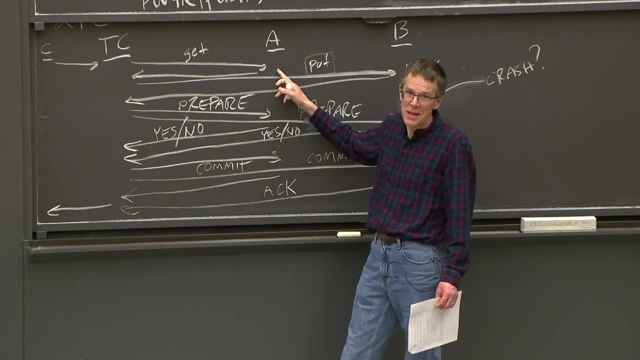 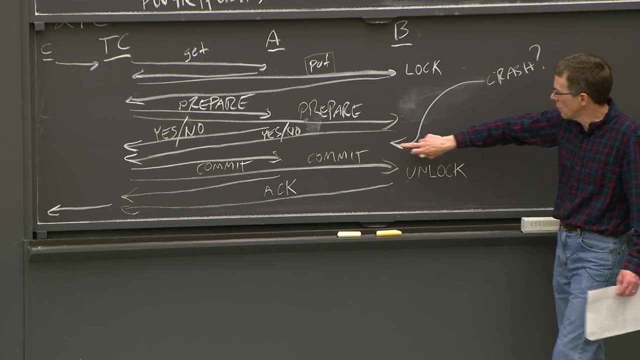 so that A actually will do its part of the transaction and make it permanent and release locks. And in that case, in order to honor all or nothing, we're absolutely required, if B should crash at this point, that on recovery, that it be still prepared. 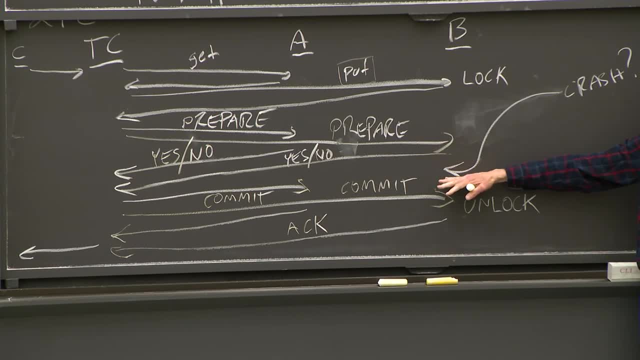 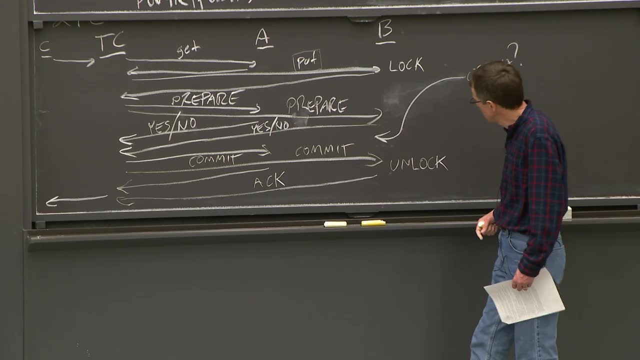 to complete its part of the transaction. It doesn't actually know at that point whether, because it hasn't received the commit yet, whether it should commit or not, but it must still be prepared to commit And what that means. the fact that B can't lose the state. 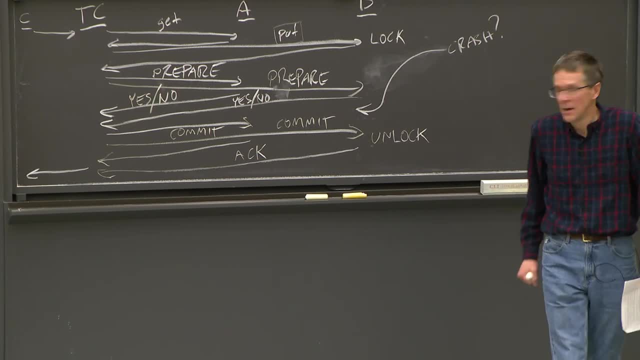 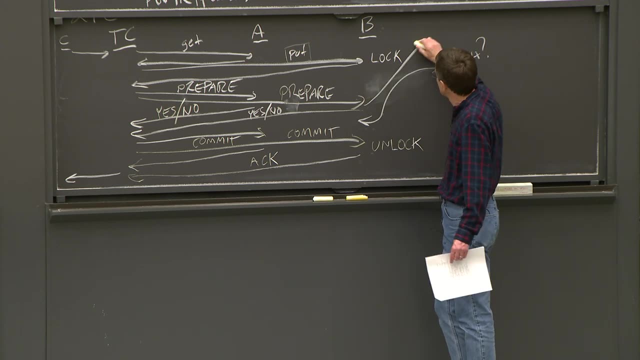 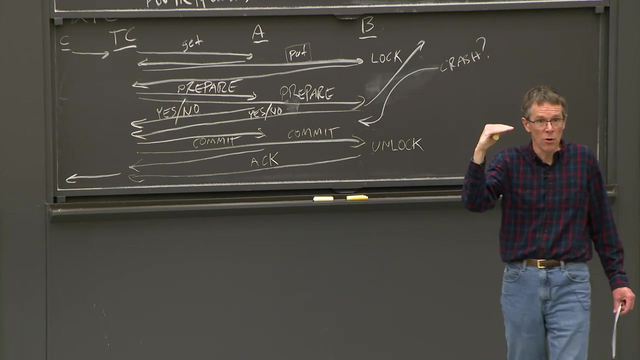 for a transaction across crashes and reboots is that before B replies to a prepare, it must make the transaction state the sort of intermediate transaction state, the memory of all the changes it's made which may have to be undone if there's an abort. 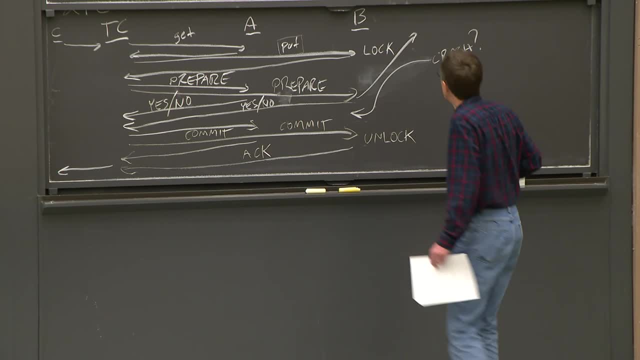 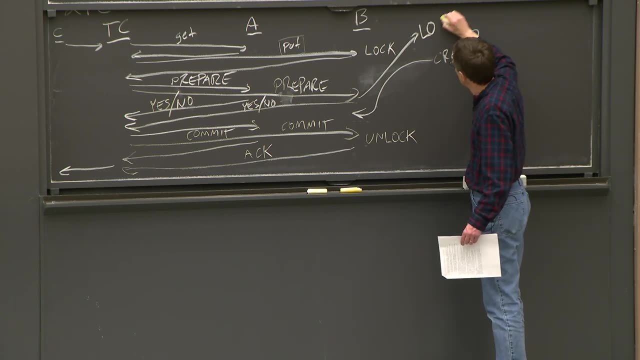 plus the record of all the locks the transaction's held. It must make that durable on disk. in particular, it's almost always in a log on disk. So before B replies yes. before B sends the yes in reply to a prepare message: 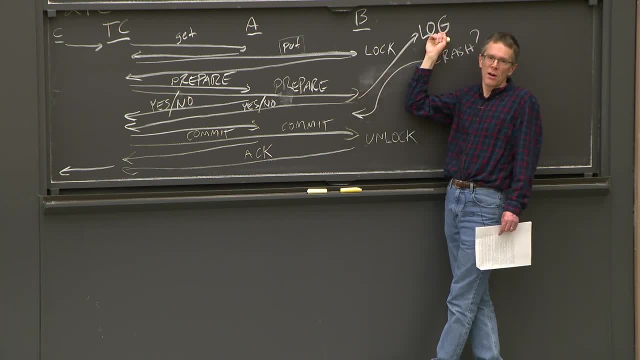 it first must write to disk in its log all the information required to commit that transaction, That is, all the new values produced by put, plus a full list of locks on the disk or some other persistent memory, before replying with yes. And then, if B should crash after sending the yes, 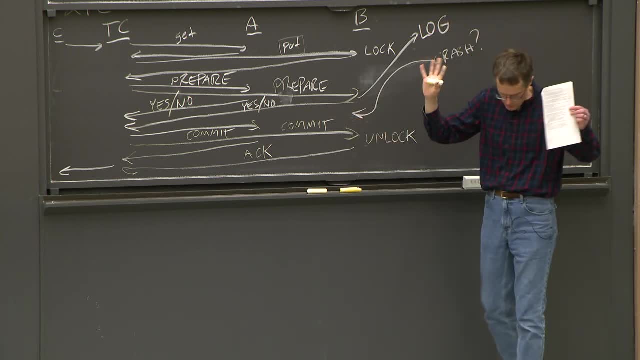 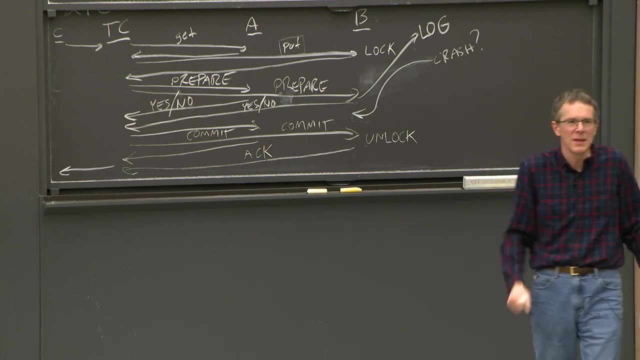 as part of recovery. when it restarts, it'll look at its log and say: oh gosh, I was in the middle of a transaction. I had replied yes for transaction 92. I mean, here's all the modifications it should make if committed, and all the locks it held. 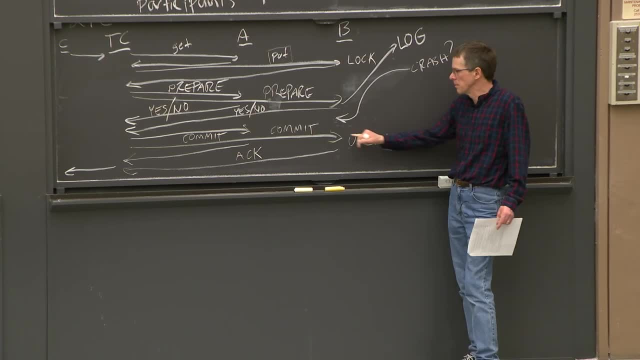 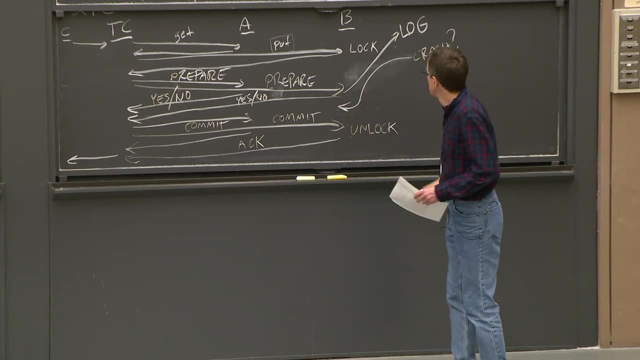 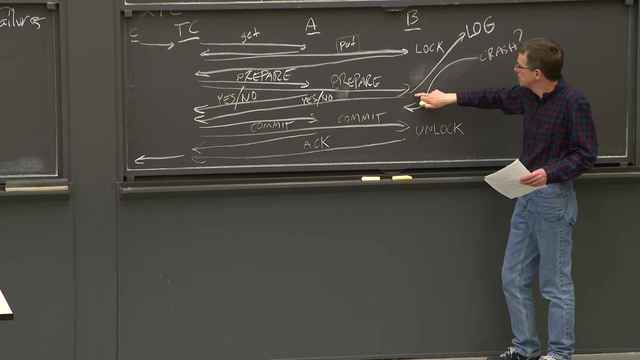 I better restore that state And then when B finally gets a commit and an abort, it'll know from having read its log how to actually finish this part of the transaction. So this is an important thing I left out of the original laying out of this protocol. 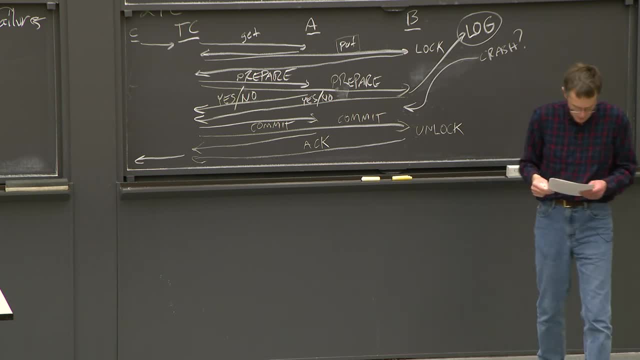 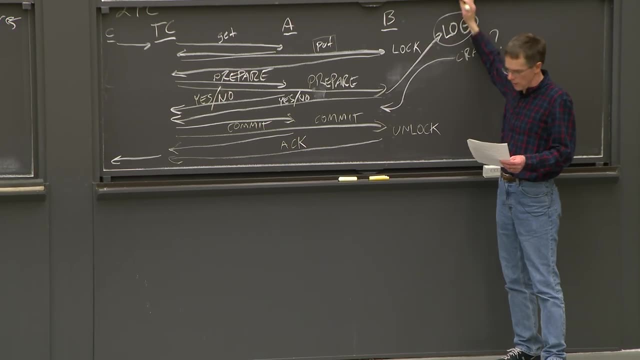 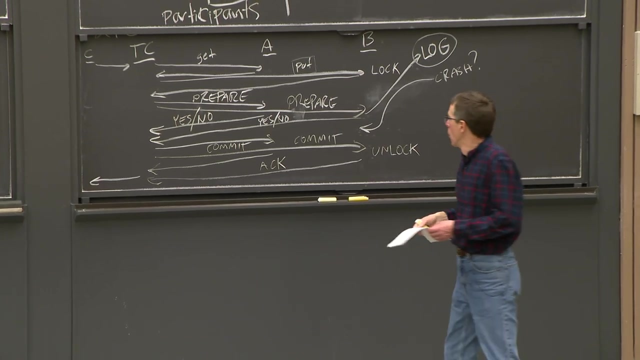 is that B must write to its disk at this point- And this is part of what makes two-phase commit a little bit slow- is that there's the necessary persisting of information here. Okay, so we also have to worry about, okay, and the final place, I guess. 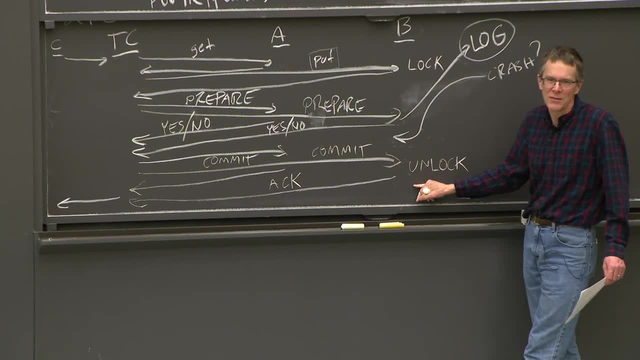 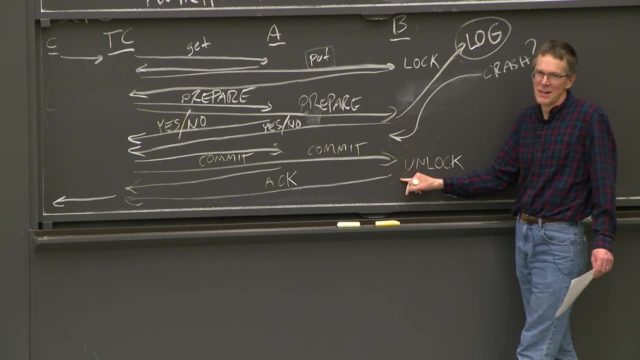 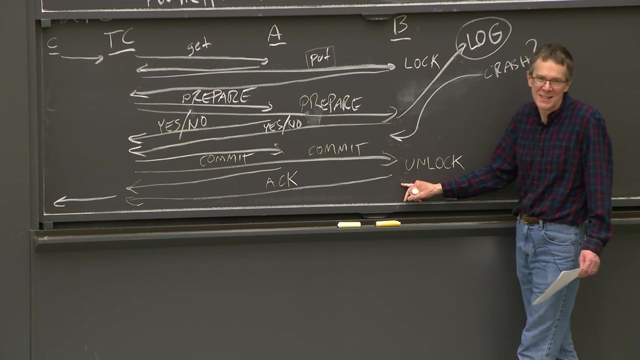 where you might crash is: you might crash B might crash after receiving the commit or after- well, you might crash after actually processing the commit, But in that case it's made the modifications that the transaction needed to make permanent in its database, presumably also on disk, before. 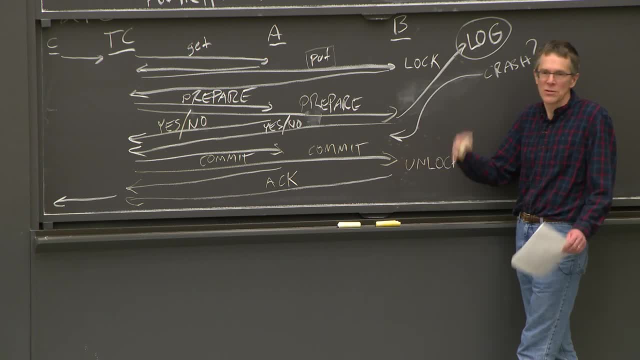 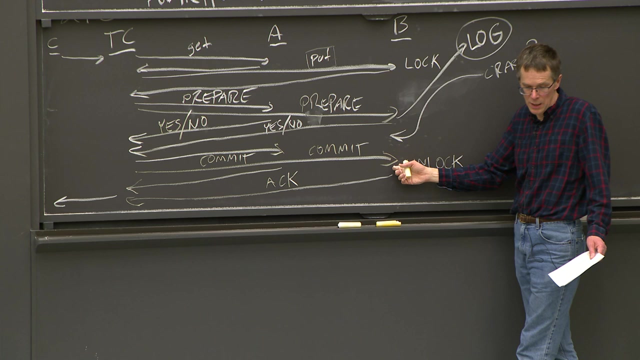 or after it received the commit message, And in that case there's maybe not anything to do if it restarts because the transaction's finished. So when B receives the commit message it probably writes the copies, the modifications from its log onto its permanent storage. 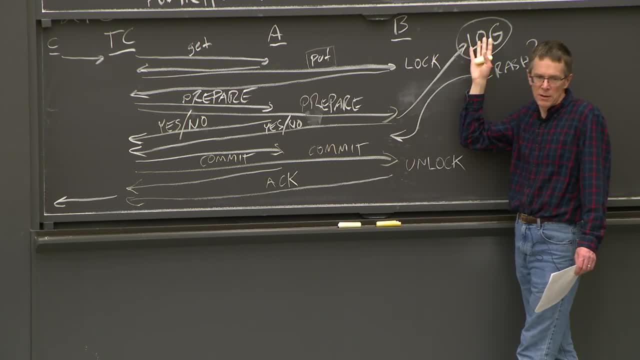 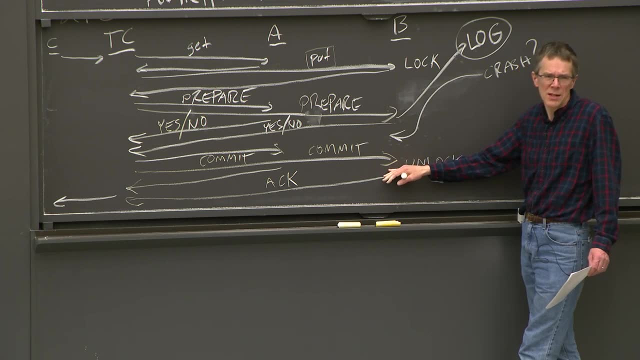 releases its locks, erases the information about the transaction from its log and then replies. And of course, we have to worry about you know what if it receives a commit message twice. Probably the right thing to do is either for B 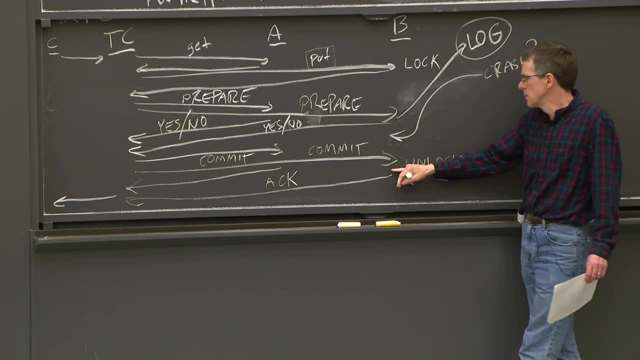 to remember about the transaction that takes memory. so it turns out that if B simply forgets about committed transactions that it's made durable on disk, it can reply to a repeated commit message if it doesn't know anything about that transaction by simply acknowledging it again. 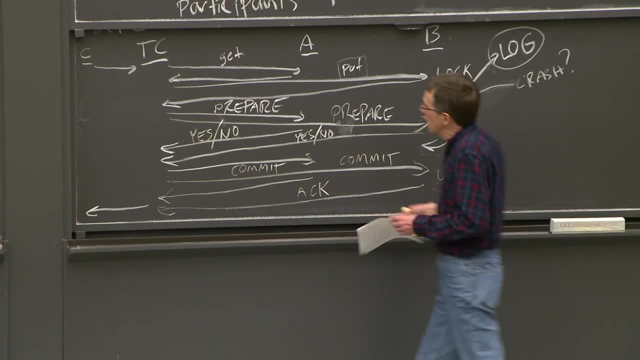 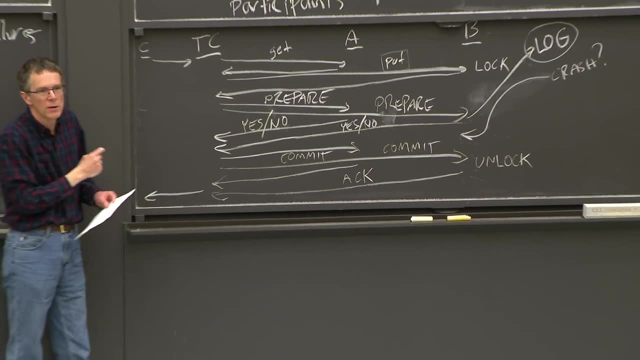 And that'll be important a little bit later on. Okay, so that's the story of one of the participants crashes at various awkward points. What about the transaction coordinator? It's also just a single computer, So you know, if it fails might be a problem. 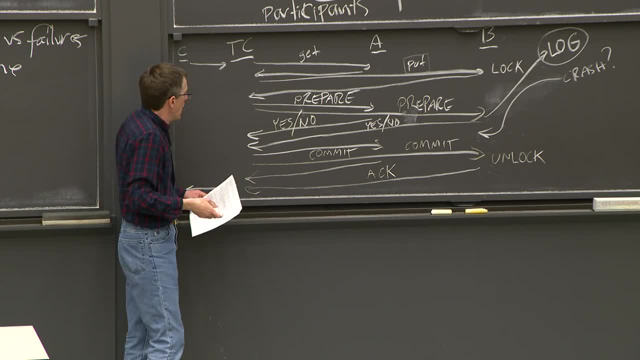 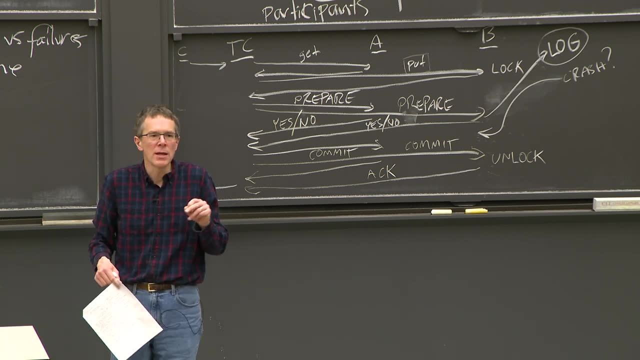 Okay, so again the critical- where things start getting critical- is if any party might have committed, then we cannot forget about that, If any either of these participants might have committed, or if the transaction coordinator might have replied to the client. 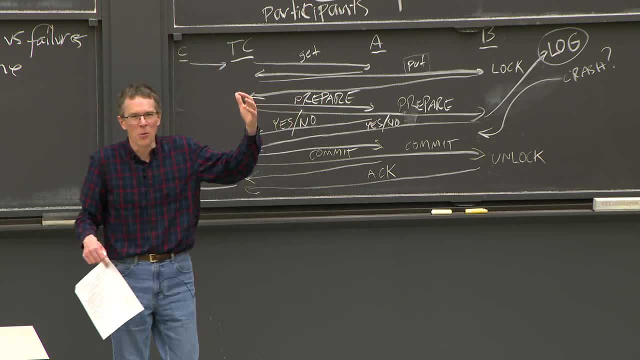 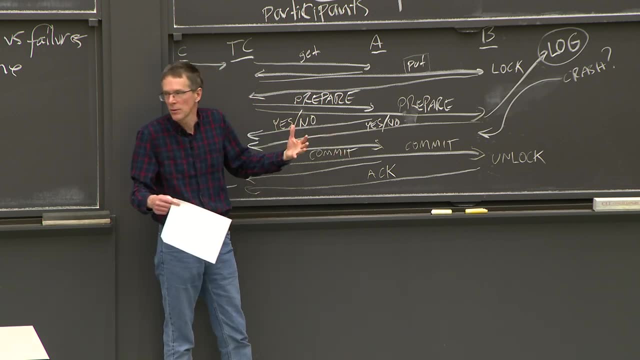 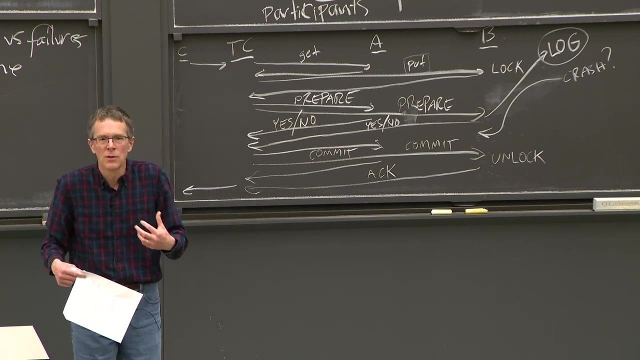 then we cannot have that transaction go away. Right, if A is committed, but maybe the transaction coordinator sent out a commit message to A but hadn't gotten around to sending a commit message to B. if it crashes at that point, the transaction coordinator must be prepared on restart. 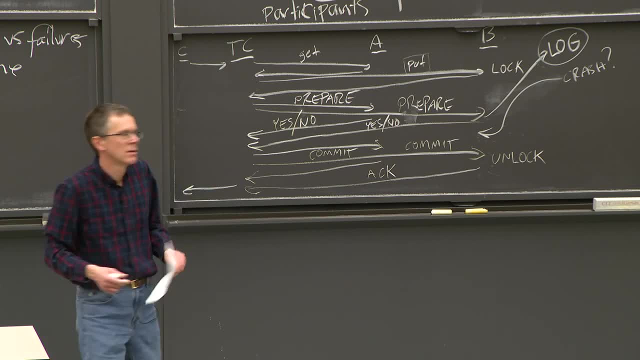 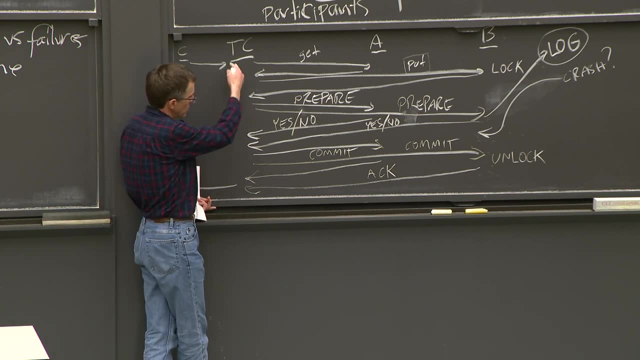 to resend the commit messages to make sure that both parties know that the transaction is committed. So okay, so you know. whether that matters depends on where the transaction coordinator crashes. If it crashes before sending commit messages, it doesn't really matter. 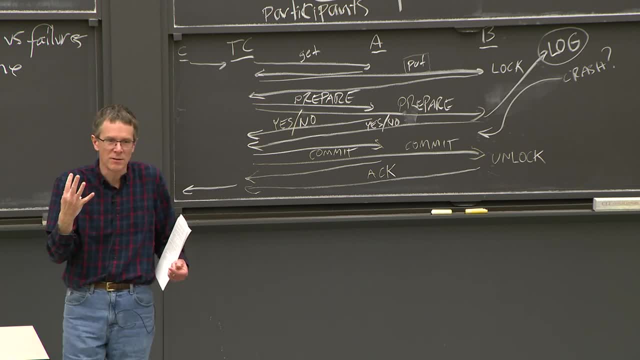 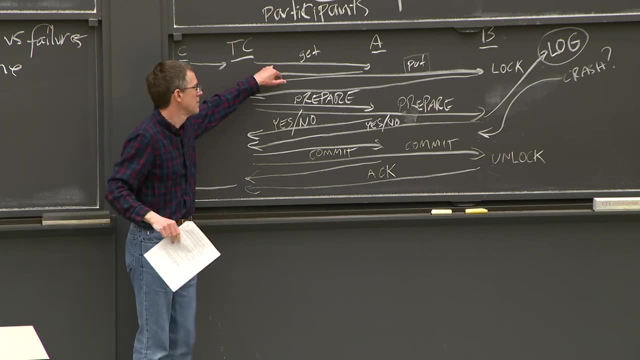 Neither party. if you know, since the transaction coordinator didn't send commit messages before crashing, it can just abort the transaction. And if either participant asks about that transaction because they, you know, see it's in their log but they never got a commit message, 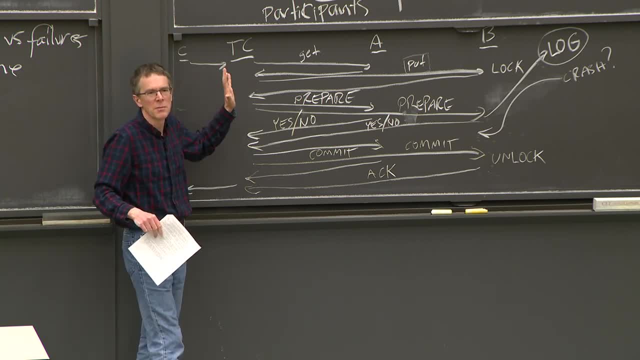 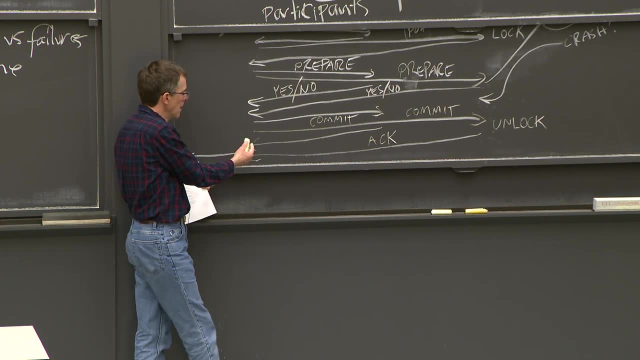 the transaction coordinator can say: I don't know anything about that transaction. It must have been aborted, possibly due to a crash. So that's what happens if the transaction coordinator crashes before the commit, But if it crashes after sending one or more commit message, 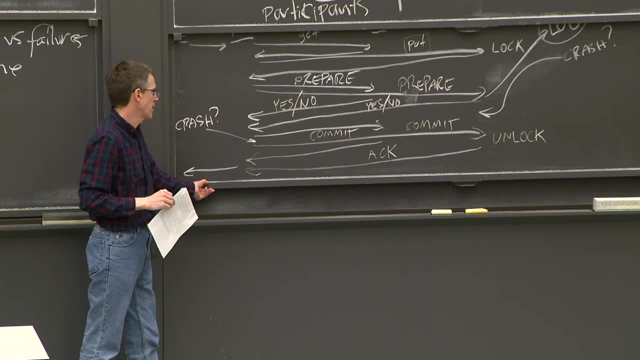 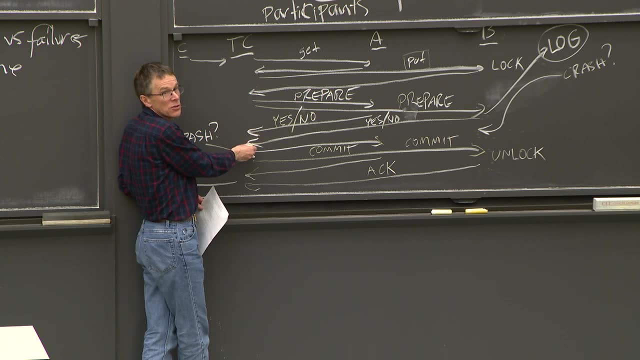 then it cannot. the transaction coordinator can't be allowed to forget about the transaction, And what that means is that, at this point, when the after the transaction coordinator has made its commit versus abort decision on the basis of these yes, no votes. 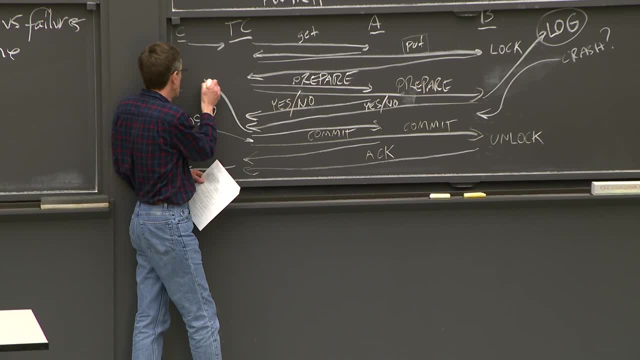 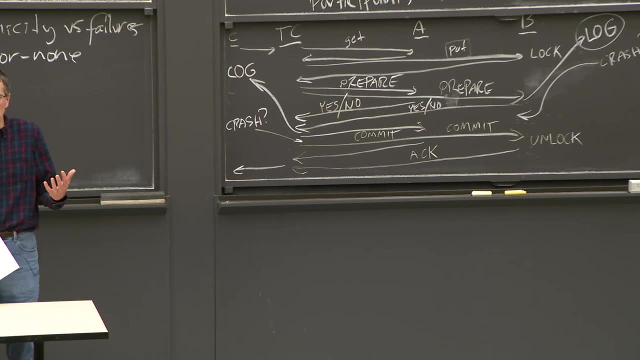 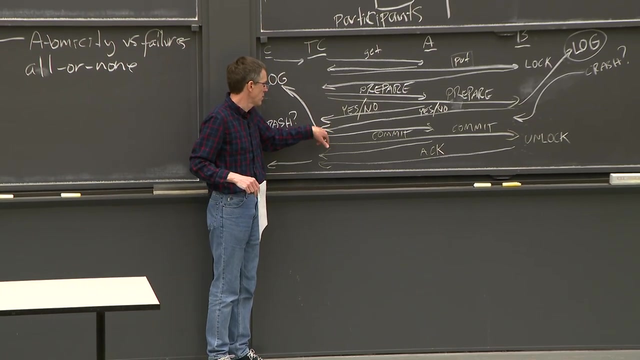 before sending out any commit messages it must first write information about the transaction to its log in persistent storage like a disk that'll still be there if it crashes and restarts. So, transaction coordinator, after it receives a full set of yeses or nos. 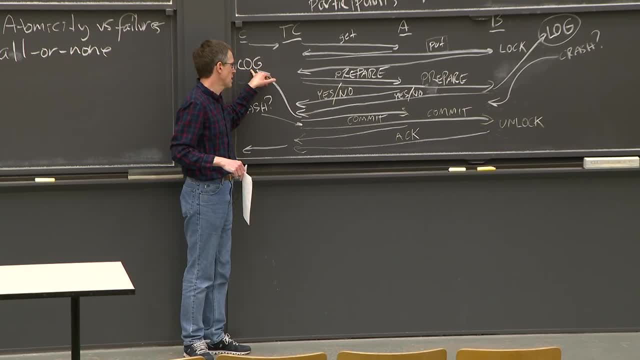 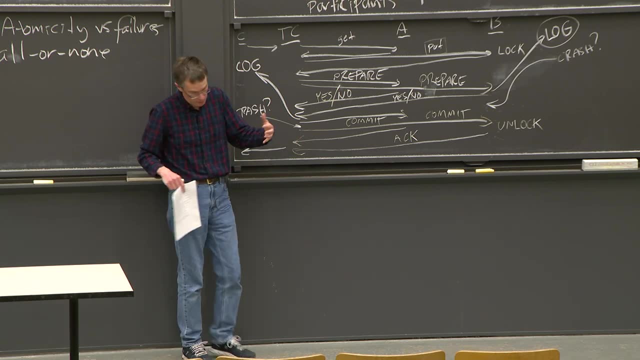 writes the outcome and the transaction ID to its log on disk and only then starts to send out commit messages. And that way, if it crashes at any point, maybe before it sent the first commit message, or after it sent one, or maybe even after it sent all of them, 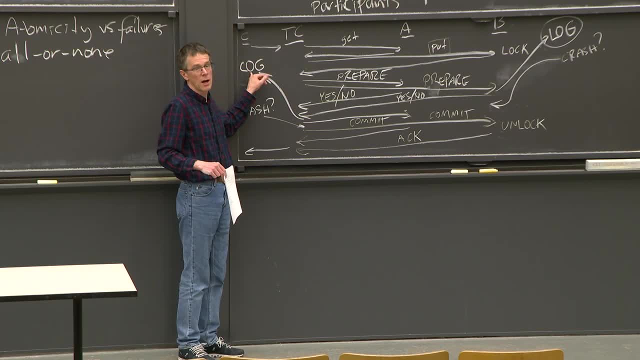 if it crashes at that point, its recovery software will see in the log: aha, it was in the middle of a transaction. the transaction was either known to have been committed or aborted and, as part of recovery, it will resend commit messages to all of the participants. 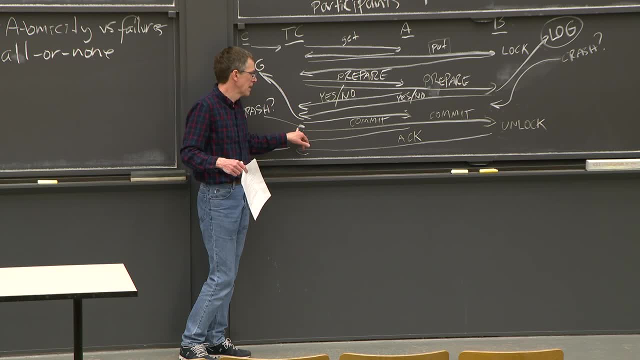 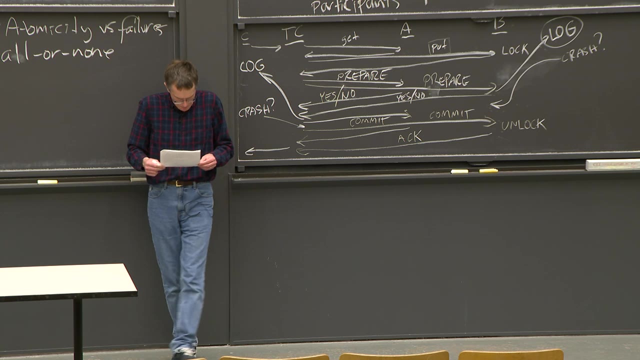 or abort messages, whatever the decision was, in case it hadn't sent them before it crashed, And that's one reason why the participants have to be prepared to receive duplicated commit messages. Okay, So those are the main crash stories. We also have to worry about what happens. 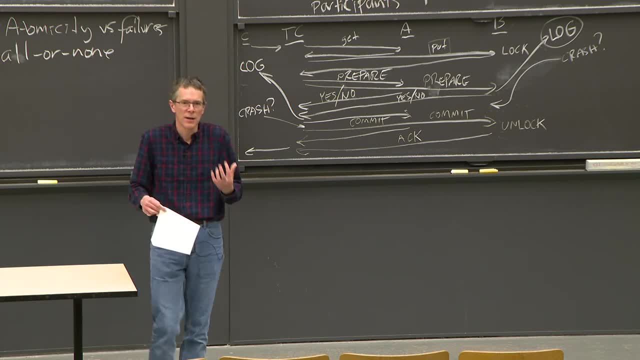 if messages are lost in the network, We might send a message. maybe the message never got there and we might send a message and be waiting for it to crash. you might send a message and be waiting for it to crash. You might send a message and be waiting for it to crash. 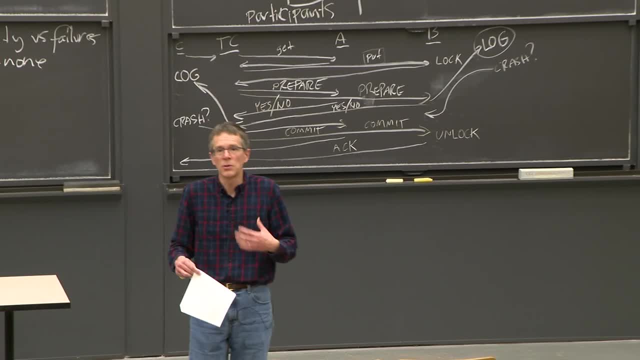 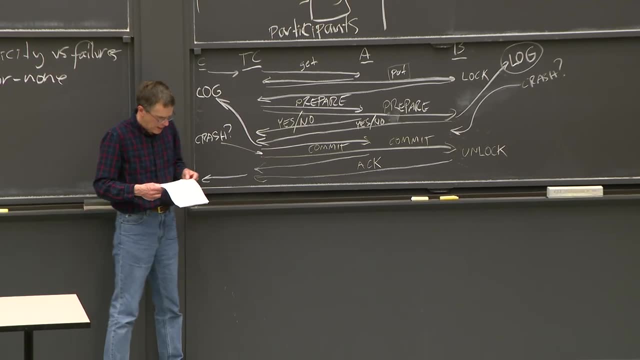 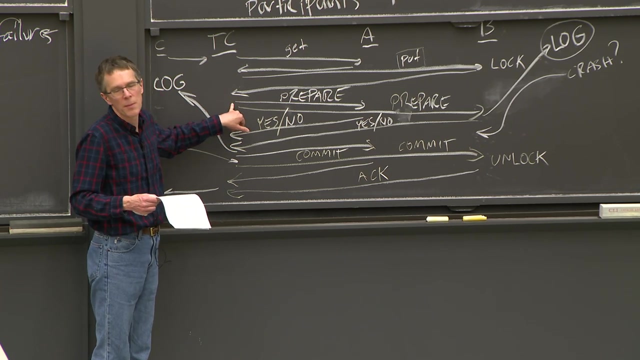 for a reply. Maybe the reply was sent, but the reply was dropped. So any one of these messages may be dropped and you need to think through what to actually do in each of these cases. So, for example, supposing the transaction coordinator sent out, prepare messages, but 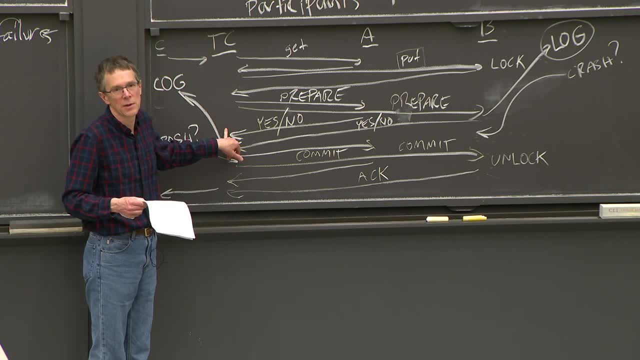 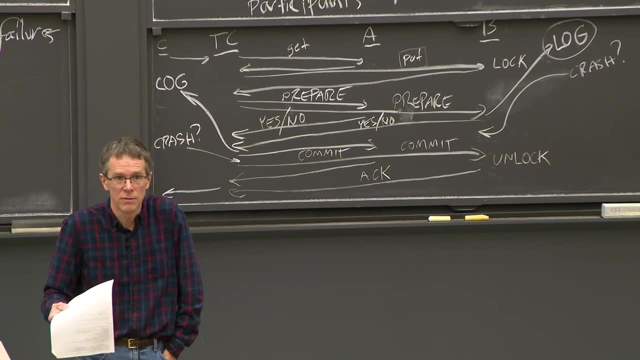 hasn't gotten some of the yes or no replies from participants. What are the transaction coordinator's options at that point? Well, one thing it could do is send out a new set of prepare messages saying: you know, I didn't get your answer. Please tell me your answer. 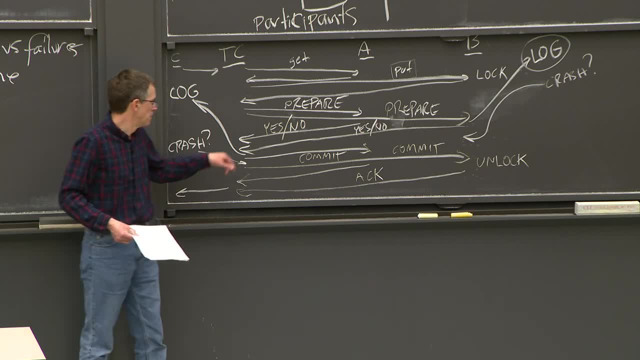 yes or no, And you know it could keep on doing that for a while. But if one of the participants is down for a long time, we don't want to sit there waiting with locks held right, Because you know supposing A is unresponsive but B is up, but because we haven't committed. 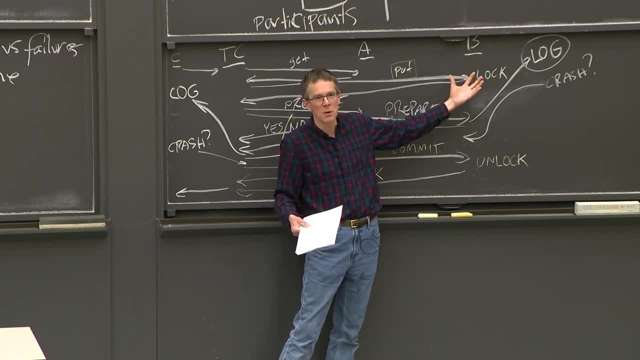 or aborted B is still holding locks and that may cause other transactions to be waiting. So we don't want to wait forever if we can possibly avoid it. So if the transaction coordinator is down for a long time, we don't want to sit there waiting with locks held. So if the 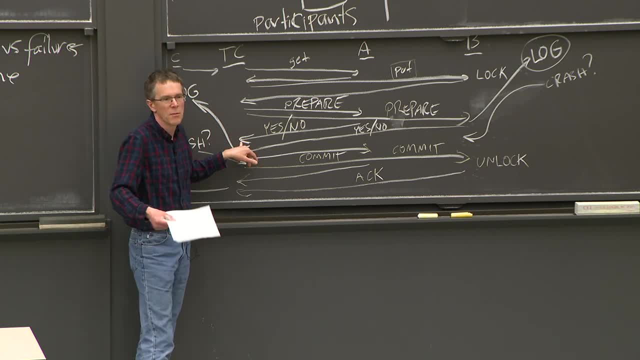 transaction coordinator hasn't gotten yes or no responses after some amount of time from the participants, then it can simply unilaterally decide: oh, we're going to abort this transaction Because it knows, since it didn't get a full set of yes or no messages. 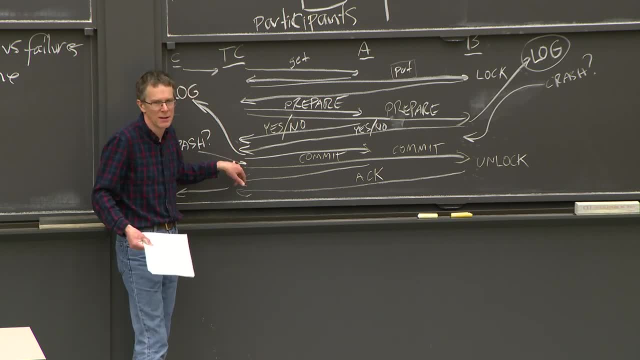 of course it can't possibly have sent a commit yet, So no participant could have committed. So it's always valid to abort if the transaction coordinator hasn't yet committed. So the transaction coordinator times out waiting for yeses or nos, because messages were lost. 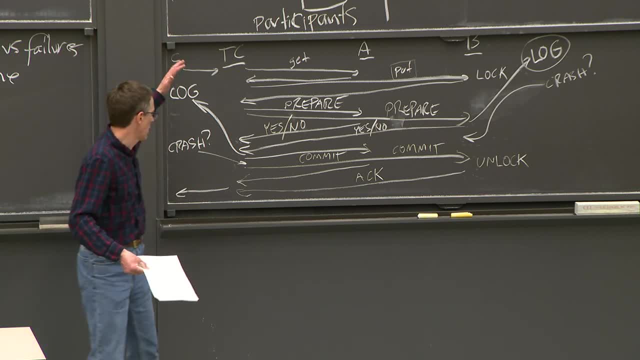 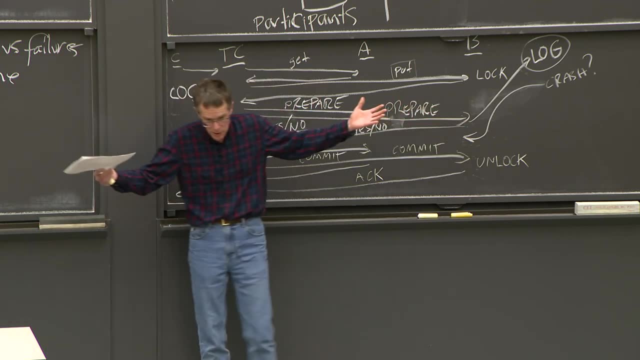 or somebody crashed or something, it can just decide. all right, we're aborting this transaction. we'll send out a round of abort messages And if some participant comes back to life and says: oh you know, I didn't hear back from you about transaction 95, the transaction coordinator will. 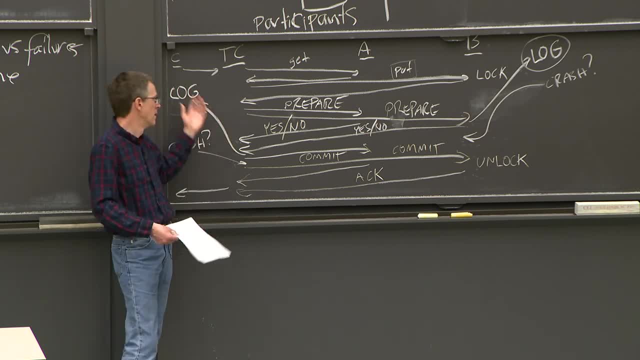 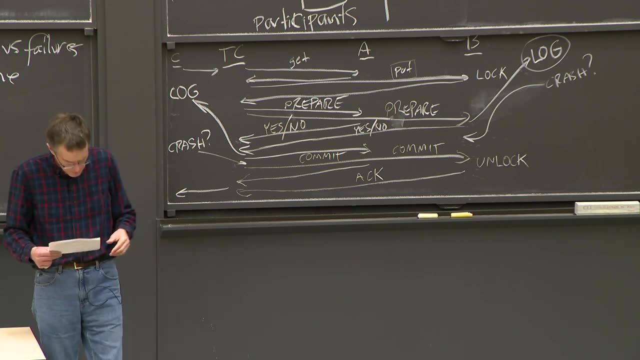 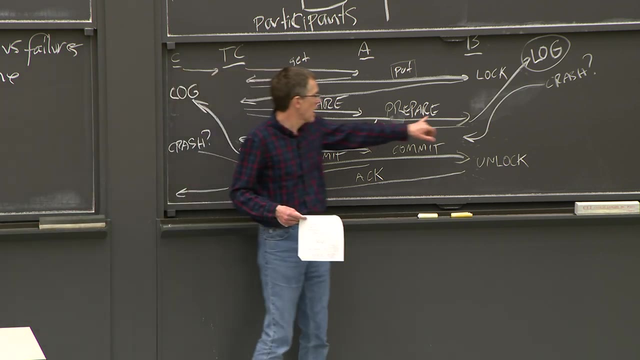 say: oh well, I don't know anything about transaction 95, you know because it aborted it and erased its state for that transaction And it'll tell the participant. you know you should abort this transaction too. Similarly, if one of the participants times out waiting for the prepare here, 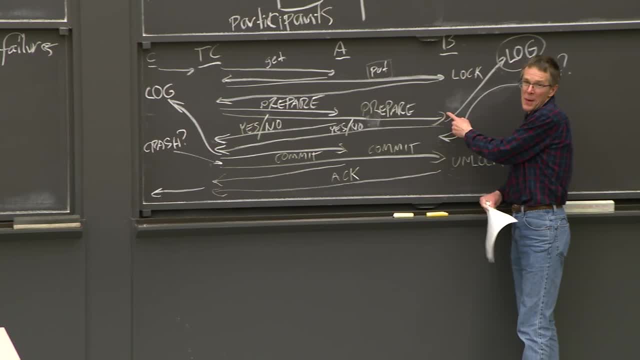 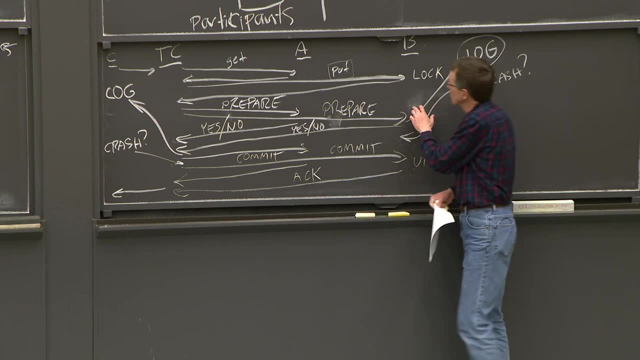 then you know, if a participant hasn't received a prepare, that means it hasn't sent a yes message back And that means the coordinator can't possibly have sent any commit messages. So if a participant times out here waiting for the prepare, it's also always allowed to just 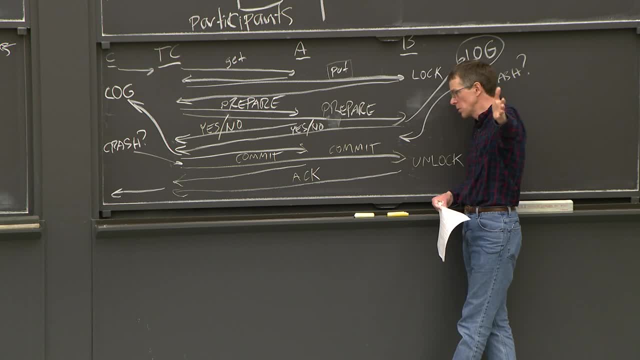 bail out and decide to abort the transaction. And if it's some future time, the transaction coordinator comes back to life and sends out prepare messages, then B will say no, I don't know anything about that transaction, so I'm voting. 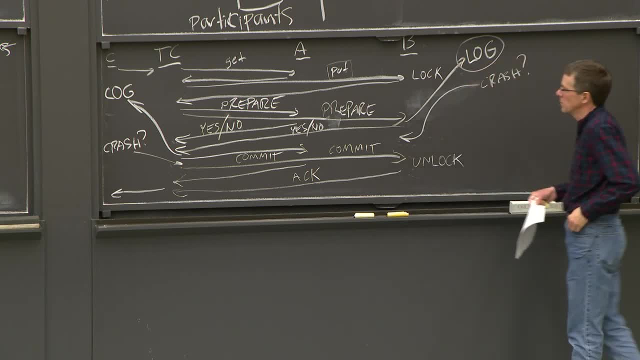 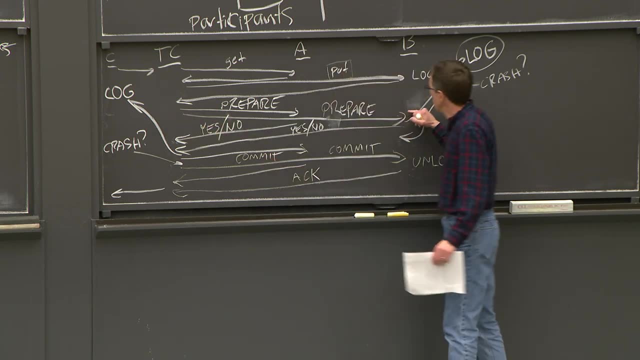 no, And that's okay, because it can't possibly have started to commit anywhere. So again, if something goes wrong with the network or the transaction coordinator is down for a while and the participants are still waiting for prepares, it's always valid for participants. 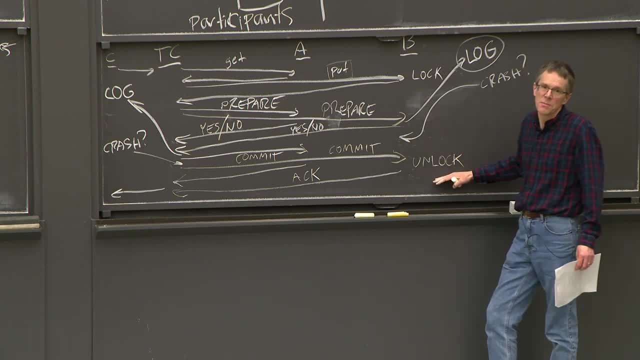 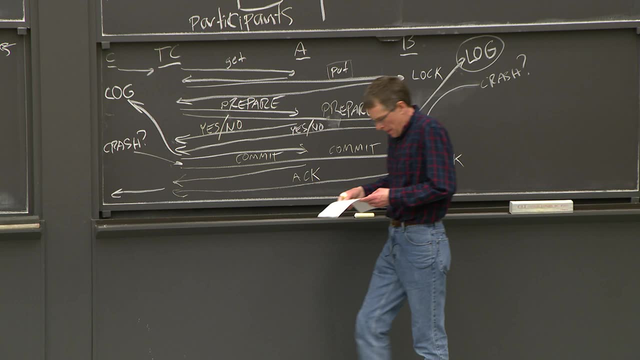 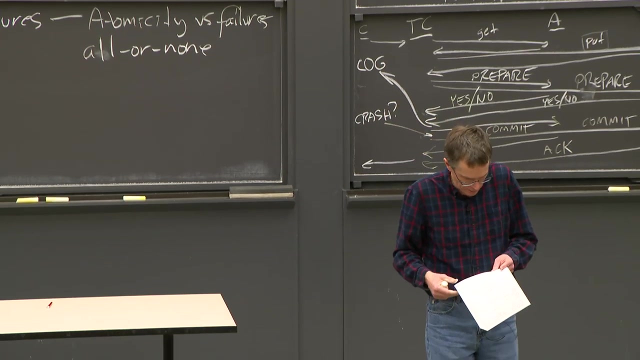 to abort and thereby release the locks that other transactions may be waiting for, And that can be very important in a busy system. So that's the good news about if the participants or the transaction coordinators time out waiting for messages from the other parties. 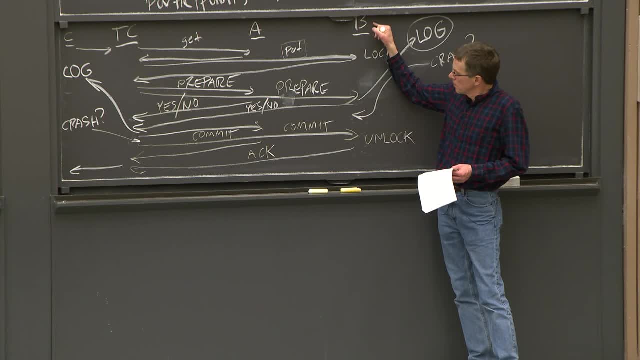 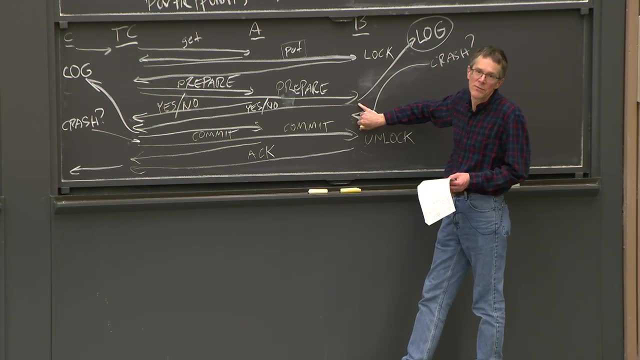 However, suppose participant B has received a prepare and sent its yes, and so it's somewhere around here, but it hasn't received the commit and it's waiting and waiting and it hasn't gotten it. So B is waiting to commit back. Maybe something's wrong with the network, maybe the transaction. 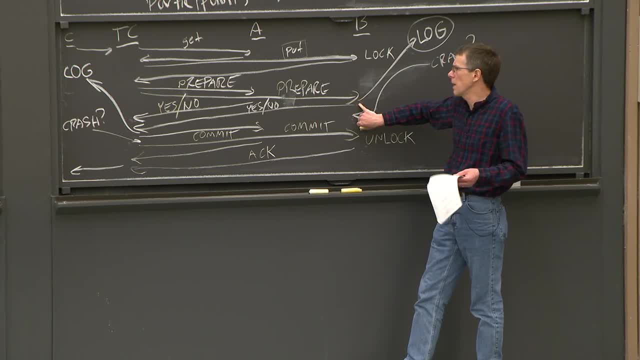 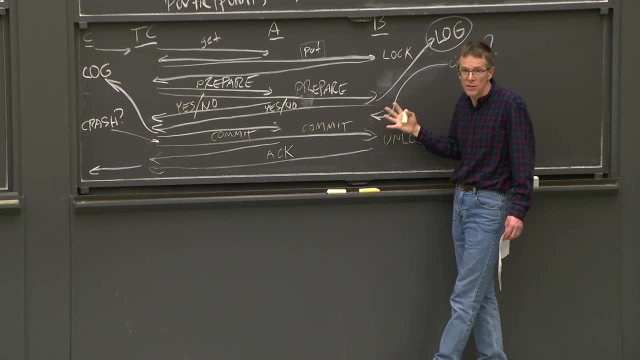 coordinator. its network connection has fallen out or its power's failed or something, but for whatever reason. B has waited a long time and it still hasn't heard a commit. But it's sitting there holding locks. it's still holding on to those locks, for all the records that. 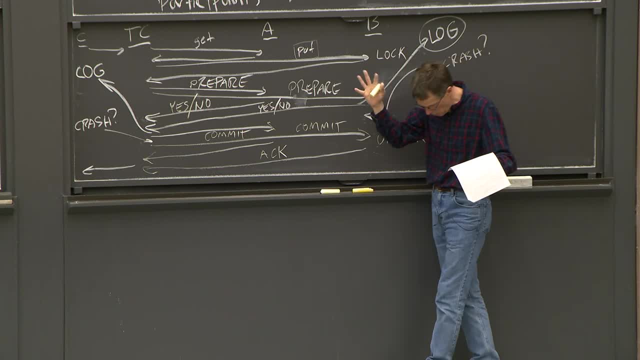 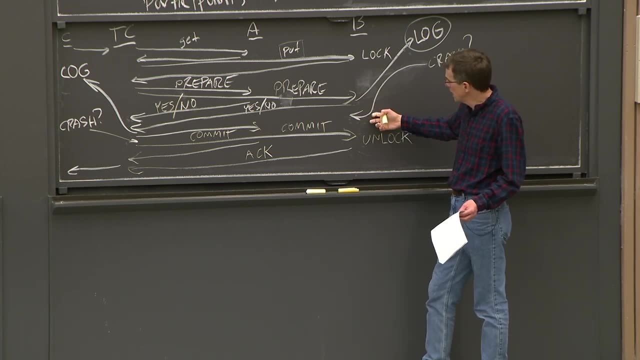 were used and it's part of the transaction, And that means other transactions may be also blocked waiting for those locks to be released. So we're pretty eager to abort if we possibly can, or release the locks. And so the question is: is B going to commit back? 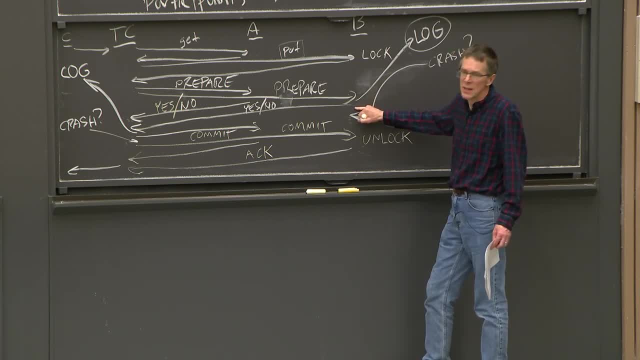 So if B has received prepare and replied with yes, is it entitled to unilaterally abort after it's waited, say 10 seconds or 10 minutes or something, to get the commit message? And the answer to that, unfortunately, is no In this region after receiving the prepare. 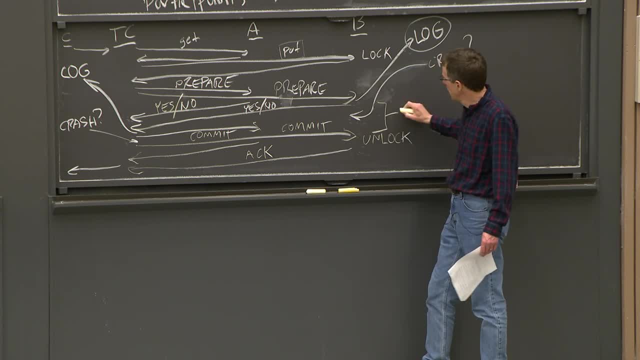 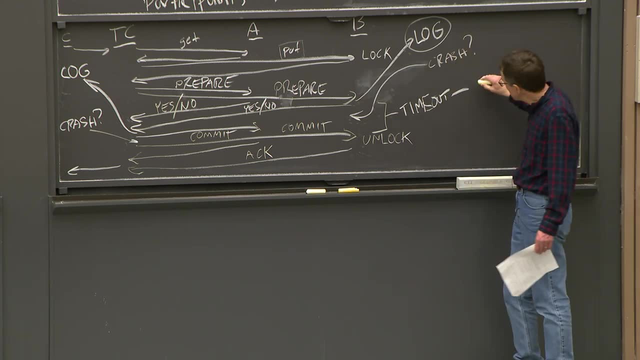 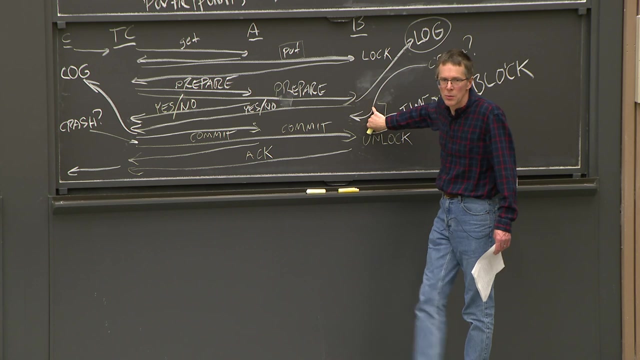 or really after sending the yes and before getting the commit. if you time out waiting for the commit, you're not allowed to abort. You must keep waiting. You must. it's usually called block. So in this region of the protocol, if you don't receive the commit, you have to wait. 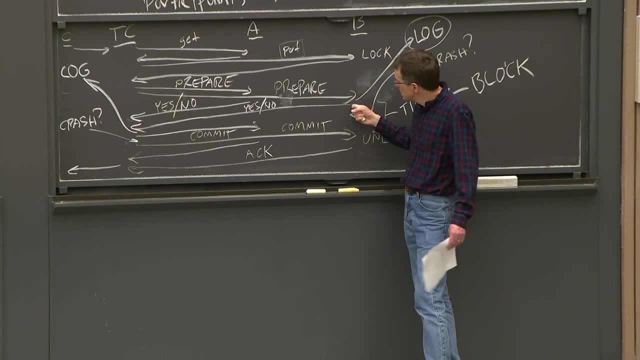 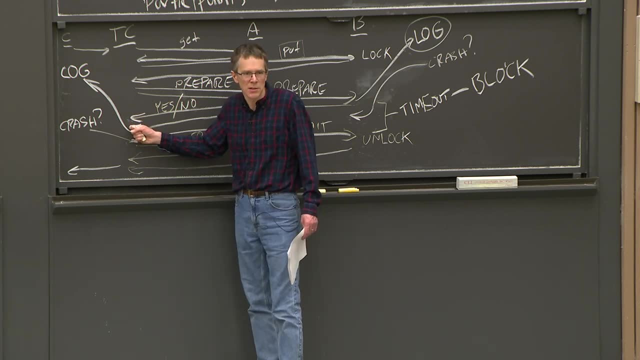 indefinitely And the reason is that since B sent back a yes, that means the transaction coordinator may have received the yes, It may have received yes from all of the participants and it may have started sending out commit messages to some of the participants. And 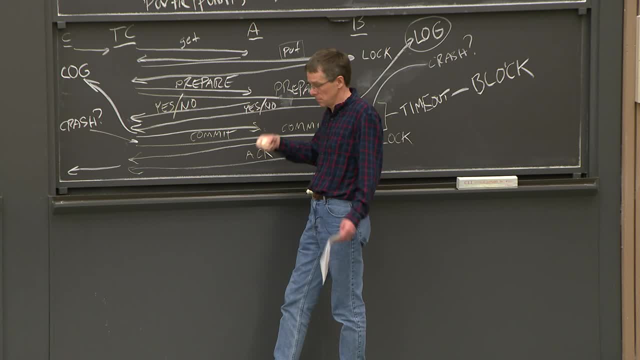 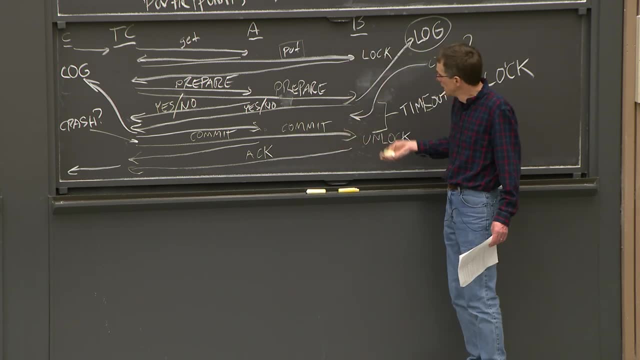 that means that A may have actually seen the commit message and committed and may have made those changes permanent and unlocked and shown the changes to other transactions. And since that could be the case for all B knows in this region of the protocol, B cannot. 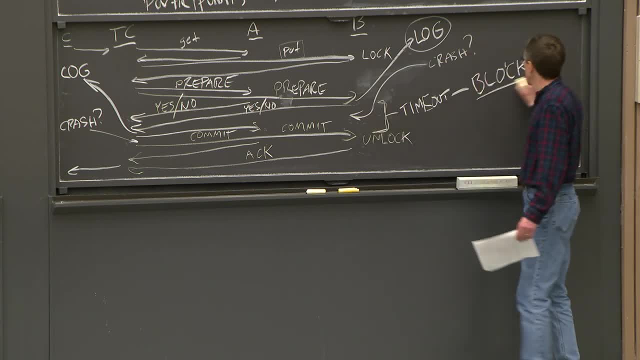 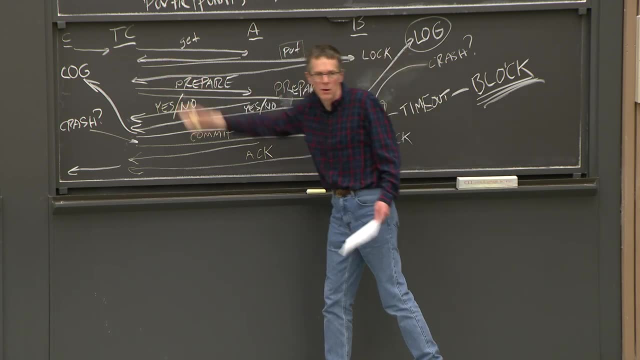 unilaterally decide to abort if the time's out. It must wait indefinitely to hear from the transaction coordinator as long as it takes, because some human may have to come and repair the transaction coordinator and finally get it started again and have it read. 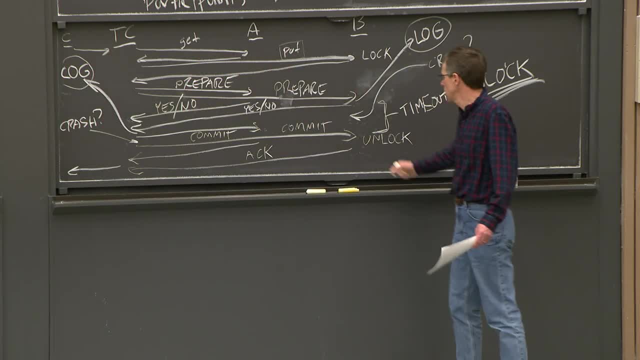 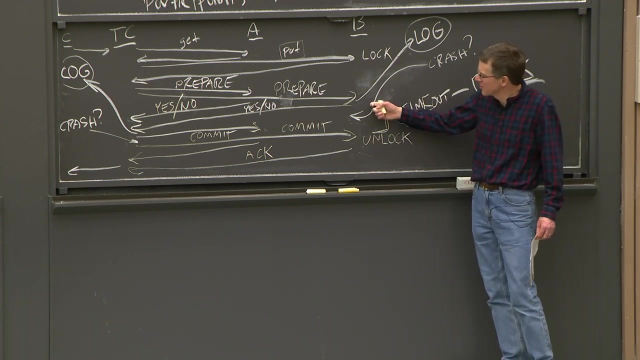 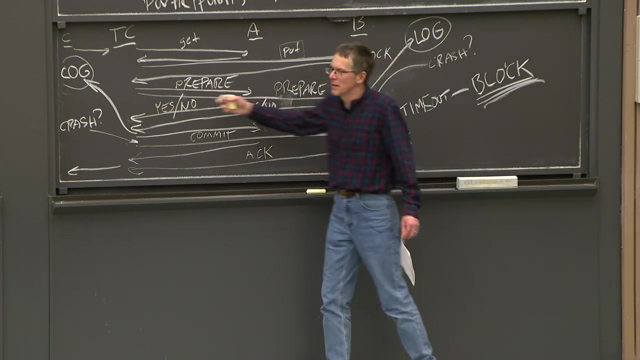 its log and see, oh yes, we committed that transaction and finally send long-to-late commit messages. So, and similarly, on a timeout, you can't unilaterally abort, It turns out, you can't unilaterally commit either, because, for all B knows, A might have voted no, but B just. 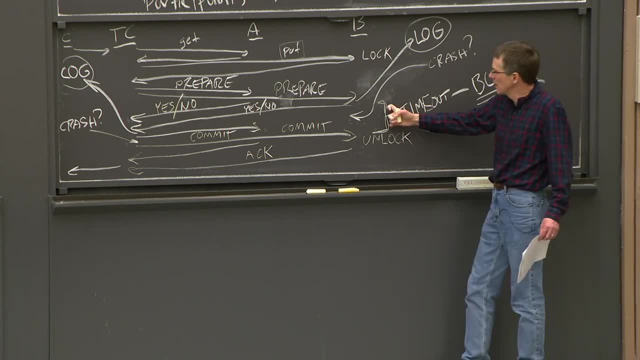 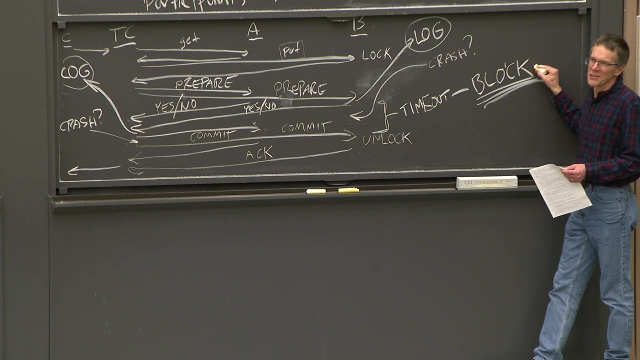 hasn't got the abort message yet, So you could. In this region you can neither abort nor commit on a timeout. So this, actually This blocking behavior, is a sort of critical property of two-phase commit, and it's not a happy property. 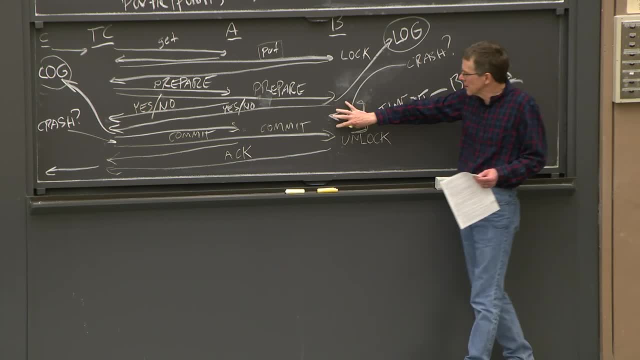 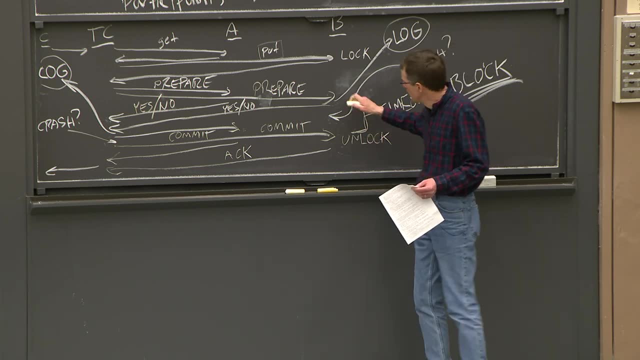 It means, if things go wrong, you can easily be in a situation where you have to wait for a long time with locks held and holding up other transactions, And so, among other things, People try really hard to make this part of two-phase commit as fast as humanly possible. 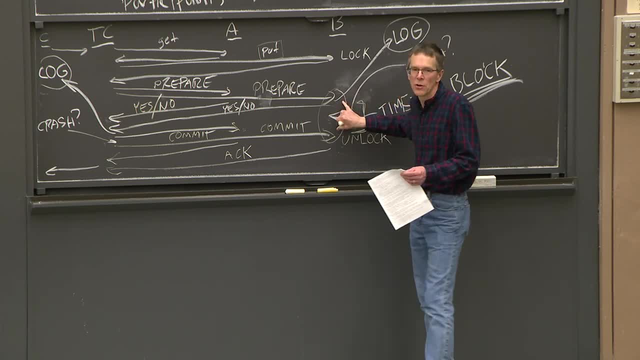 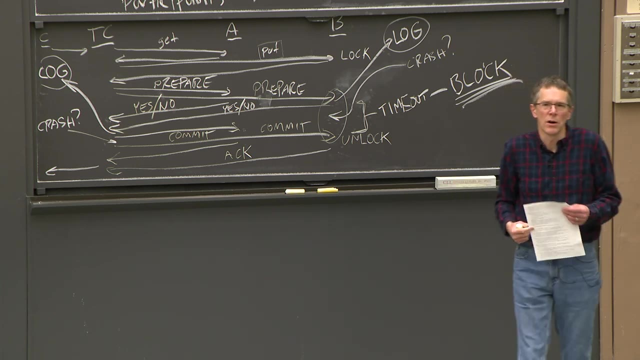 so that the window of time in which a failure might cause you to block with locks held for a long time is as small as possible. So they try to make this part of the protocol very lightweight or even have variants of the protocols that, for certain special cases, may not have to wait at all. 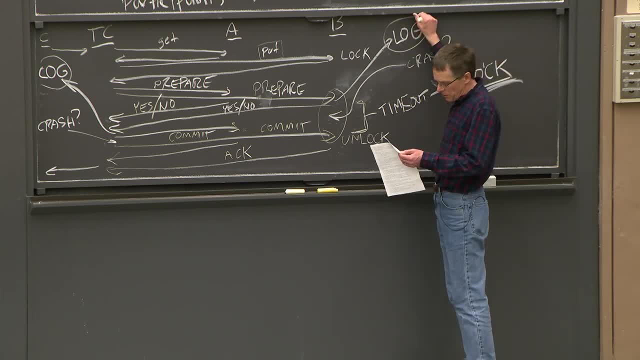 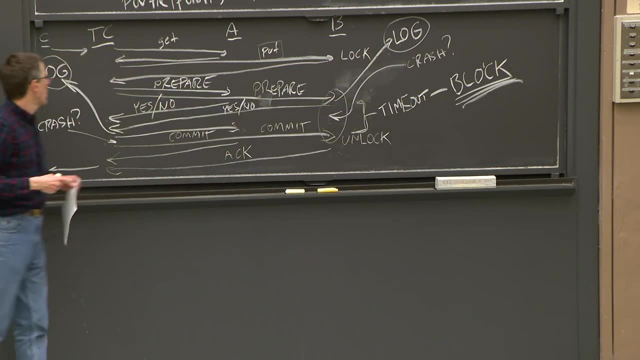 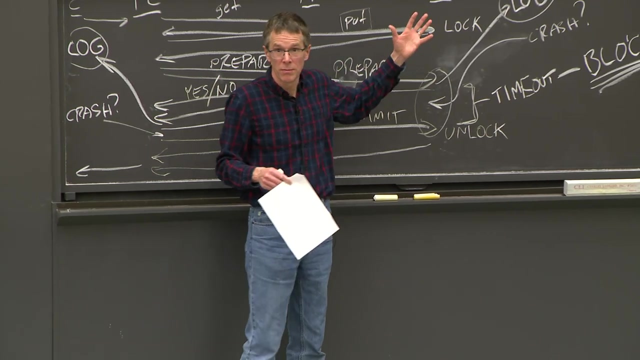 Okay, So, Okay. So that's the basic protocol. One thing to notice about this: that is a fundamental part of why we're able to get to actually build a protocol that allows A and B to sort of both: They both commit or they both abort. 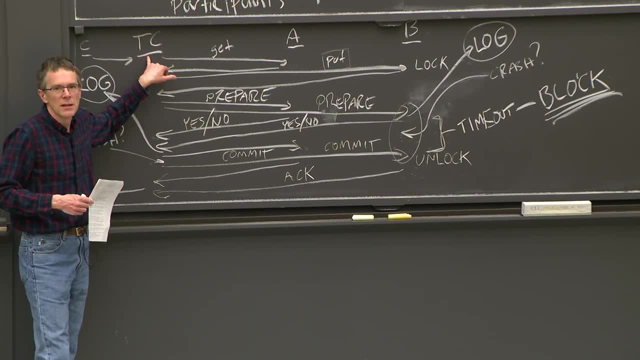 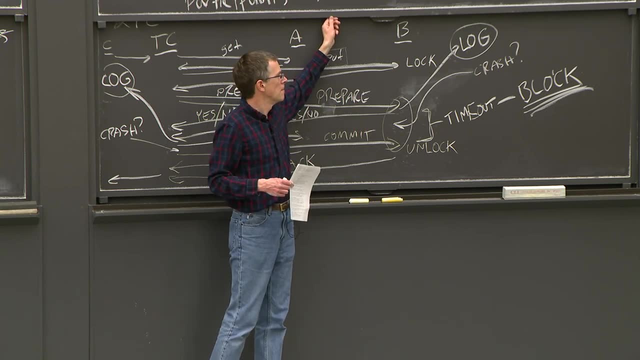 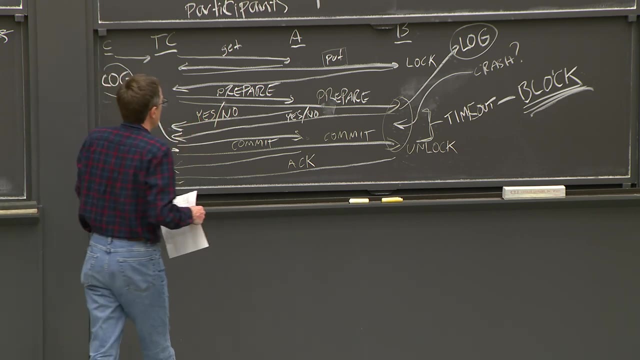 One reason for that is that really, the decision is made by a single entity. It's made by the transaction coordinator alone. A and B are neither of them, except that they vote no. Okay, So Neither A nor B is deciding whether to commit or not, and they certainly are not engaged. 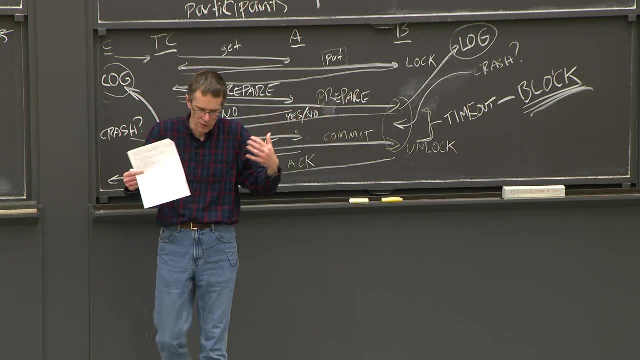 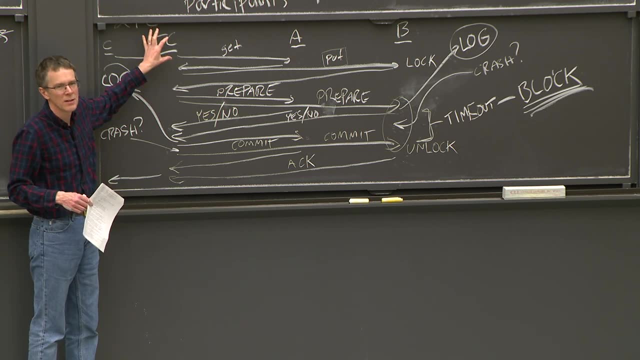 in a conversation with each other to try to reach agreement about. oh, what is the other thinking? Are they thinking commit, Maybe I'll commit too? Instead, we have this much, This quite sort of fundamentally simple protocol in which only the transaction coordinator 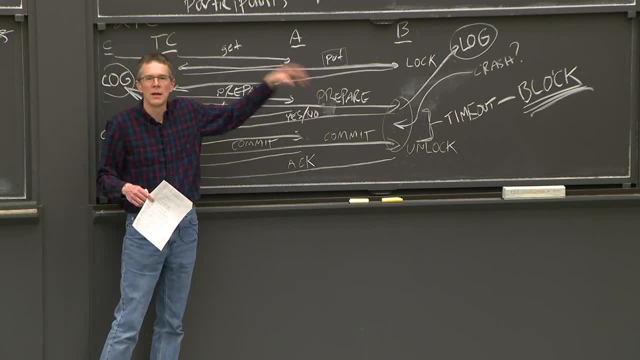 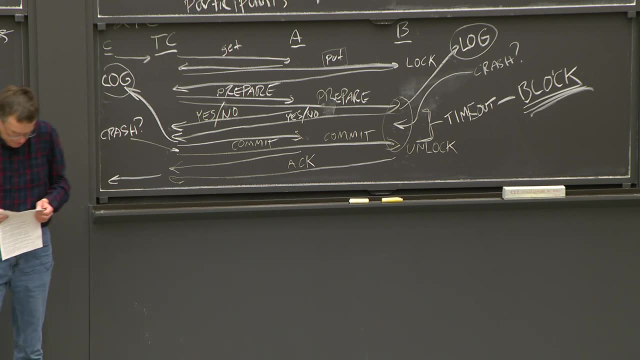 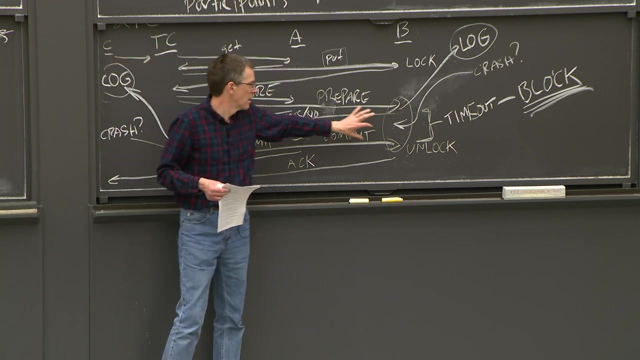 makes the decision a single entity and it just tells the other party: here's my decision, Please go do it. Okay, So The penalty for that- for having the transaction coordinator- really the single entity- make the final decision again- is the fact that you have to block. 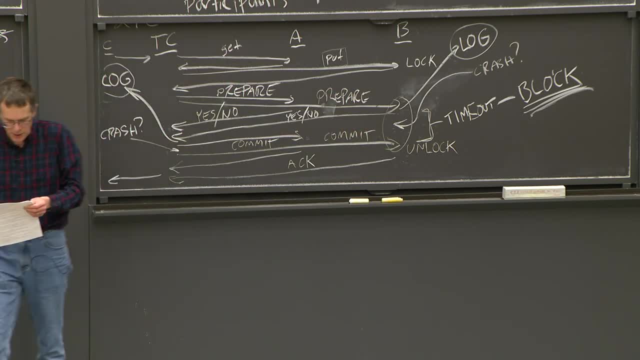 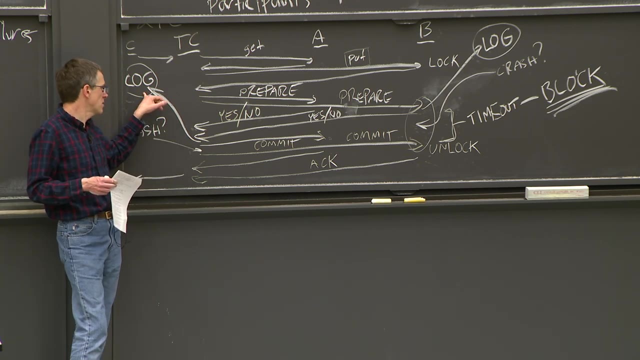 There's some points in which you have to block waiting for the transaction coordinator to tell you what the decision was. One further question is that we know the transaction coordinator must remember information about transactions in its log in case it crashes, And so one question is when the transaction coordinator can forget about information in 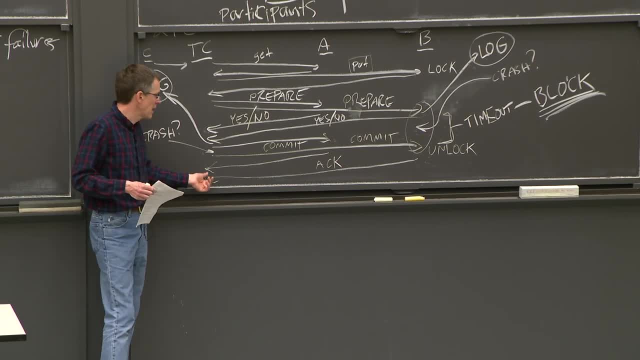 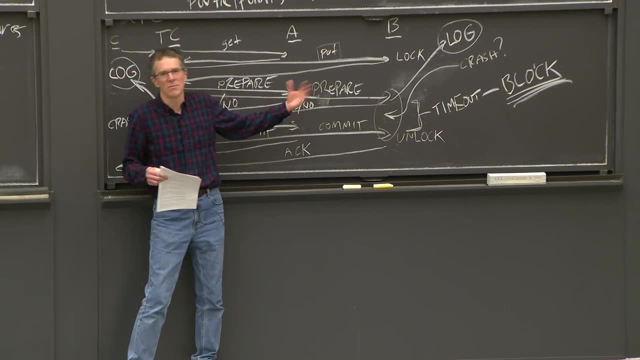 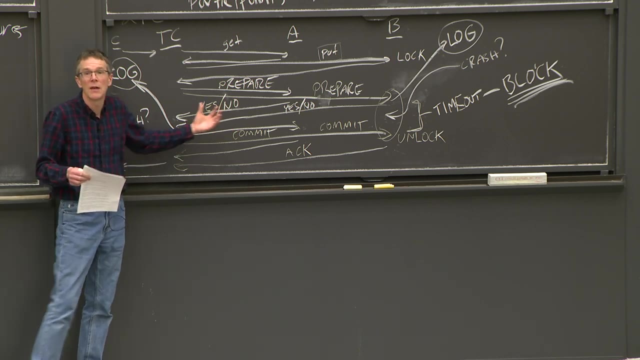 its log about transactions? And the answer to that is that if it manages to get a full set of acknowledgements from the participants, then it knows that all the participants know that that transaction committed or aborted, that all the transactions know Participants know the fate of that transaction and have done their part in it and will never. 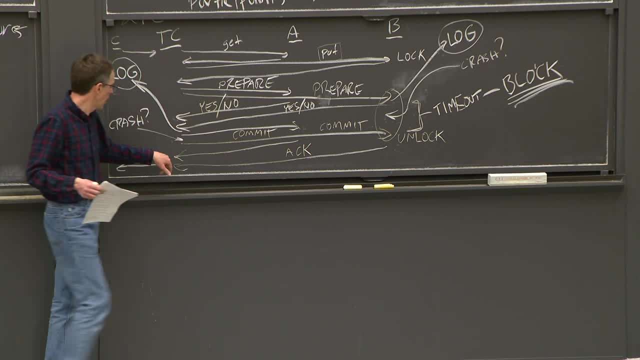 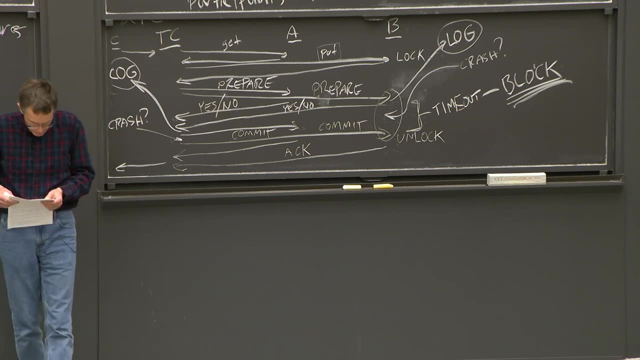 need to know that information right, since they both acknowledge it. So when the transaction coordinator gets acknowledgements it can erase all information, all memory of the transaction. Similarly, participants, once they've received a commit or abort message and done their, 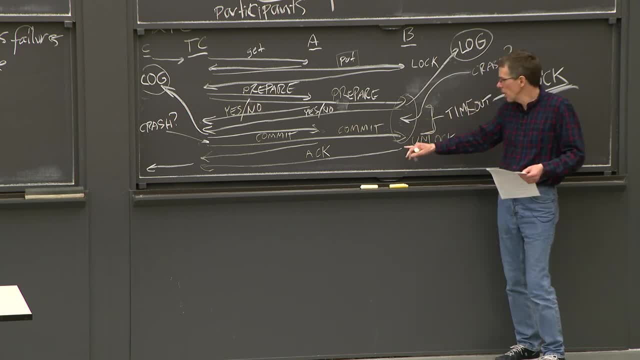 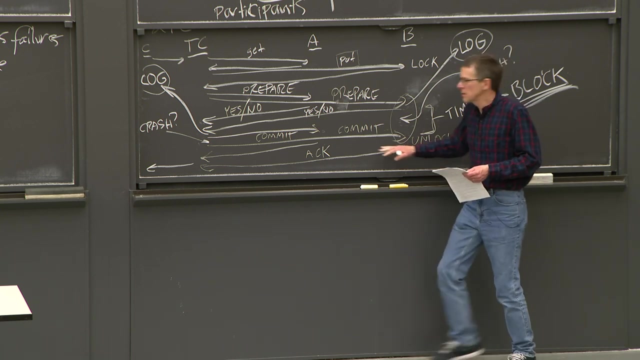 part in the transaction and made their updates permanent or released their locks. at that point, the participants also can completely forget about that transaction after they send their acknowledgement back to the transaction coordinator. Okay, Now of course, the transaction coordinator may not get their acknowledgement and may. 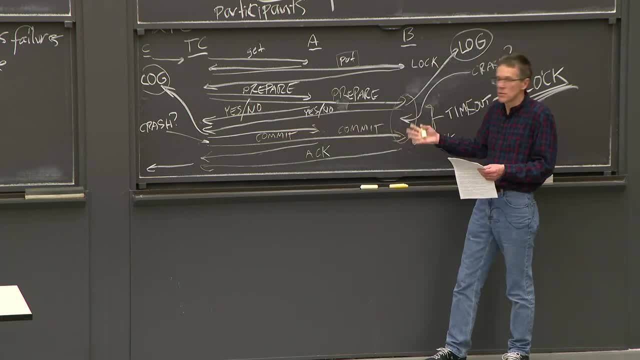 send and may therefore decide to resend the commit message on the theory that maybe it was lost, And in that case the participant, if it receives a commit message for a transaction which it knows nothing about because it's forgotten about it, then the participant can. 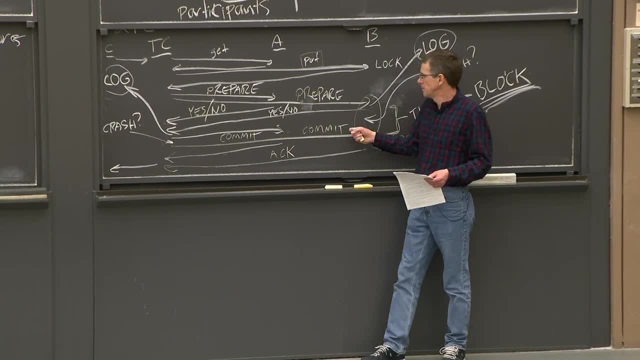 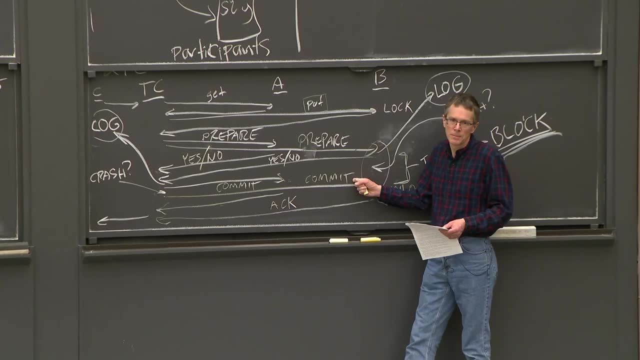 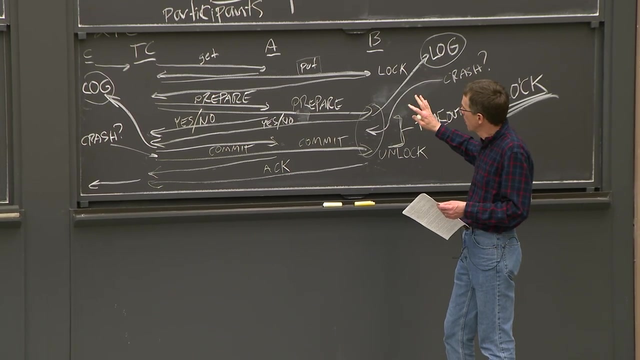 just send another acknowledgement back, because it knows that if it gets a commit message for an unknown transaction, it must be because it had forgotten about it, because it already knew whether it committed or aborted. Okay, So that's two-phase commit for atomic commitment. 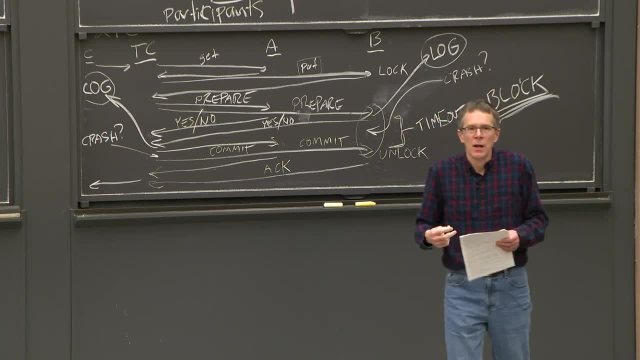 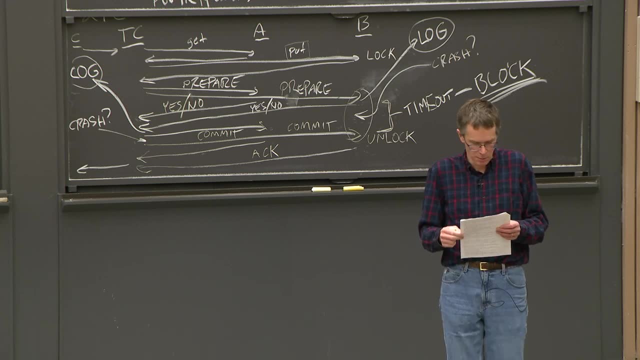 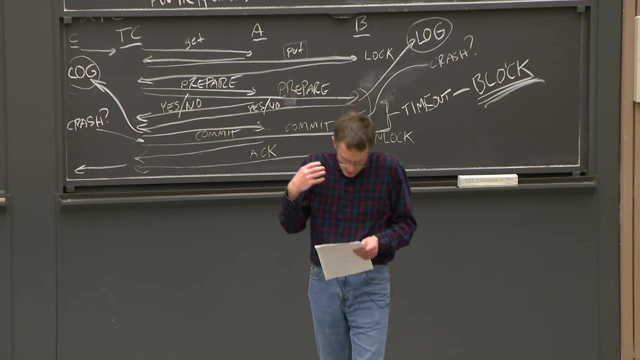 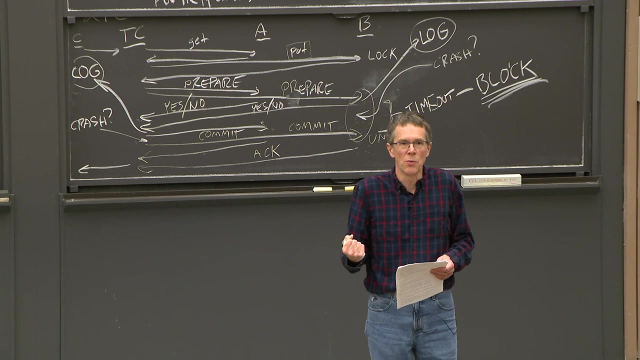 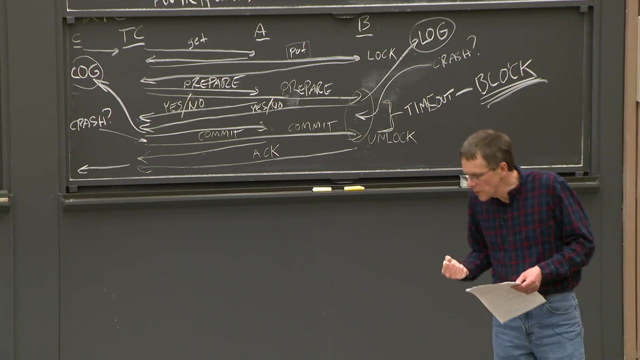 For a little perspective. two-phase commit is used in a lot of sharded databases that have split up their data among multiple servers, and it's used specifically in databases or storage systems that need to support transactions. There's a lot of more specialized storage systems that don't allow you to have transactions. 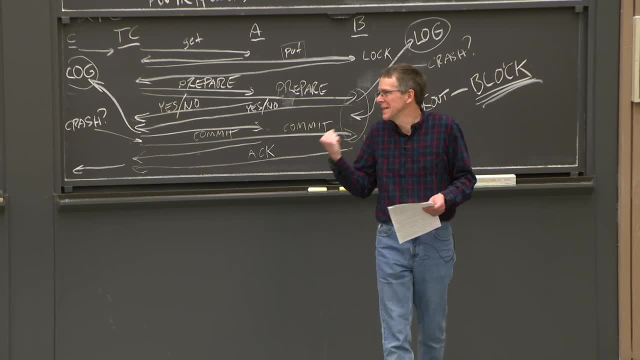 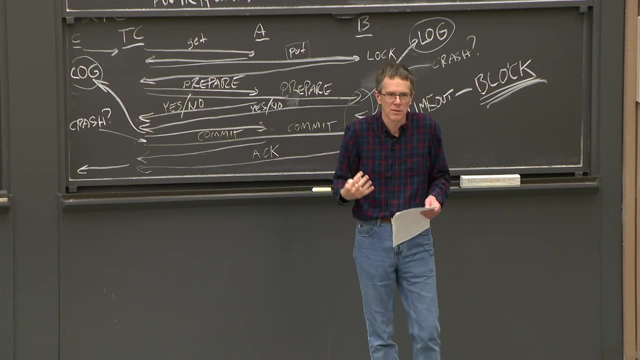 on multiple records and for them you don't need this kind of you don't need two-phase commit if the storage system doesn't allow multi-record transactions. But if you have multi-record transactions and you shard the data across multiple servers, then you need to support either two-phase commit or two-phase commit. 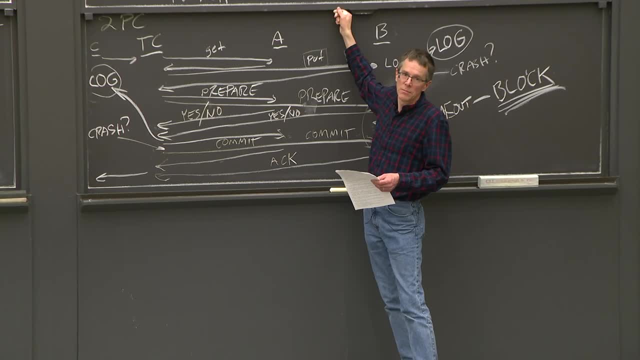 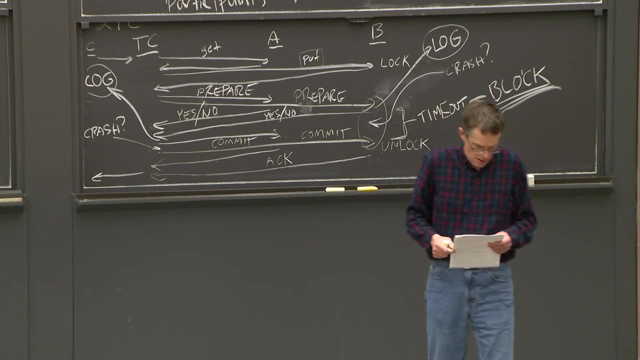 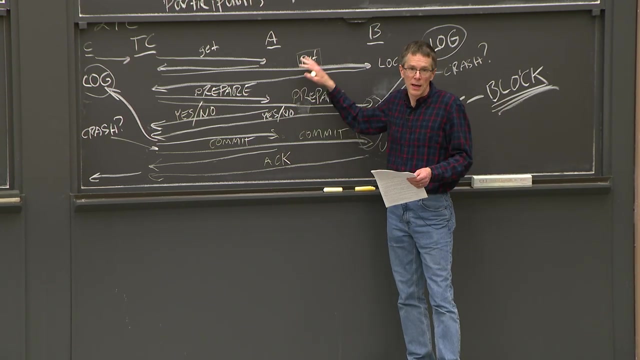 Okay, So you need to support two-phase commit if you want to get ACID transactions. However, two-phase commit has an evil reputation. One reason is it's slow due to multiple rounds of messages. There's a lot of chit-chat here in order to get a transaction that involves multiple participants. 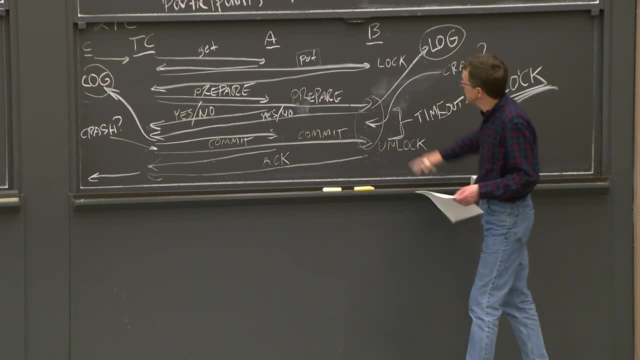 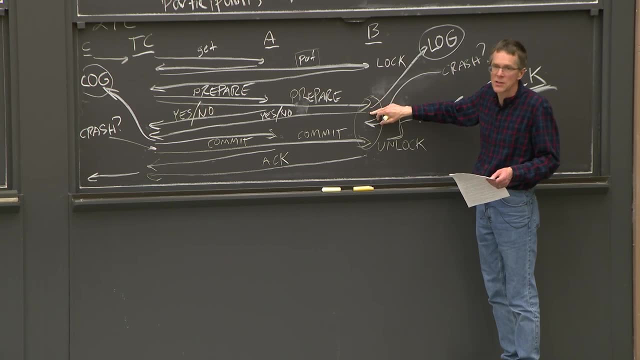 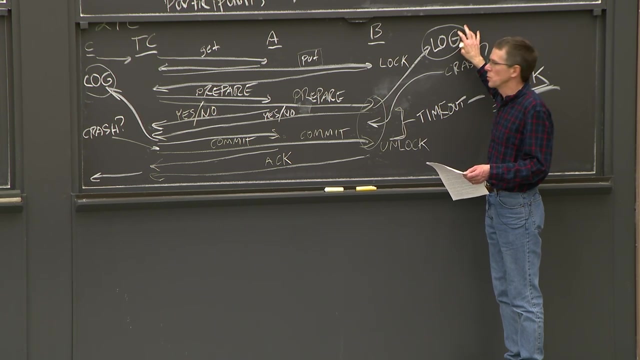 to finish. There's, in addition, a lot of disk writes. Both A and B have to not just write data to their disk between the prepared, They have to wait for that disk write to finish. So certainly if you're using a mechanical drive, that takes 10 milliseconds to append. 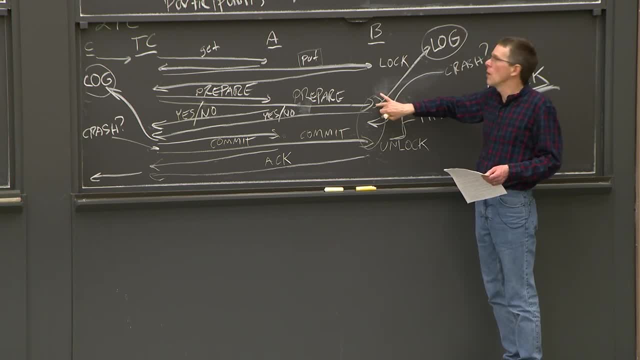 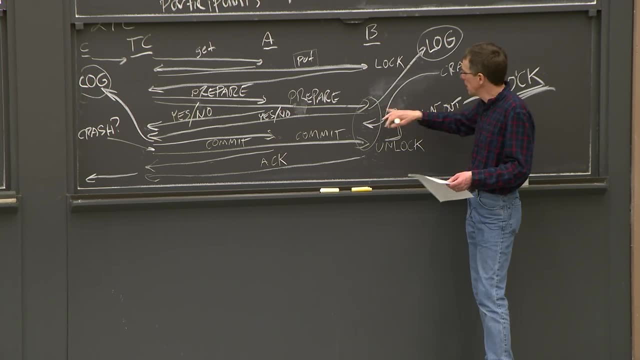 to the log. that puts a real serious limit on how fast participants can process transactions. You know, 10 milliseconds a pop means, you know, without some cleverness you're limited to 100 transactions per second, which is pretty slow. 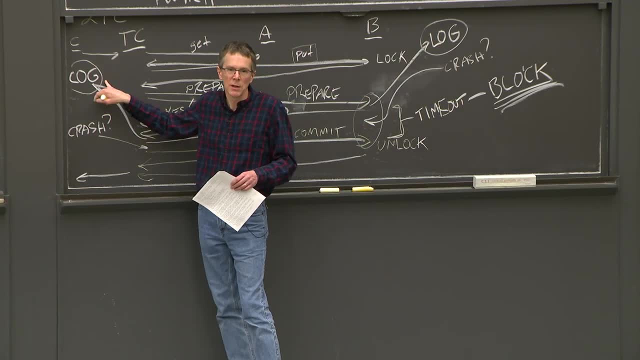 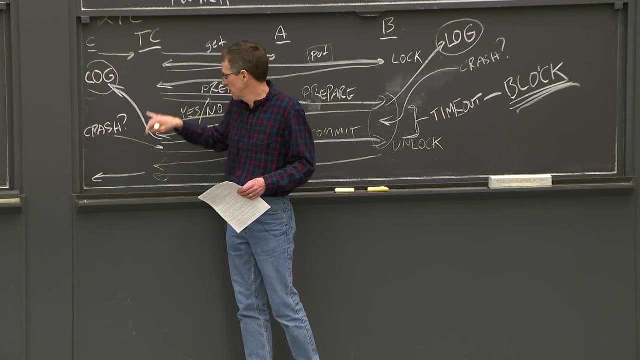 And in addition, the transaction coordinator also has a point in which it must, after it receives the last yes, It must first write to its log, make sure the data is safe on disk, and only then is it allowed to send the commit messages. 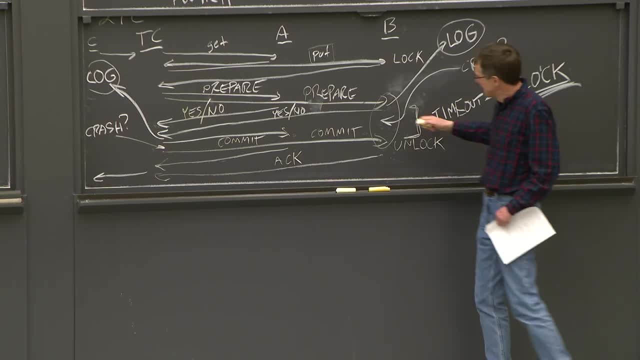 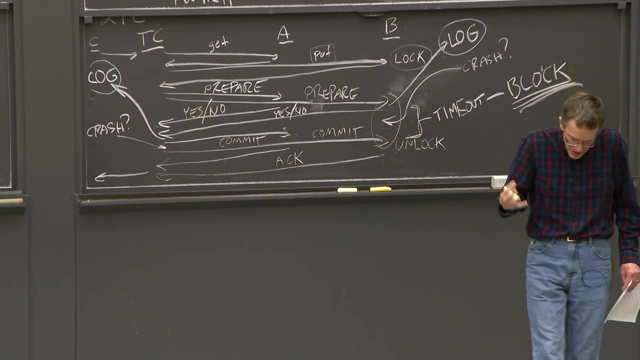 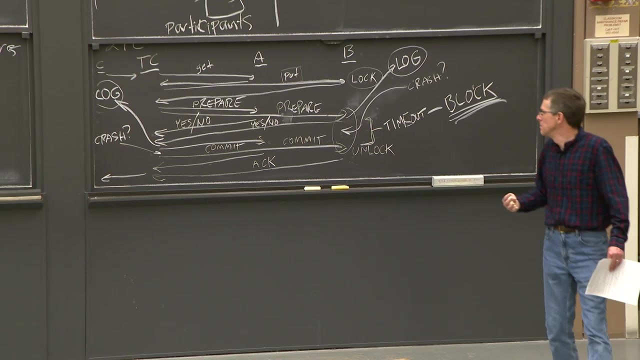 And that's another 10 milliseconds, And both of these are 10 millisecond periods in which locks are held and the participants and other transactions are slowed up, And I keep mentioning that. but it's very important because in a busy transaction processing system there's lots and lots of transactions. 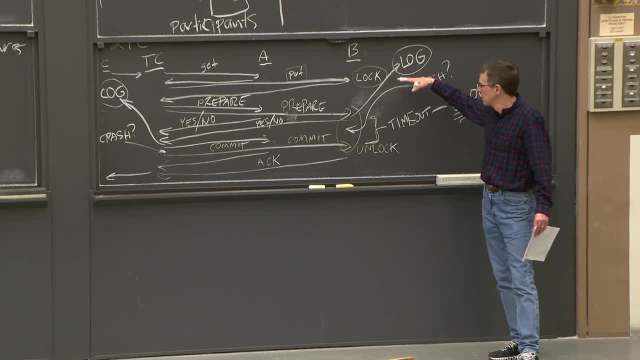 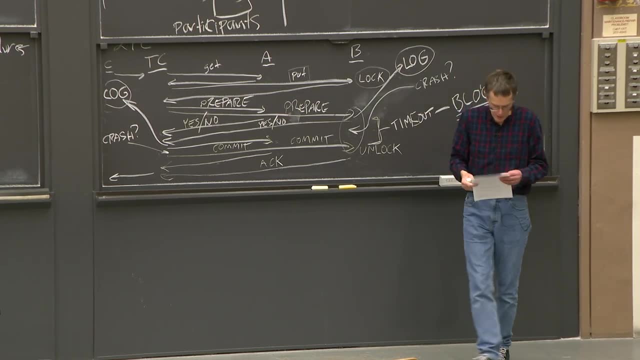 And many of them may be waiting for the same data, And we'd really prefer not to hold on to that, Not to hold locks over long periods of time in which there's lots of messages going back and forth and we have to wait for long disk writes. 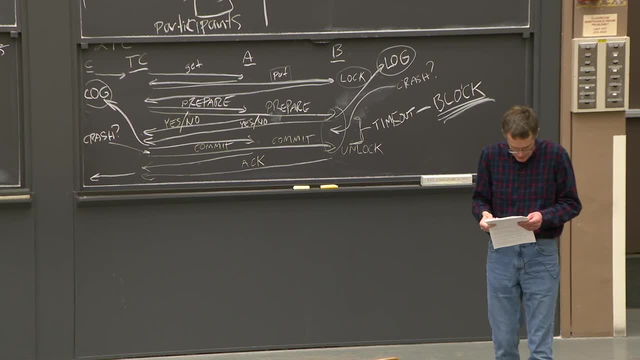 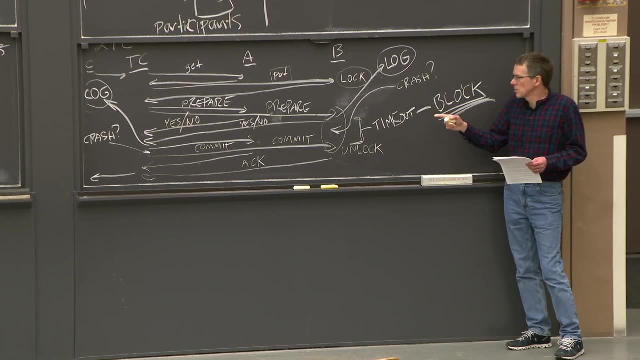 But Two-Face Commit forces us to do those waits. And a further problem with it is that if anything goes wrong, messages are lost, something crashes, then if you're not, if you're a little bit unlucky, then the participants have to wait. 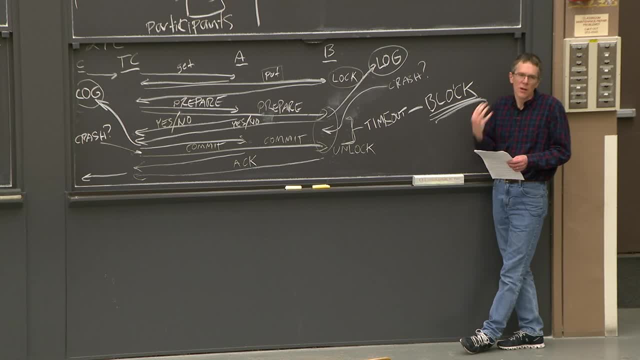 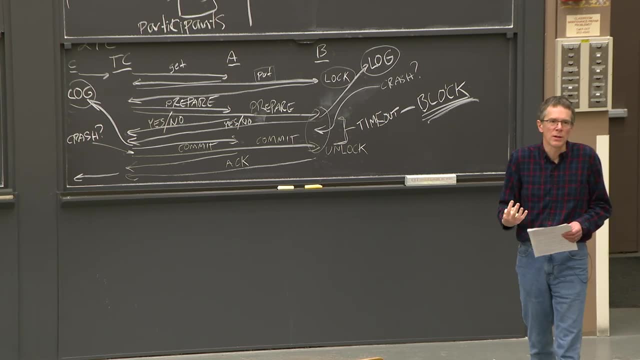 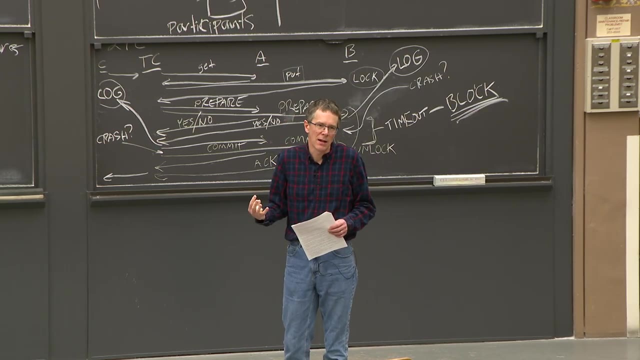 for long times with locks held. So therefore, Two-Face Commit, You really only see it within relatively small domains, within a single machine room, within a single organization. You don't see it, for example, to do transfers between banks, between different banks. 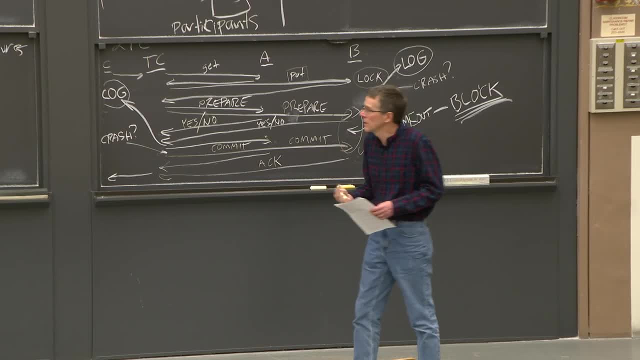 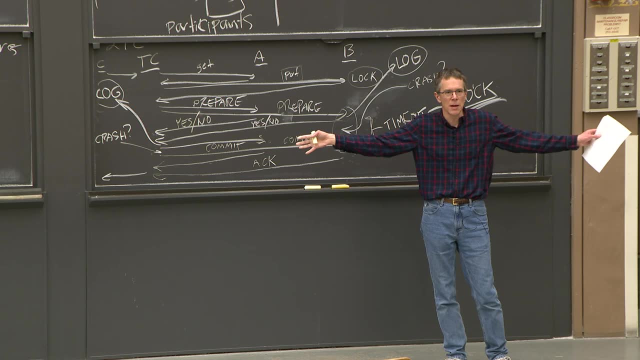 You might possibly see it within a bank if it's sharded its database, but you would never see Two-Face Commit run between distinct organizations that were maybe physically separate because of this blocking business. You don't want to put the fate of you know your database and whether it's operational. 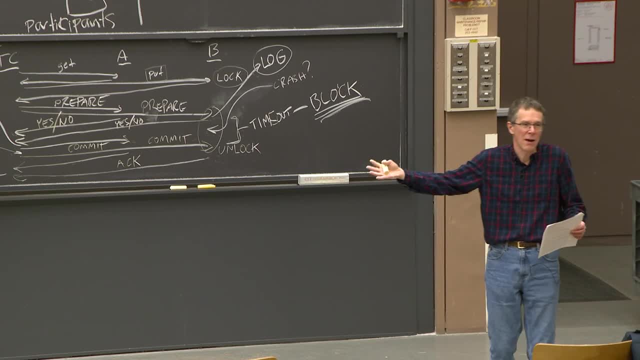 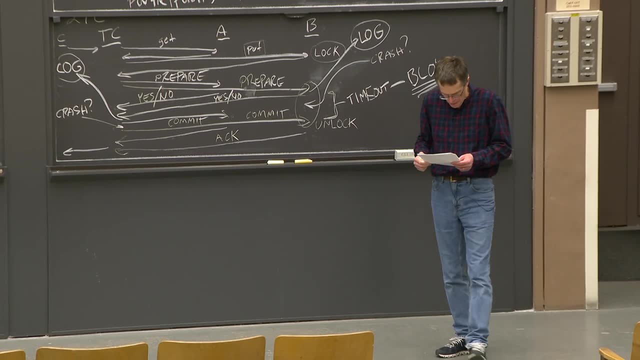 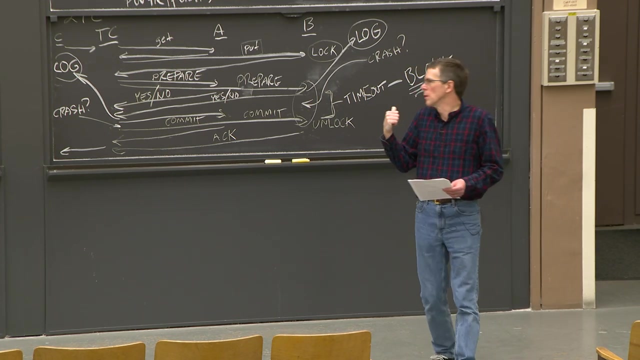 in the hands of some other organization where, if they crash at the wrong time, you're forced, your database is forced- to hold locks for a long time, And because it's so slow. also, there's a lot, a lot of research has gone into either making 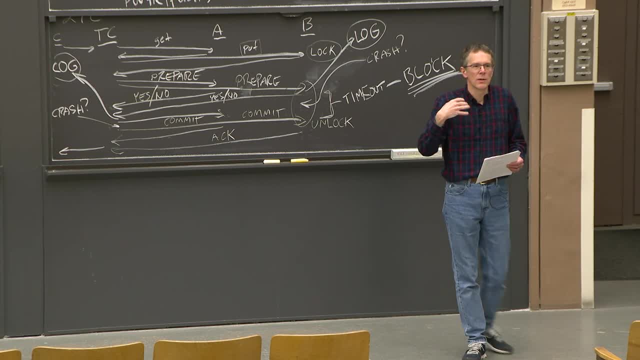 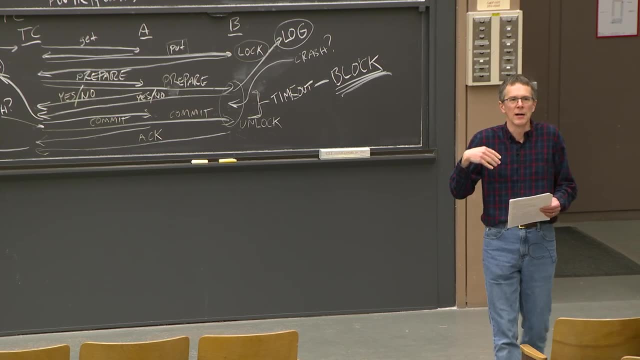 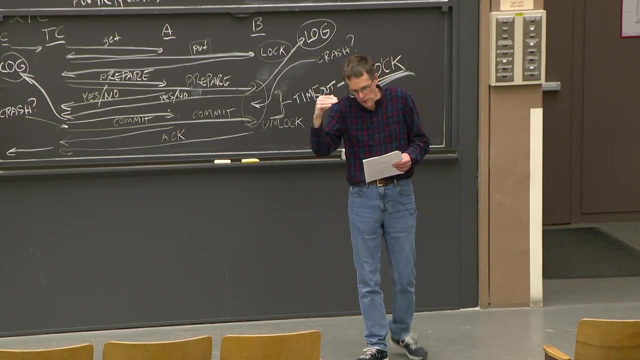 it fast, or relaxing the rules in various ways to allow it to be faster, or specializing Two-Face Commit for very specific situations In which you know you can shave a message or write to the disk or something off it, because you know you're only supporting a certain limited kind of transaction. 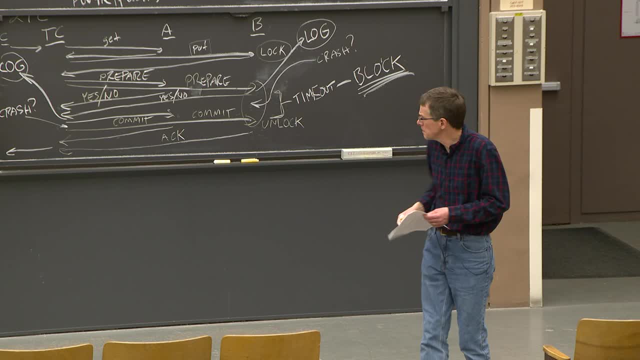 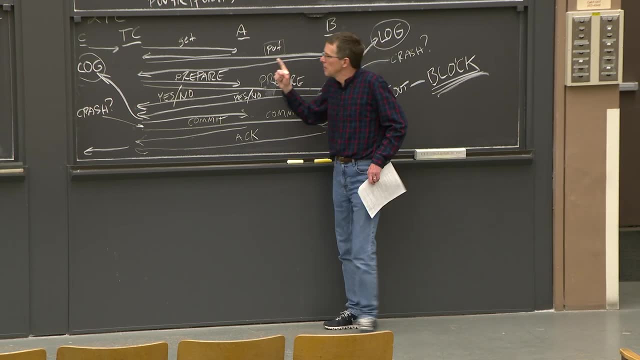 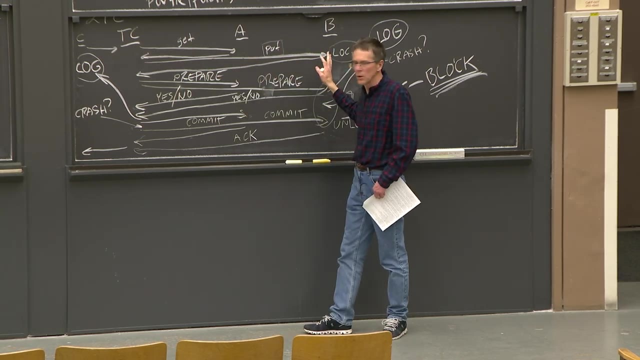 So we'll see a fair amount of this in the rest of the course. One question that comes up a lot: this exchange here, where you have a leader, essentially, and it sends these messages to the followers, And you know we can only go forward. 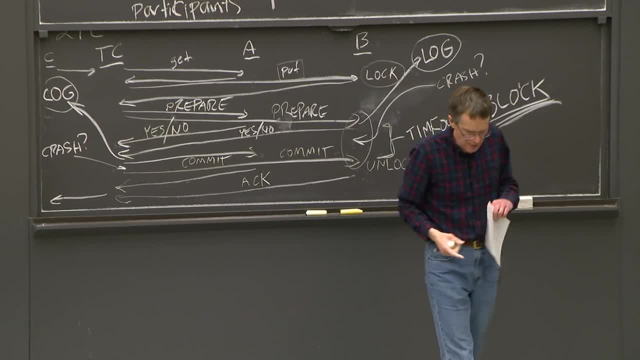 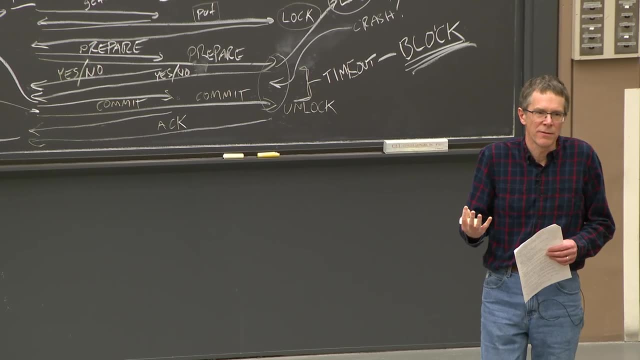 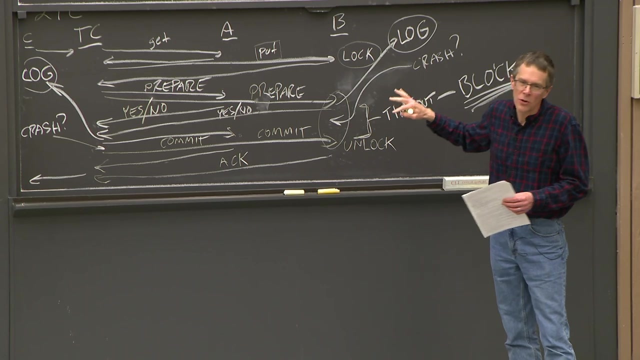 We go forward if the leader can only proceed if it receives, you know, acknowledgments, replies from enough of the followers. This looks a lot like Raft. This construction looks a lot like Raft. However, the properties of the protocol and what you get out of it turn out to be quite 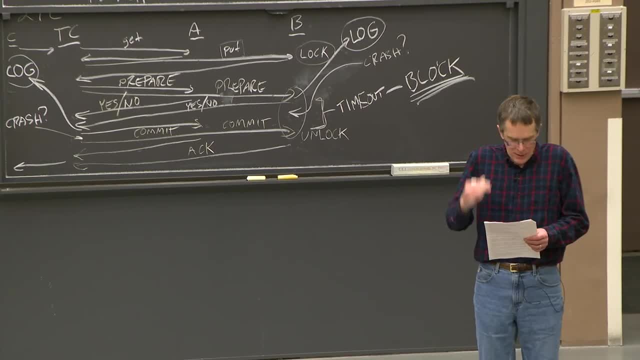 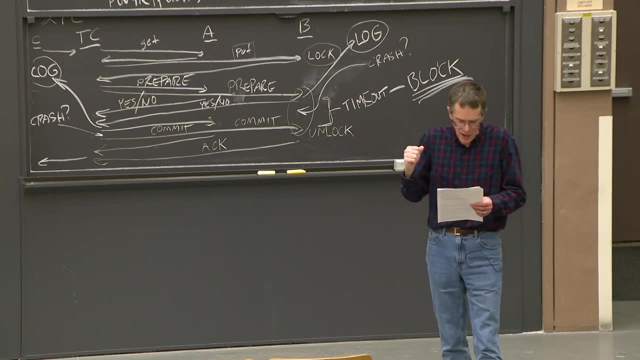 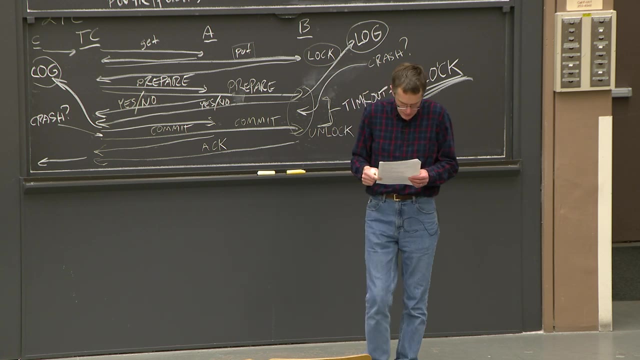 different from what we get out of Raft. They solve very different problems. So the way to think about it is that you use Raft. You use Raft to get high availability by replicating data on multiple participants, on multiple peers. That is the point of Raft, is to be able to operate, even though some of the servers involved 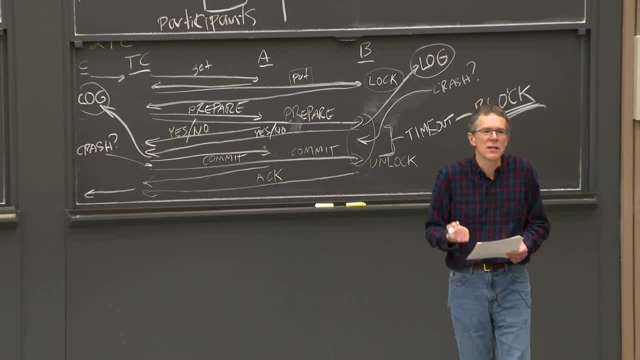 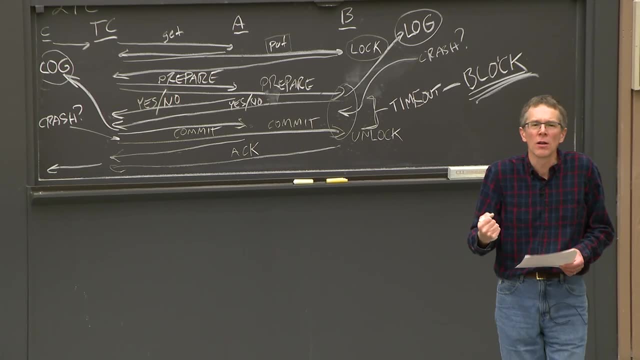 have crashed or are not reachable, And you can do this in Raft. Raft can do this because all the servers are doing the same thing. They're doing the same thing, So we don't need all of them to participate, We only need a majority. 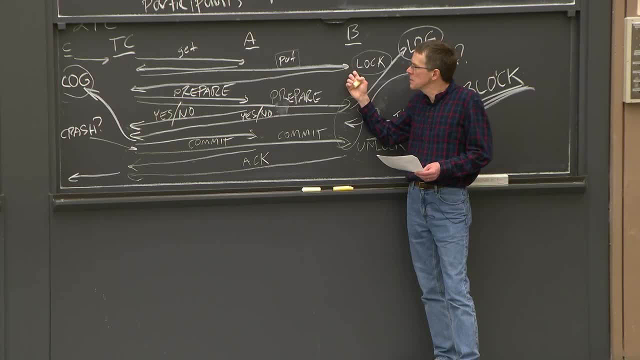 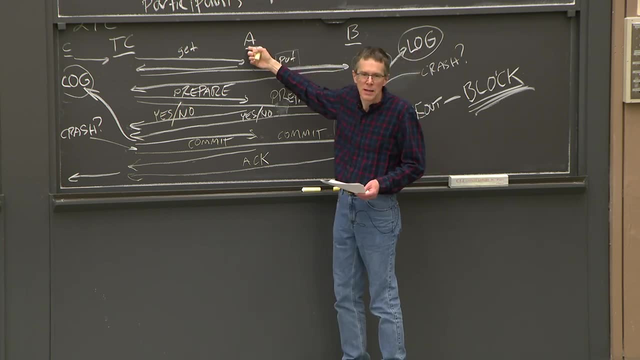 Two-Face Commit. Two-Face Commit. however, the participants are not at all all doing the same thing. The participants are each doing a different part of the transaction. You know, A may be incrementing record X and B may be decrementing record Y. 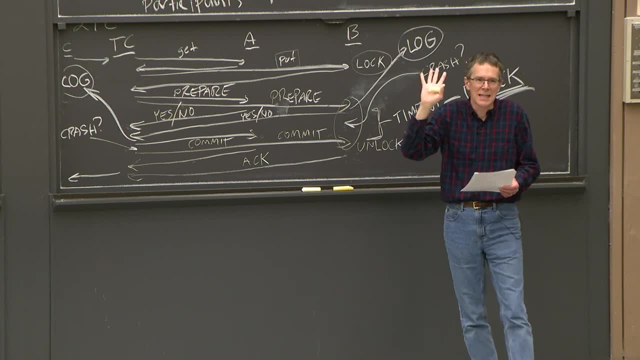 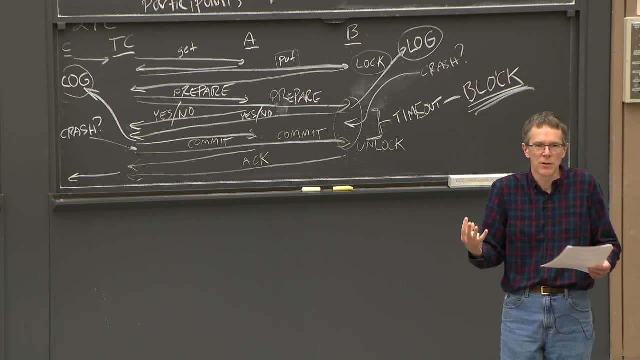 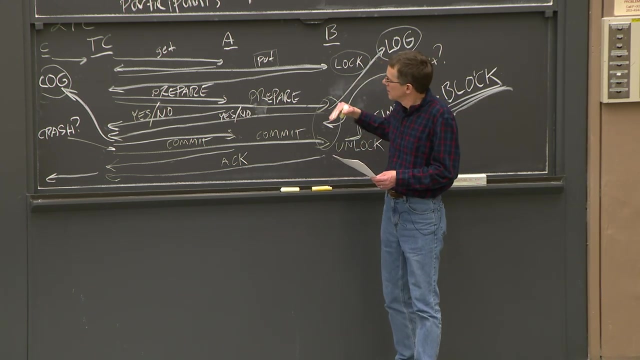 So Two-Face Commit: all the participants are doing something different. They all have to do their part in order for the transaction to finish. You really need to wait for every single one of the participants to do their thing. Okay, So, okay. so we got you know. Raft is replicating, doesn't need everybody to do their thing. 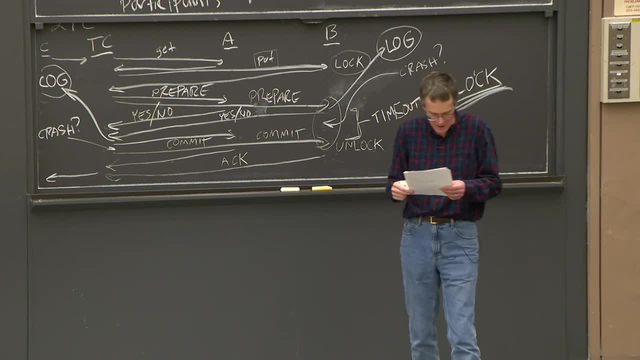 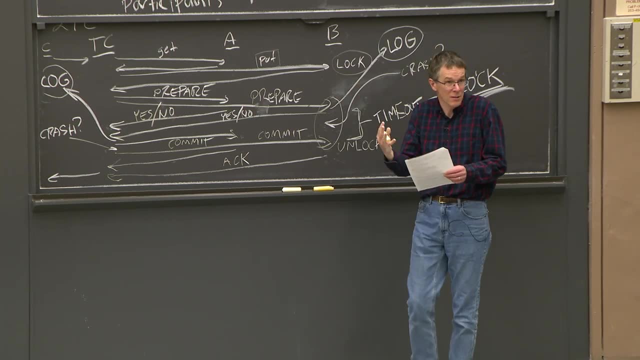 Two-Face Commit. everybody's doing something different that has to get done. Two-Face Commit does not help at all with availability. You know, Raft is all about availability. It can go on, even if some of the participants are not responding. 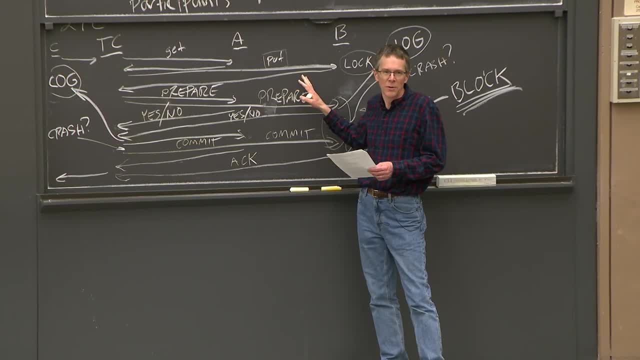 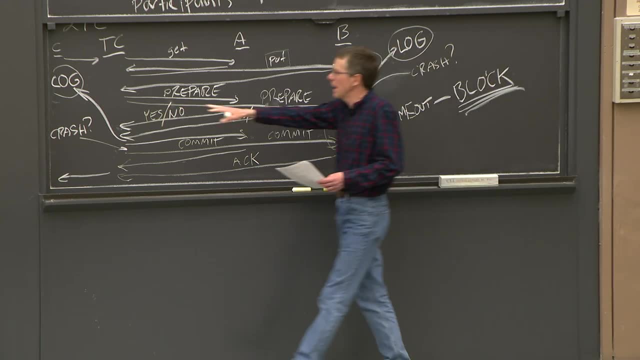 Two-Face Commit is actually not at all available. It's not highly available at all. If anything goes wrong, we risk. We risk having to wait until that's repaired. If the transaction coordinator crashes at the wrong time, we simply have to wait for. 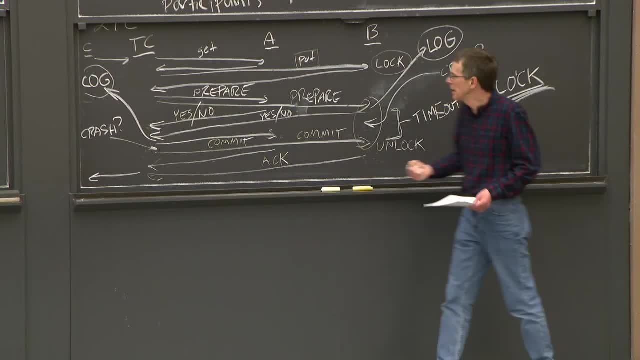 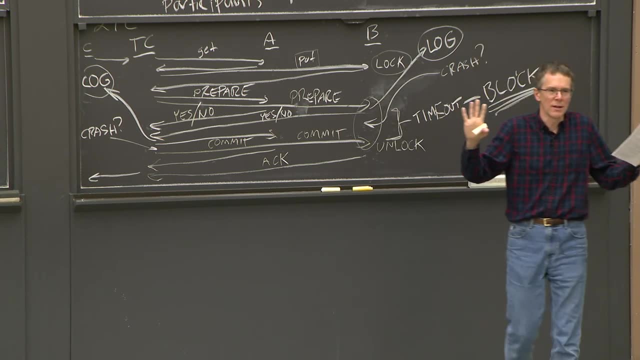 it to come up and read its log and send out the commit messages, Right? If one of these participants you know crashes at the wrong time, you know, if we're lucky, we simply have to abort And if we're not lucky, we have to say: you know, did you finish that? 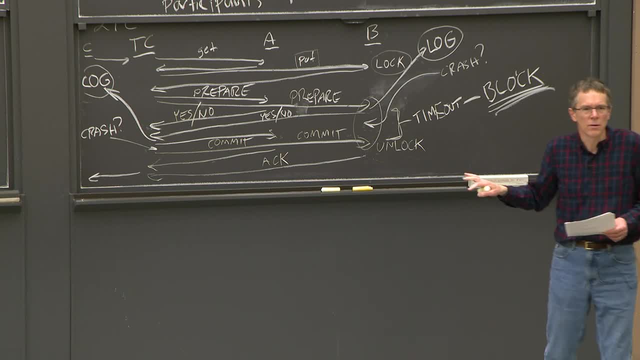 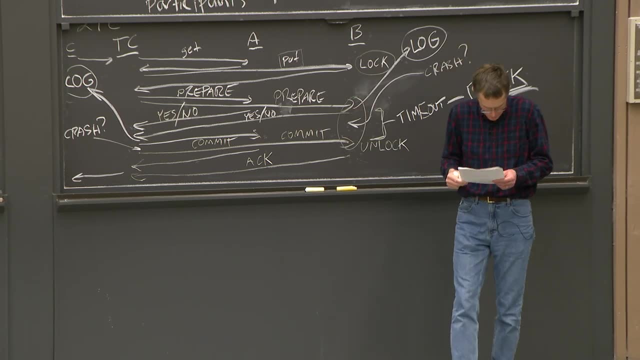 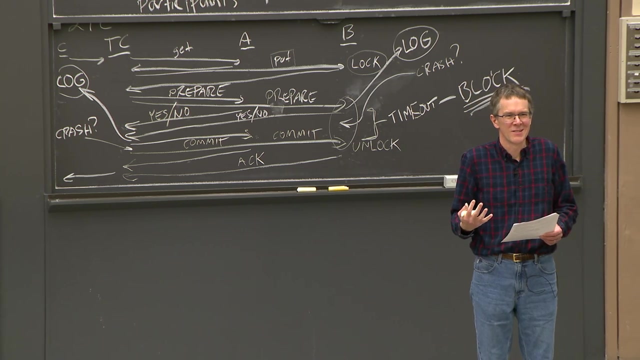 Did you finish that? So Two-Face Commit is not at all about high availability. In fact it's quite low availability as such things go. Any crash can hold up the whole system And of course Raft doesn't ensure that all the participants do whatever the operation. 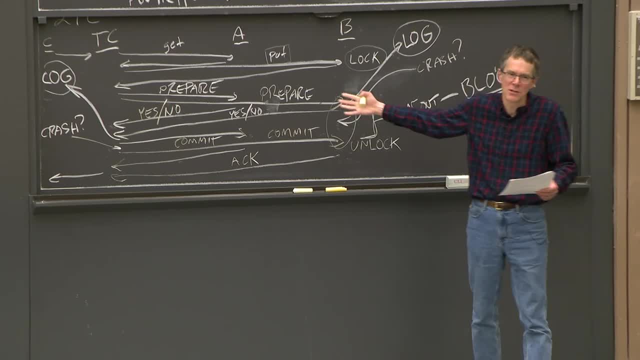 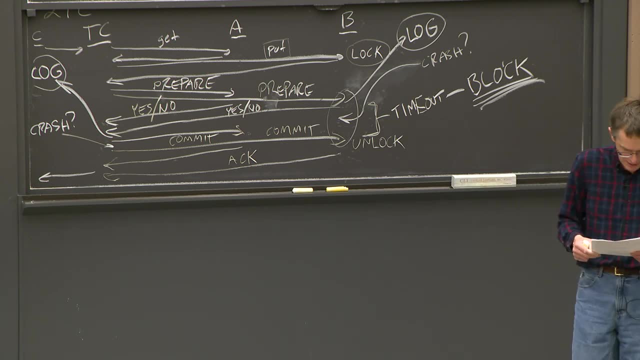 is. It only requires a majority. There may be a minority that totally didn't do the operation at all, And that's how. the fact that Raft all the participants do the same thing and we don't have to wait for all of them is why Raft gets high availability. 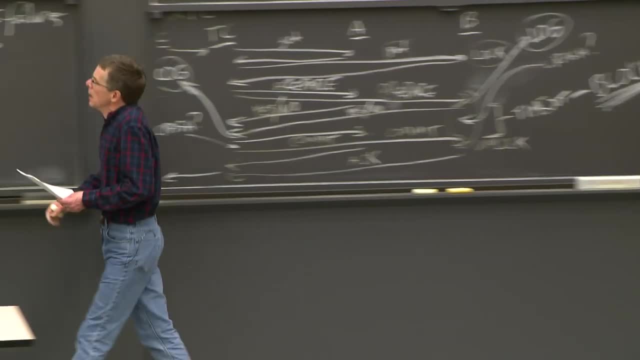 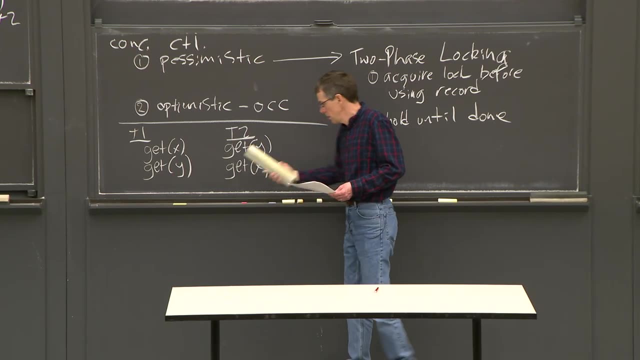 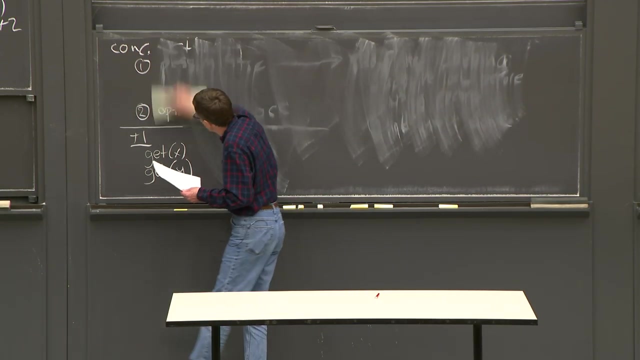 So these are quite different protocols. It is, however, possible to usefully combine them. The Two-Face Commit is, you know, really vulnerable to failures. It's correct with failures, but it's not available with failures. So the question is: could you build some sort of combined system that has the high availability? 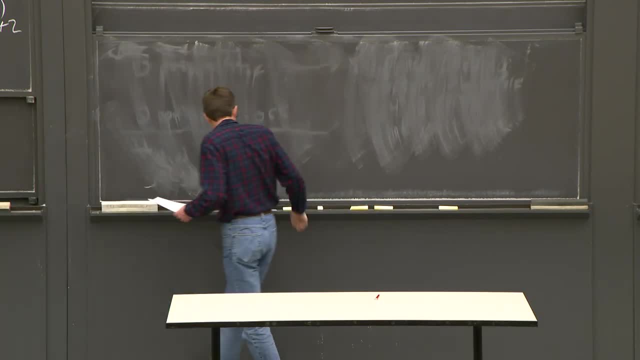 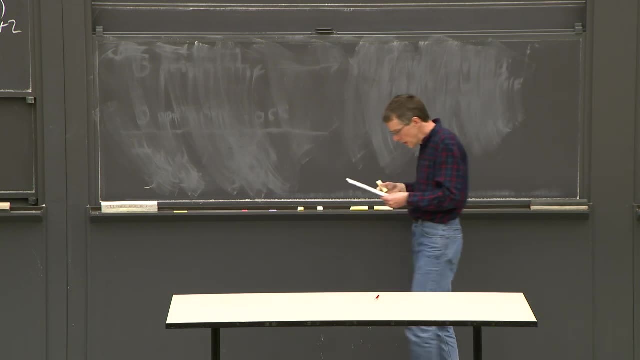 of Raft through replication, but has Two-Face Commit's ability to cause various different parties each to do their part of the transaction, And the construction you want actually is to use Raft or Paxos or some other kind of system. 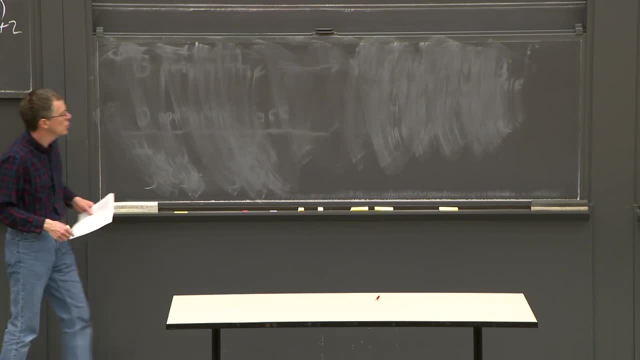 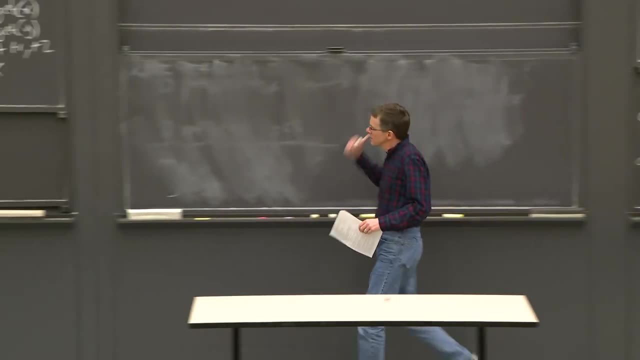 And that's what we're trying to do. We're trying to use Raft or Paxos or some other protocol like that to individually replicate each of the different parties. So then we would, for this setup, we would have three different clusters. 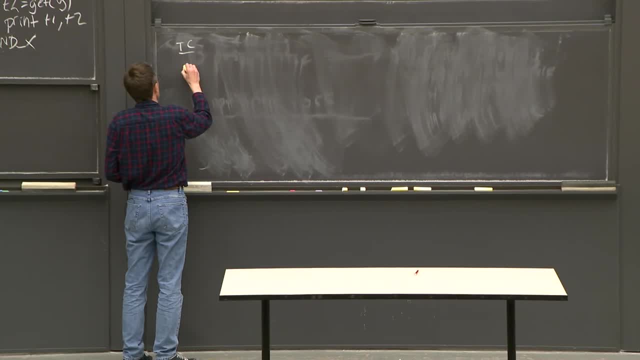 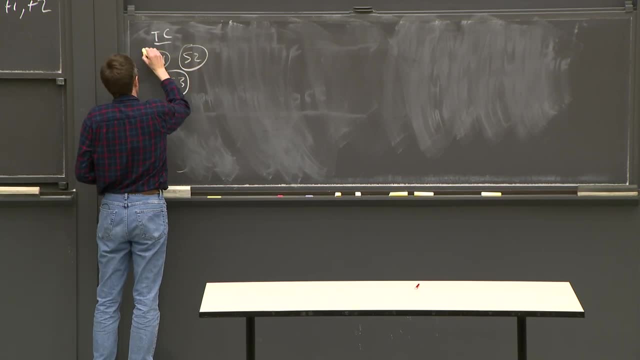 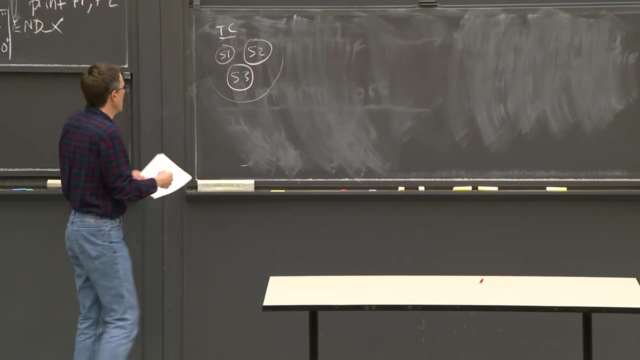 The transaction coordinator would actually be a replicated service with three servers And we'd run Raft on these three servers. One would be elected as a leader. They'd have replicated state. They'd have a log. They'd have a log that helped them replicate. 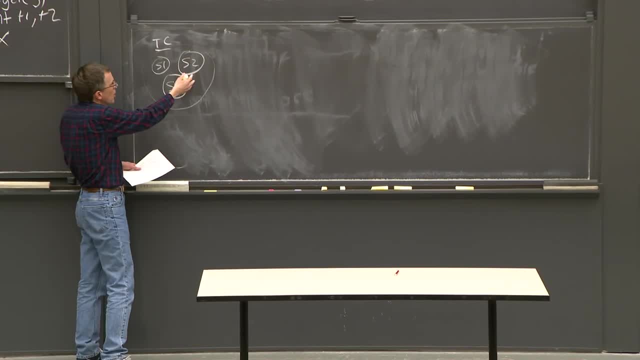 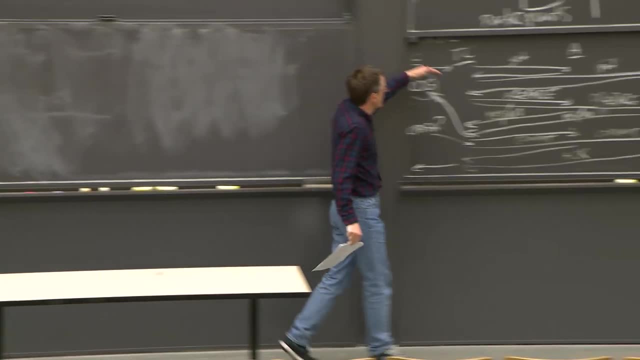 We'd only have to wait for a majority. The leader, we'd only have to have a majority of these to be up in order for the transaction coordinator to do its work, And of course they would all then, you know, sort of execute through the various stages. 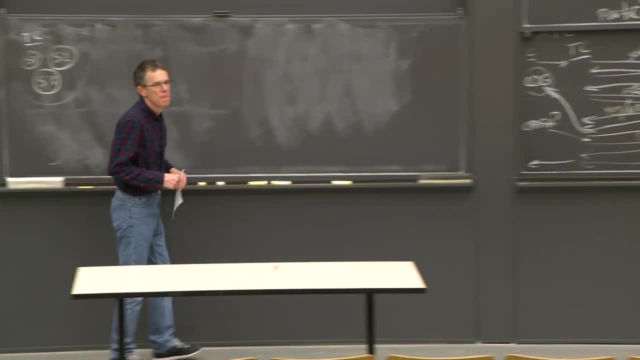 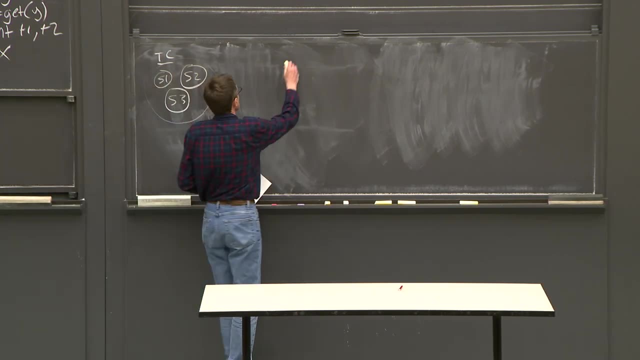 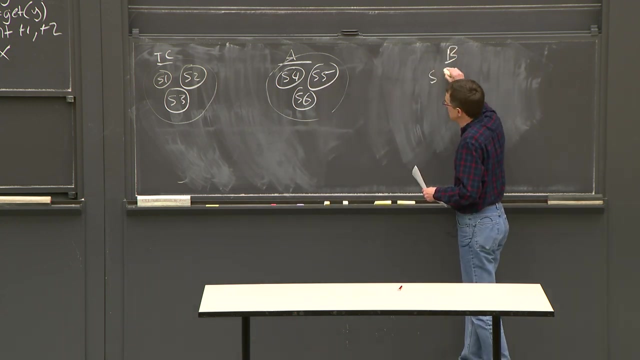 of the transaction and the Two-Face Commit protocol by, basically by appending relevant records to their logs, And then each of the participants would also be a cluster of Okay, Okay, Evaluate API, Araft replicated cluster. So we would end up, and you know, they would exchange messages back and forth. 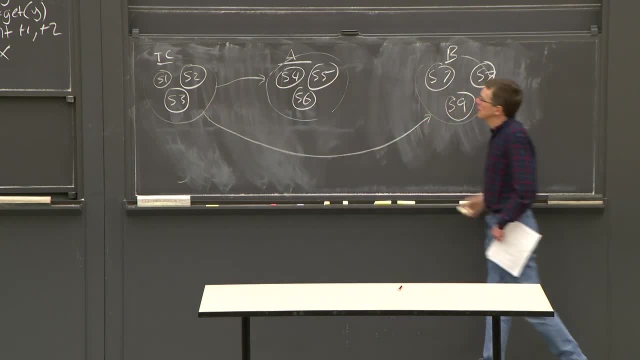 You know we'd send a commit message from the replicated transaction coordinator service to the replicated A server and the replicated B server Exchanged messages back and forth. You know we'd send a commit message from the replicated transaction coordinator service And this is you know.